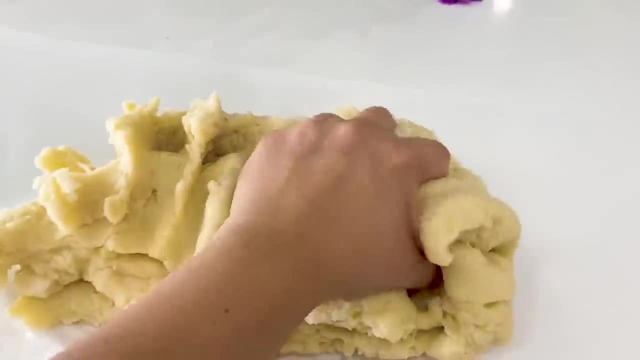 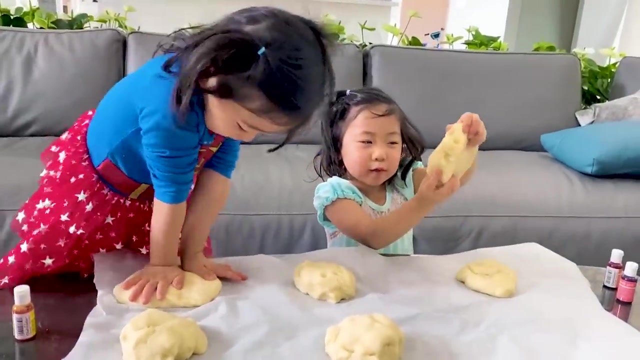 kneel the dough like the bread, So just keep doing it until it's smooth. Whoo, I got all the Play-Doh out and my cake's going to test it. Does it feel like Play-Doh? Yeah, Mom, I want to stretch these. 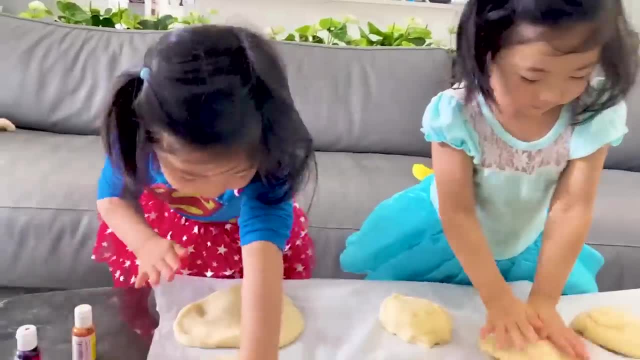 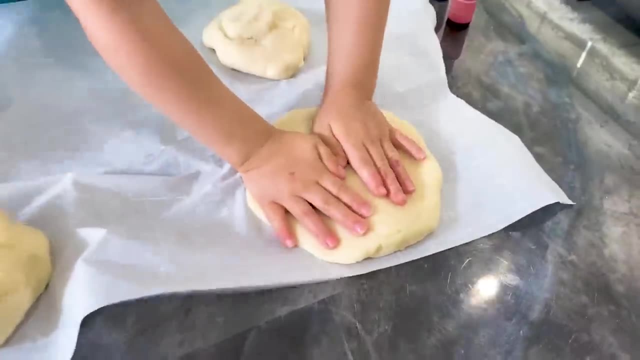 Yeah, like Play-Doh. Well, it's like a pancake. Make it like a pancake. Okay, Emma wants to make each one like a pancake. Good idea, Oh, love it. I want to make mine like a pancake, Okay. 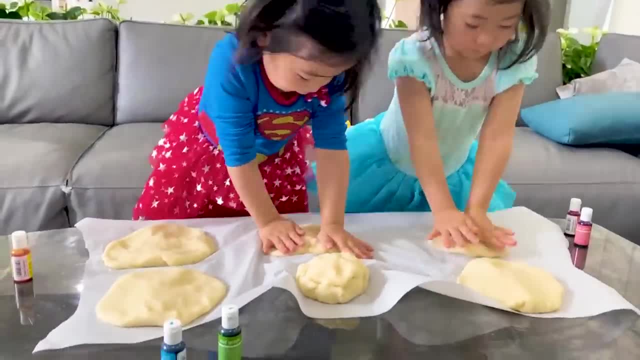 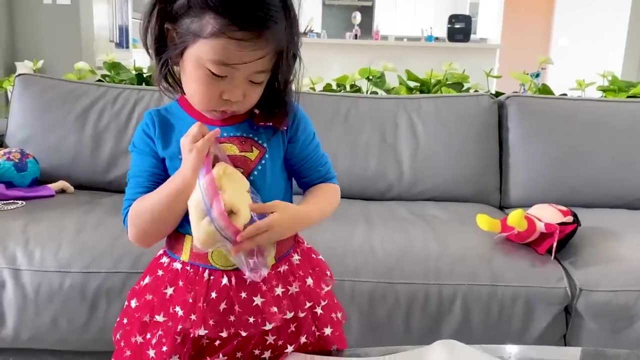 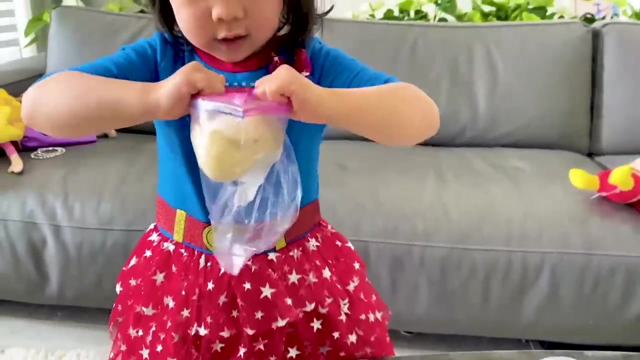 You do this part. Next step is to flatten it out like a pancake. Emma says: There you go. We're going to put each one in a Ziploc bag. Emma's helping me right now. Good job, Emma. Yeah, There you go like that, Good job. 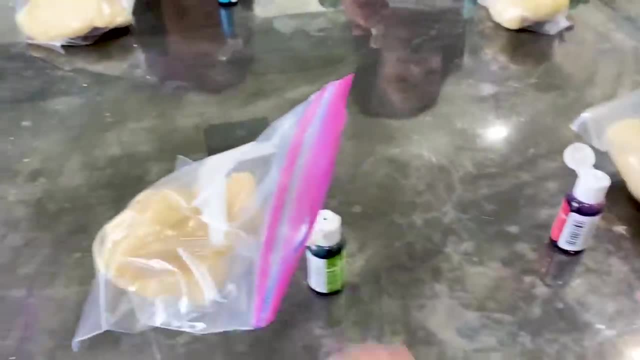 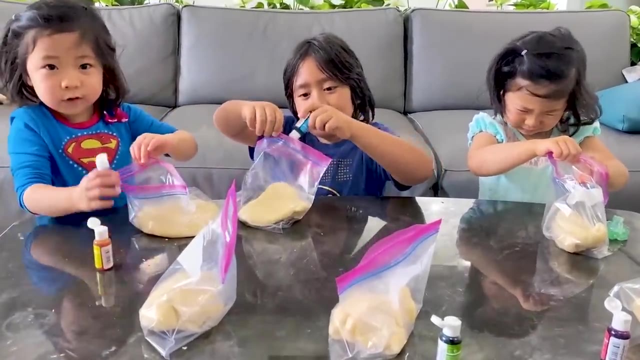 So now we put each one in a Ziploc bag, Then we're going to add color to each one. Alright, so go ahead, add the colors. Can I put this one first? Sure, Okay, Only a little bit, Yeah. 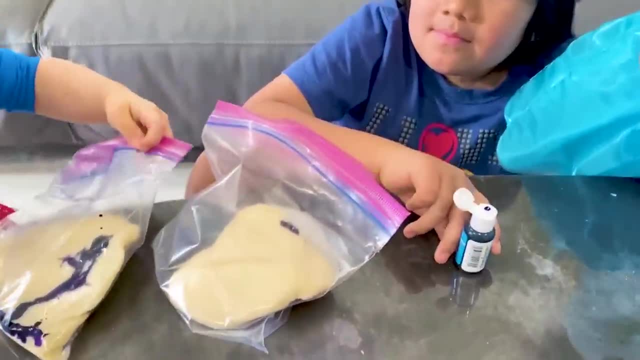 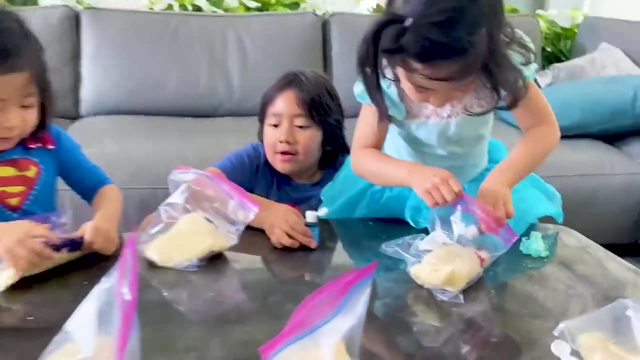 Oh, there you go. So Emma put in purple, Ryan put in blue. You can add a little bit more. Ryan And Kate add in pink red. There you go, Mew it together on the outside. There you go, like Emma. 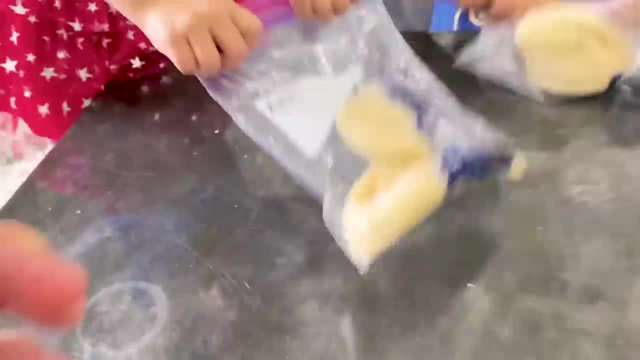 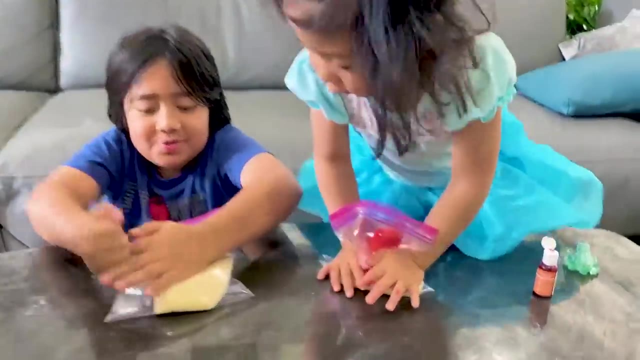 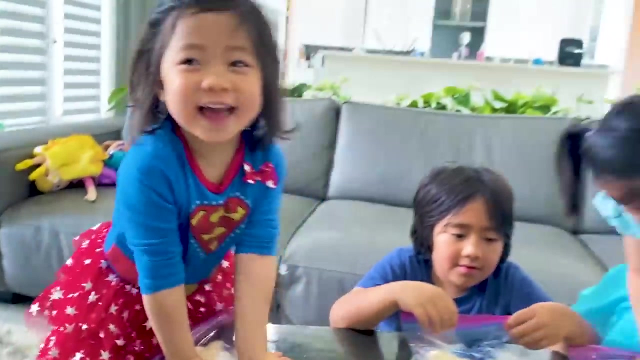 Not shake guys Like this, Like this, Just mew it like that. There you go, There you go, Good job, Kate. Yeah, There you go. Good job guys. Make a pizza, Make a pizza, Make a pizza. 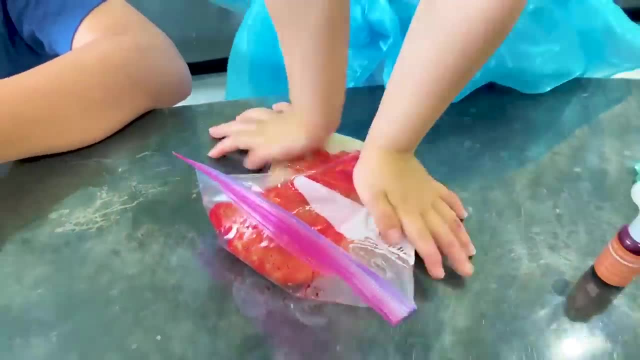 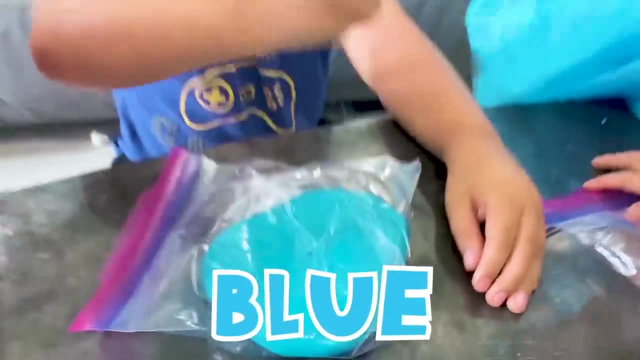 Feeling it like a pizza. That's right, Emma. Yours is almost done, Kate. Good job Emma. you too. Good job, Emma. Keep going, Guys looking good already. Look It's purple for Emma, blue for Ryan. 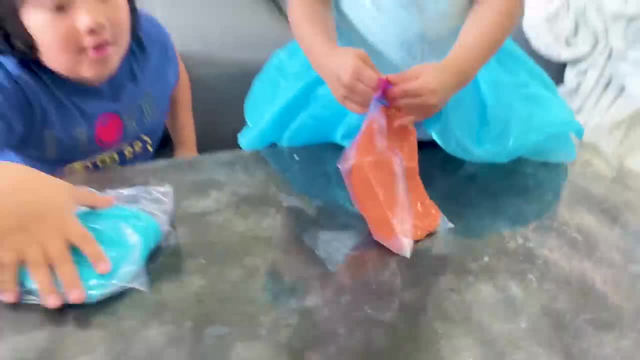 And then I thought it was pink, but Kate was doing orange. Yeah, looking good, You guys can take it out now. Actually, it feels like Play-Doh, Does it? Yeah, Homemade Play-Doh, We made it ourselves. 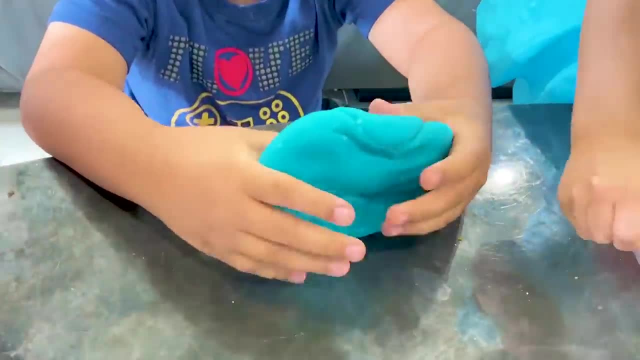 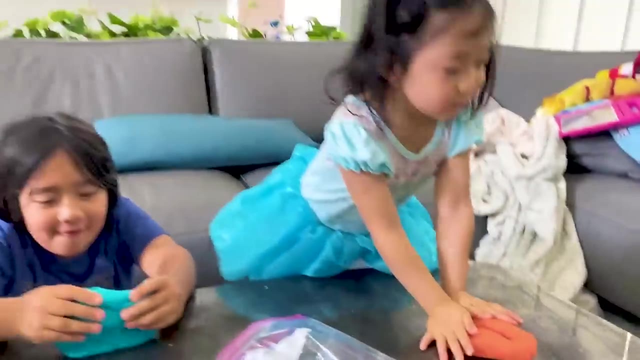 Is this already Play-Doh, Yeah, Or is it something we need to add? Nope, It's already. Play-Doh, Wow, Play-Doh, Play-Doh. It's cool, It's cool, Yeah, I like this Play-Doh. 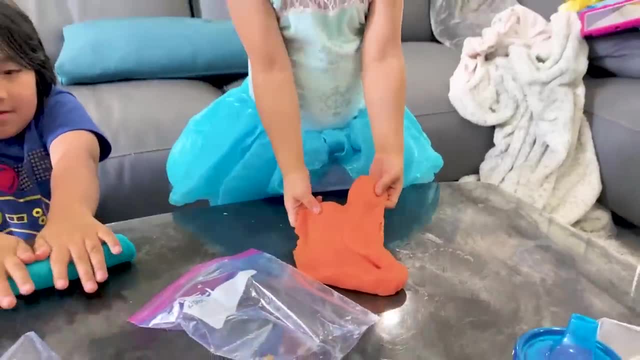 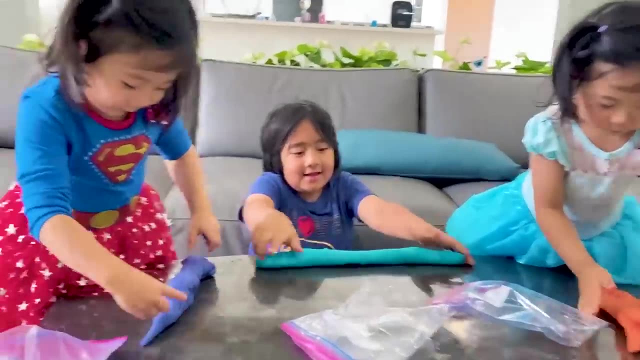 Did you bake it? Yeah, I did, We baked it. I bake it, but you guys made it too. You guys helped me. Good job, girls. Wow, Ryan, You guys make super long. I'm making Play-Doh. 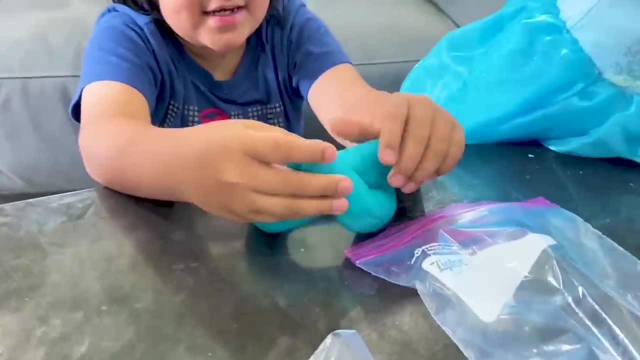 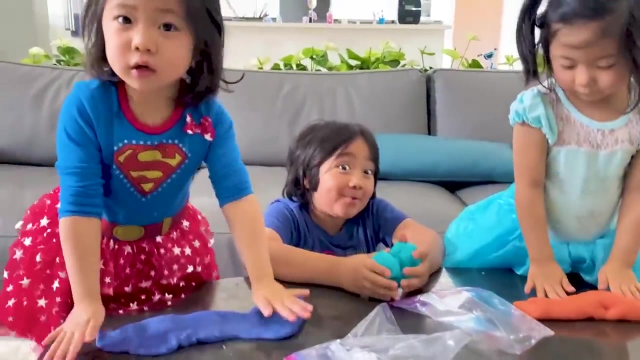 I know I'm going to do whatever this is. What is that? Mom, can you buy me a roller or something? Oh, you're Ryan. Next time I buy you a roller, Good idea. And then cutters- Homemade roller. 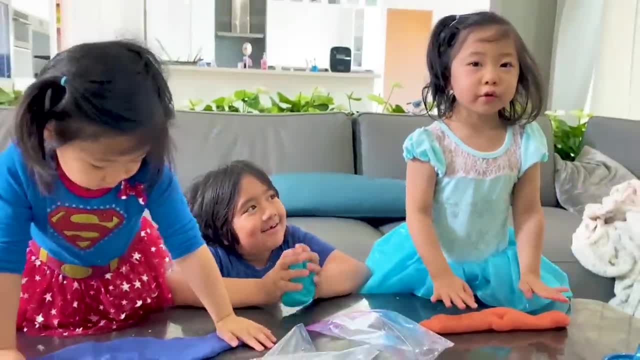 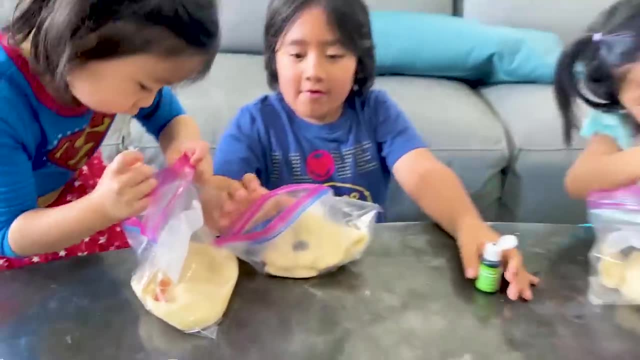 Yeah, Oh, homemade roller. What about cutters? You're Ryan. You need to buy roller and cutters for next time. All right, we're going to continue making our Play-Doh. Emma's putting in yellow, Ryan's putting in green. 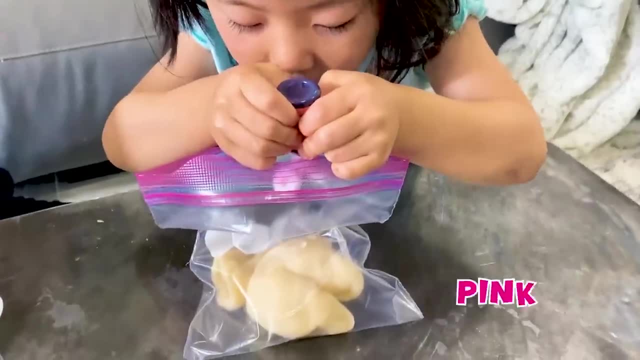 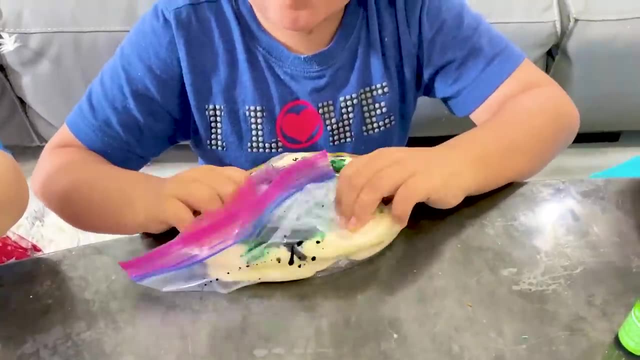 And then Kate's putting in pink. Good job, Kate, There you go. I see some color going in there. Nice, Yeah, Yeah, Keep milling it, There you go. Yeah, Oh my gosh, Mine went pretty far already. 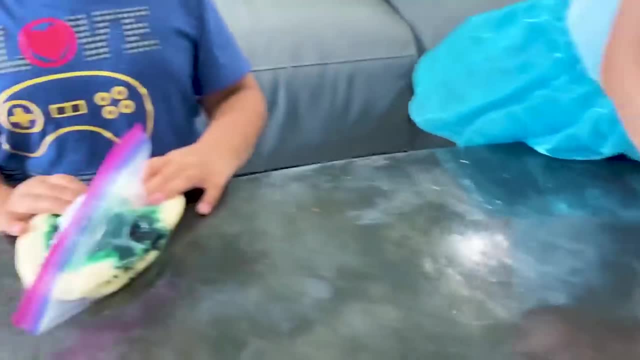 Yeah, There you go. Good job, Spreading it all out, guys. Spreading it all out. Good job, Emma. Emma's looking good too. All right, I'll show you guys the final result when they're done. 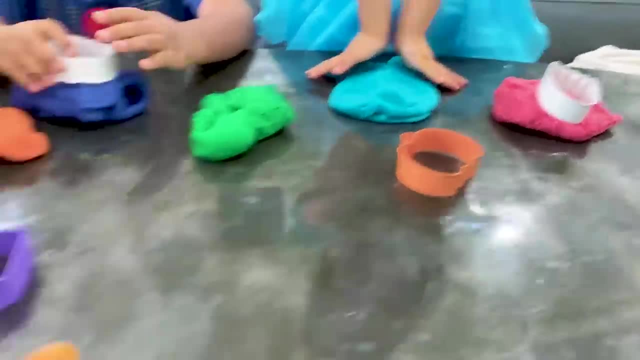 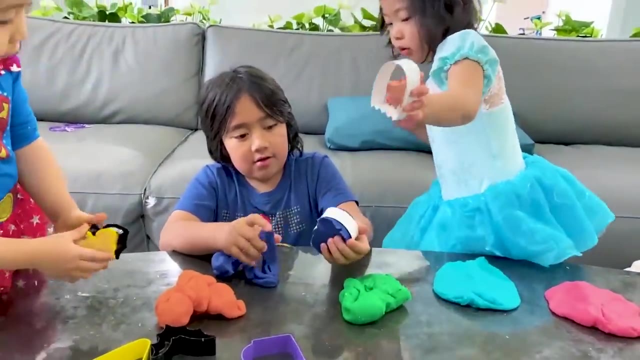 So we got all our colors are ready now. So we have leftover Halloween cookie cutter We're going to use that. You guys can use any cookie cutters if you have it. Mom, this is a ghost. Oh, that is a ghost, You're right. 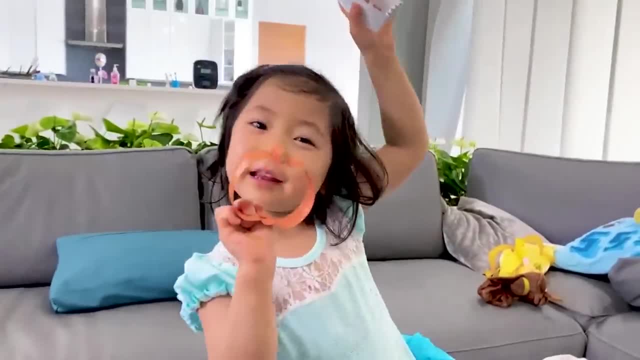 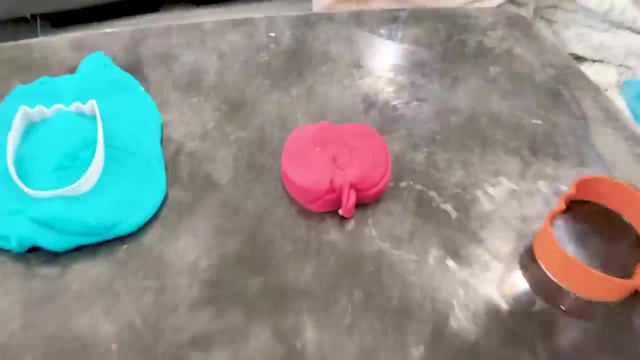 Oh yeah, That is a ghost And this is a pumpkin. That's right, Pumpkin. I see your bat, Emma. Good job, That's a bat. I made a pumpkin You did. Oh, it is a pumpkin, Good job. 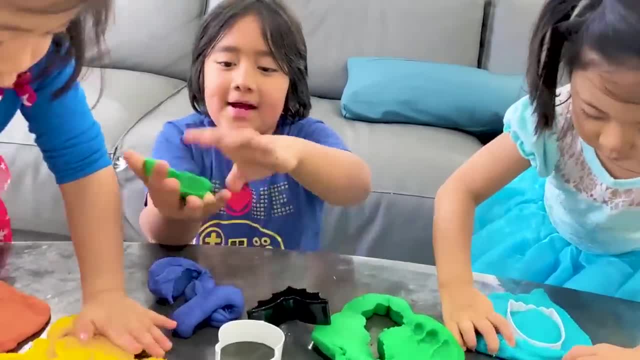 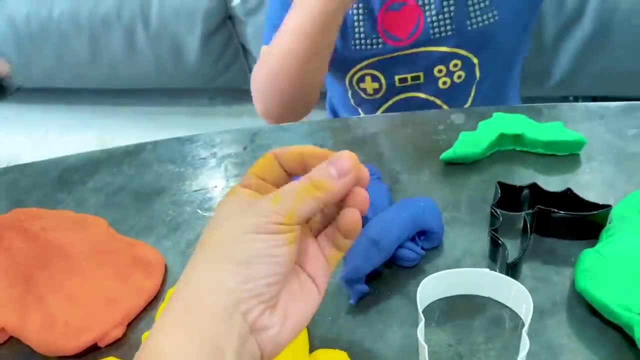 All right, Let me see your bat, Ryan. Okay, My bat is like this. Oh, it does look like a bat. Good job, All I was missing is some eyes. Good, The thing about Play-Doh is you can just get a little thing like this: 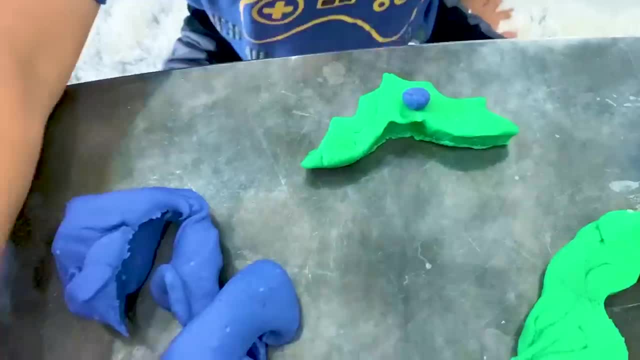 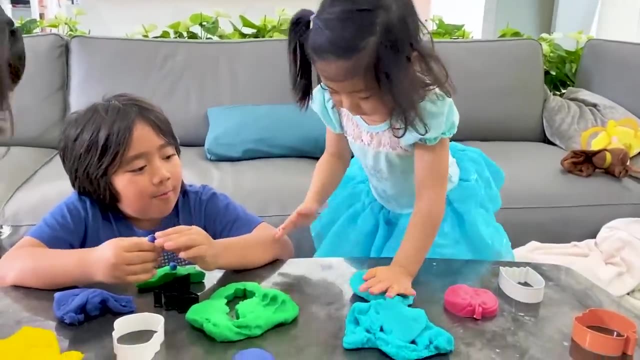 Right, And then you just make eyes. Mom Ryan's bat has a giant one-eye bat. Yeah, Can I smash it and make a bat? Sure, You can smash it. Oh, Kate smashed her bat. What are you making, Emma? 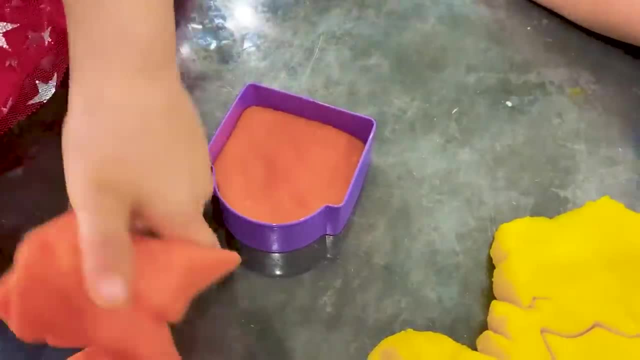 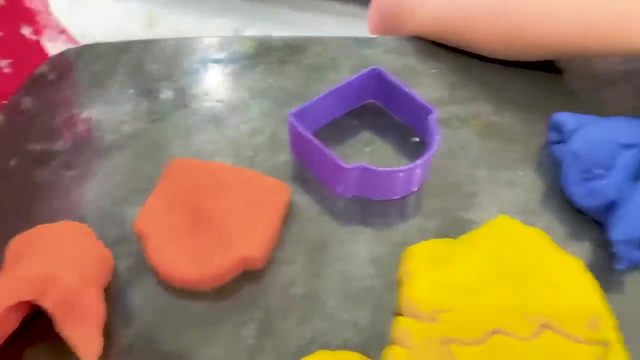 I'm going to make a house. Oh, it's a house. I'm going to make a cookie. Love it, Because I'm making a cookie, A cookie house, Yeah, Wow, Oh, look, Ryan made a face, Love it. 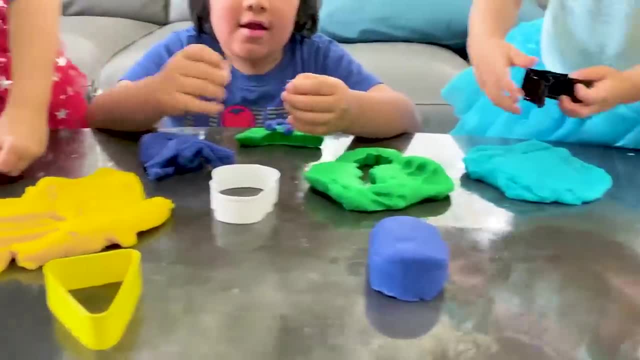 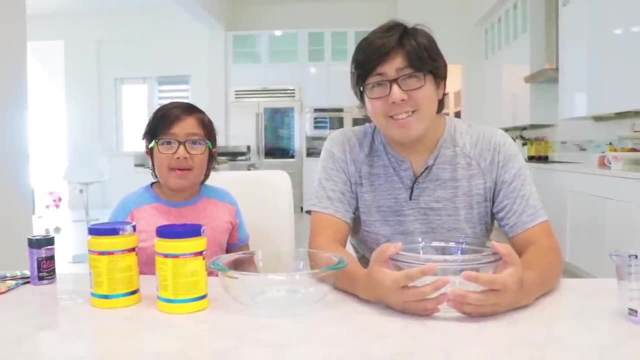 There it is, guys. That's how you make a do-it-yourself Play-Doh, Yeah, And when you're done, you can just put it in a Ziploc bag and save for later, Right, Yeah, Hi guys, Today we're going to be making oobleck with cornstarch and water. 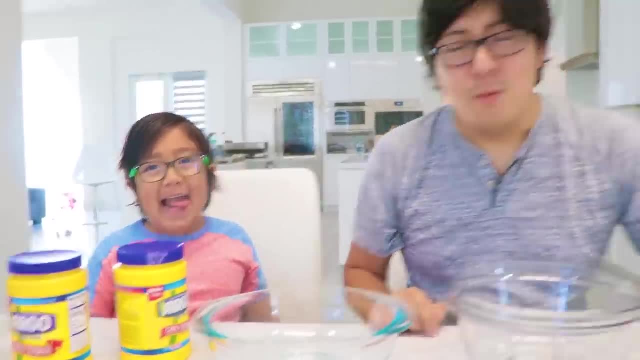 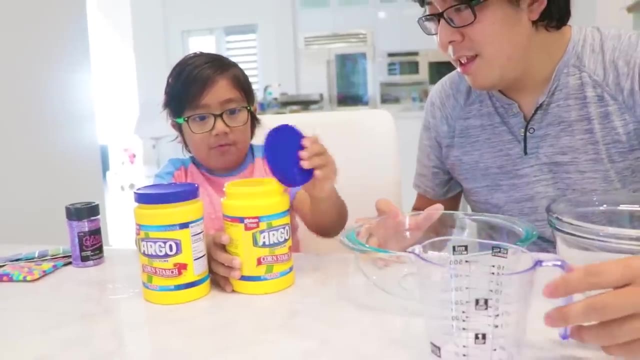 Whoa, First ask a grown-up for help, Which is me All right. So first we need one and a half cup of cornstarch. Okay, Ryan, open it up, Start pouring in here. Good, More, more, more. 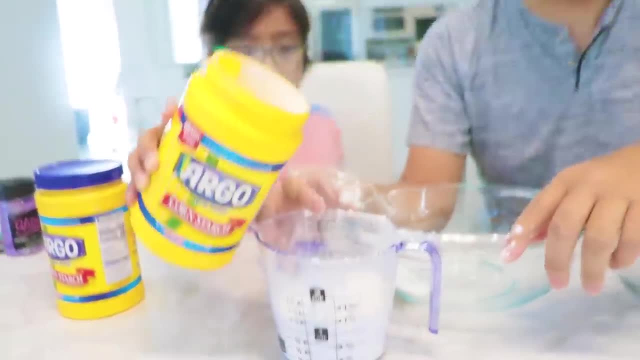 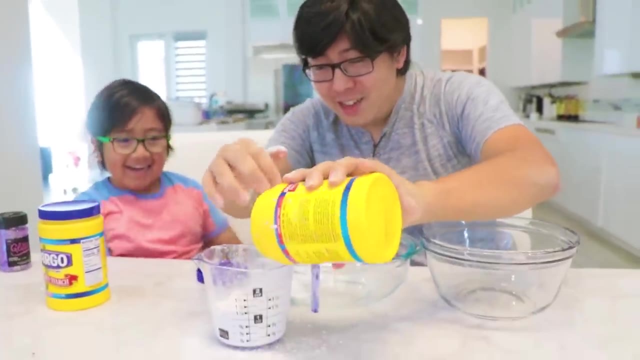 Do you see the line where it says one and a half? Oh, Ryan, Too much. This is why you need help from grown-ups. It's okay, It's okay to be messy a little bit. You tell me when. Okay, Ryan. 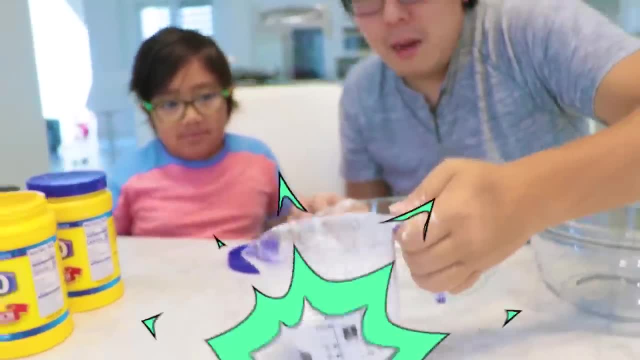 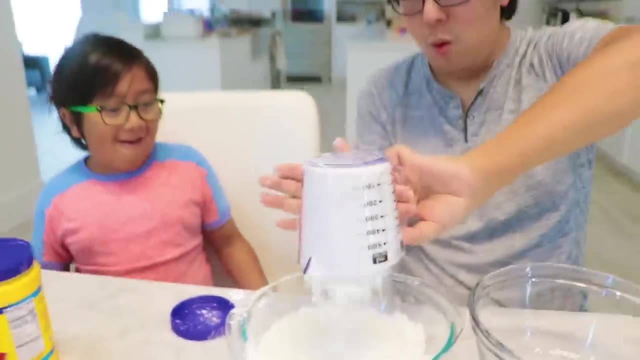 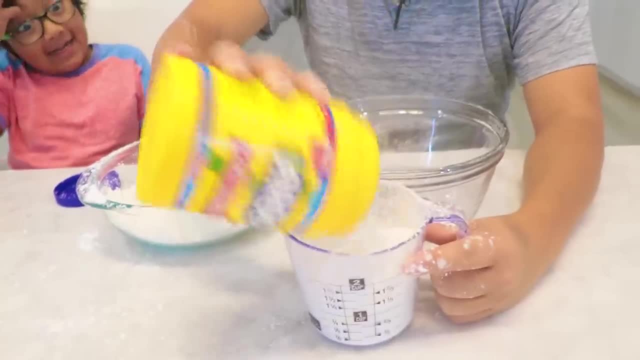 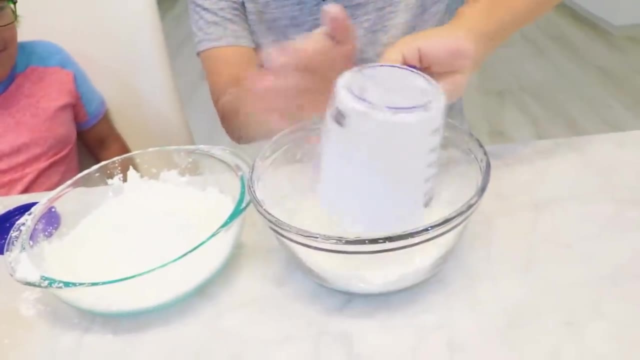 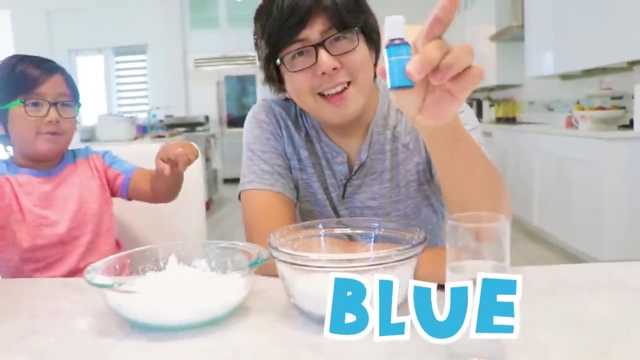 For me. I'm going to do the same thing. Wow, It's finally like flour. Yeah, You know never to eat anything when you do an experiment. Next, measure out one cup of water. I'm going to use green and Daddy's going to use blue. 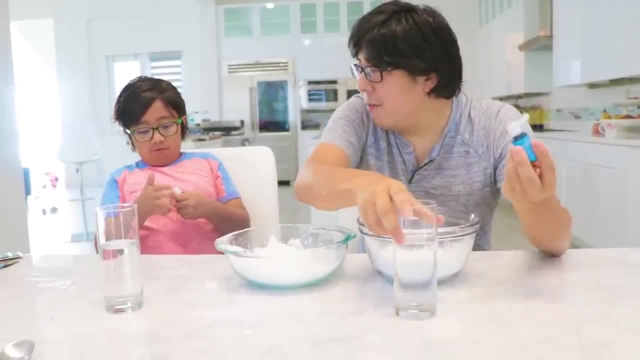 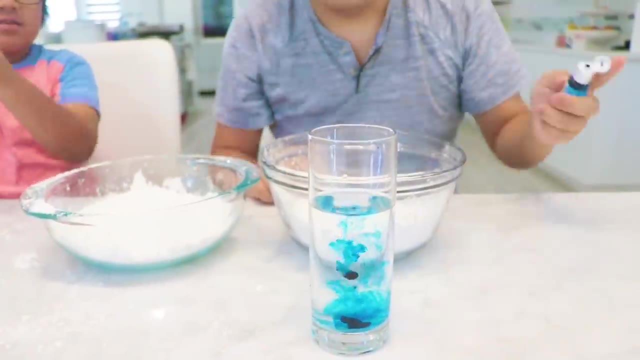 All right, That's my favorite color. Okay, So probably three drops is enough, Ryan, Yeah, If you do too much it's going to be too dark. So one, two, three, I think that's good. 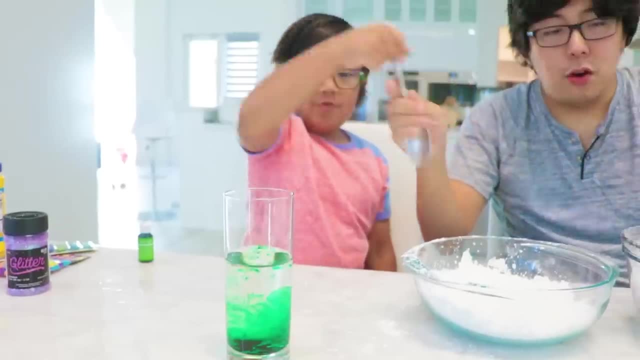 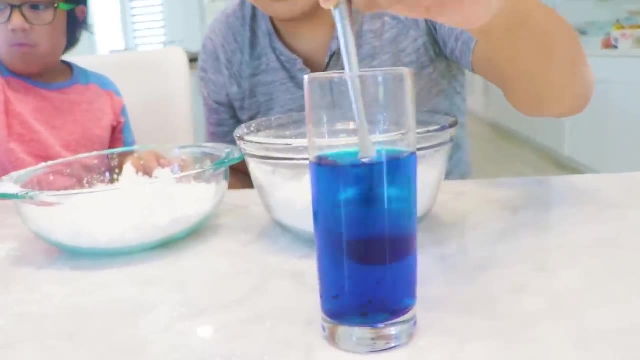 All right, One, Oh, That's good, That's good, Just stir it, Yeah, Whoa, Look at that, Mine's definitely blue color. Whoa, How's yours going? Oh nice, It's green. Next, put the water into your corn starch. 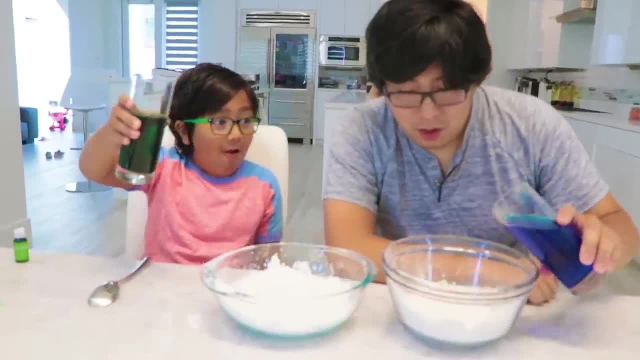 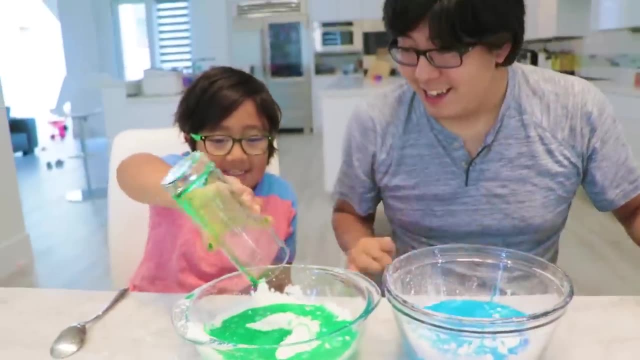 All right. Whoa, Whoa, It's looking good. Whoa, The color came out. nice, It's like a volcano. Yeah, All right, I like it. All right, Now we got to mix it up Oh. 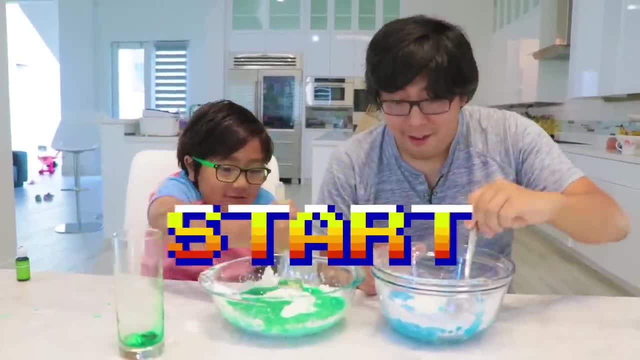 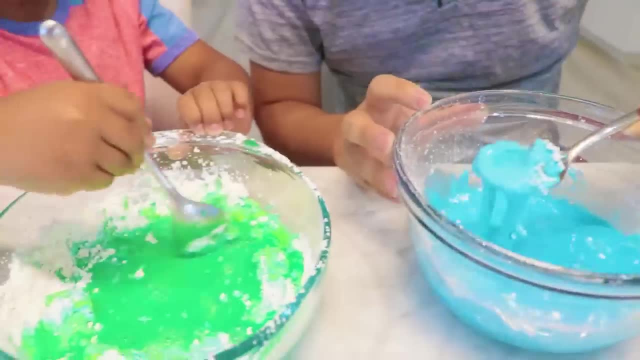 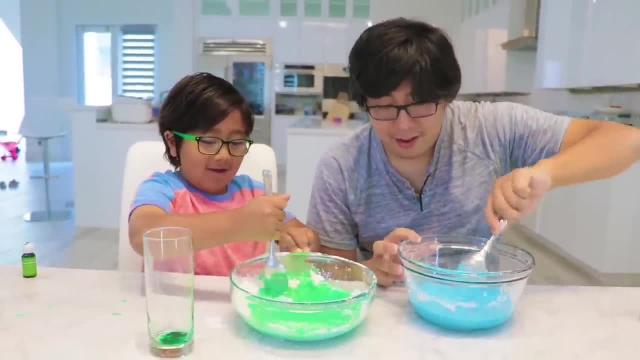 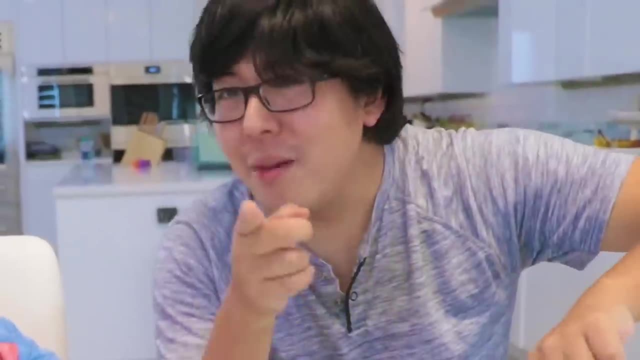 Yours looks like soup. It looks like slime. Yours looks like a slime color. Yeah, Oh, It smells so good. If you guys like messes, you should definitely make oobleck, But don't make a mess intentionally, okay. 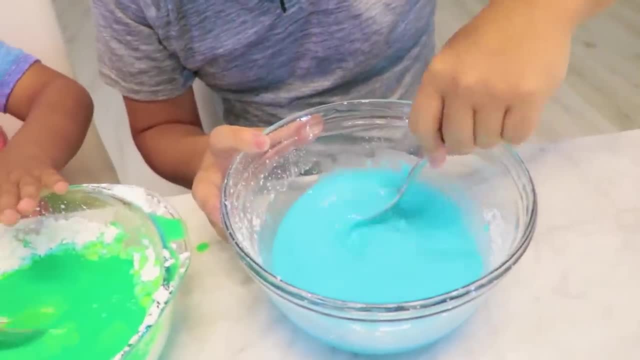 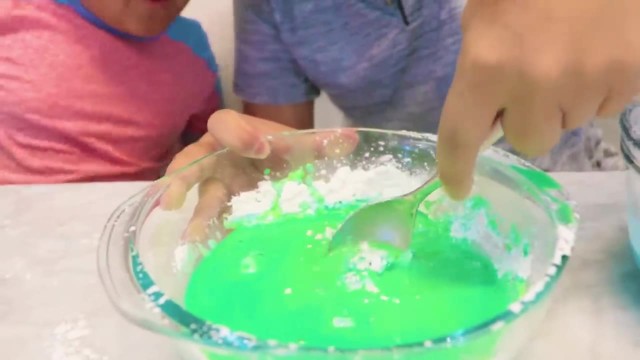 Don't do that on purpose. It's all dissolved. I don't feel anything anymore. It's all liquid. I feel so much. This is why you need the help from the grown ups. Whoa, Whoa, Whoa, Whoa. 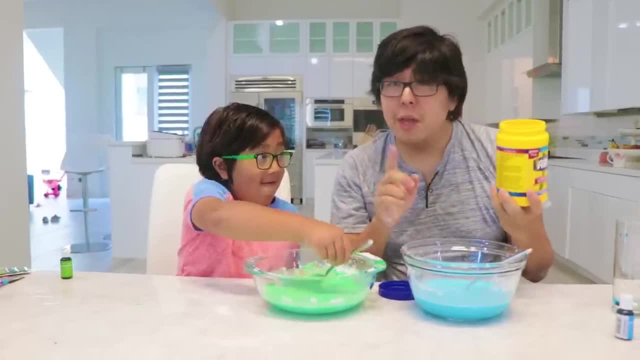 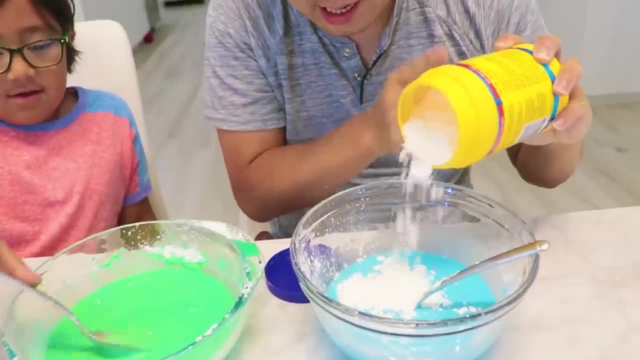 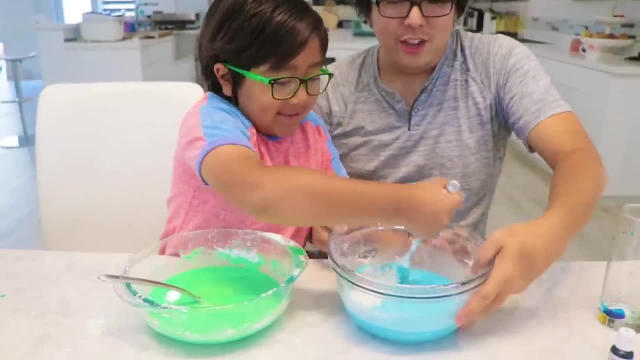 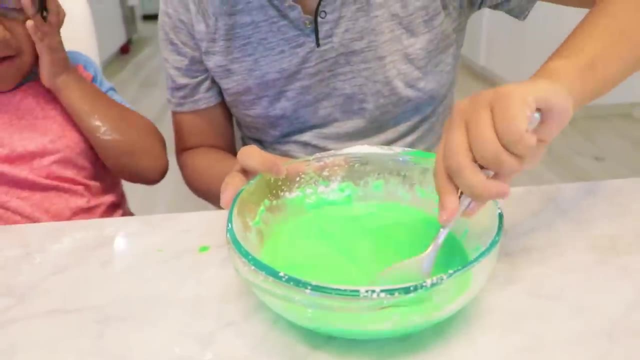 Mine's good, Yours good, Okay, Yeah, I'll just add a little bit. Okay, That should be enough. All right, We exchange Here, You help me and I help you. Here you go. Oh yeah, Ryan needs a little bit more too. 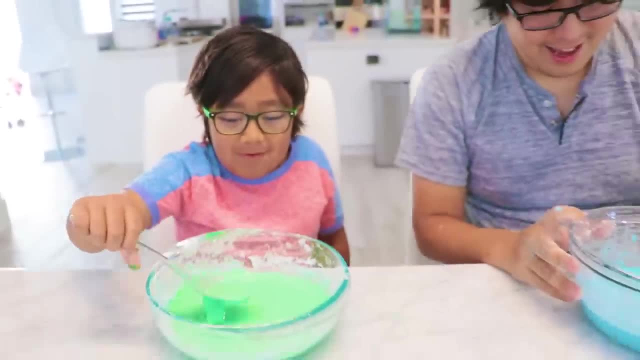 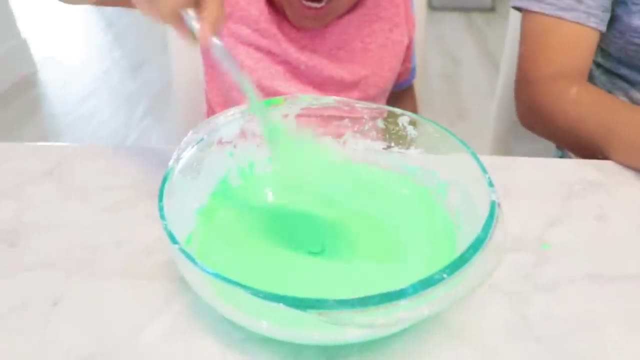 Look, It's very liquid. That's definitely ready, And mine too. look at this: It looks liquid, right, Slap See, you can slap it. All. right, Ryan, why don't you try and touch it and see what it feels like? 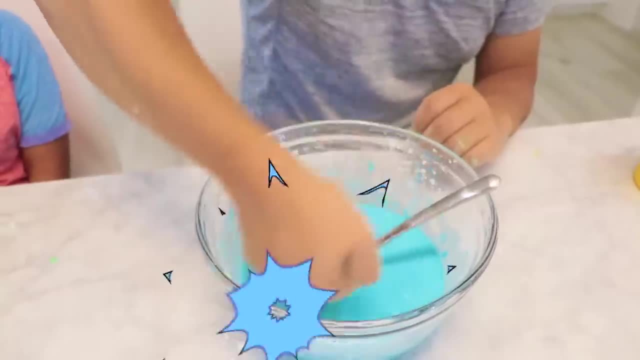 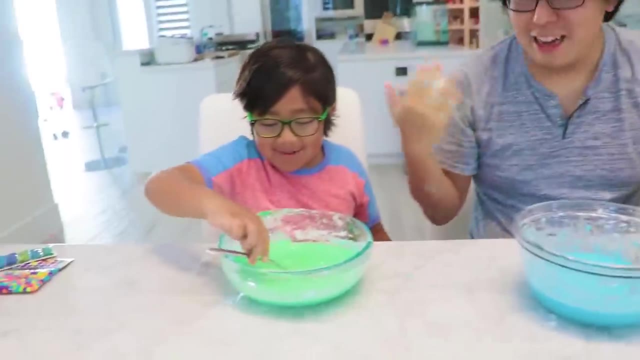 See, if I try to slap it, I can punch it. see, My hand doesn't go in. Look, Ah, I can't punch through What? Let me try. let me try See What? So it's like slime, like that. 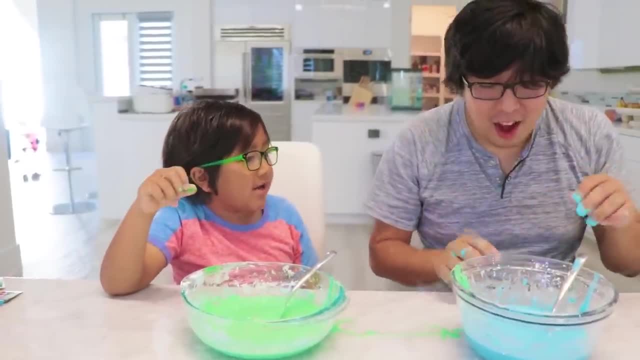 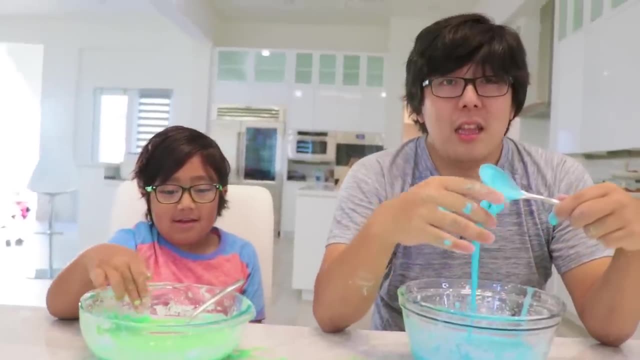 It's kinda like slime, It's like concrete. It's like slime that's not ready yet. Oh no, I dropped mine, mine, mine, no. So, guys, I have a question for you. What Is this Oo Black? is it a solid or is it a liquid? 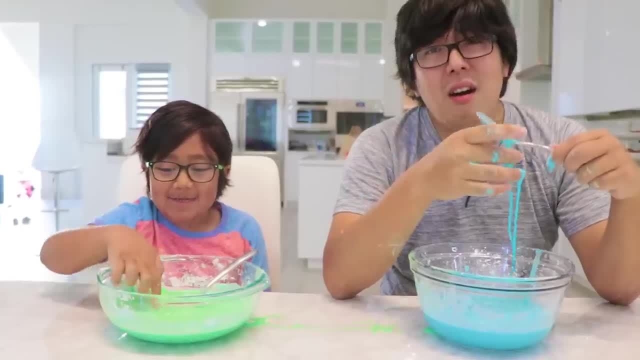 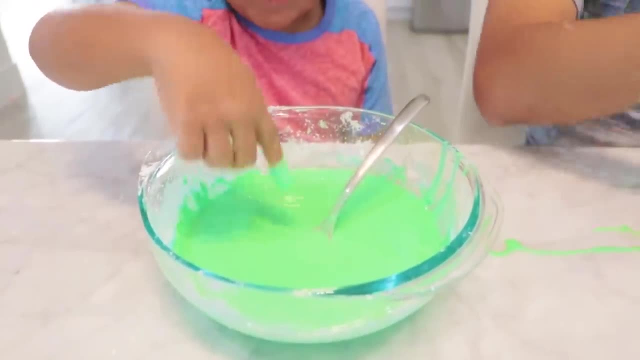 It's both. Why do you think it's both? Because when you stay still in it, it like sinks you down and whenever you hit it, it's a solid. It's a solid, So it's like invincible. Oh, I don't think it's invincible. 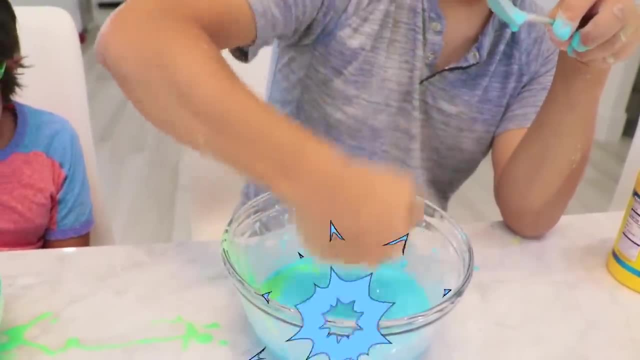 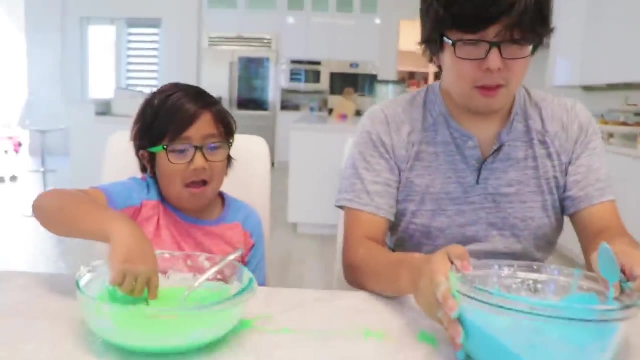 but yeah, I feel like it has both properties. This is like: look, it feels like solid, right, But then see It moves like liquid, Yeah. so I want you to pick up some and put it and squeeze it between your hands. 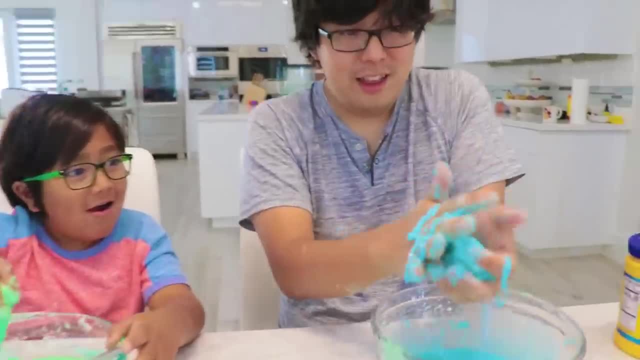 Ah, Does it feel hard or soft? It's hard. Yeah, when you put it in your hand it feels hard like a solid. I'm making a ball, right. Yeah, I'm making a ball. Let go, let go. 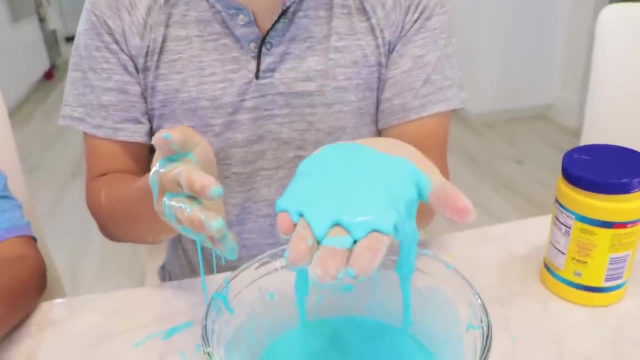 So that's like a solid. Oh Wait, wait, wait. Why can't you let go? It's liquid. Yeah, I'm so confused. which one is it? All right, you try, Ryan, It's both, obviously. 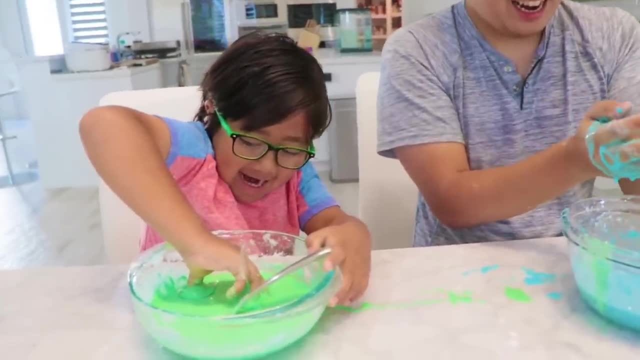 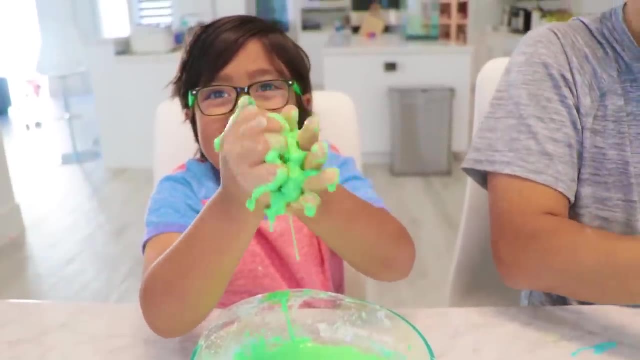 Ah, seven years old, it's teaching me. You try, you pick up a whole bunch and then just squeeze it, don't leave any space. Does it feel like a solid or a liquid? Solid, Yeah, but if you let go, 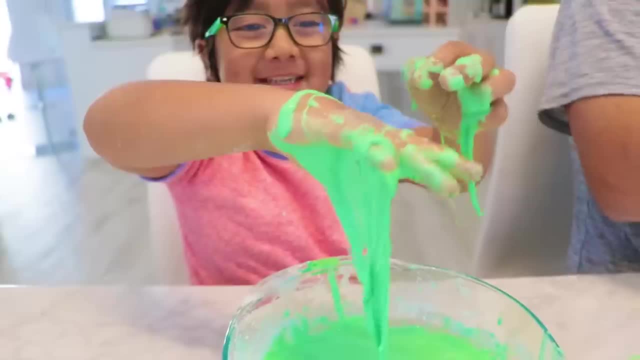 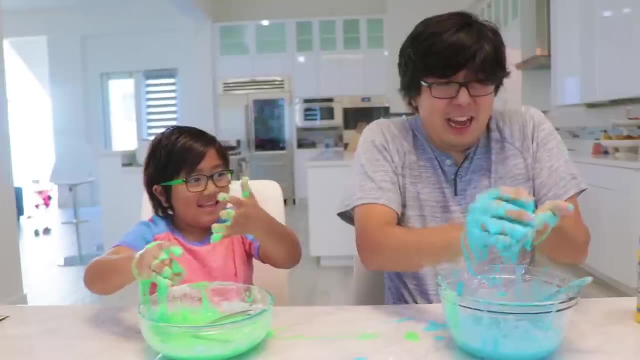 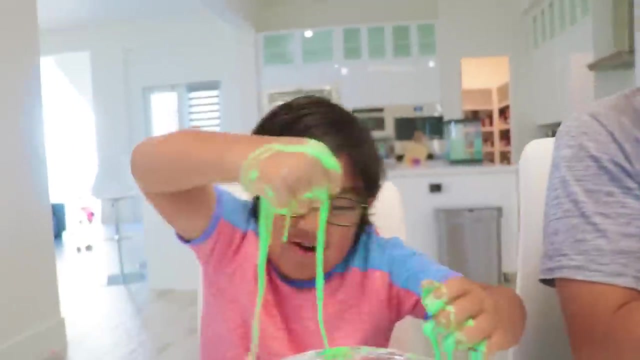 Oh, What happens? It becomes a liquid. Yeah, so it's not your typical solid liquid, right, Right? So if I want to keep it solid, I have to do this forever. Yeah, Ah, it's melting. I'm getting mad. 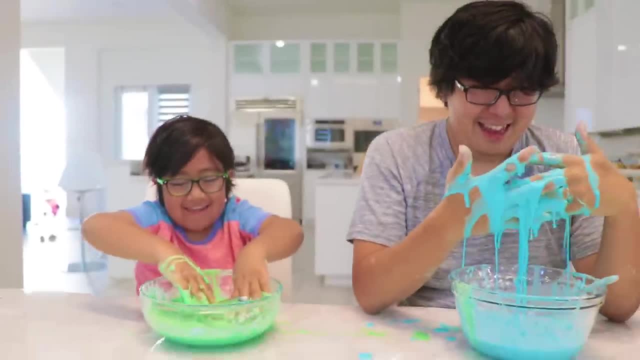 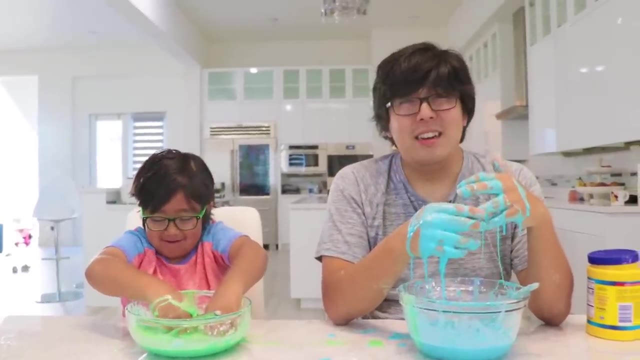 Ugh, Yeah. so this is really cool. This is actually called a non-Newtonium liquid. Huh, Non-Newtonium liquid, That's what it's called. What is Newtonium? Yeah, Newtonium, after so Isaac Newton. 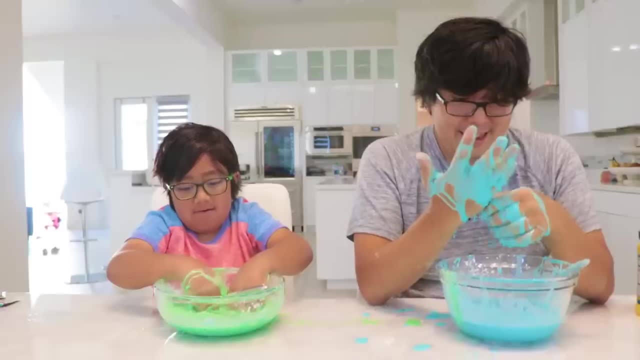 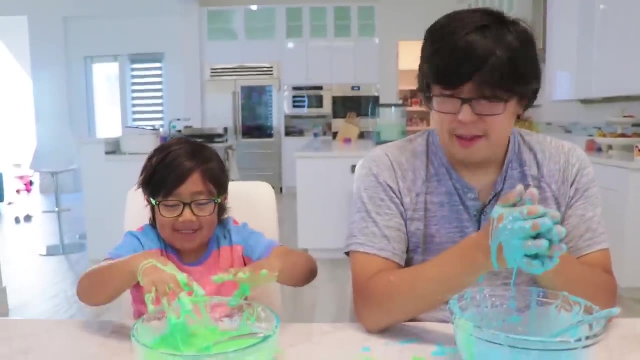 Okay, It's not a typical definition of a solid liquid and gas. It's a solid or liquid and it changes its property based on pressure. So if you apply pressure, it behaves differently. Mommy, you try to punch it, Okay. 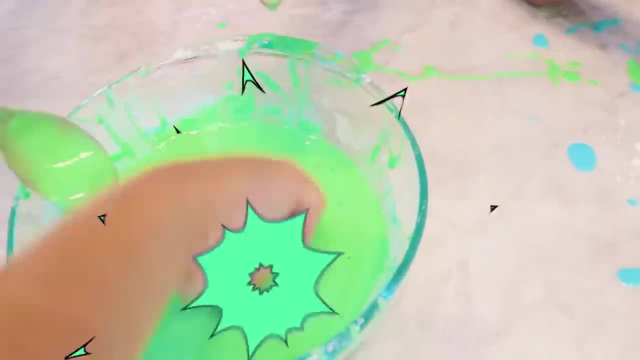 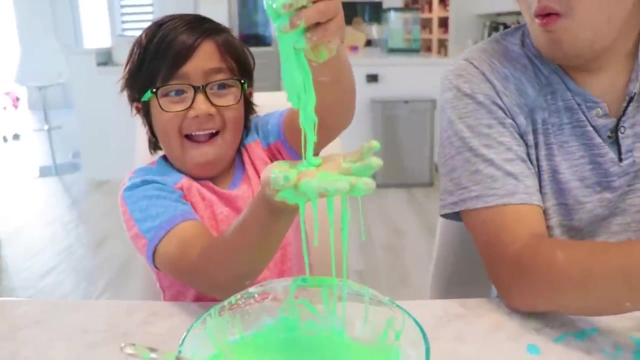 Mommy's gonna try to punch. Let's see. One, two, three, Whoa- I know That's super hard like concrete. That's so fun. Whoa, look at Ryan. If you let go, it just dropped down. 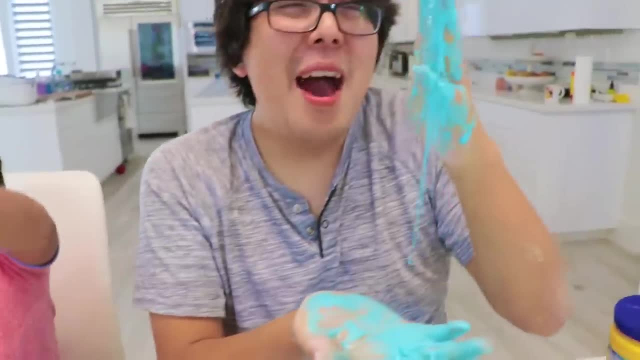 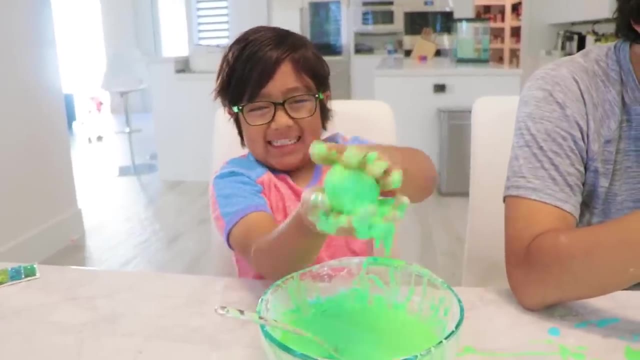 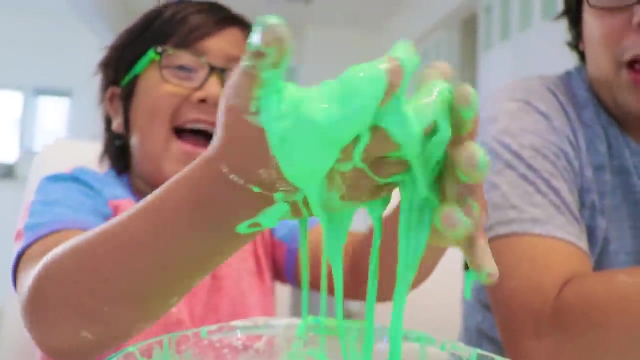 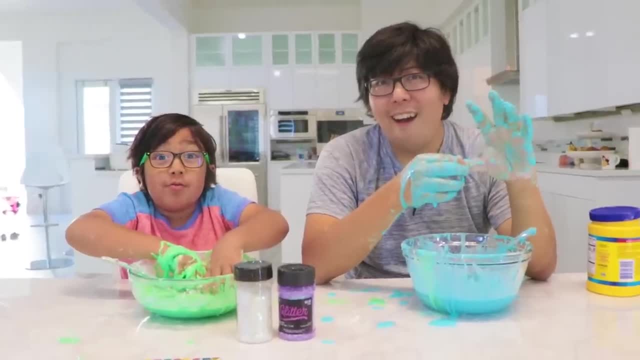 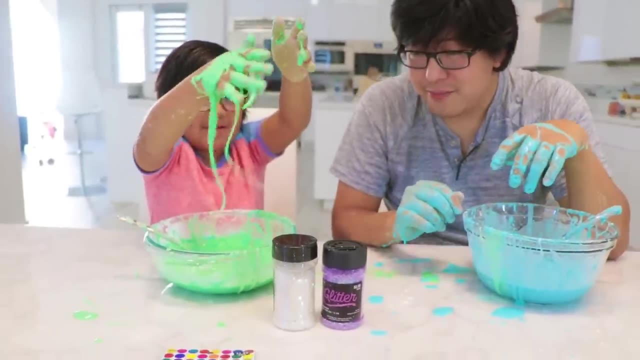 Matcha flavor, Maybe a rocky road. You can make your oobleck even more exciting with adding glitter. Wow, Which one? which one? There are two kinds. I wanna do the bigger one. Okay, I'll get the purple one. 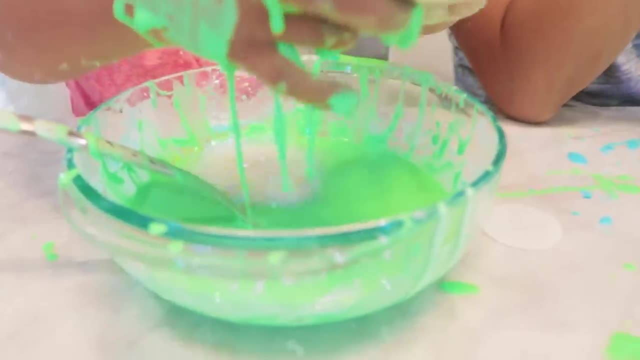 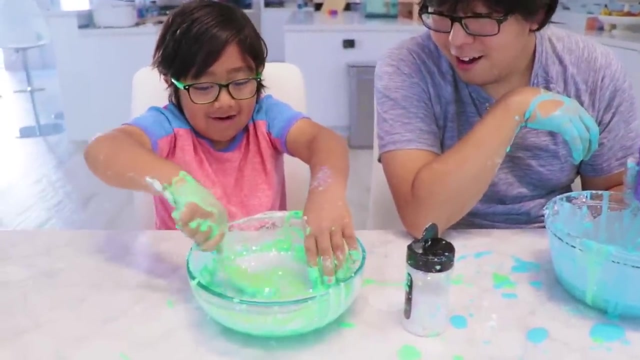 Glitter. Ooh, that's a lot. That's enough, Ryan Shiny. Oh, how am I gonna mix the? Oh Glitter? Oh, it's on your hand now. Oh, This is the only way I can mix it. 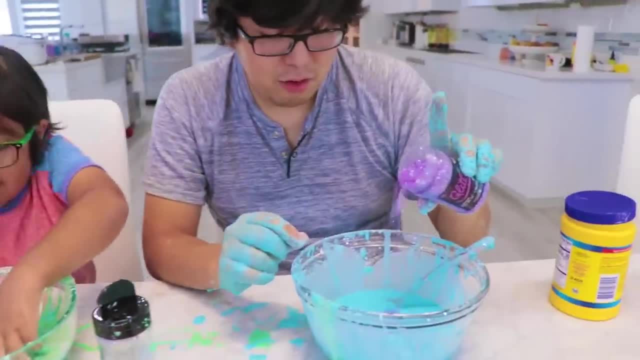 Ryan added way too much glitter. All right, I'll do it right? Well, I need a lot more. I need a lot of glitter. Wow, look at that, I like it. The only thing is it's hard to mix. 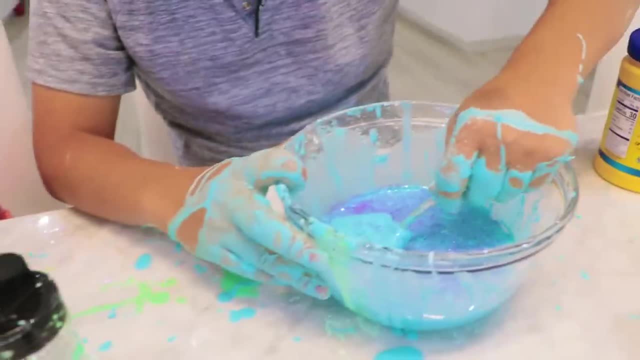 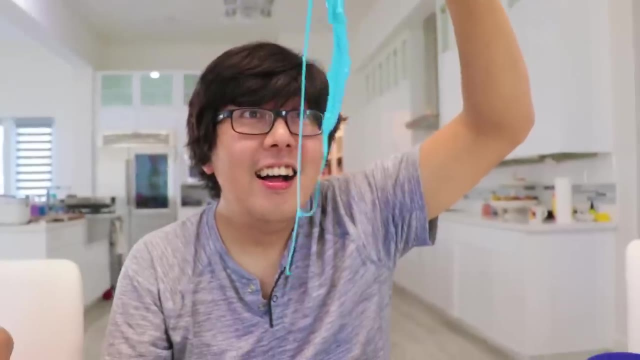 Do you like that? Oh, Oh, Oh, Whoa. But if you leave it like this, it's actually hard to get out. Oh, Oh, Oh, So cool, Okay, guys. so that's how you make oobleck. 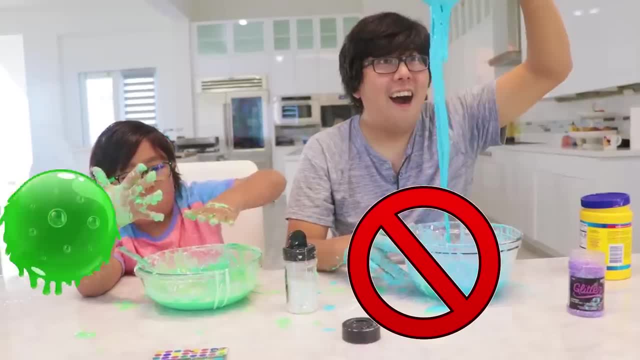 And when you're done playing, just do not throw it into the sink. You know why? Why It could clog up your sink. Oh no, no, no, no, no, no. Yeah, I don't want that. 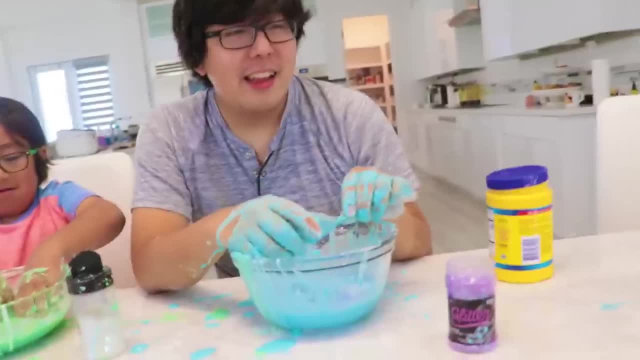 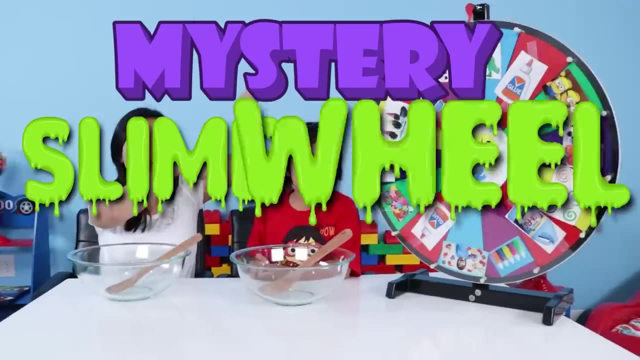 So if you're done playing, you just throw it in the trash, or you can just put it in a Ziploc bag like this. You can play again later. Hi guys, Today we're doing the mystery slime challenge, So it's gonna be Mommy versus Ryan. 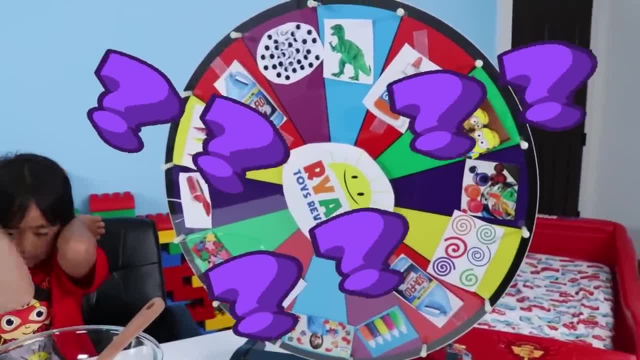 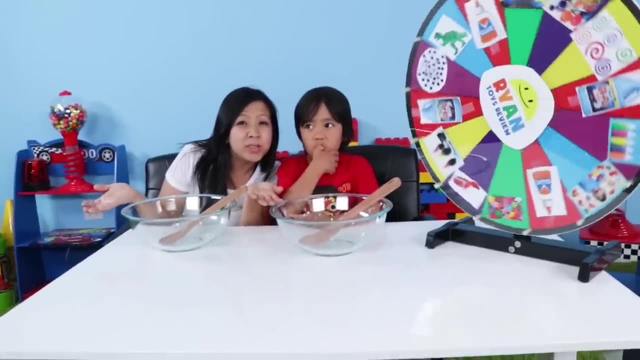 There's lots of mystery ingredients here on the board, So we're gonna spin And whatever we land on, that's what we get. So hopefully we will get slime. We are not sure. Are you ready to get slime, Mm-hmm? 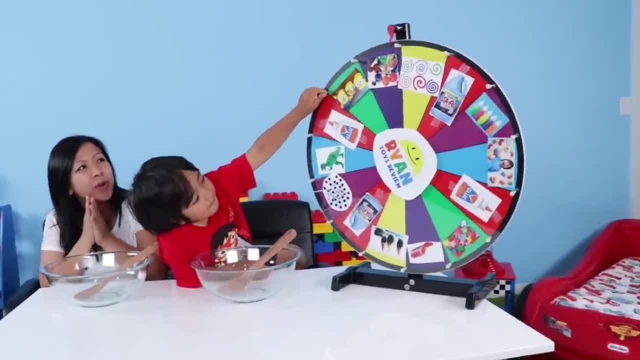 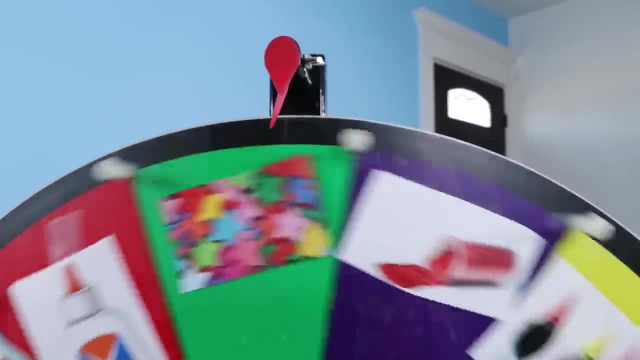 Okay. Okay, Ryan, I'll let you go first. So let's see what we are gonna get. I want glue. I know we're gonna need glue to make slime, So let's see what is the first ingredient. Oh, do I actually get glue? 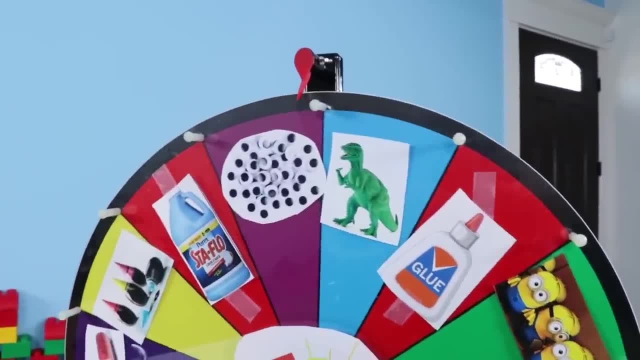 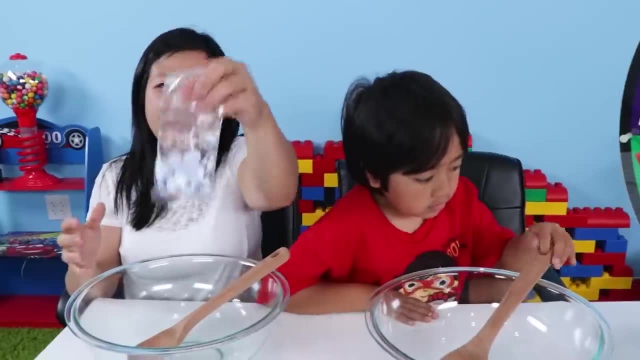 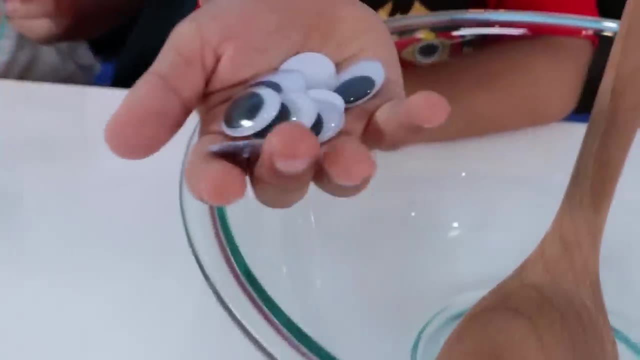 You can trick us. Uh-oh, Put it back, Put it up, Up Eyeballs. So Ryan's first ingredient is eyeballs. All right, Ryan, here's some fun eyeballs. Here you go Some yummy, delicious eyeballs. 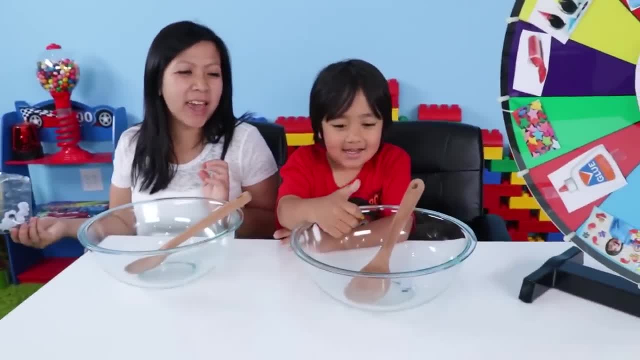 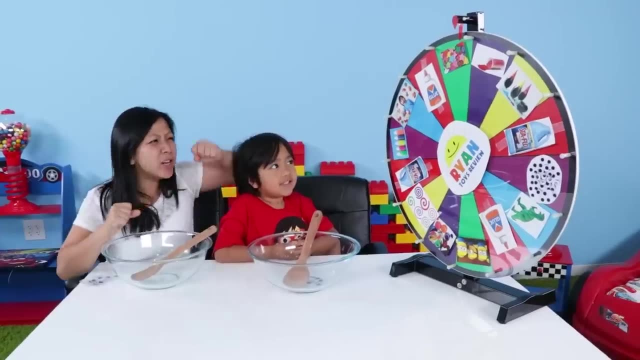 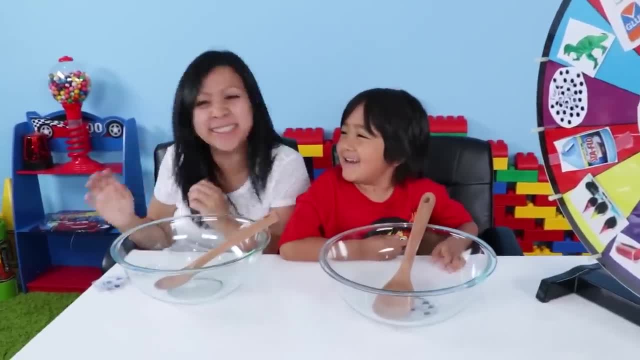 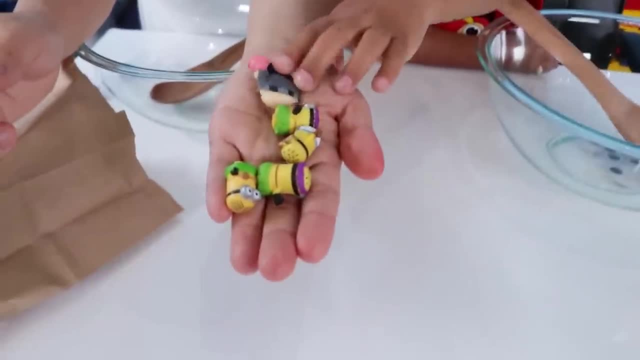 Inions. I guess it's better than eyeballs. Ooh, Let's check out some yummy, delicious Minions. Minions, look at that. I don't know his name. If you know, let me know Drew. 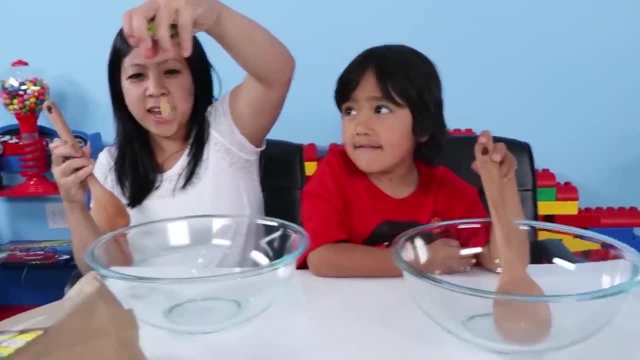 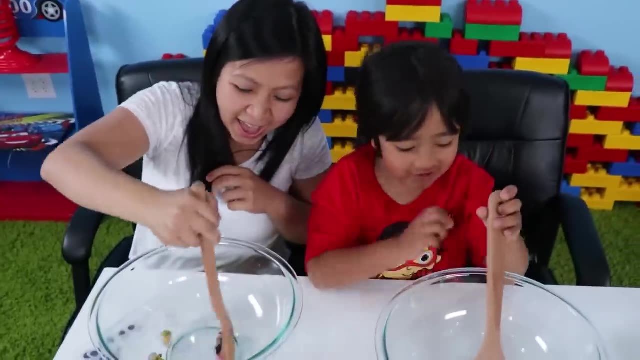 Drew, and Drew too. He gets to go into the slime, Into my slime balls. His brother's name is Drew too, And then I'm gonna mix it up too. Look at them bouncing around in the balls. Okay, Ryan, let's see what is your next ingredient. 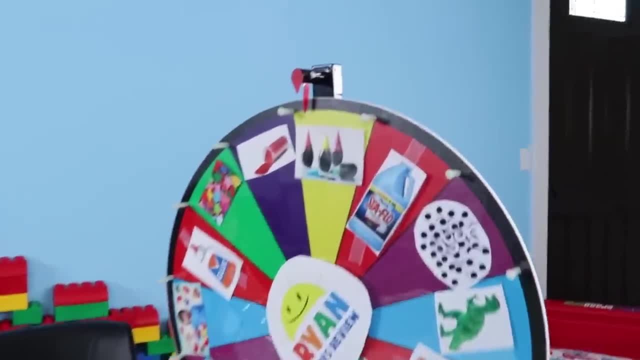 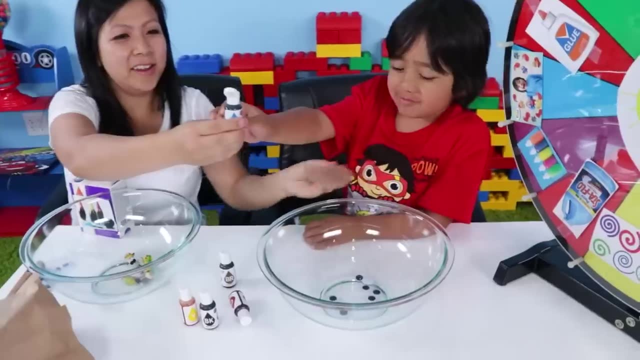 Let's see, Let's see Coloring. Ooh Okay, Ryan, what color would you like? Blue, blue, blue, Oh, blue, Okay, Here you go, Have fun. Ooh Okay, Mix it, Mix it. 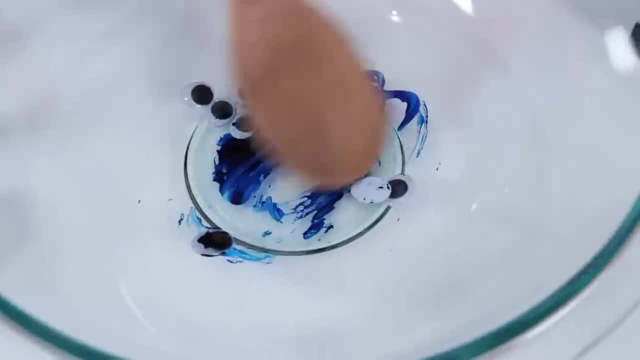 Ah, Slimey blue eyeballs. All right, Mommy's turn. so far, None of us has glue. Do you need that too? Yes, we do. We need the activator. Come on, Glue Ah. 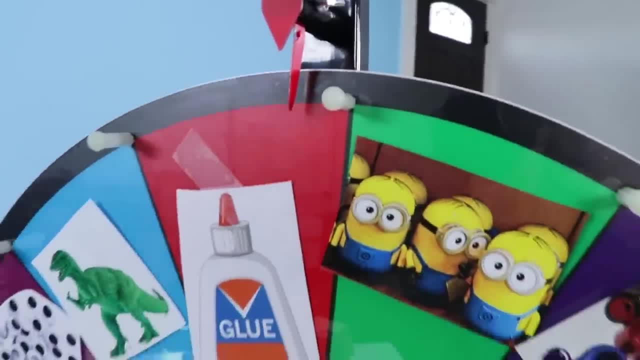 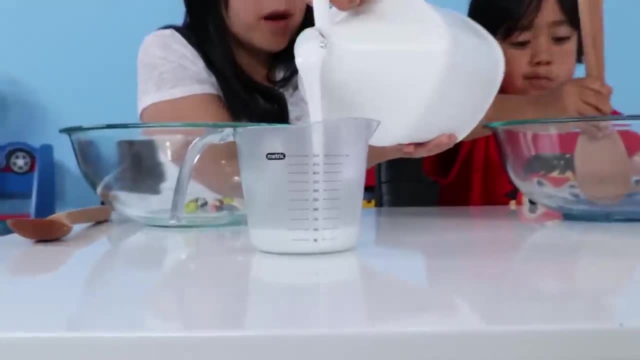 Got a giant container full of glue. Okay, Okay, Okay, Okay, Okay, Okay, Okay, I'm gonna put a bunch of glue here. You can never have too much glue. One half cup of glue. There we go. Now I'm gonna dump it into the Minion. 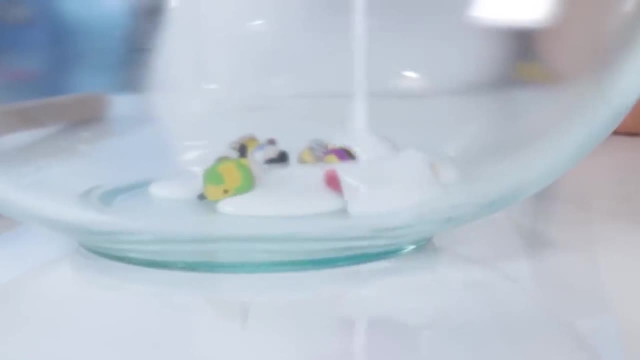 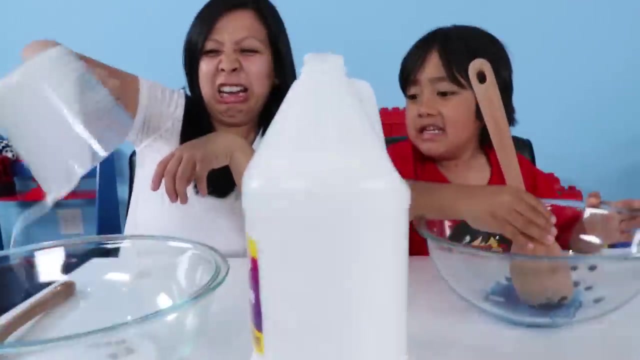 Whoa, look Ryan, The Minion is covered with glue. Oh, Oh What. I'm gonna stir them up. My turn. Whoa, You got liquid starch, So that is also an ingredient to start with. It's cool. 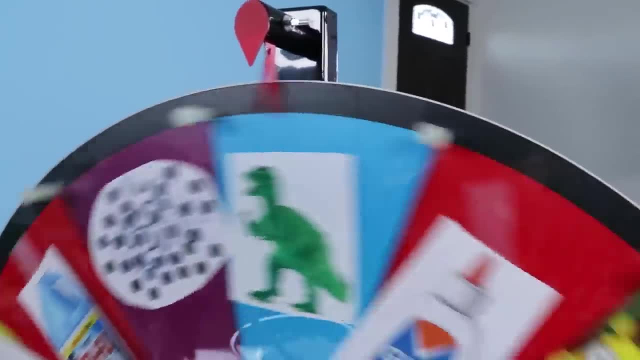 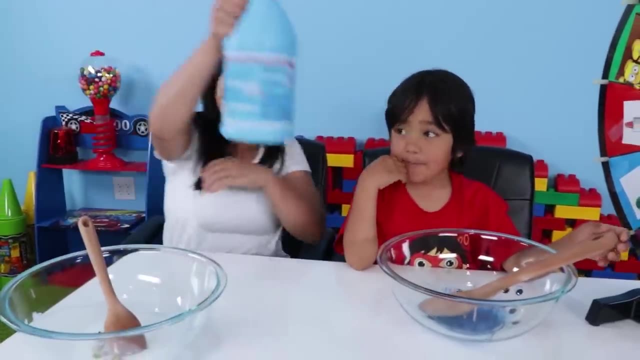 I'm gonna add this in here: Okay, Okay, All right, Okay, All right, All right, Okay, Okay, All right, All right. slime, so that's good. That's a good start. Here's some cornstarch. Okay, so we need one over four. 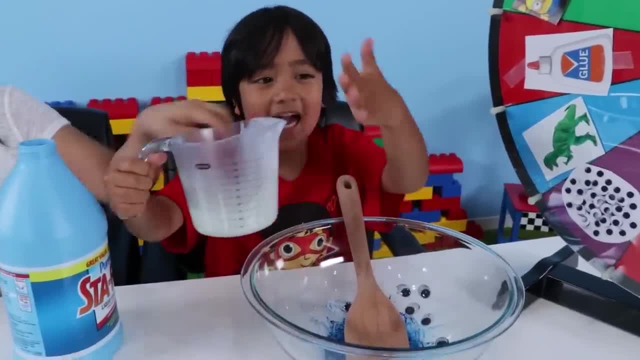 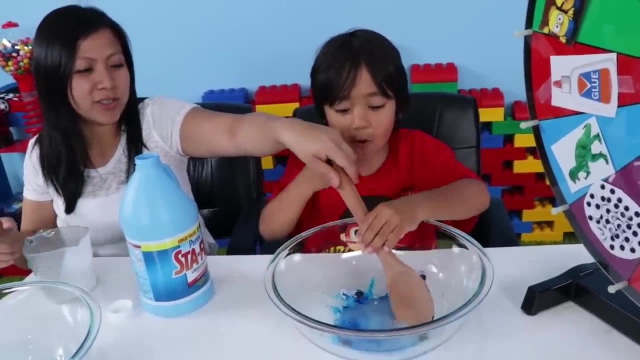 There you go. All right, Ryan, go ahead. Ah, Whoa, All you have is eyeballs in color, so you can color the cornstarch. Oh, Let's see if it works. Oh yeah, look, The liquid is turning blue, so that's pretty. 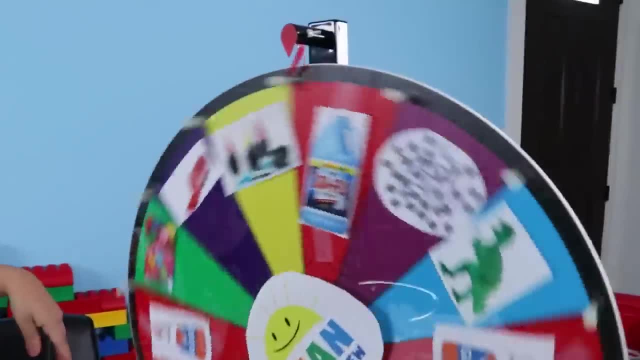 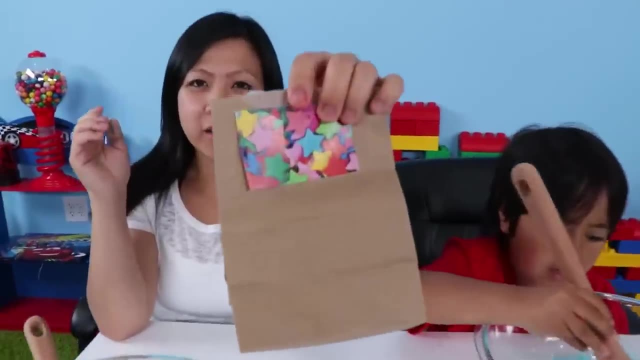 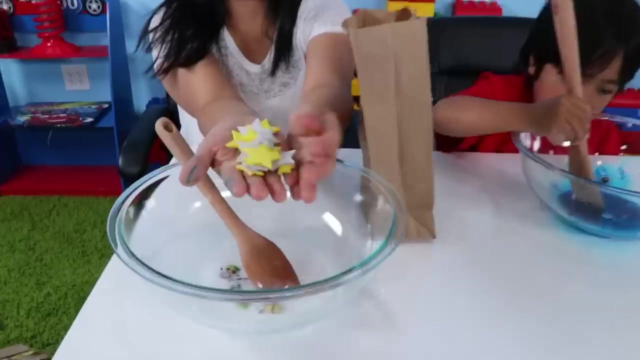 cool. All right, let's see what I'm gonna get. No liquid stars, No liquid stars. Whoa, I got stars. Got a container of stars here, Put it into my bowl. Whoa, Yeah, Oh, look at all these yellow stars. so that's fun. 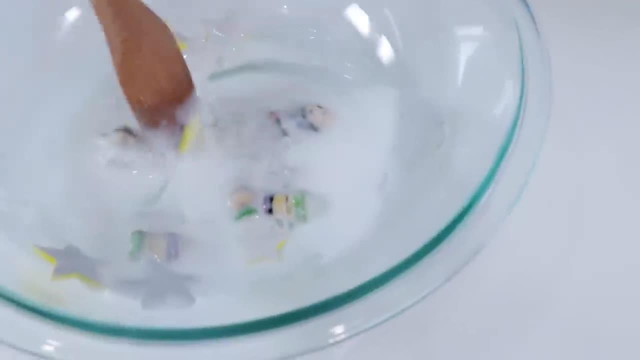 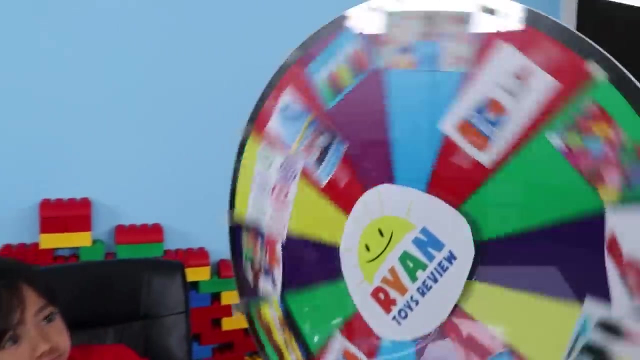 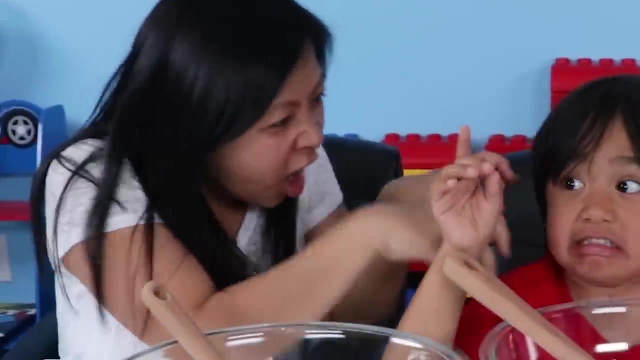 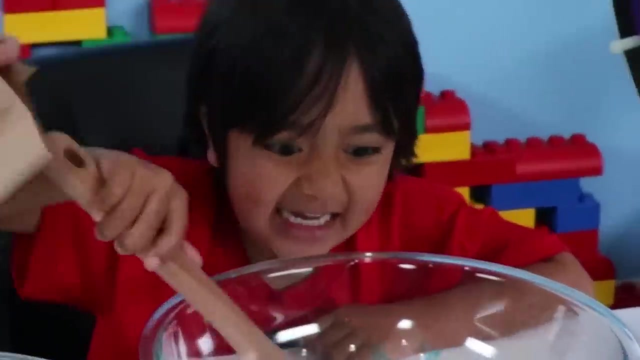 That goes in too with the minions. What do you think, Ryan, of my slime? Let me see. Ah, My turn. Whoa Ryan, Oh my goodness. Ah, All right, Ryan, here is your mystery bag of dinosaur. Here you go. 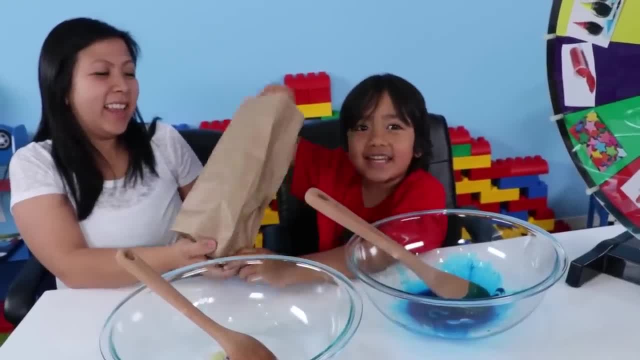 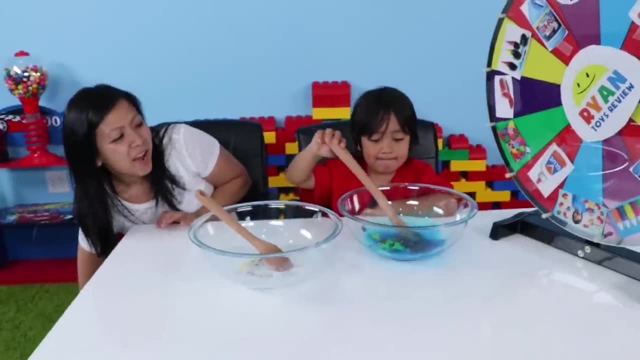 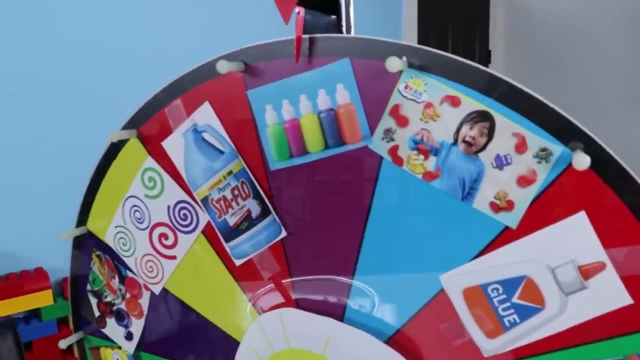 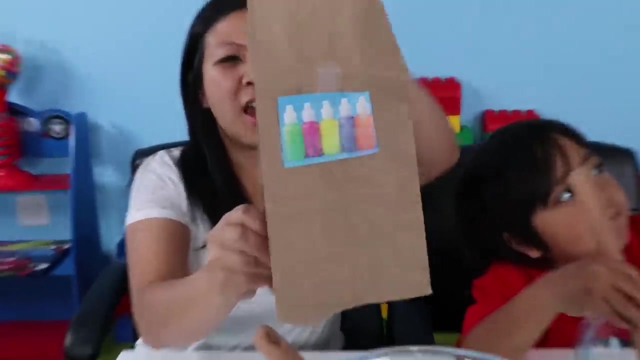 Mystery bag of little dinosaurs. Whoa, somebody got oh, oh, oh, oh. All right, Ryan, my turn, Let's see what I'm gonna get. You got it, I know, Come on. Whoa, what is that? Is that glitter, Glitter glue, Glitter, Glitter. So here it is, Let's see what it is. 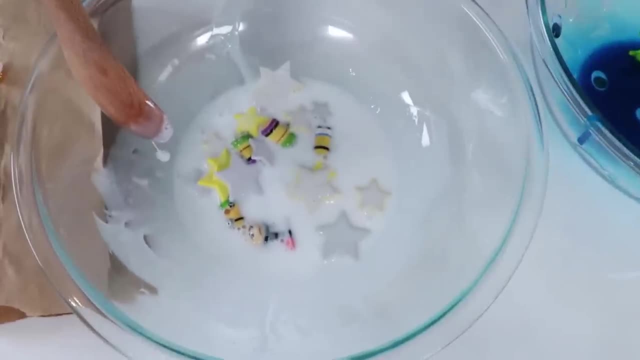 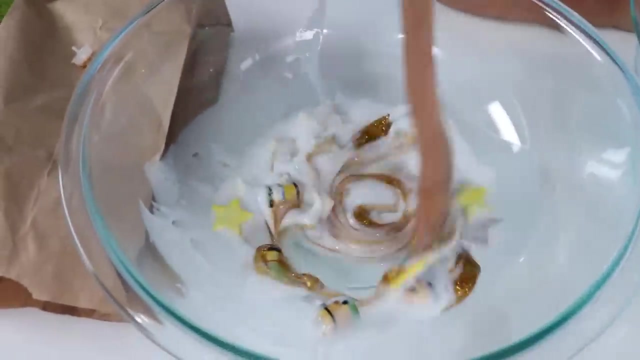 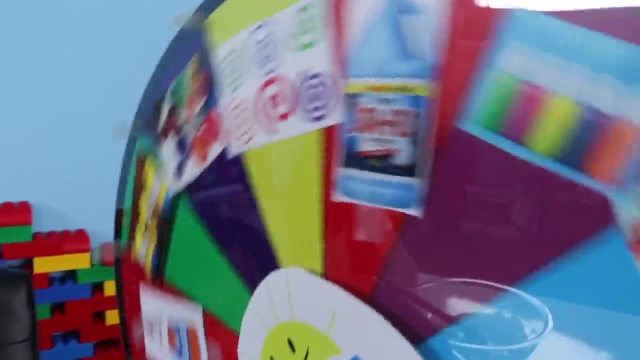 Whoa it is, It's glitter glue Dumping into the minion. Whoa, Okay, I think that is enough. I'm gonna swirl it up. Whoa, Whoa. Three, two, one. It is my turn Go. 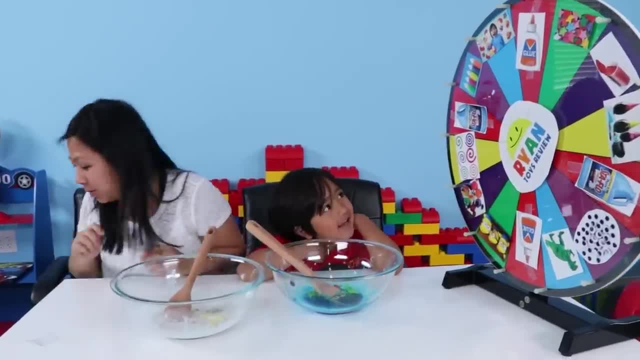 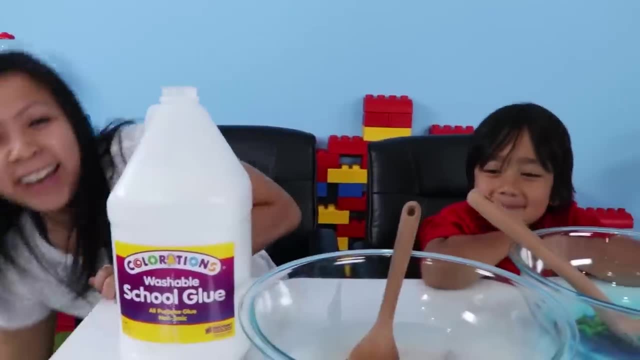 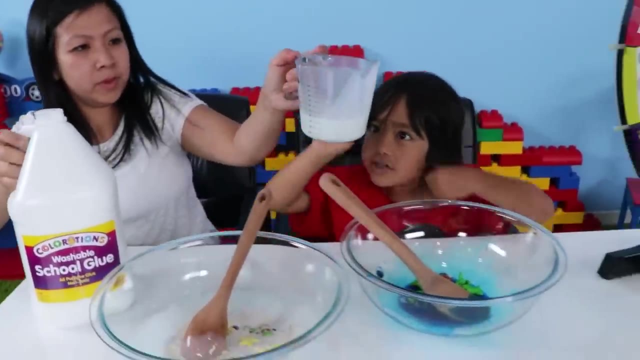 Nice, Ryan glue- Exactly what you needed. A giant container of glue always comes in handy, Are you sure? Yeah, who doesn't need glue? I have both of the ingredients, I know, There you go. One and a half. There you go, Ryan. One and a half. one and a half, one and a half, Okay. 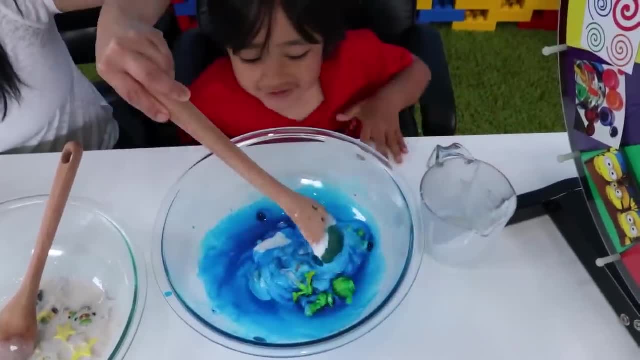 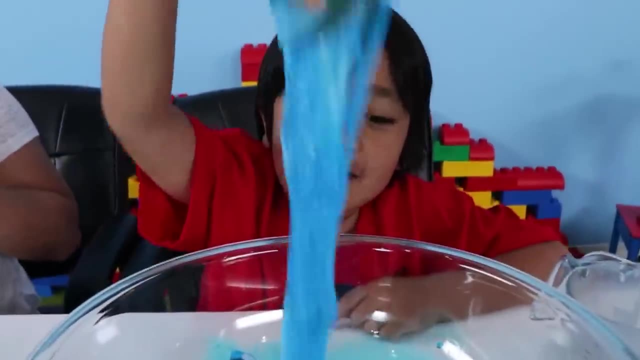 Mix it, Mix it. It looks like all the slime. Yeah, it looks super close to slime, I know. You know what else you're missing? What water? We'll add that last Whoa. So Ryan is really close to. 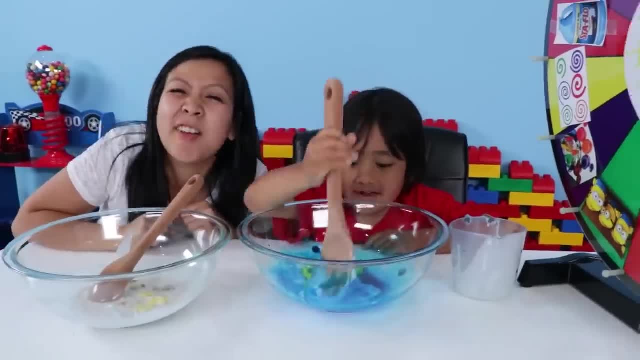 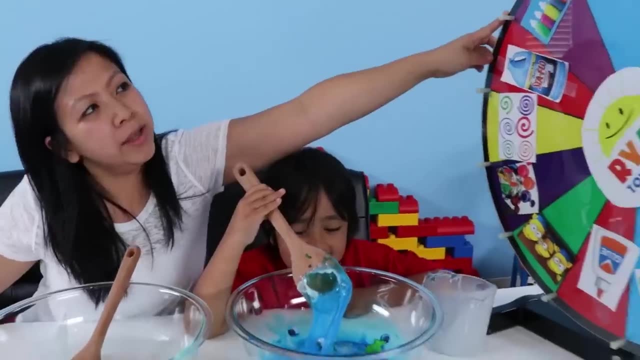 slime. so I'm going to need some of that liquid starch, or else I can't beat Ryan. Okay, Ryan, we're going to do two more rounds each, okay, Okay, Whoa, Alright, let's see what I get. 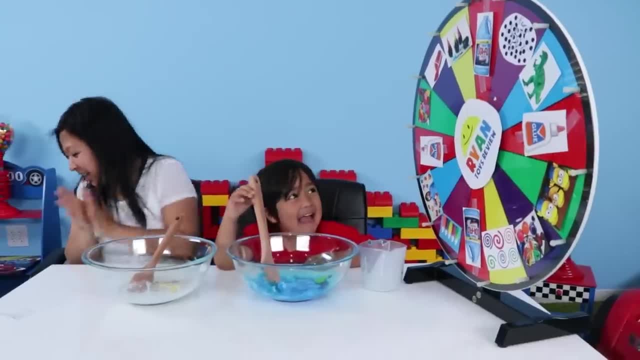 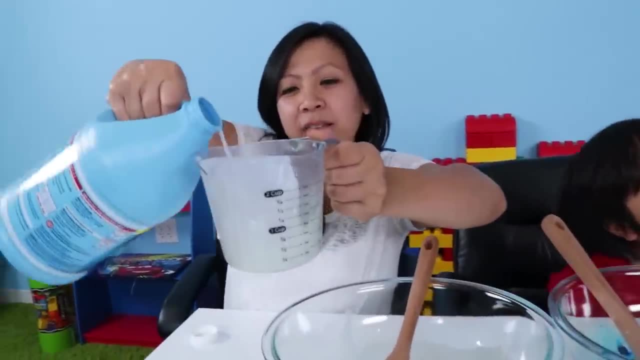 Oh, so close, So close. Yay, Exactly what I needed. Woohoo. Liquid starch, Ryan, we can both make slime, So I got my liquid starch here. Alright, One, two, three, Woohoo. 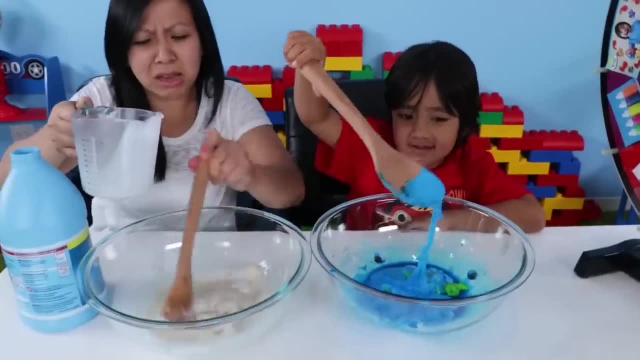 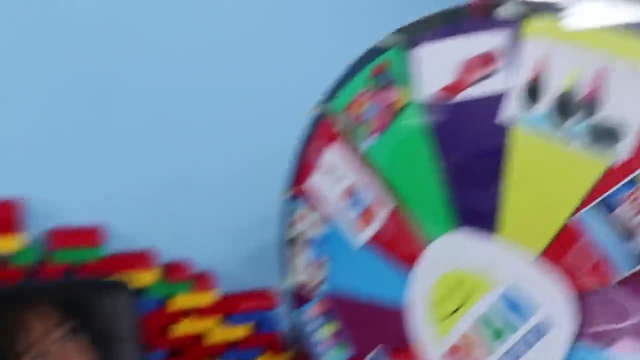 Ryan, we need some color in my slime. That's what I need. This does not look good. Your turn, My turn. Let's see what we're going to get. Glitter, Glitter. Here's some fun color. There you go. 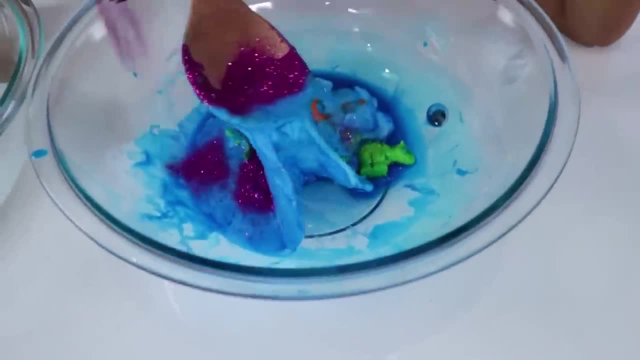 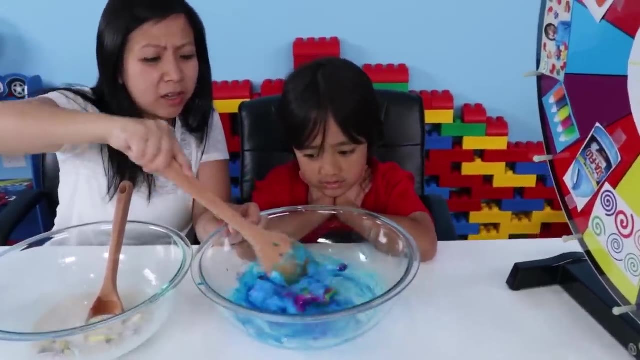 Hey, I want you in. Okay, that's perfect, I want you in here. Okay, Okay, Mix it up. Mix it up. Oh, your slime looks good, Ryan Ugh, Looks like a big blob, but it looks kind of cool. 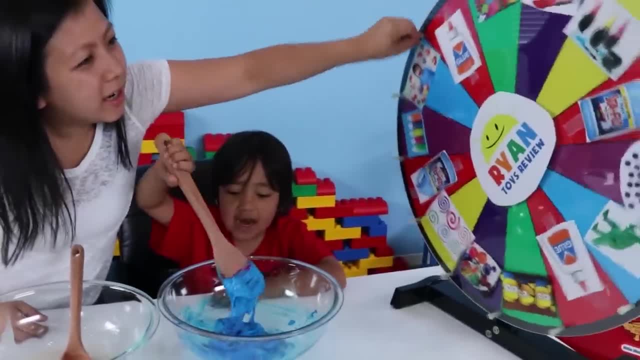 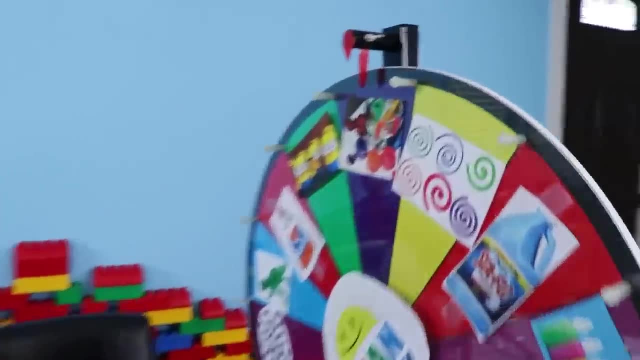 My turn. Let's see what I get. You have one last round. Okay, let's see what I get. What is that? What is it? Is it paint? It is some color paint. Let's see what color I get. 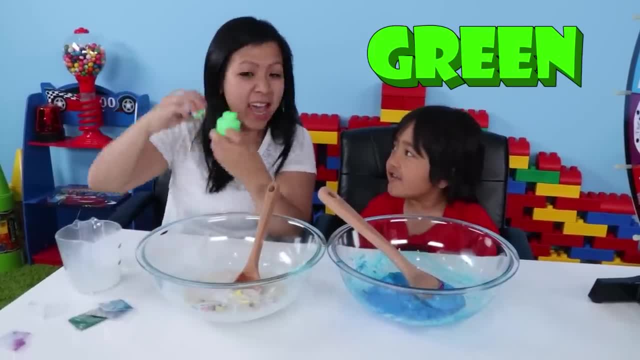 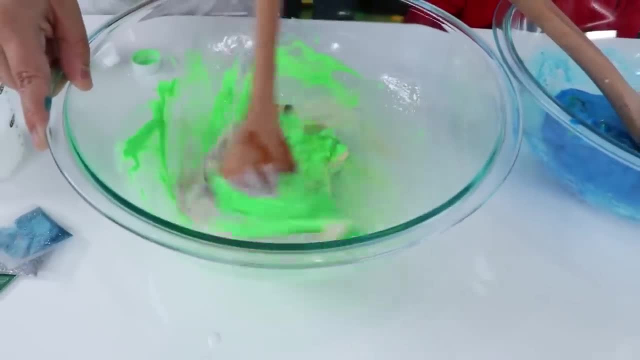 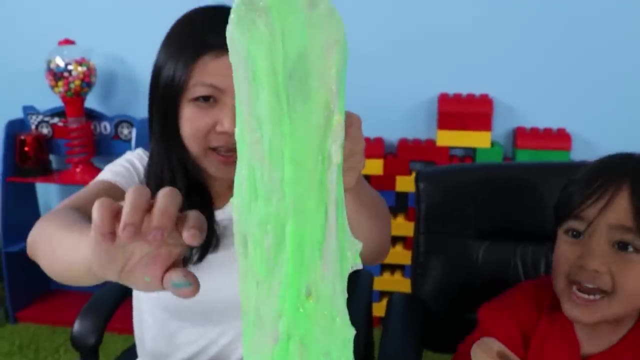 Oh, green, So I get green slime, That's all. Wow, look at this. Oh, Mix it, Mix it. Wow, mine really does look like slime. almost, Mix it up, Mix it up. Does it look like slime to you guys? 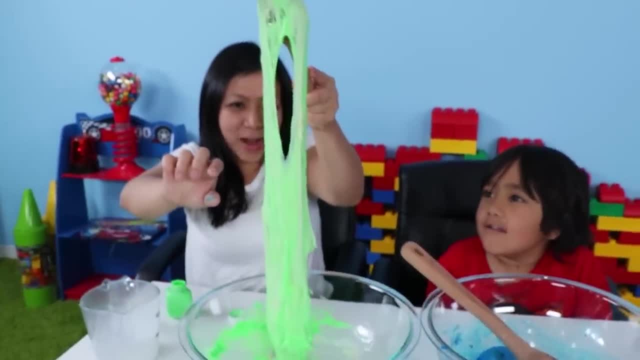 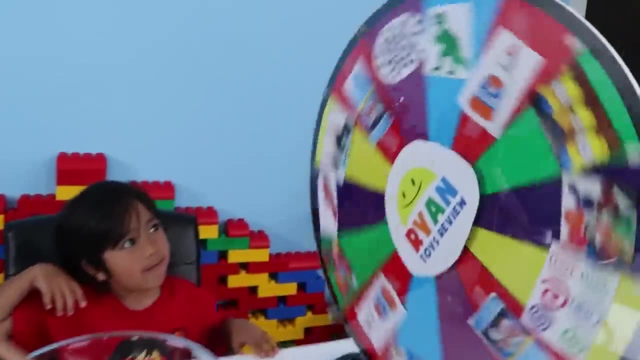 Hey, I see a star. I do me too. I see the minions, too, dropping out. Oh Okay, Ryan, last turn for you. Joy, That looks like tornado. That looks like a little swirl Tornado. 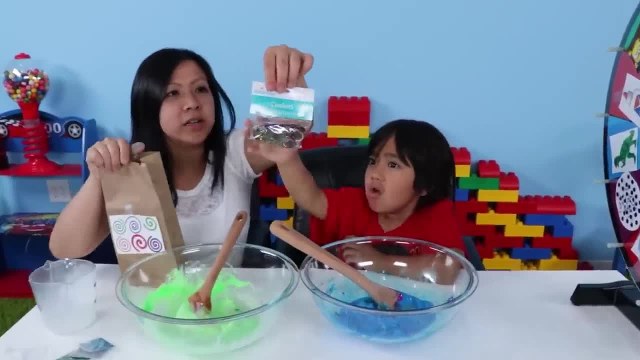 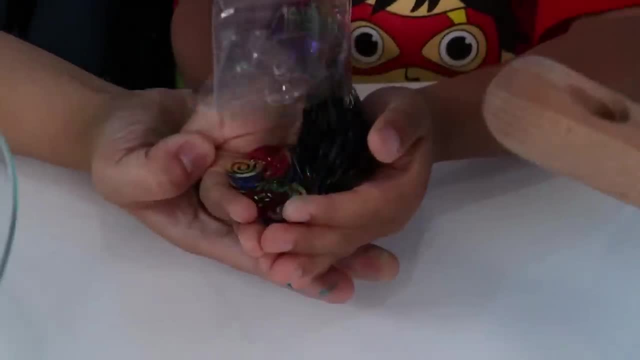 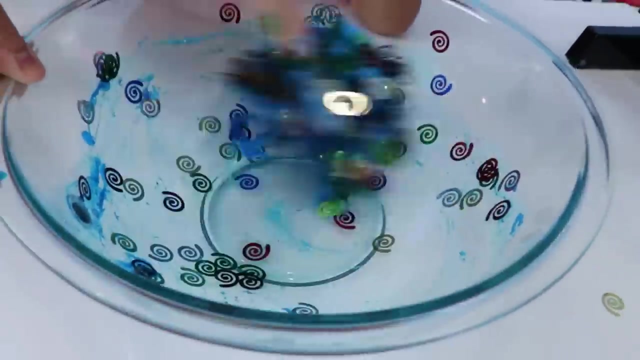 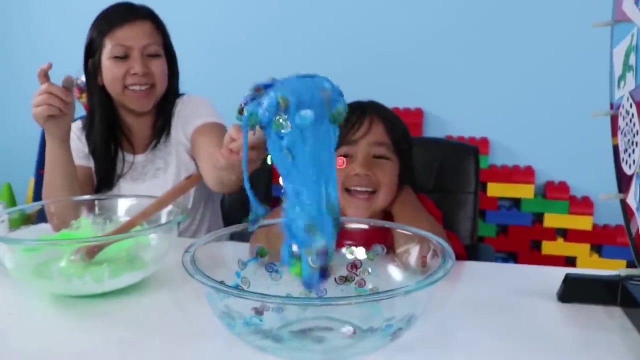 here it is. what is it? oh, are these little confettis? oh, there you go the whole thing. i'm gonna get those two. whoa, it doesn't even swirl anymore. it's missing water. look it's. it's just a piece of blob on a stick. look at this last one for mommy. 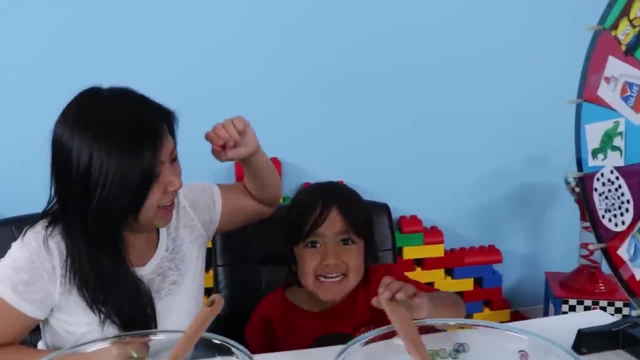 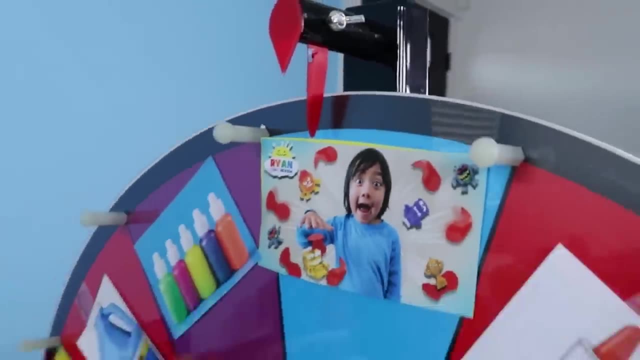 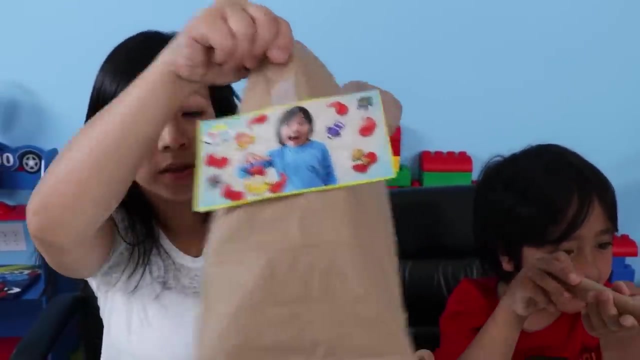 and then we're gonna compare who did the better. slime you ready, no spin, what is that? ryan has your face in it. so we got a whole bunch of these little zero smasher toy sports here. they look fun and they go all go into the slime bowl. 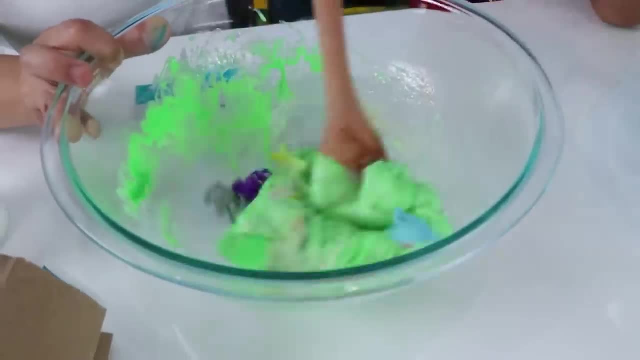 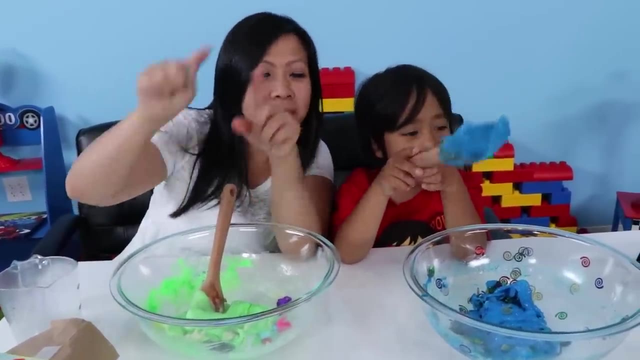 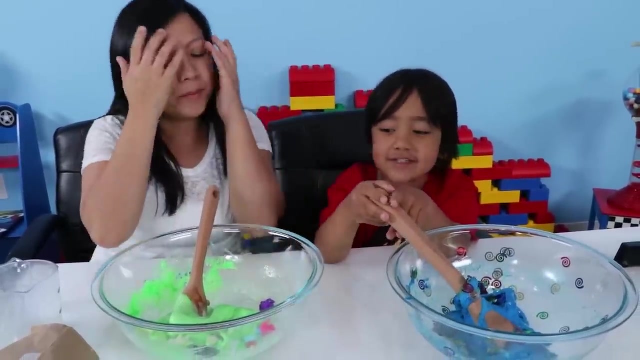 whoa mix it up? whoa do we have water yet? yeah, so last thing, we need to actually water. so i'm gonna put water in mine and ryan and then we're gonna create slime and you guys, let us know who create the better slime. okay, and then, after the video is done, i'm not like: oh, you mix it together. yeah, that's a. 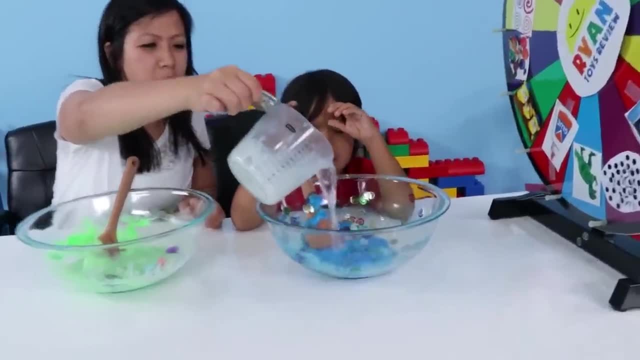 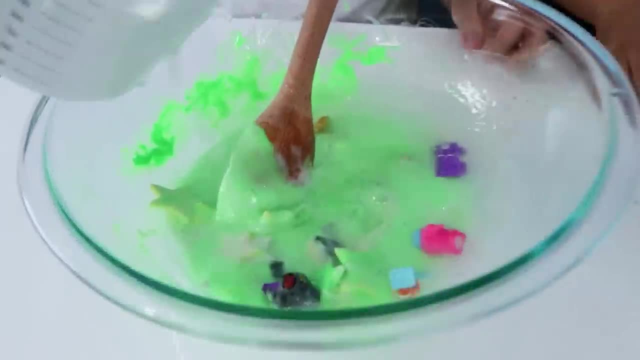 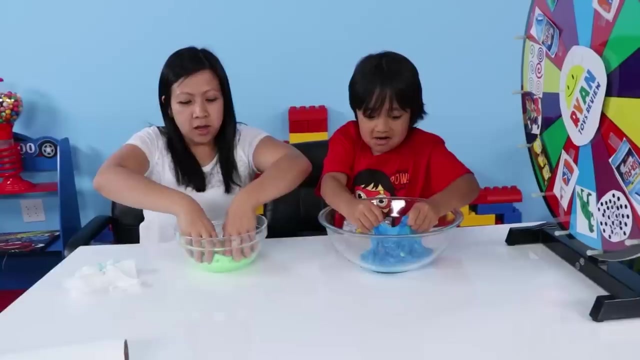 good idea. yeah, i got the water. put some water into ryan. there you go. now you have to mix it up and then put some water in mine. okay, and then what we do is just mix it up. oh, this is a little bit liquidy. yeah, it's hard to mix. all right, so we mix for a while. 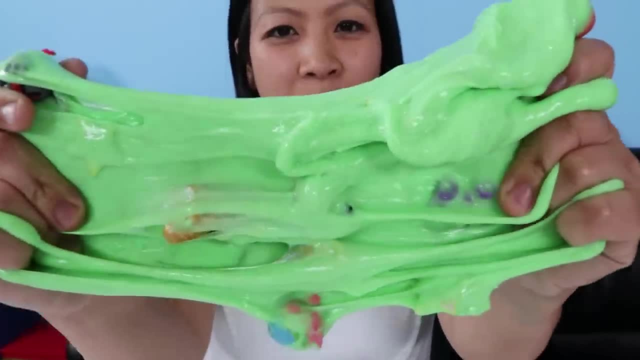 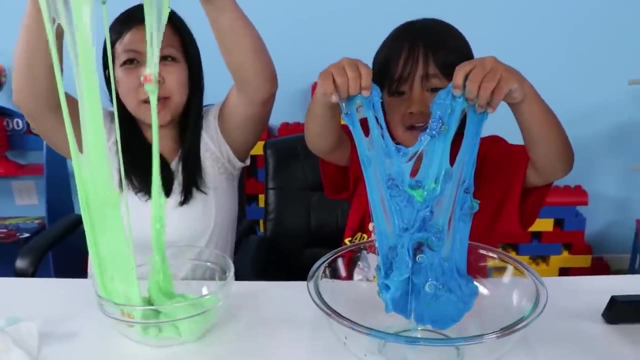 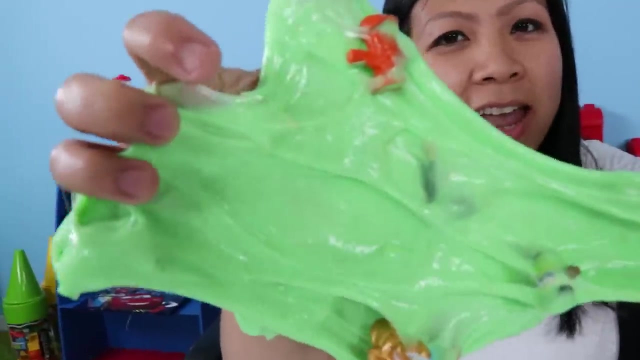 and our slime is done. so here's my slime. whoa. here's my slime. i took everything out, whoa. so you guys, let us know who did a better slime job. mine is like harder to hold, is it so? mine had minions in it. it has glitter and it has little sports figurines. mine has little. 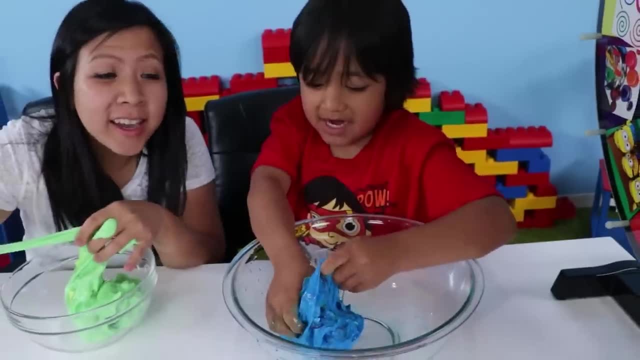 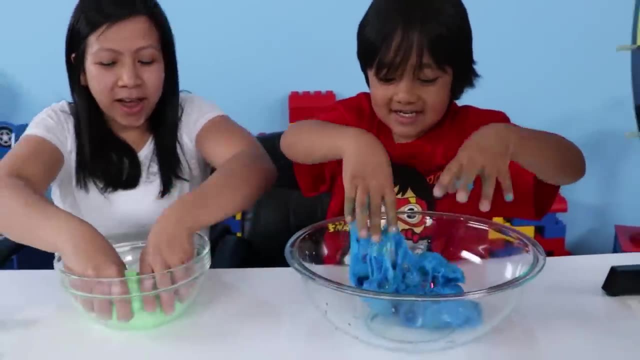 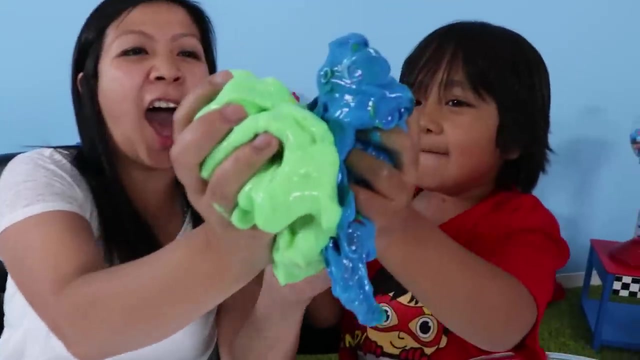 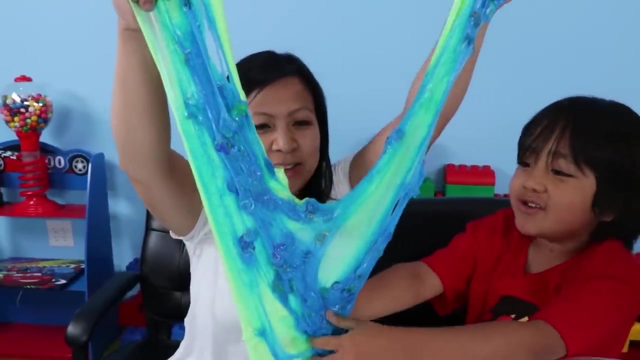 pools uh-huh and eyeballs and, yeah, i am blue coloring whoa doing a mix size. okay, all right. so ryan said he wants to mix ours together. are you ready? one, two, three, put it in. green is stronger than blue. did you know green is stronger than blue, is it? it is. 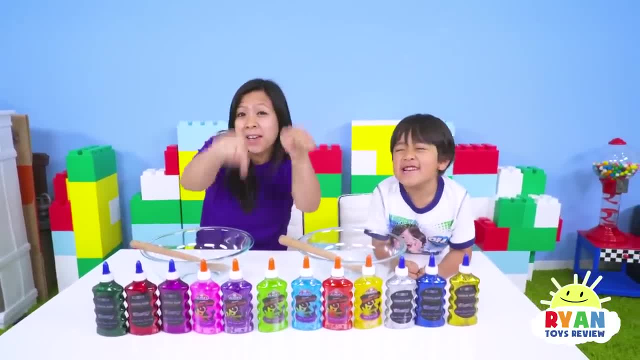 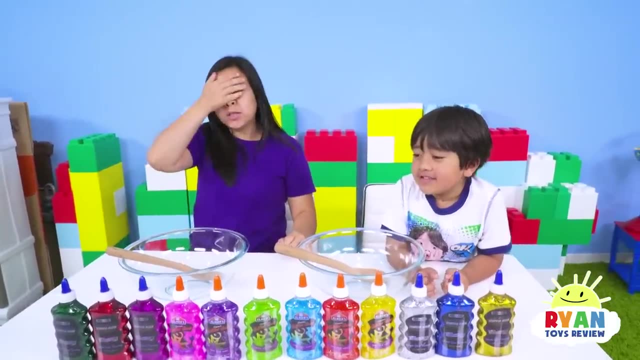 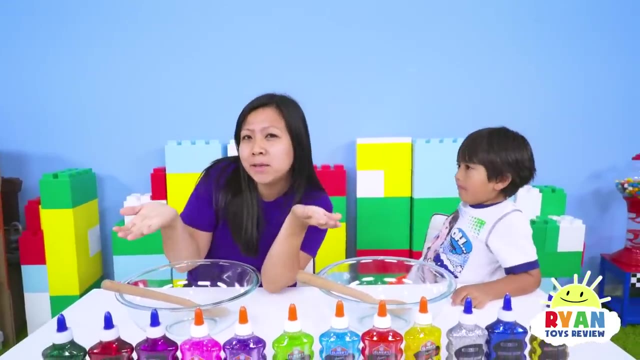 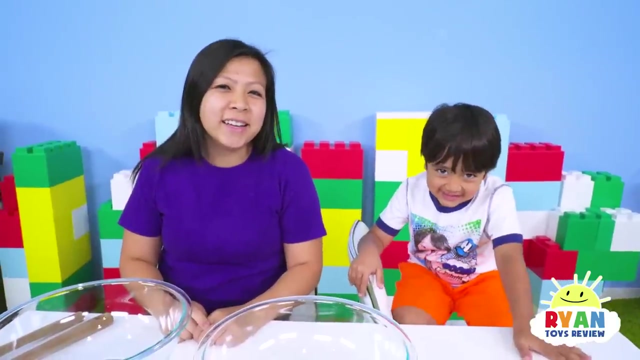 hi guys, today we're doing the three glue slime challenge. it's gonna be mommy versus ryan. so what do we do? we're each gonna close our eyes, squiggle it around and pick three, uh, randomly, and whoever creates the best looking slime wins. so you guys, let us know who create the better looking slime. are you ready? okay, let the slime challenge. 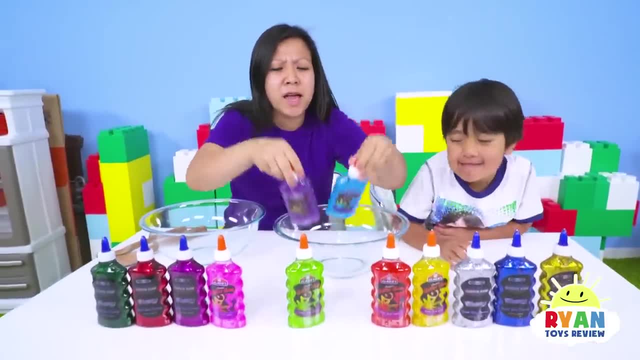 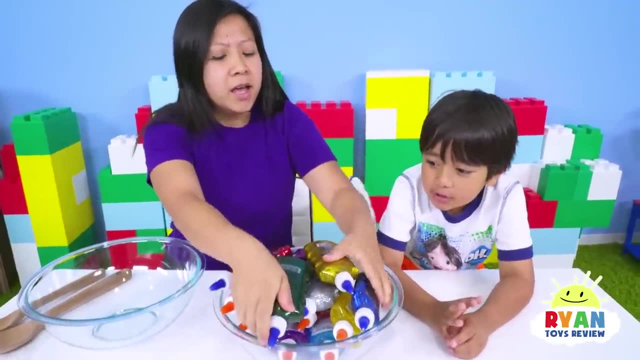 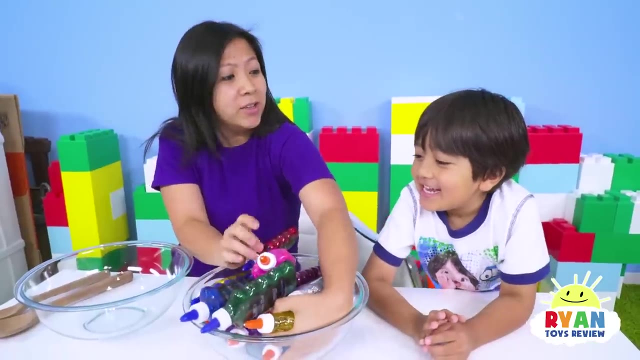 begin. so first i'm gonna put all the slime glue bottle into this container here and i'm gonna squish it around and ryan closing his eyes. we'll take three. okay, all right, ryan, close your eyes while i squish it around. squishy, squishy. ryan, you cannot look squishy, squishy. 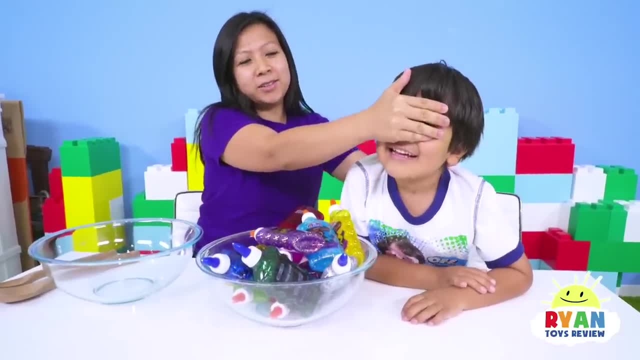 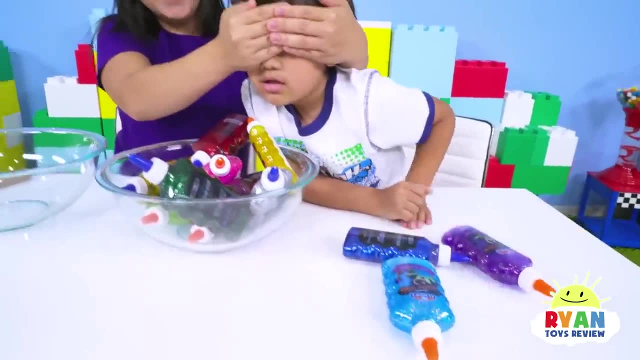 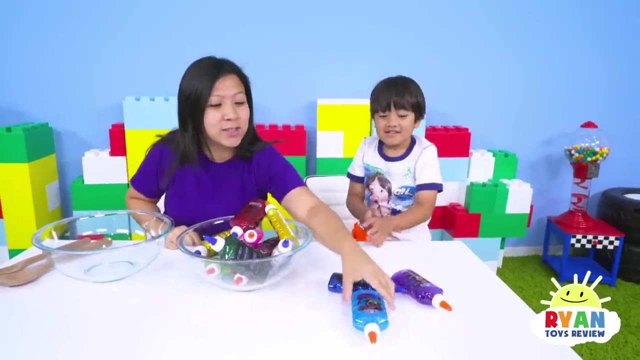 i'll help him go ahead. ryan. three colors. okay, he got one, two, three. are you ready for your color? uh-huh, that's what i wanted, really. this is a good color. i got light blue, dark blue and purple. that's good. okay, ryan, i'll let you squish. 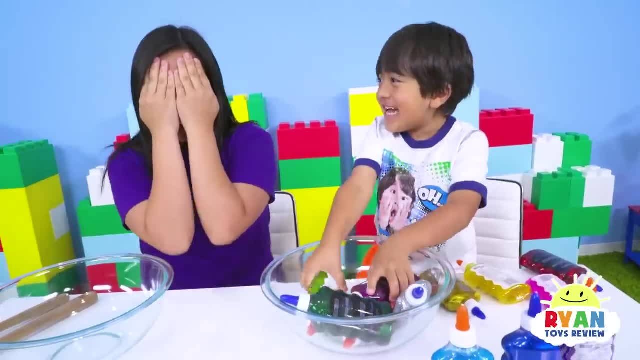 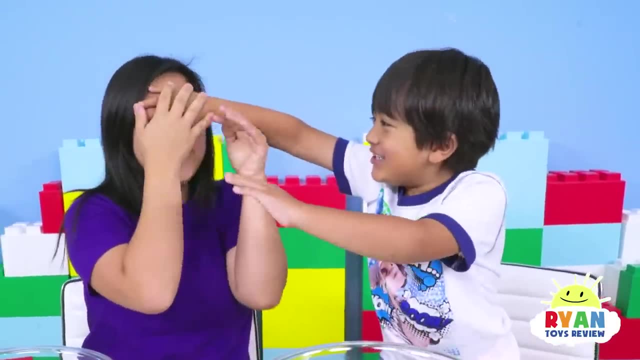 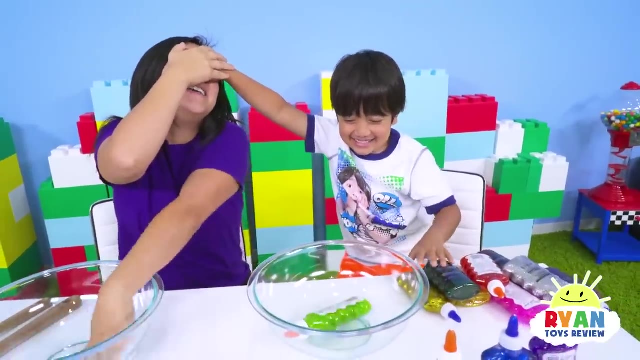 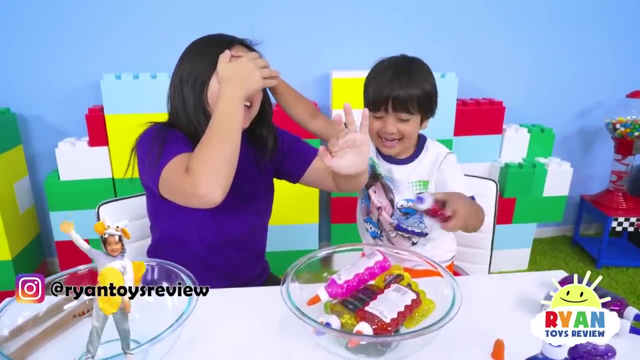 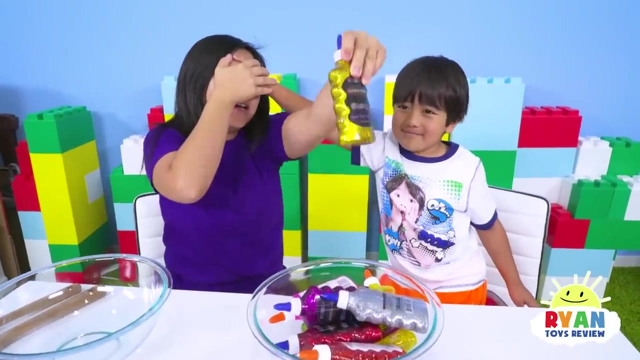 ready, not ready, yet, not yet. do not look. done, done, okay, close your eyes and do not look, okay, okay, wait, there's the slime. where's the slime? ryan, put it back, you, trickster. is it ready? yep, okay, better not lie. you want color it a good color. 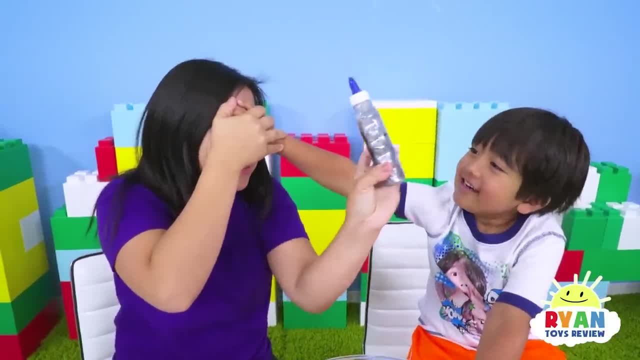 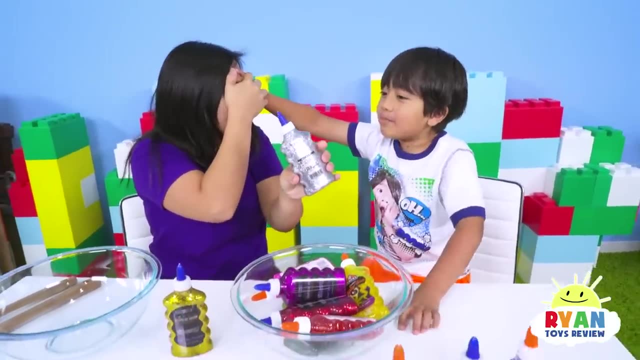 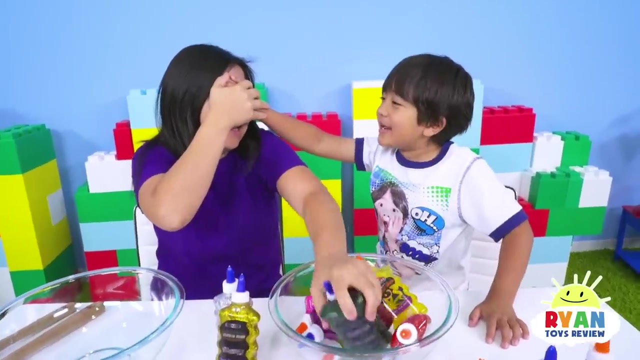 i guess okay, ah, second color: is it good? uh, is this a good color? that's expensive, expensive like gold, diamond, silver. you got two stuff that are expensive. oh okay, last color: not有 ar fu, It's not uranium. Is this a good color? That's like a dirty color. 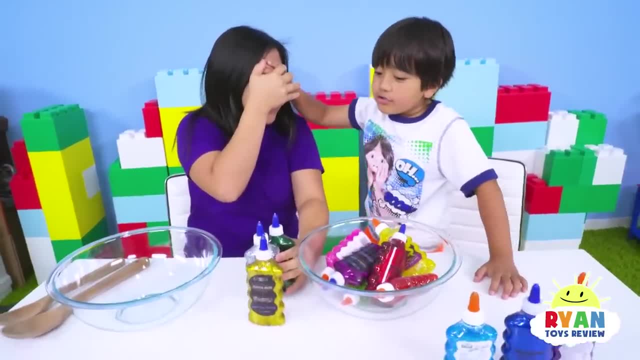 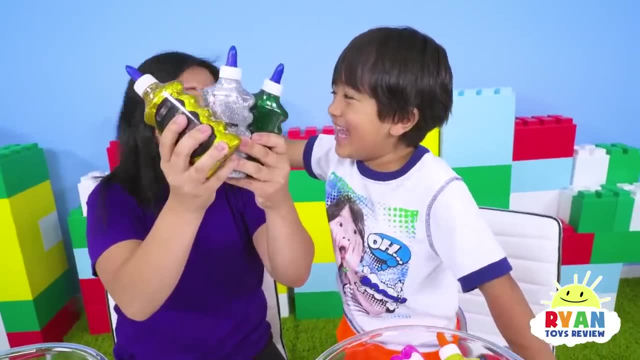 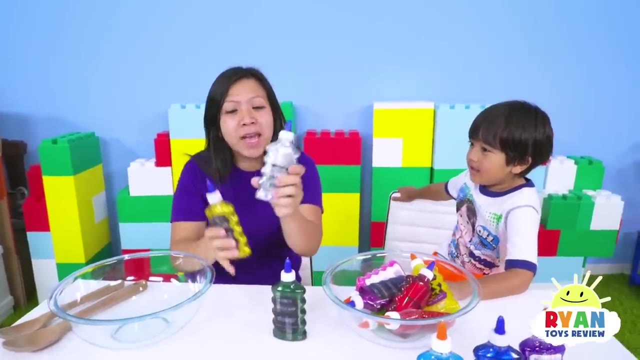 Dirty, All dirty colors. That's not good. No, you have two expensive colors and one dirty color. Okay, alright, One, two, three. Let's see, Let's go. This is too dark of a slime, But maybe because I have silver. 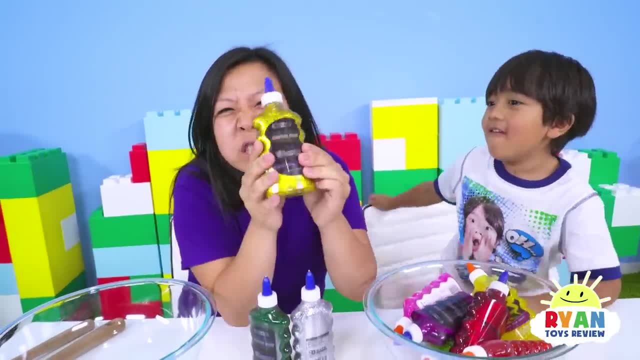 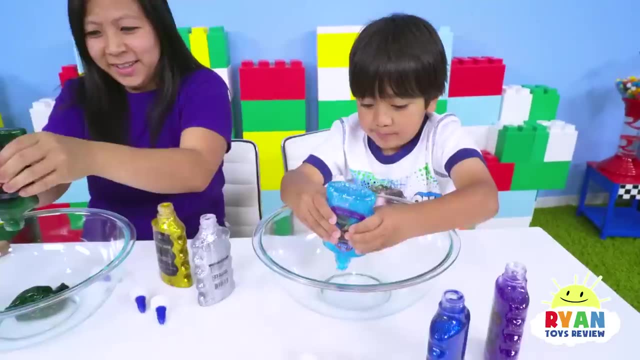 maybe I'll make it lighter. And then, who doesn't love gold slime? Am I right? Let's make some slime, slime, slime, Woohoo. There you go. Whoa. yeah, I like that color. It looks under the sea theme. 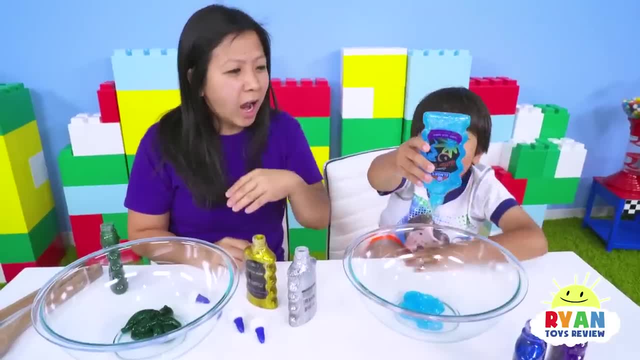 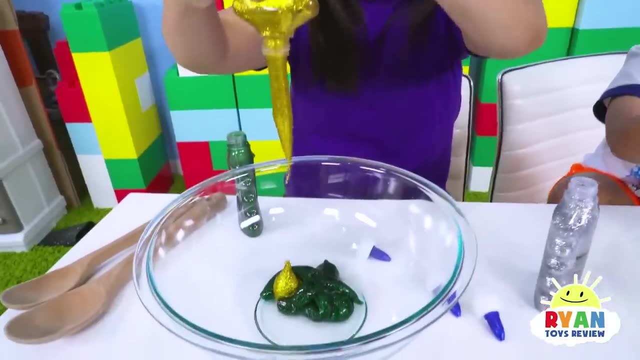 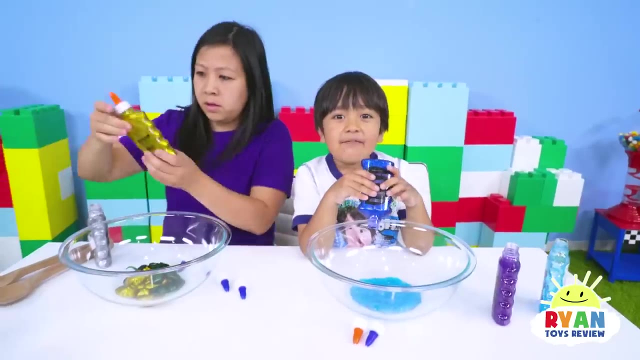 It looks really pretty. It looks like a mermaid. There's a little tail, Wiggle, wiggle, wiggle. Whoa, look at the gold Under the sea, under the sea. Yeah, Time for my second color, Mommy's just. 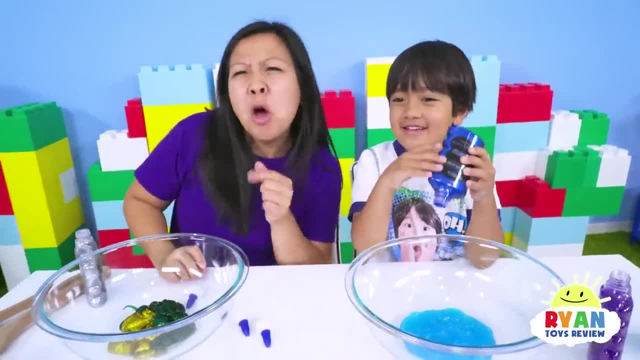 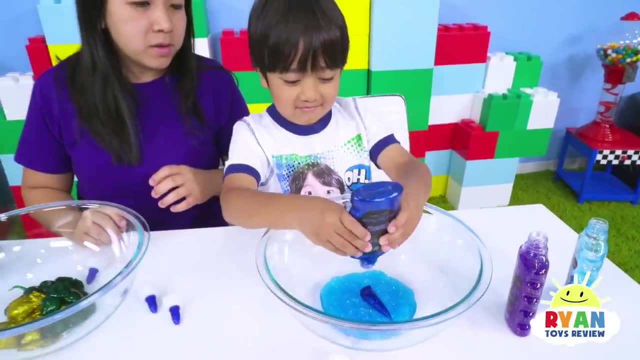 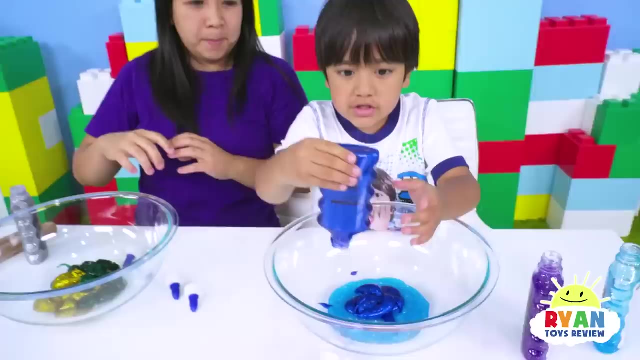 doing a blob, I'm doing layers. Okay, We'll see who comes out better. Whoa, that looks cool. Yeah, it still looks like under the sea. Under the sea. You have to just wait because it's coming down. 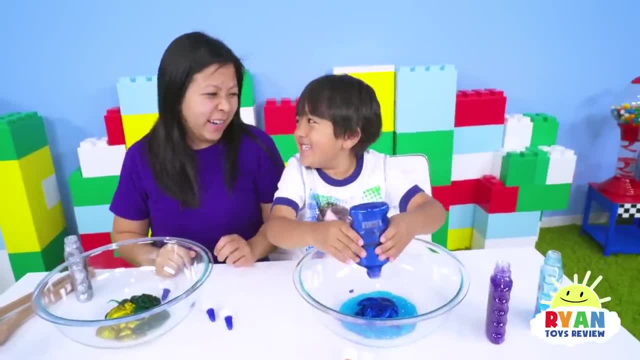 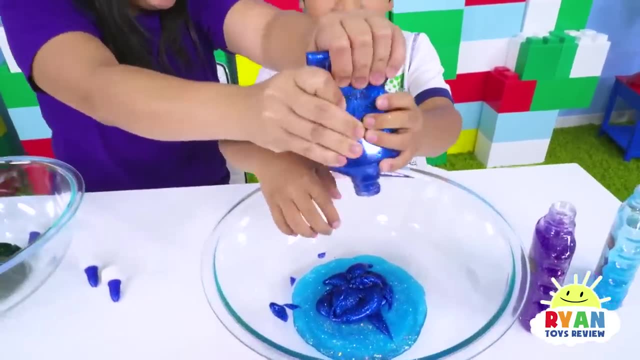 Oh, okay, You know the technique of slime glue making Technique, Do you guys see it? Do a little bit of piece hanging. Well, I want to make a layer, mommy. So Ryan's spreading it out and making a layer. 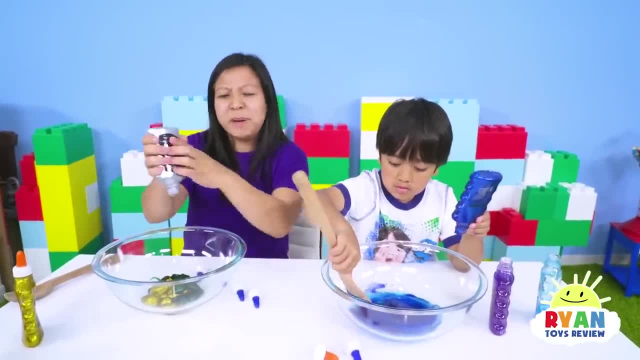 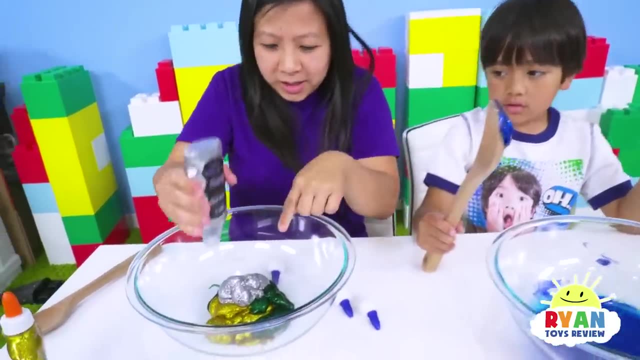 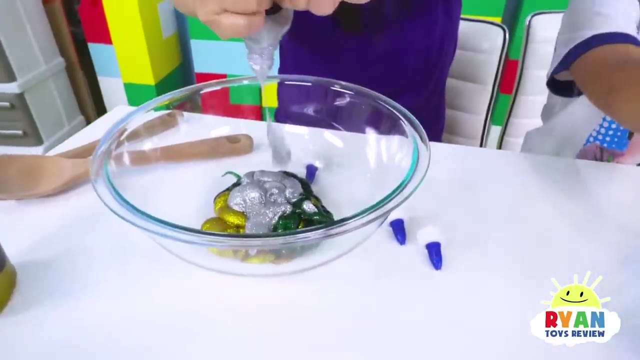 Okay, so while Ryan's making a layer, I'm going to use my last color, silver. Oh, look at this. Do you guys think this is beautiful? Is this pretty? It reminds me of Christmas. Is this Christmas color? Oh whoa. 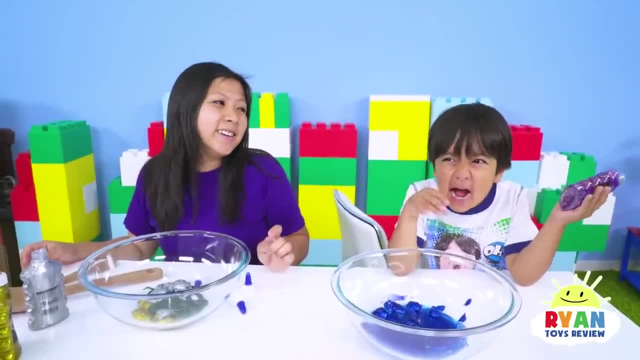 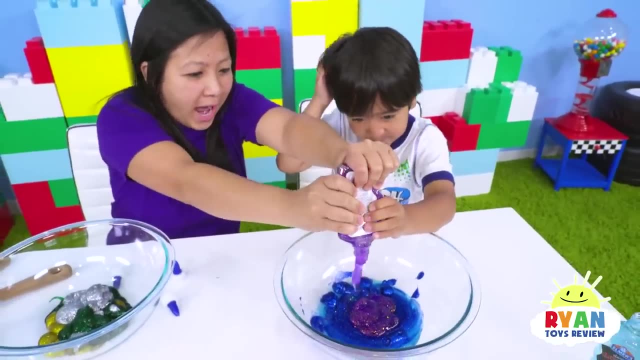 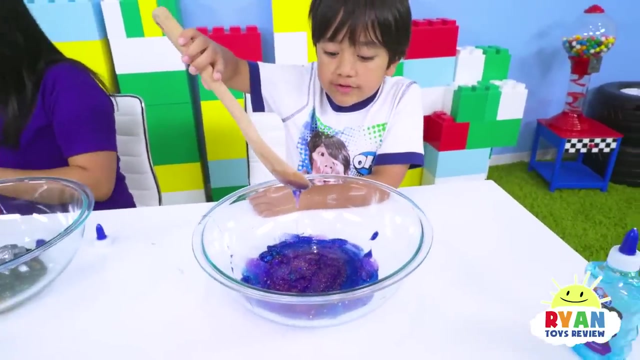 Doing my last layer. Whoa, That looks awesome. Whoa, look at that squirting out, Wah, Wah. Oh no, I think the darker blue is getting the purple. Oh no, It's getting over the purple. 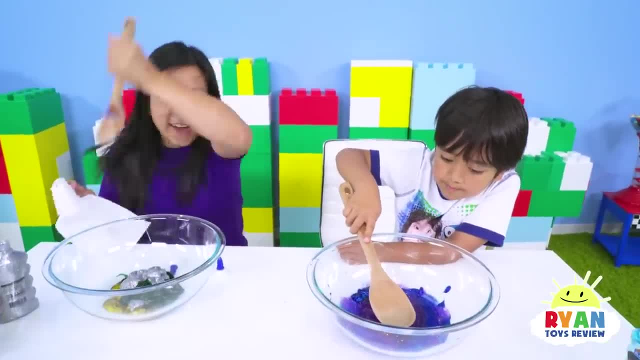 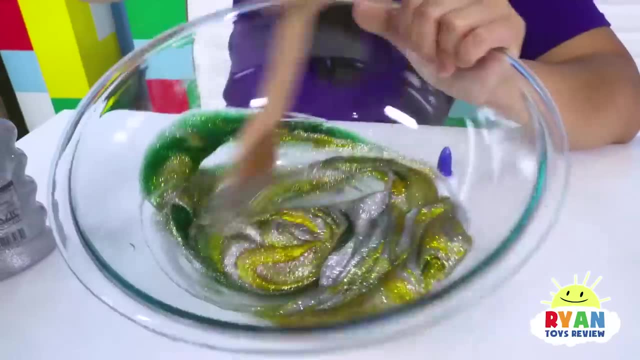 Ryan is layering it. I have a different way. I'm just going to agitate and stir it together. Are you guys ready for some fun action? Woohoo, Look at this. I feel like I'm making a cake. Yeah, Ryan, what do you think? 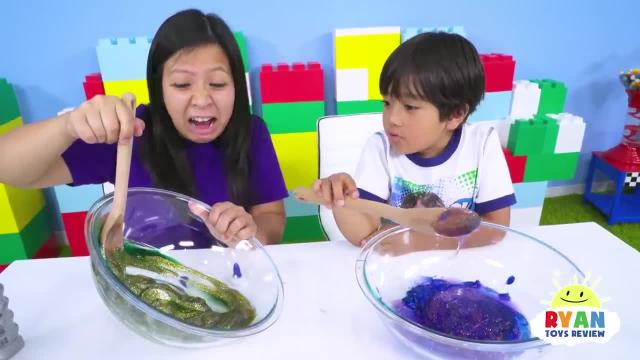 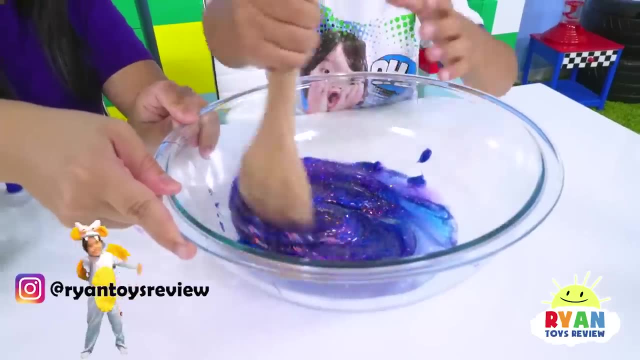 about this color? Whoa, It looks so cool, Does it? It looks like nature. so it looks like gold and nature It looks like nature. Well, thank you, then. I think yours looks cool. It really reminds me of Under the Sea. 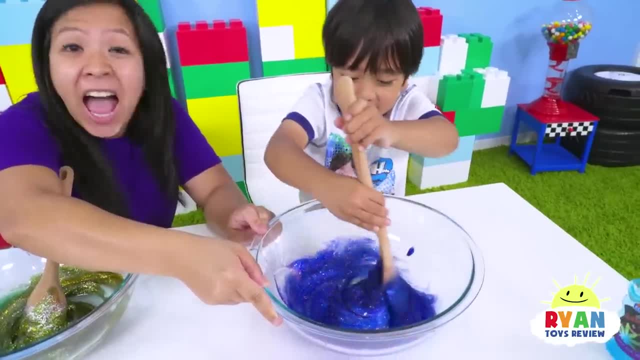 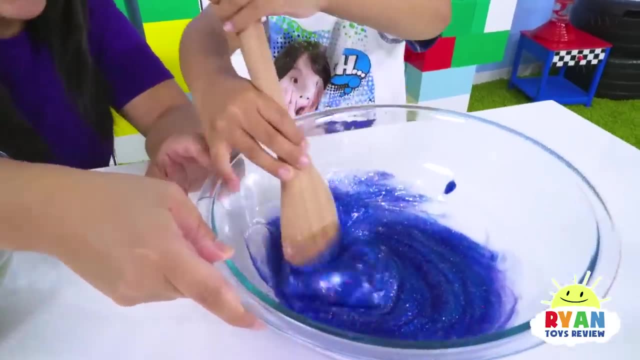 theme. Oh no, I think the only thing I have is the dark blue. I think, yeah, I think it's just dark blue. now, Dark blue is strong. It just took over the other color. Yeah, I wish I had. 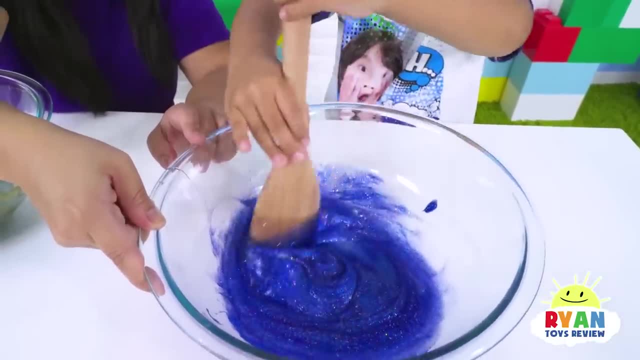 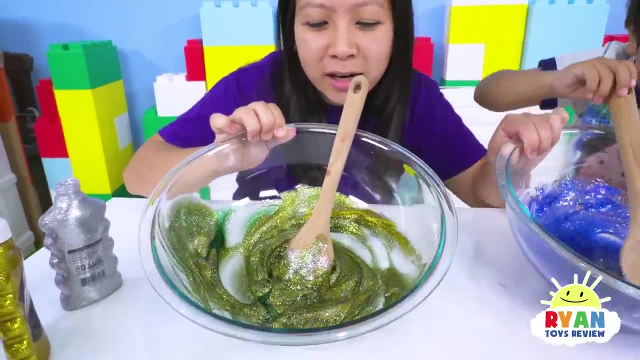 black, so I could take over the dark blue. You want black slime. That's pretty cool too, So far. who do you think has a better color So far, Mommy, Really You think mine's better? Mine looks like it has. 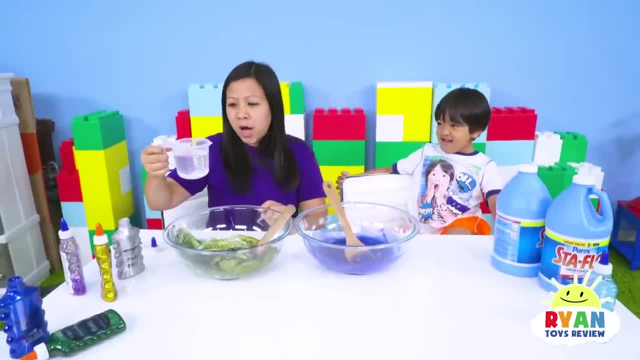 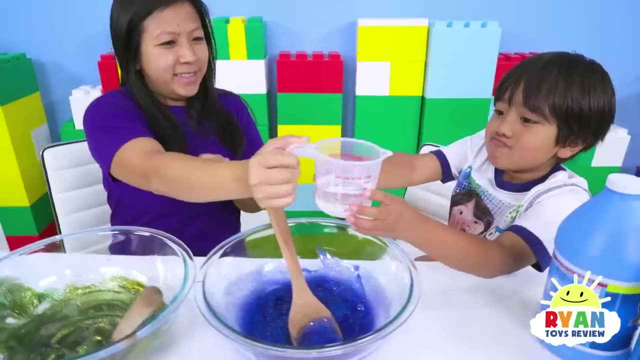 little sprinkles in it. I know Yours looks cool. Next, we're going to need some water, so I'm going to pour some water on mine. Some water, Some water. Yeah, Okay, Ryan, This is yours. Here you go, Be careful. 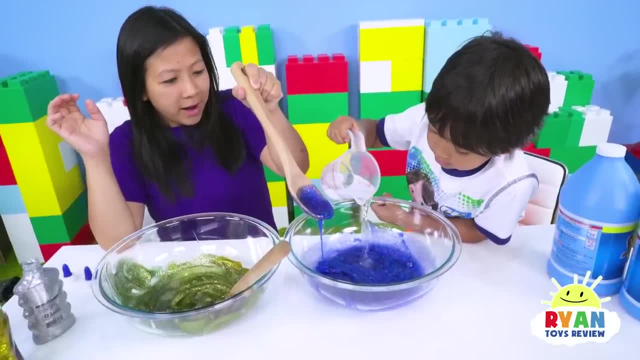 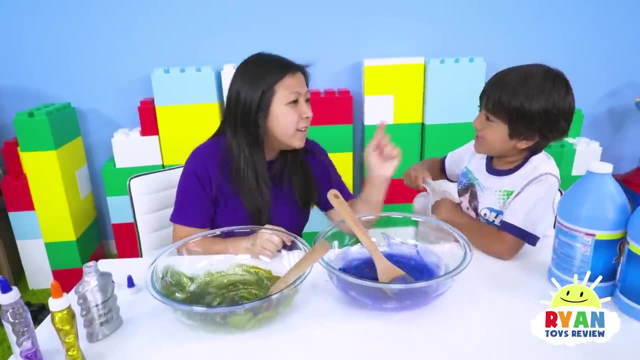 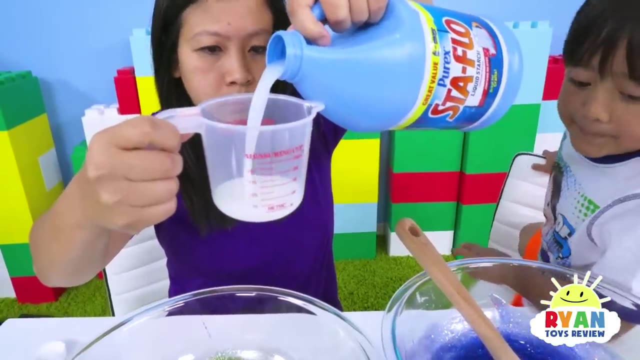 Oh, it's a little bit warm, Yeah, Whee, Nice. Last ingredient: Do you know what it is, Ryan? What Liquid starch Right here. So we need one-fourth cup of liquid starch. There we go In here. 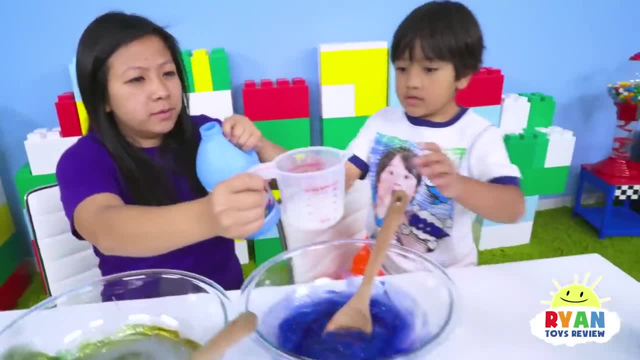 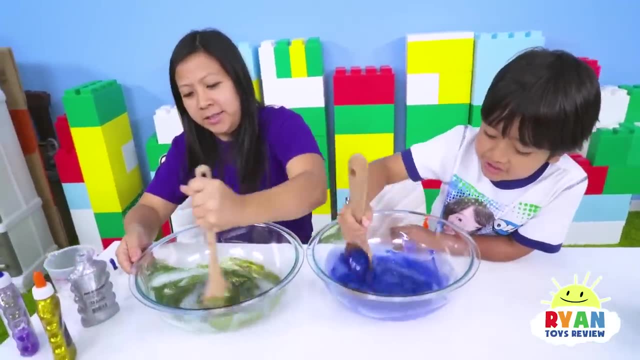 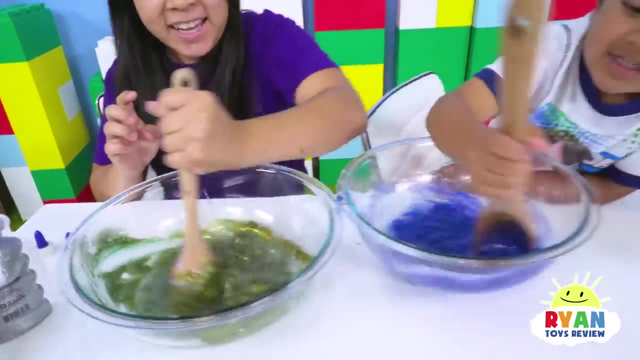 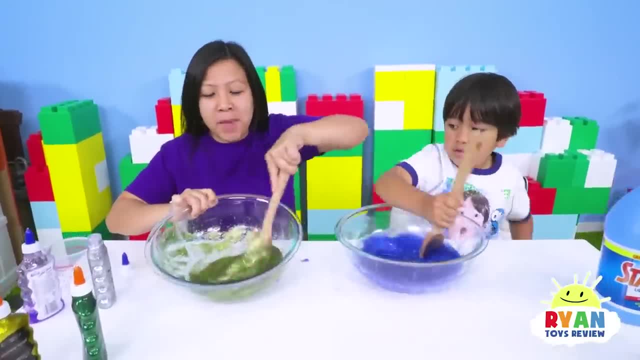 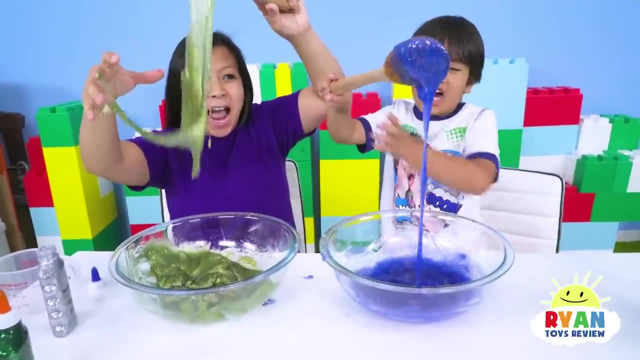 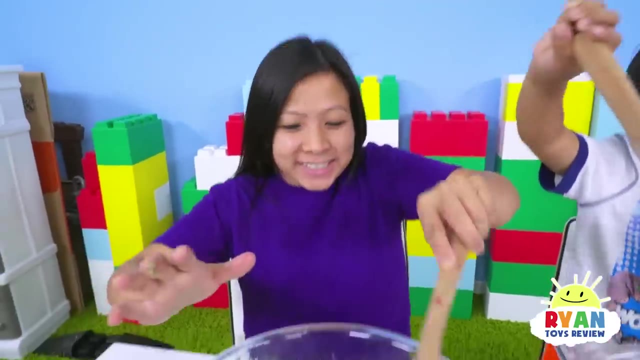 Exactly. We've been mixing for another minute or two and look, It's beautiful. Look at my beautiful slime, Slime, Slime, Slime, Slime. Who do you guys think looks better? Whoa, I only have one. 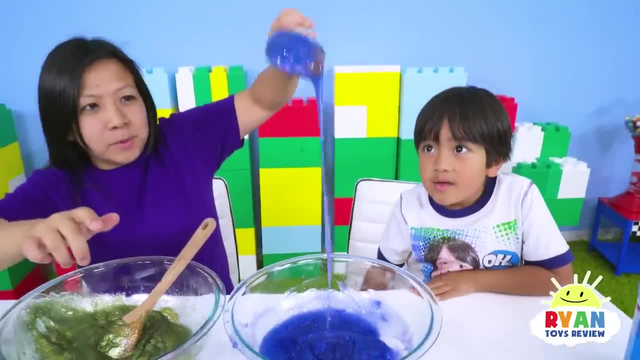 color kids. Ryan looks good too. Look at that awesome beautiful blue color. But I only have one color. I know it looks like he only used one color. The other two just dissolved. You can't even see it. 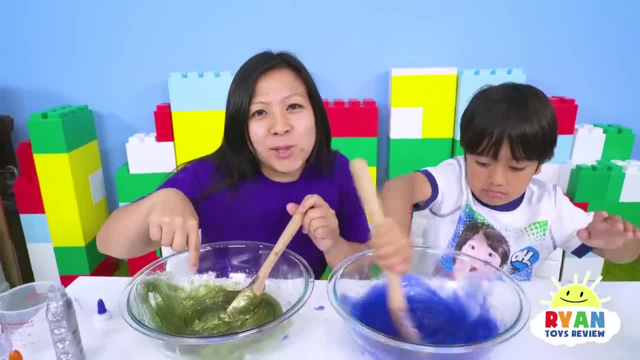 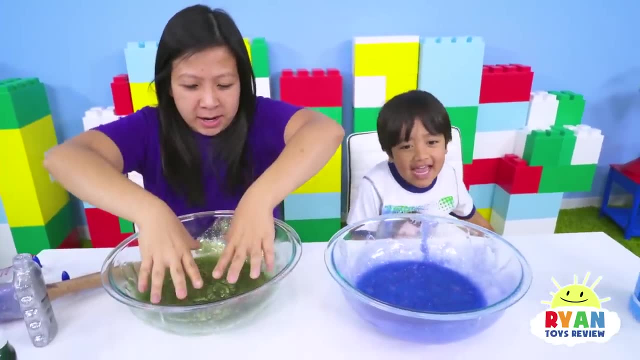 Okay, we're gonna mix a couple more minutes and we'll see if we can do the slime right. Okay, guys, so our slime is complete, I think, hopefully. Let's dig into our slime. Let's dig into our slime. Oh, it feels weird. 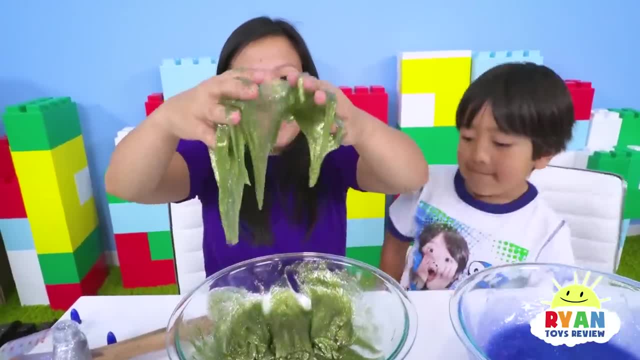 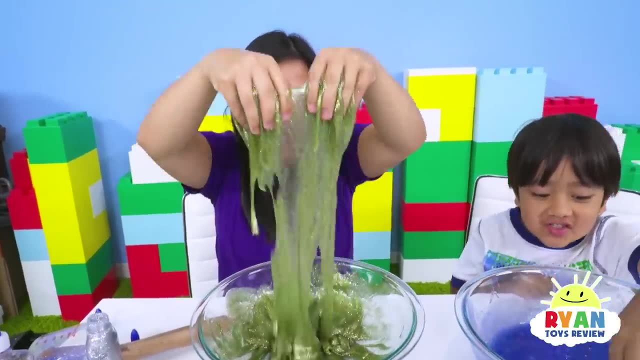 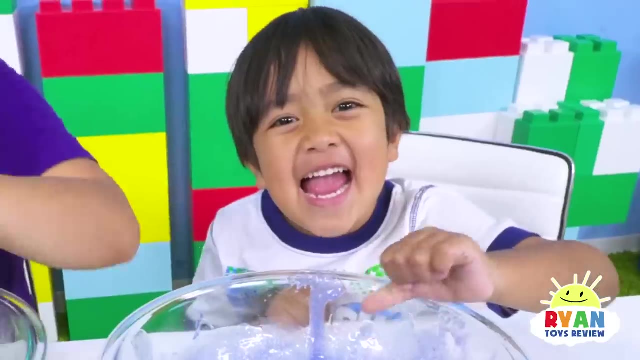 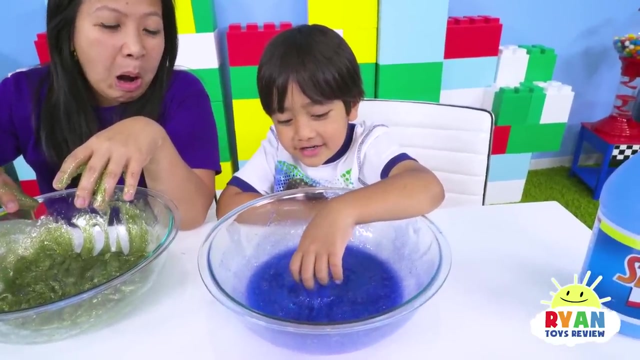 I don't think I did mine right. It's very mushy. Oh, look at this. This is not slime. What about yours? I have some bubbles: Bubble, bubble, bubble bubble. It's dissolving on my hand. 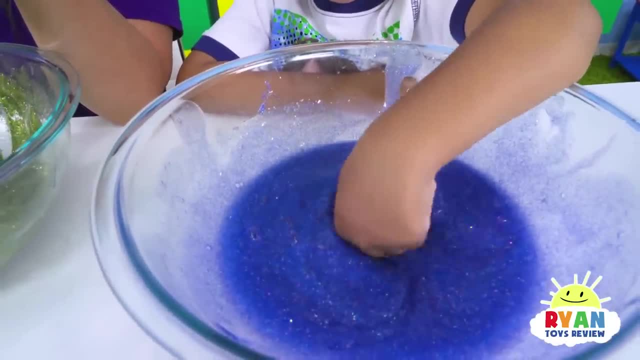 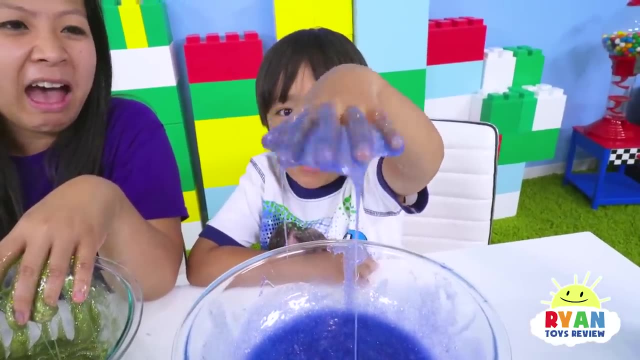 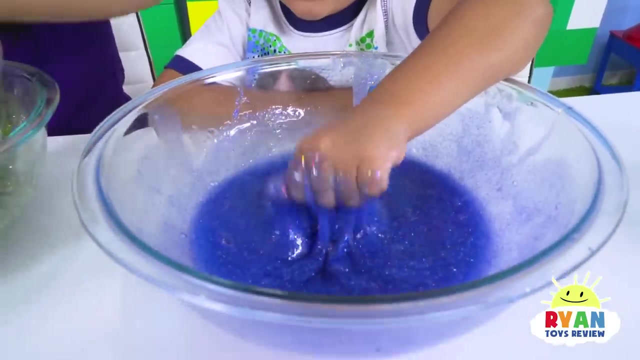 It's dissolving on my hand. How does it feel? It feels super weird. Whoa, So mushy. So it is. I think we made ours wrong. Oh wait, I have a surprise. Close your eyes. Close your eyes. 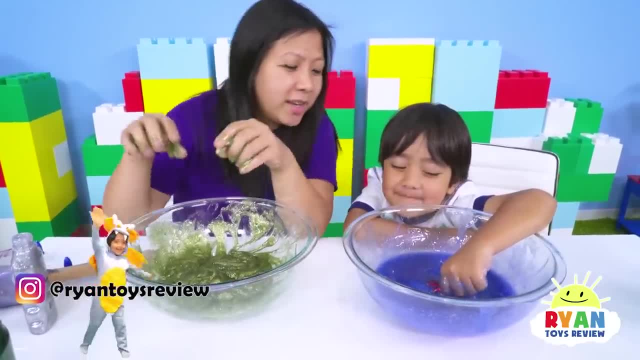 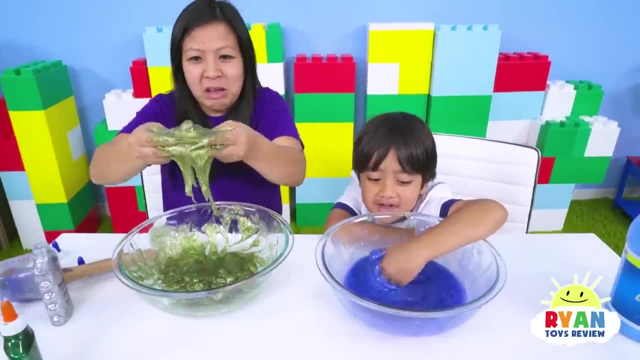 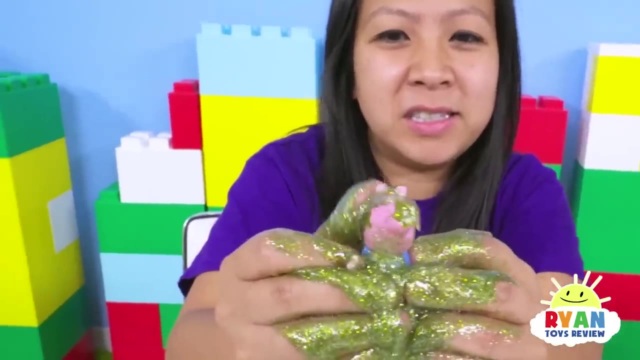 So what we did was I put a surprise toys in Ryan and Ryan, Are you ready to find it? Where is it? I feel somebody. I'm looking all around. Who's that? Do you guys know who this is? That's in slime. Oh, is this Peppa Pig's brother? 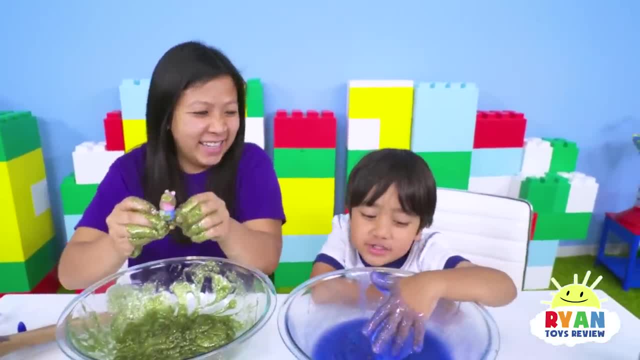 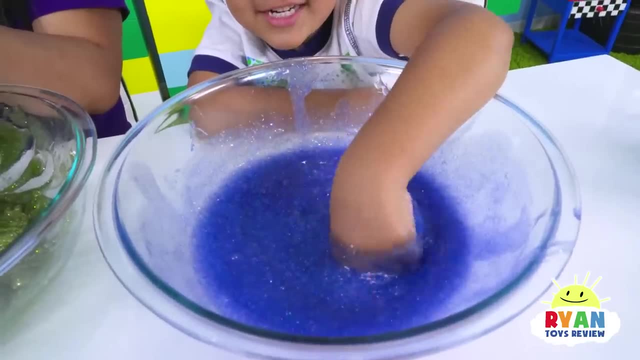 Hello, where's my dino? Is that how he says it? His name is George. Did you find it? Maybe it's in the middle. No, I don't feel anything. Maybe it'll be right here. Oh, it's something. 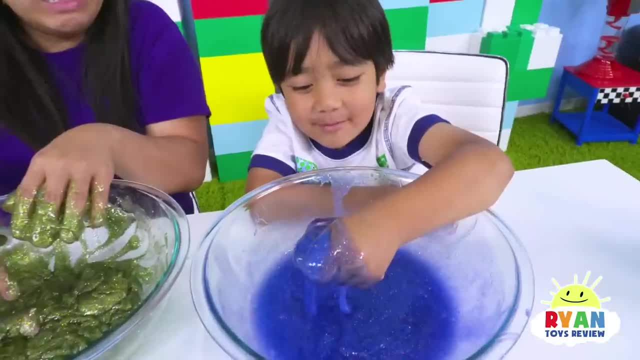 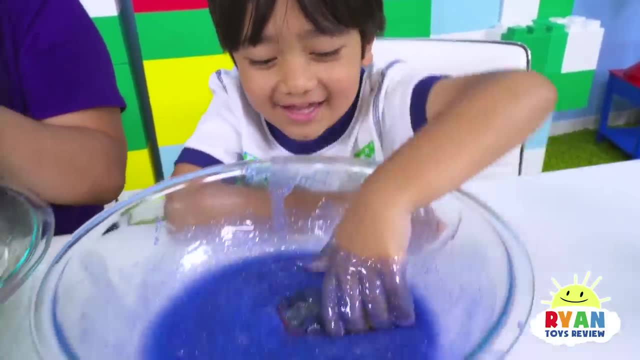 Oh, what is that? Ah, It's something red. Oh, something red. My hand is slippery so it's hard to like hold it. Yeah, what is that? Ah, Mine is. I can't even see it. 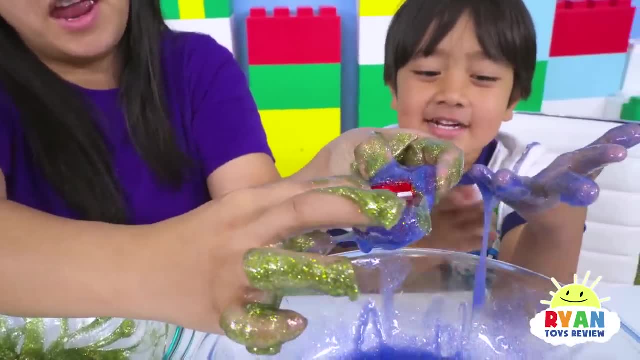 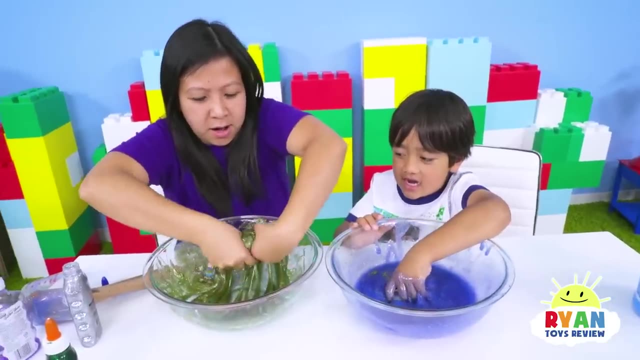 Nope, Here's Ryan. It is Lightning McQueen. I took some of your slime. Why don't we just combine the slime? So I'm gonna take my slime here and just dump it into Ryan. Look at that, Mommy. I think yours is. 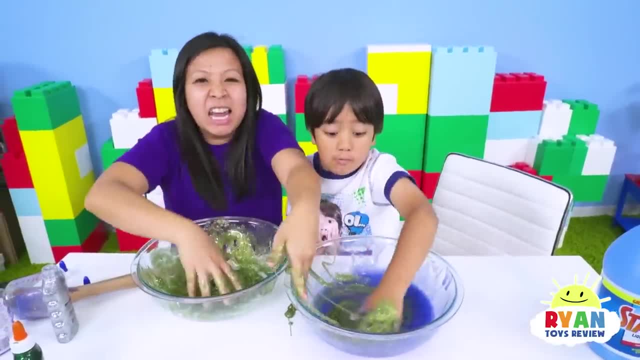 dissolving into mine. I know It looks pretty slimy, Wait. but Mommy, they're both dark, So which one's gonna dissolve? I don't know. Let's see which color. Okay, I'm gonna mix them in my. 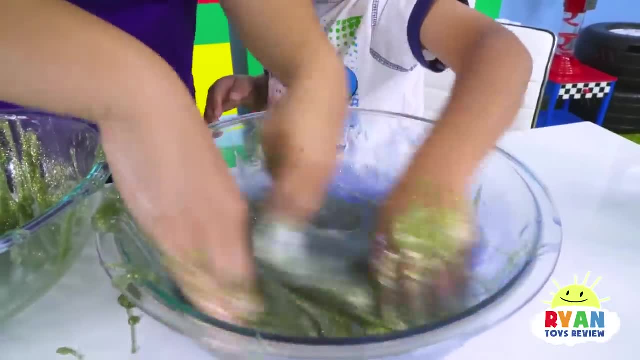 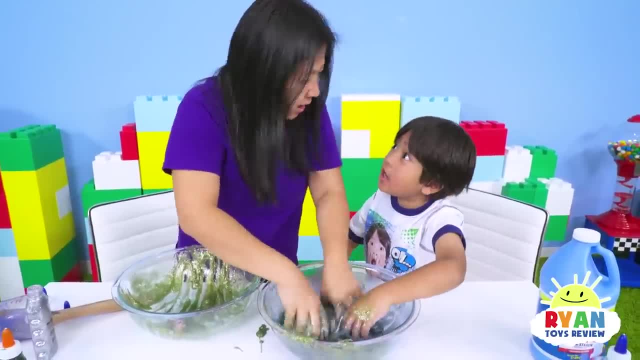 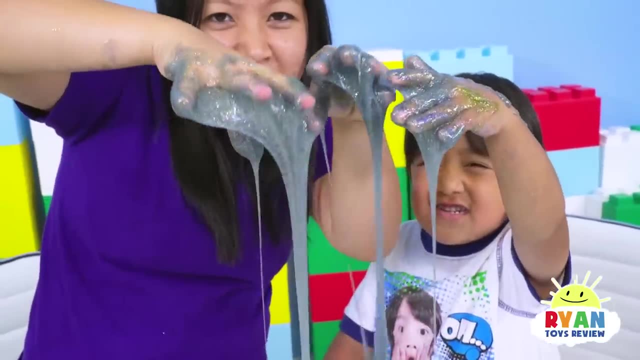 green. Wait, wait, Mommy. some of them looks like teal. It does Look at this color. It looks teal, but it looks washed out. Ooh, Okay, guys, we gotta take our slime. Whoa, Hey guys, Today I'm gonna make homemade. 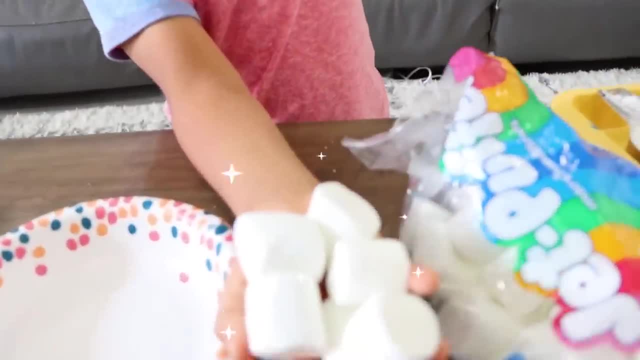 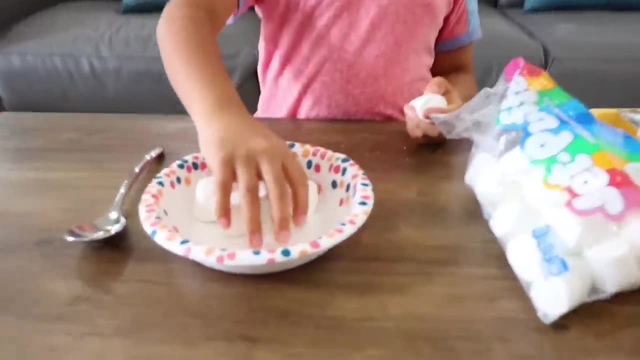 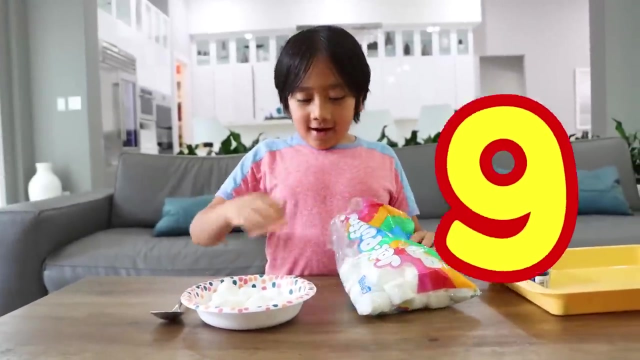 Plano with marshmallows. First thing you're gonna need is marshmallows. Here I'm gonna use ten marshmallows- Five already- Six, seven, eight, nine and ten. Next thing you need is half a cup of cornstarch. 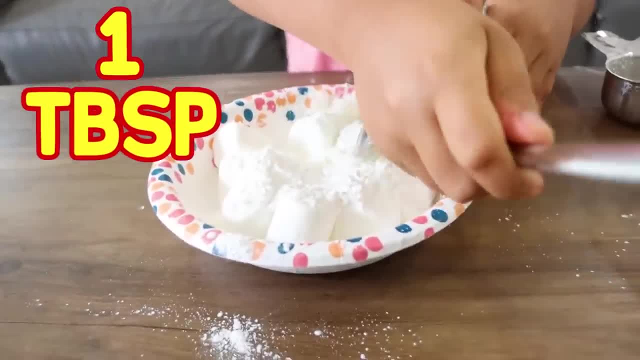 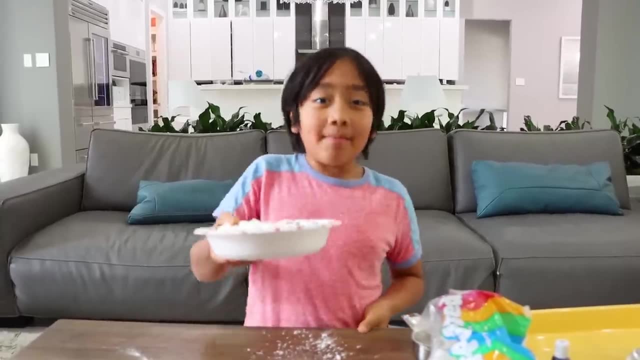 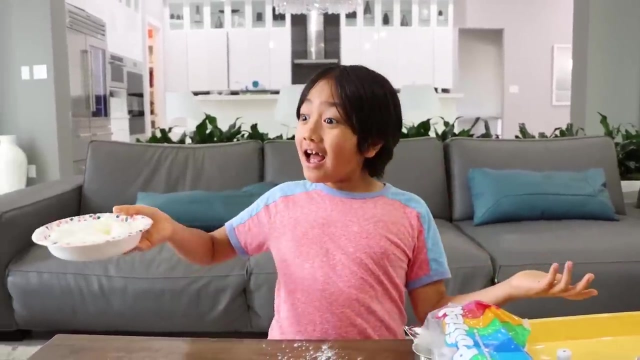 Next is one tablespoon of coconut oil, And there Next thing, ask your grown-up to microwave this for 30 seconds. Mommy, can you microwave this for 30 seconds? Of course, Ryan, I'm right here, Oh, oh. 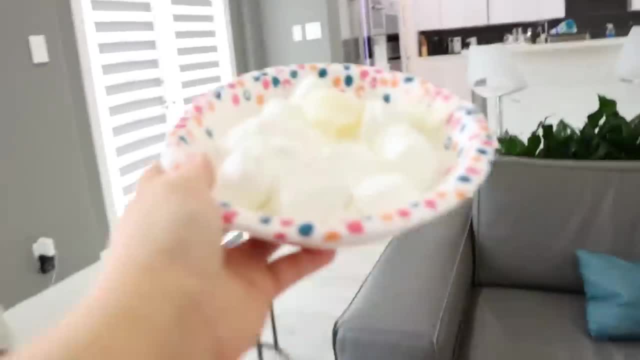 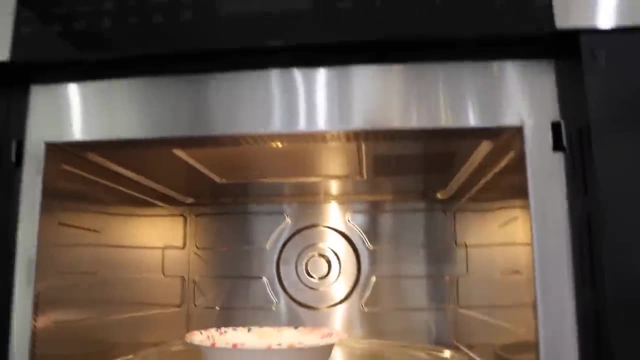 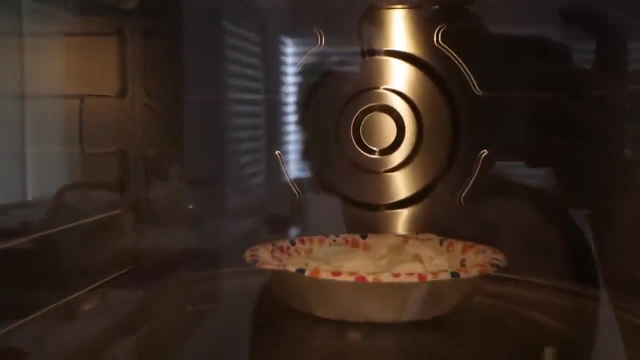 Thank you, Be right back. Okay, taking this to the microwave. Opened Microwave 30 seconds, Okay. and if you look here, notice what happened to the marshmallows. when you microwave it, The magic's gonna happen. 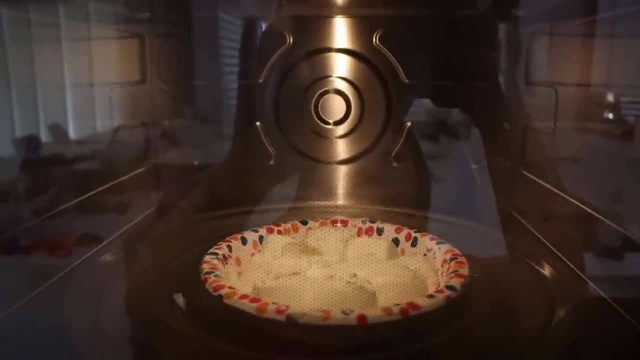 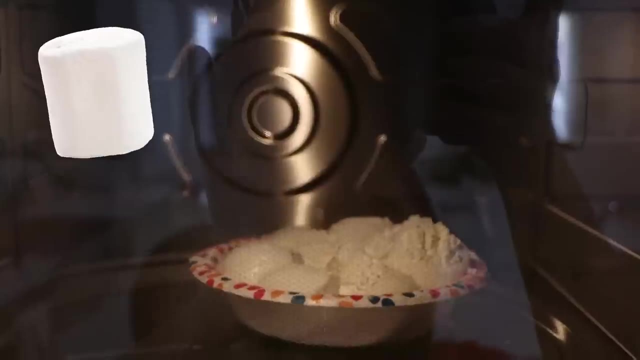 Well, I noticed what's happened, What It's spinning, But what's happening to the marshmallows? Did you notice? it got bigger or smaller? It's spinning. Do you see it? It's a giant-sized marshmallow. Oh, that's 30 seconds. 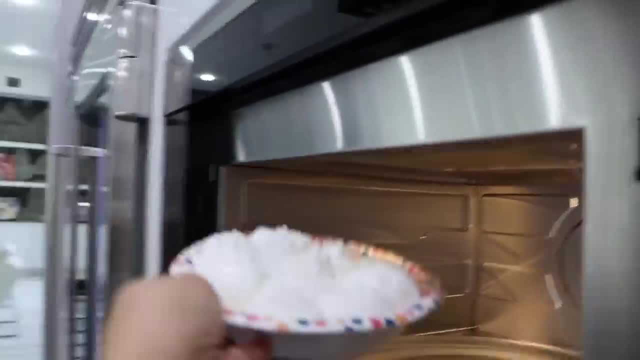 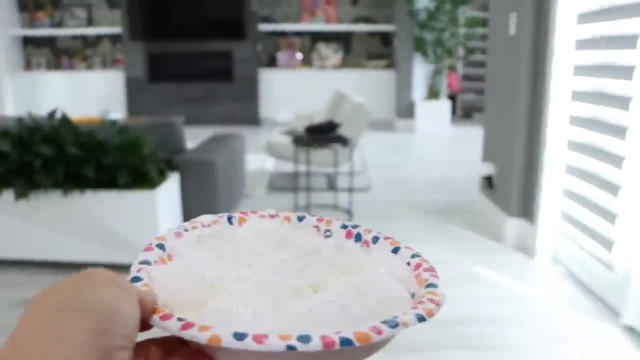 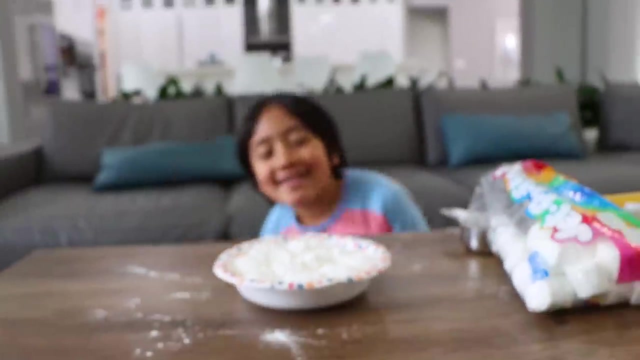 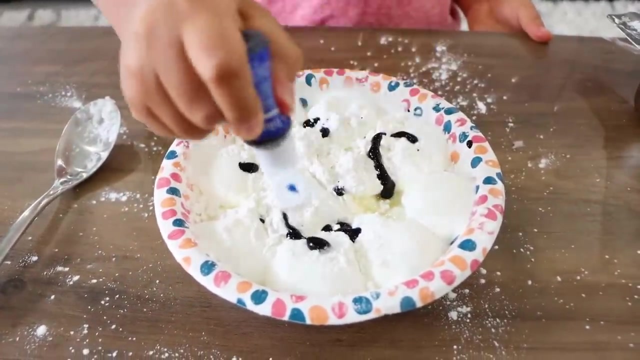 Okay, Yeah, Okay, Look, Wow, Do you see it? Okay, Let's bring it over. Smells like s'mores. Smells like s'mores. Yeah, Next, add some food coloring. Now I'm gonna agitate the blue food coloring. 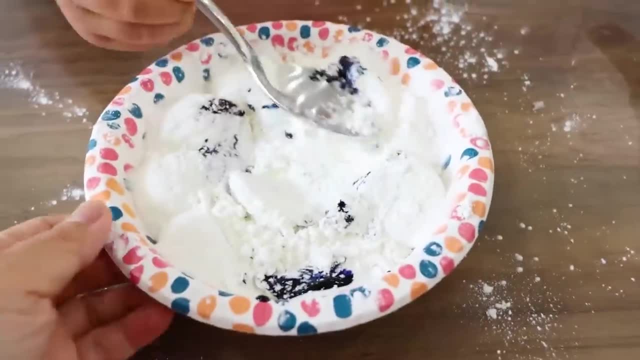 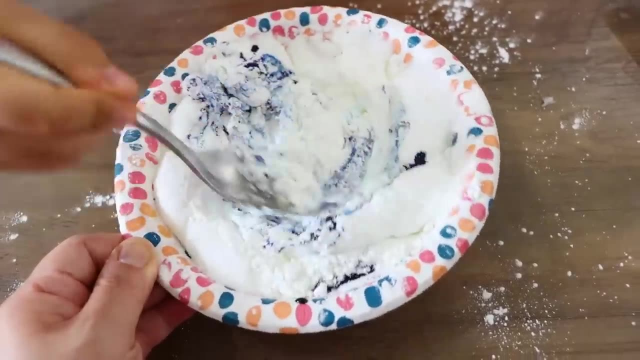 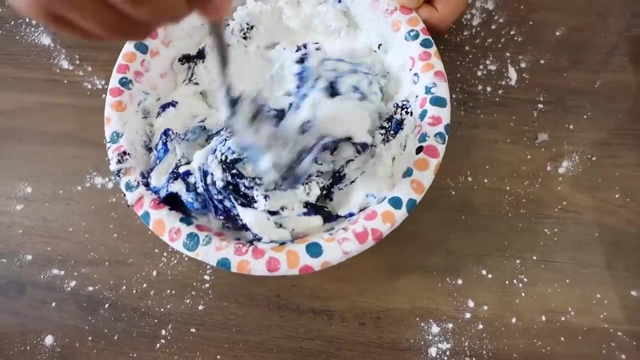 with the marshmallows. Okay, I'll hold it for you. Whoa? Okay, Exactly like mixing s'mores It does. huh, It looks kinda cool. Mix it all up. Mix it all up, Agitate, agitate. 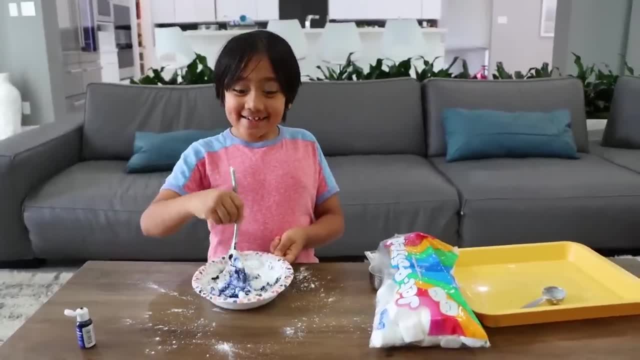 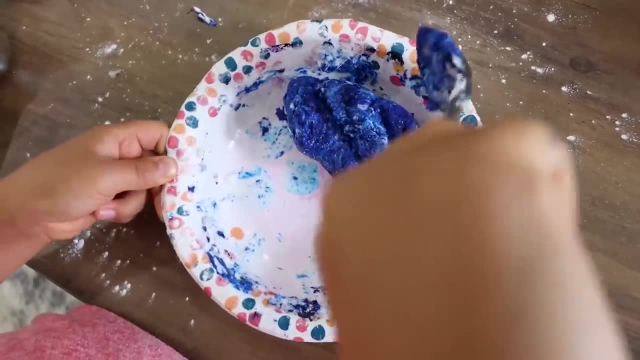 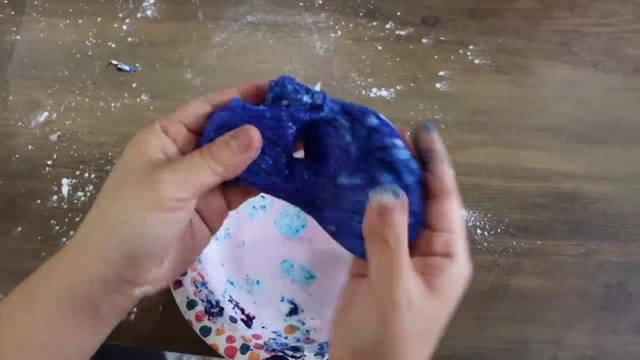 What's another word for agitate? Mix Or stir? Good, Okay, Mixing, Almost there. Good job, Almost fully blue. Alright, Now it's a little warm, so mommy's gonna take over, But all you do is just smush it. 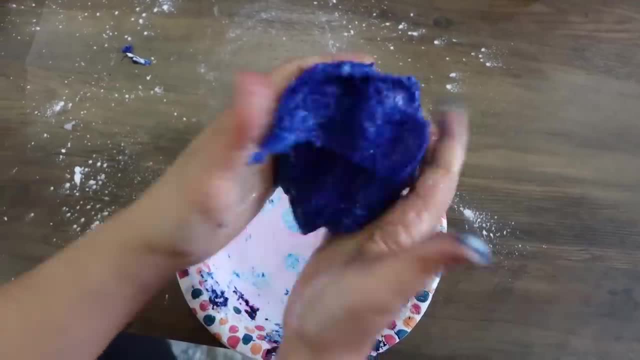 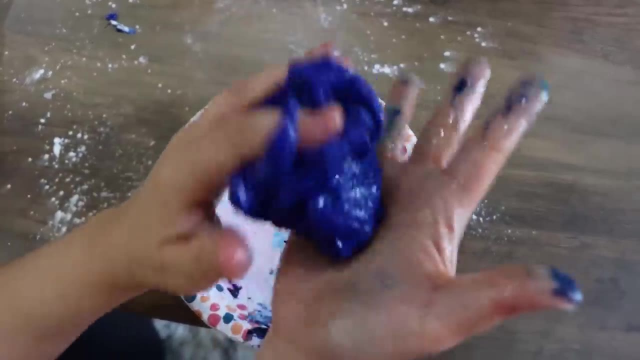 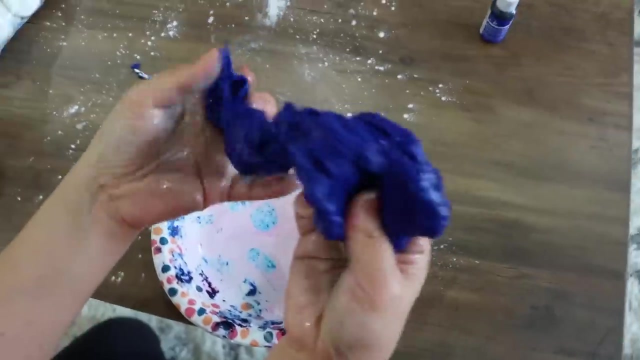 together like so Whee, It's starting to look like Play-Doh. Look, And then just, you can even roll it and twist it. See, Woohoo, Now that we have our blue Play-Doh, let's make the other colors. 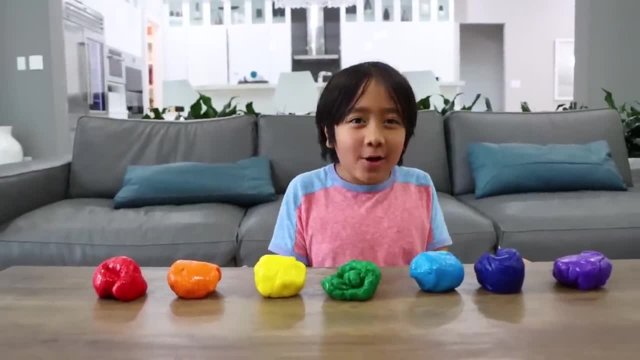 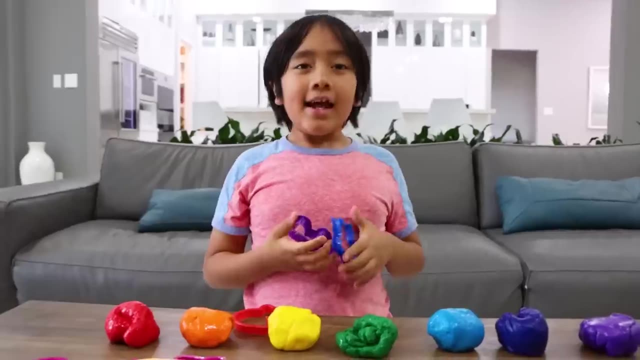 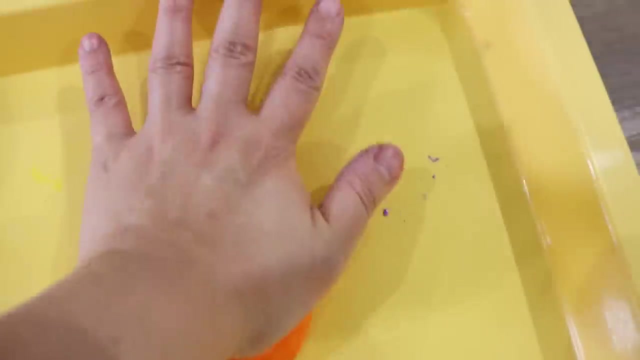 Yay, We have all the colors of the rainbow of Play-Doh Marshmallow. Now let's test it out. Okay, so first we're gonna just use orange, You just press it down, Okay, And then you put it in. 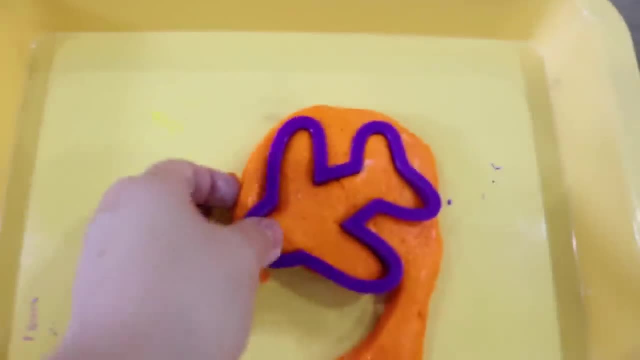 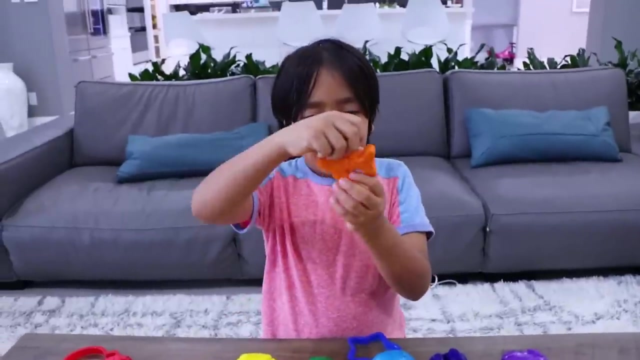 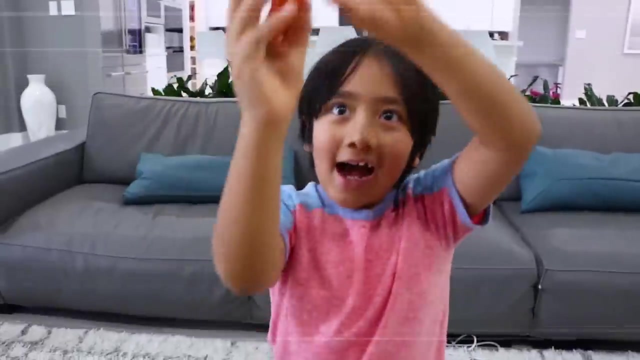 Okay, and now we're gonna take out the sides. Okay, Yay, Now we have an orange Play-Doh. Where you going? Where you going? Whoa, Watch out. Okay, now let's see if we can make a star. 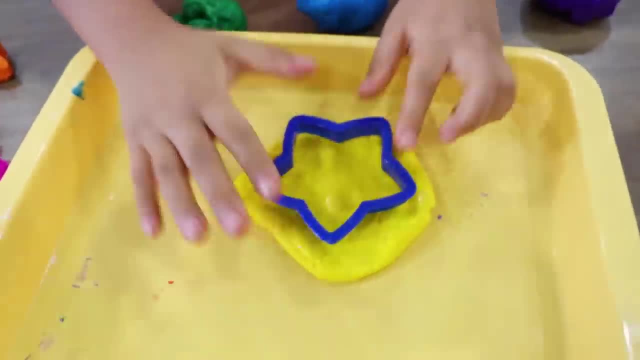 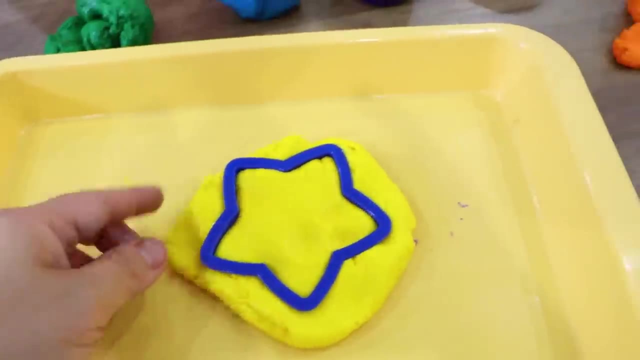 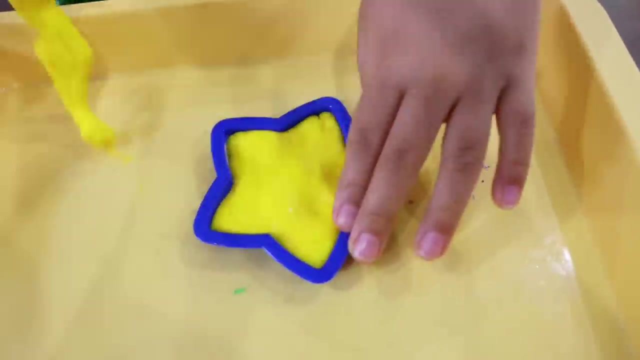 Okay, let's see if that fits, Okay. and yellow star: Okay, push it in. Nice. Teamwork, Can you hold this down? There we go, Lift up the outside layer and, bam, We got a star. Twinkle, twinkle, little star. 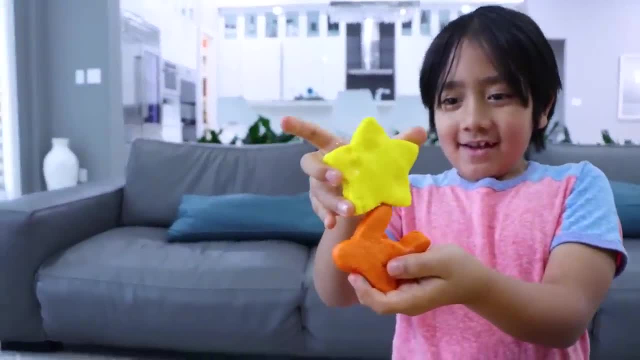 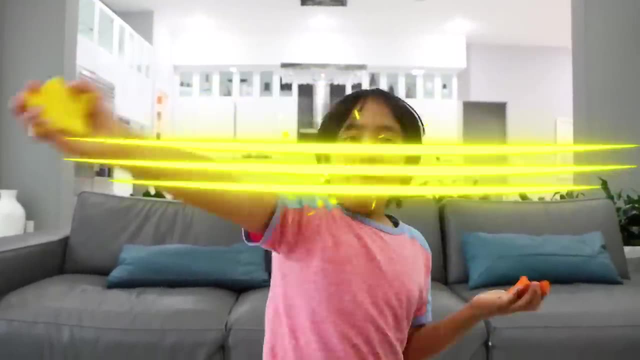 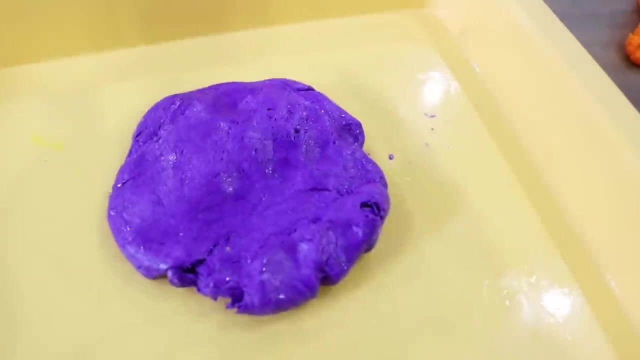 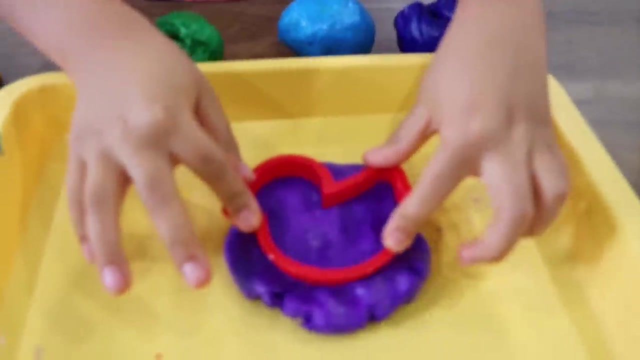 How. I wonder what you are. Star plane, What do you guys wish for? Shooting star, Shooting star, Okay. so now let's use purple, Okay, And now we're gonna make a ducky, Purple ducky, Why not? 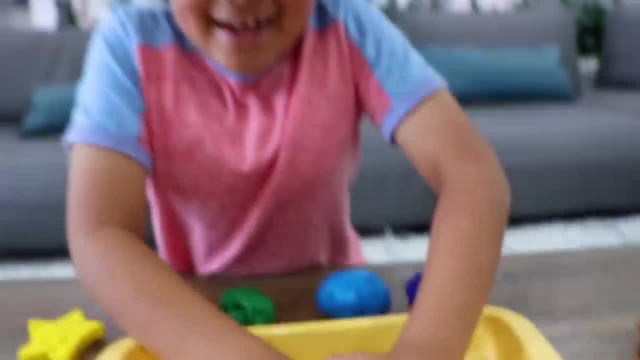 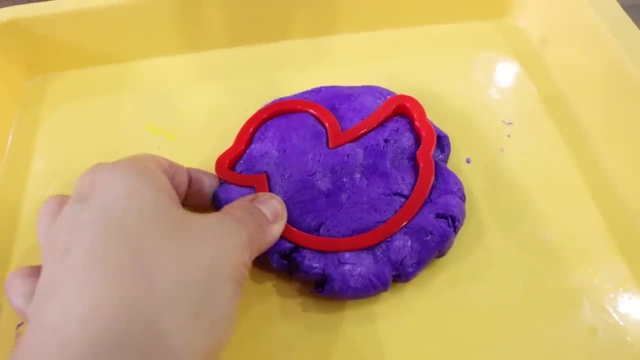 Plasma ducky, A plasma ducky. What is a plasma ducky? It's a ducky, that's plasma. Oh, fancy. Alright, Let me take out the sides. Whee, There we go. Do we have a ducky? 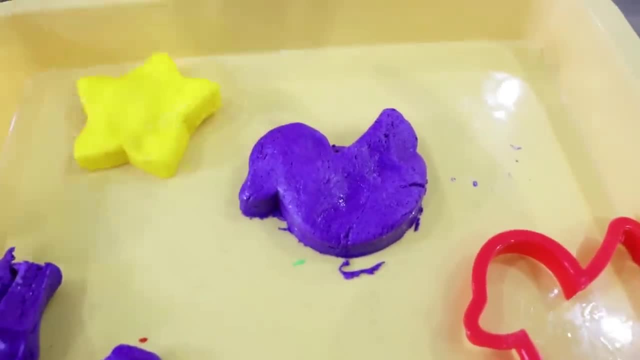 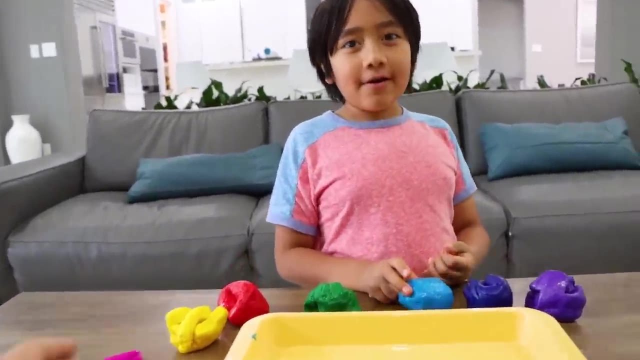 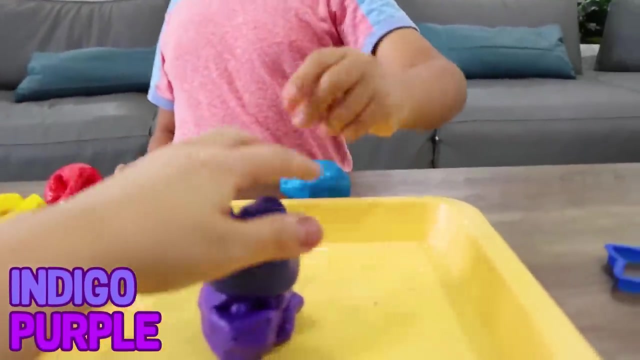 Yay, Star ducky, Star ducky plane. Now let's make a rainbow Play-Doh tower. Okay so, purple Indigo, There you go, Just smash, smash, smash, Smash on it, Then blue. 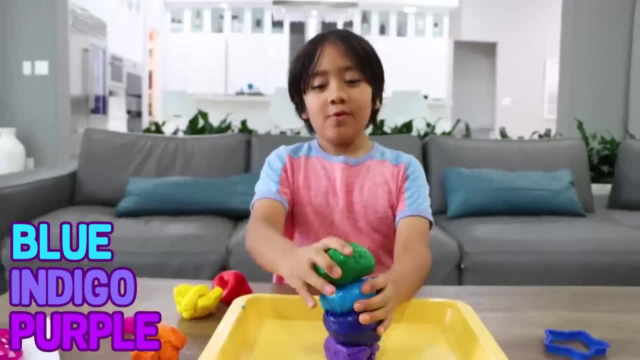 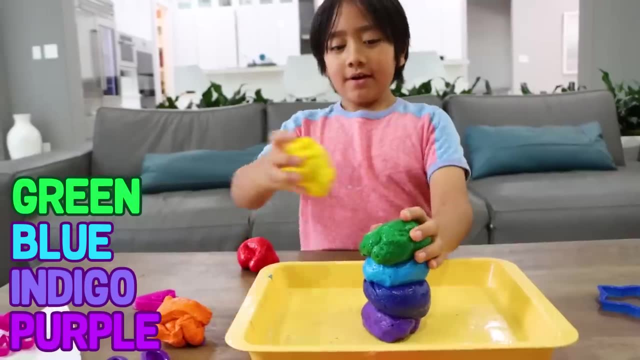 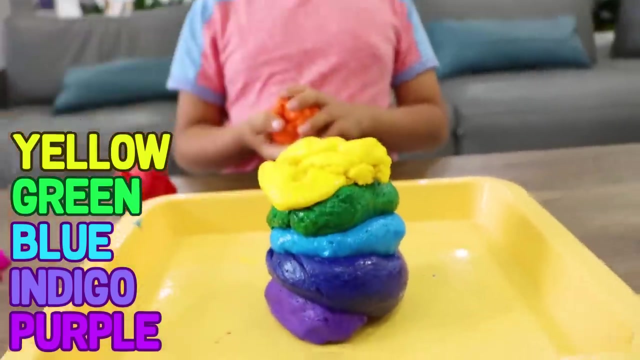 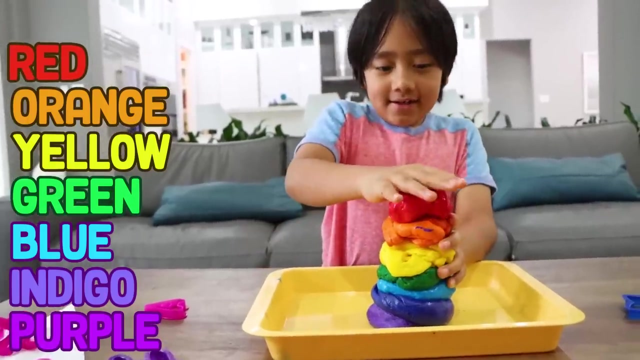 Ooh Blue, This might fall already. Green, Okay, Yellow, Nice, Is it gonna fall? Maybe, Let's see. Ooh, yay, Okay, orange And And red, Yay, Color the rainbow Play-Doh, Oh yeah. 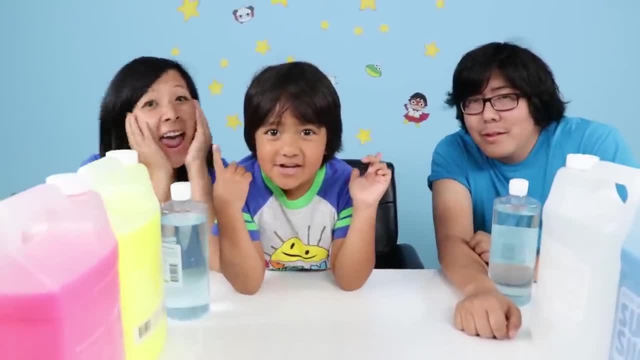 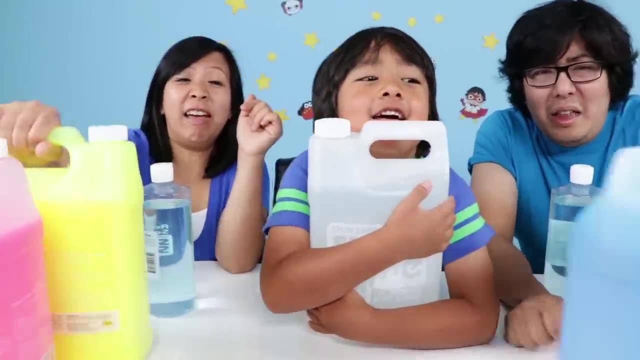 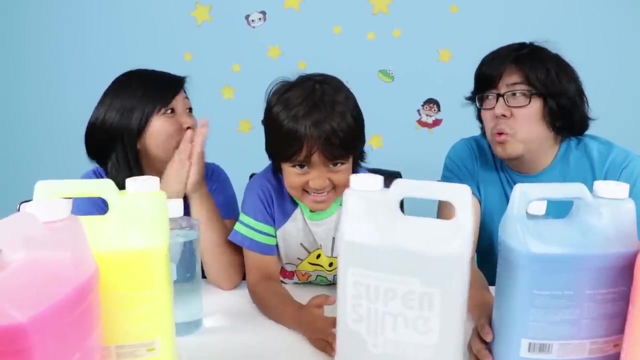 Today, my mommy and daddy are doing the super slime challenge. Super slime challenge. A lot of slime here, Yeah. there are a lot of containers here, Yeah, and whoever does the best slime creation wins. It's on, daddy, I gotta win this time. 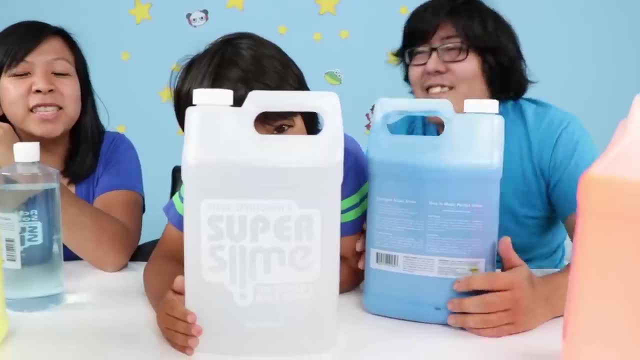 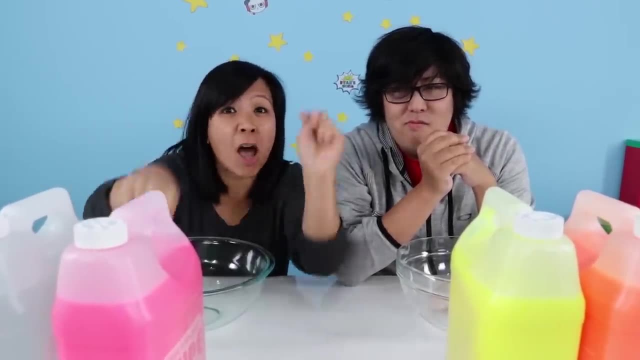 I never win so Easy with my eyes. Let the slime challenge begin. We're gonna see who can create the better slime and Ryan's gonna judge. You guys comment down below who creates the better looking art slime. okay, Those kind of challenges I always. 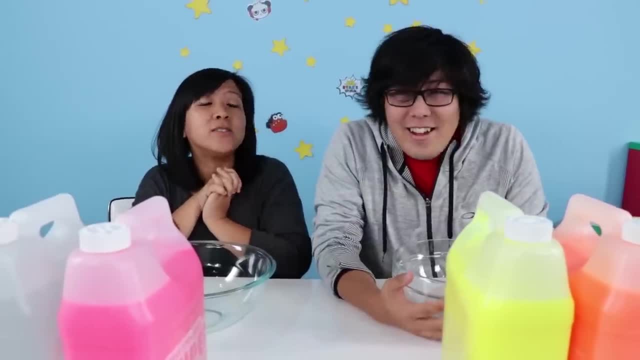 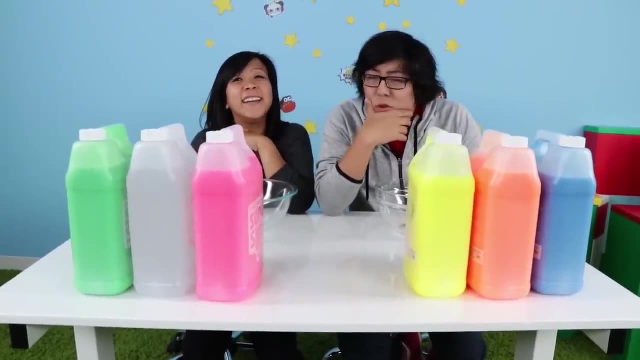 win. We will see. we will see. Alright, so since you think you're so good, I'll let you pick the first color. So many different choices. I know if you mix two colors sometimes it doesn't do well. 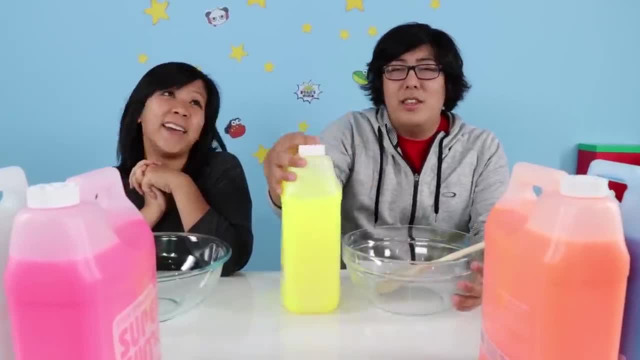 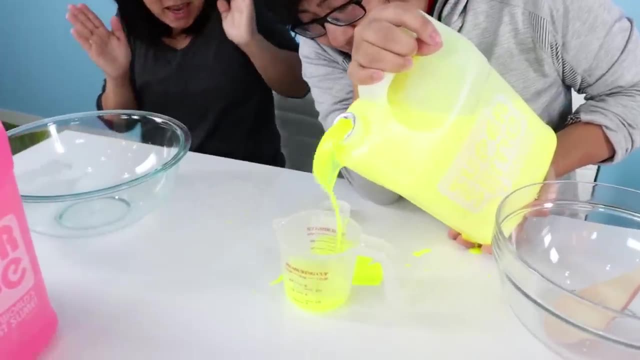 I'll pick yellow, Yellow. are you sure Yellow could go with many colors? Okay, Let's pour out some yellow slime, Yellow slime, but oops, I spilled some. You keep spilling it on the table. You're wasting good slime. 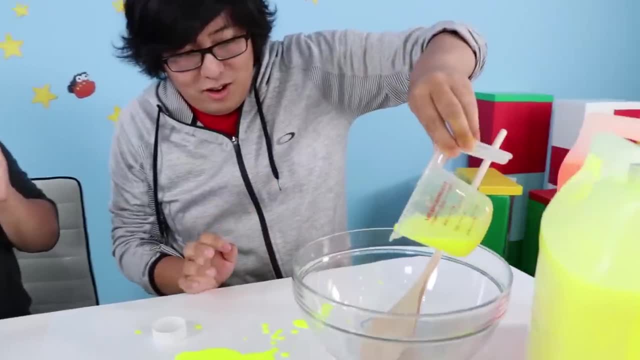 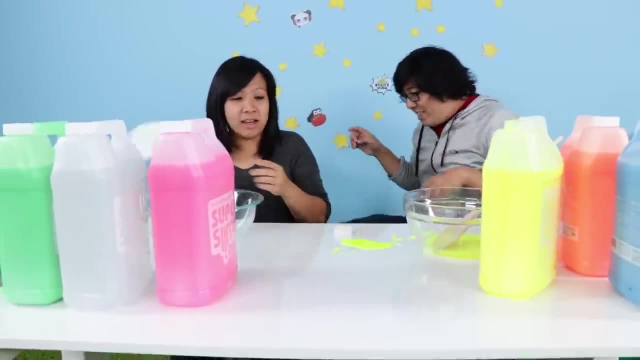 I'm sorry, And then pour in here. It is my turn. What color should I choose? There's so many colors to choose from. Maybe I should clean up first. Yeah, here you go. I think I'm gonna use pink, okay. 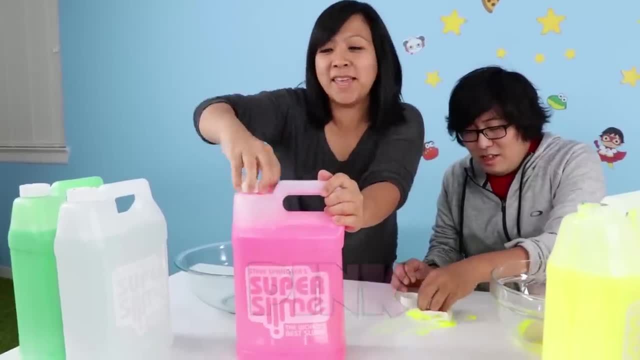 Who doesn't like pink slime? I was gonna get pink too. Too bad Pink slime. What do you guys think? No, Pink slime, Don't spill like I did. I'm not gonna spill it. I would be super duper. 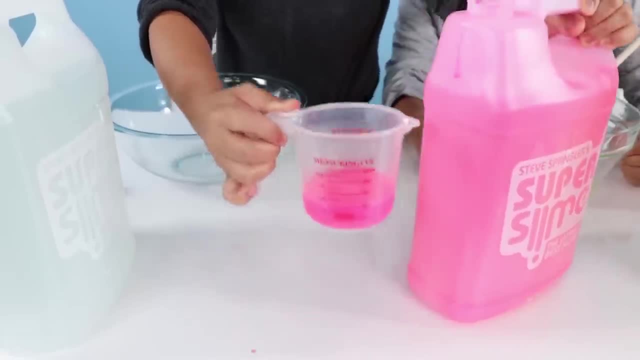 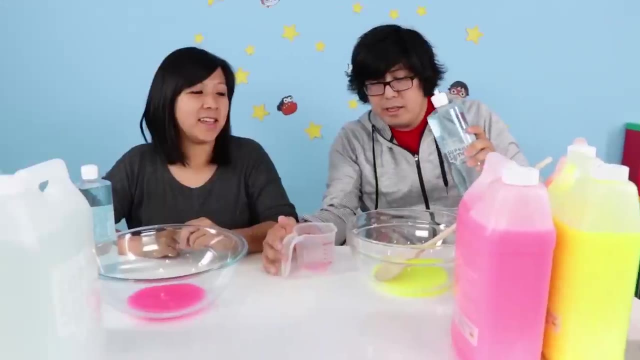 reach up here. Oh, good job, good job, Thank you. Look at this, In comes pink. Look at this Pink. Oh, that's so pretty. Let's add some activator. So this is like a very special. 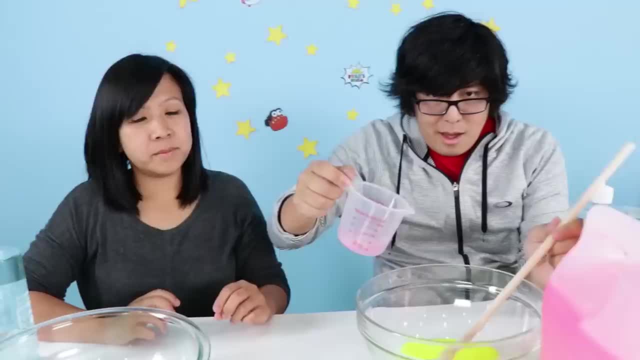 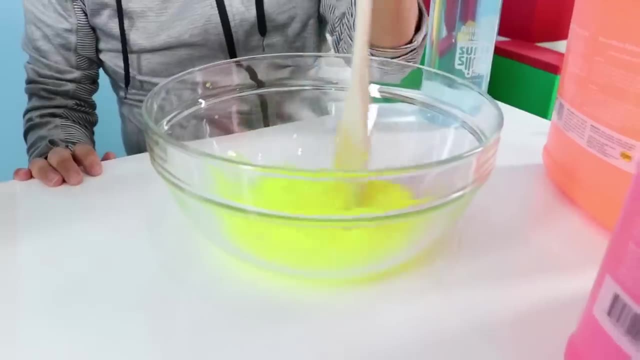 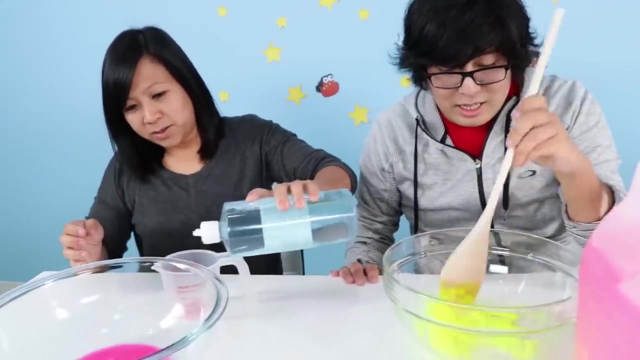 slime where you don't need glue, That's perfect. Yeah, Alright, let's add some activator And then mix it up. Ooh, I can already feel it's becoming slime. Whoa, That looks cool. Alright, my turn. 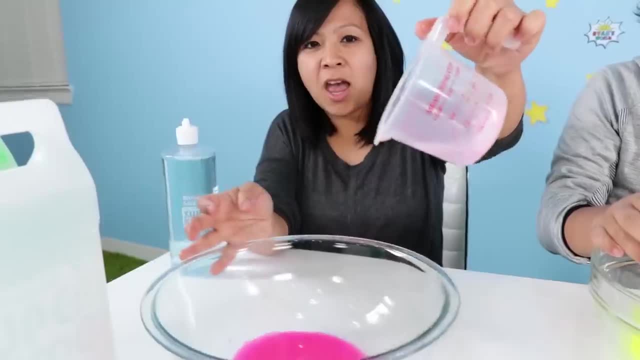 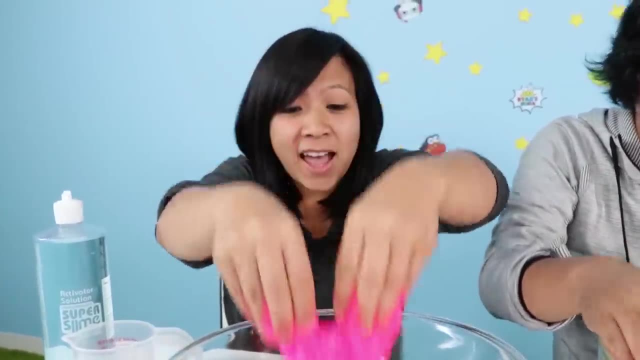 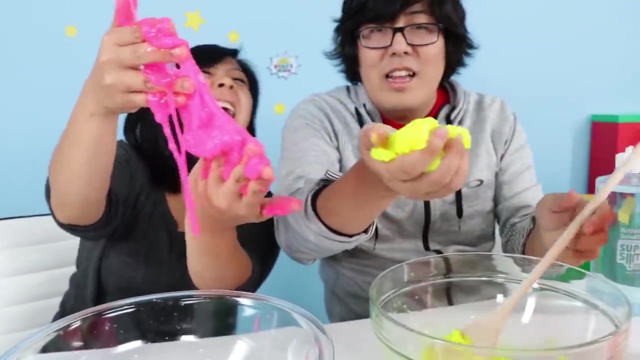 Activator in. Are you ready for some instant slime? Whoa, Already slime. Look at this. Yeah, That is super cool. Whoa. So here's my pink slime. so far, So far. who's winning? You can't tell. Mine's like a little too. 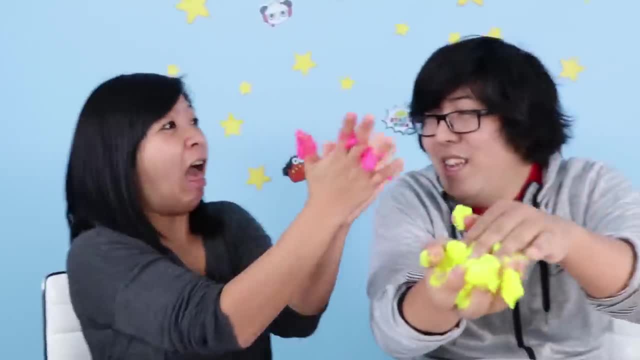 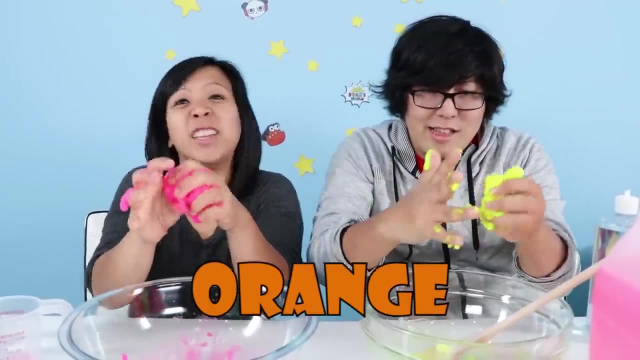 solid. I was just kidding. Don't spill it, Not on my face. What second color do you want to choose? I'm gonna pick orange. Okay, If you think that's a good choice, let us know. Be careful, be careful. 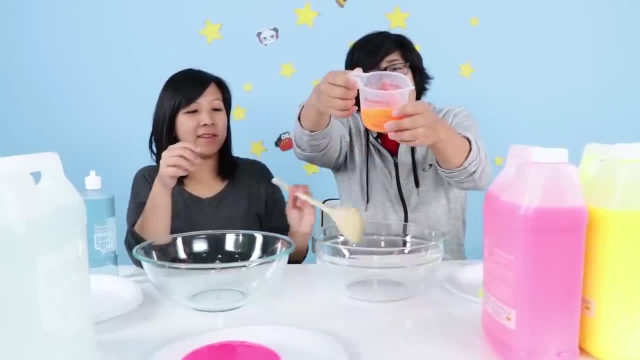 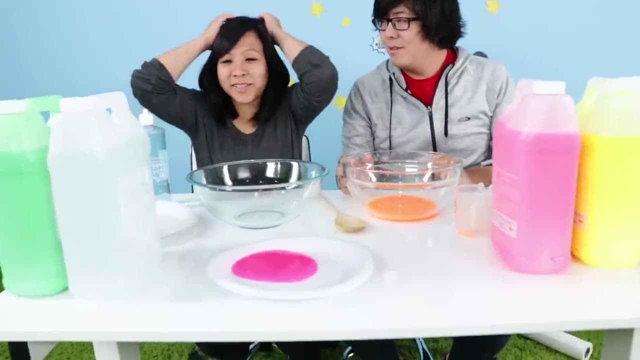 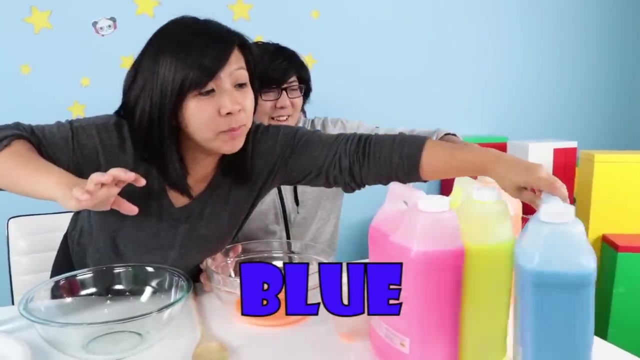 Done, Pour the orange into the bowl. Ooh nice. Ah, I don't know so many choices, I'm gonna go with blue. What do you guys think? Blue, Pink and blue, Pink and blue. Yeah, what's wrong with pink and blue? 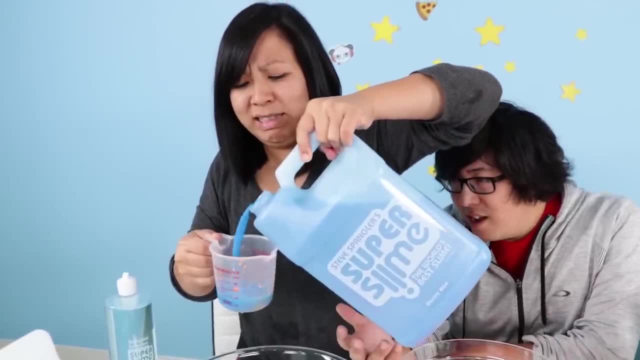 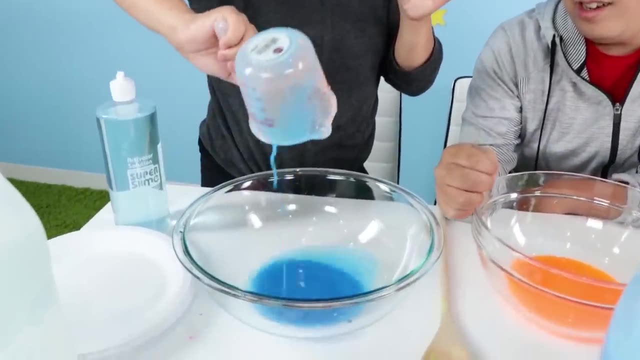 Are you okay? Ooh, you're so strong. Yeah, Too much, too much. I've been working out. Not really I've been working out, I was just holding the slime, Whoa. So now for the activator. 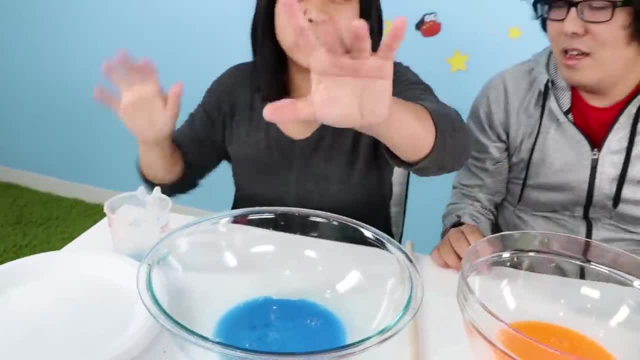 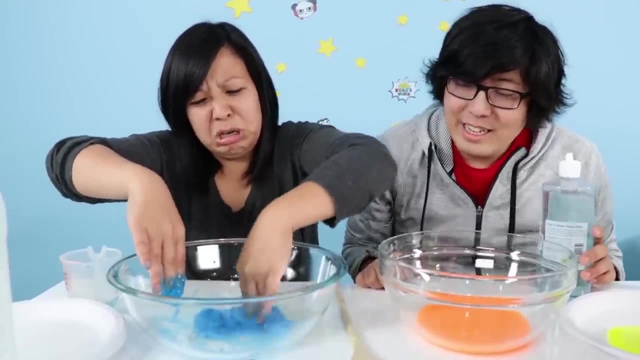 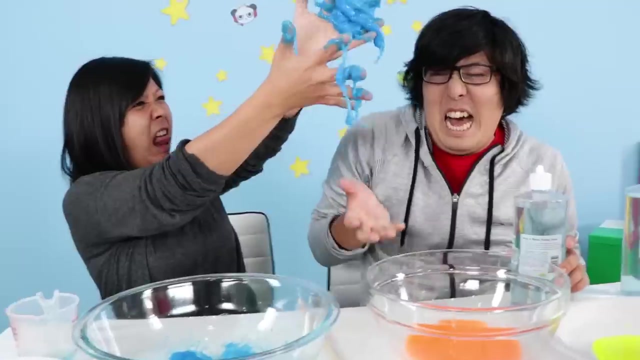 Slowly, slowly, Again using my magical hands here, Her magical hand, It needs my hand to mix it together. Oh, it's so squishy. Look at this, It's okay. It's okay, It's dripping. it's dripping. It's your fault. 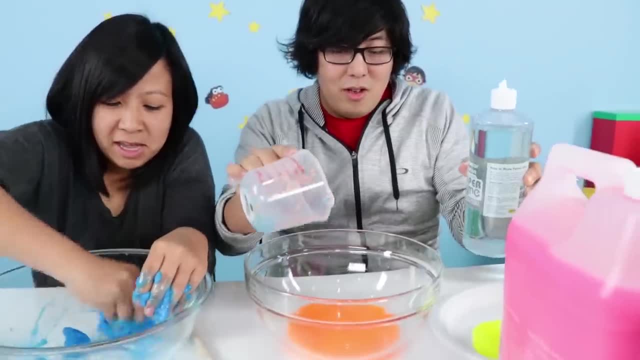 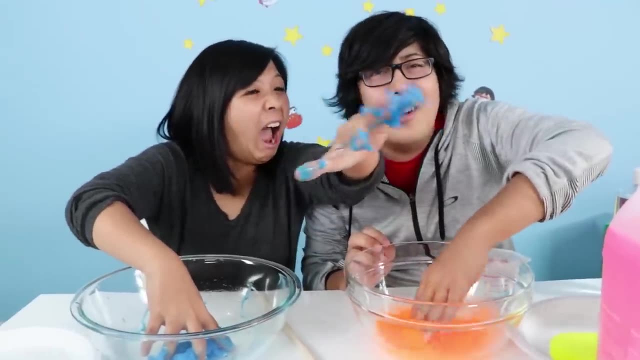 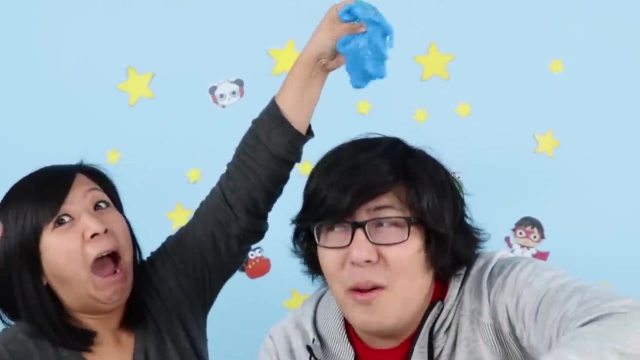 No, no, no, not to mine, My turn. No, don't mix your color. The blue and orange doesn't go together. Oh no, mine's still liquidy. Oh no, not my head. No, no, I felt it, I felt it. 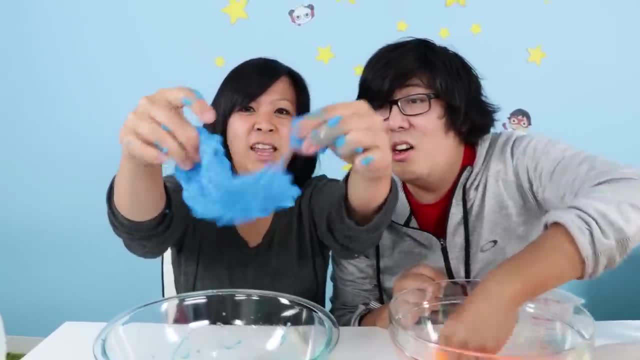 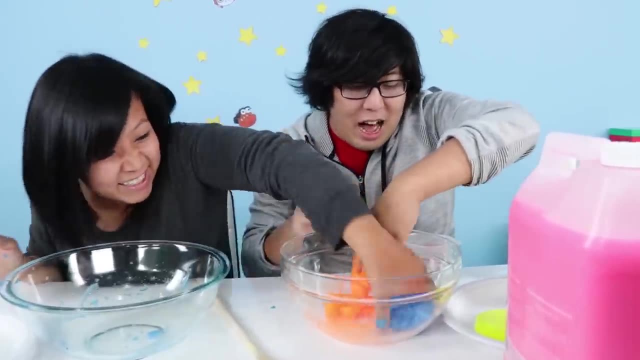 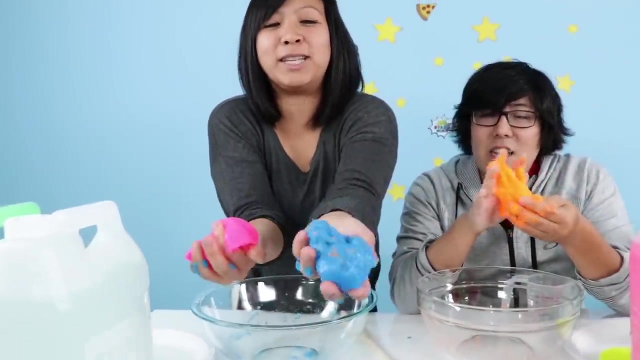 Well, this is really good slime. Look at this. Don't drop it. Keep dropping it, Sorry, Pay attention. Hey, Ah, mix it with my color. Here's mine. so far, I got pink and blue. That's mixed with. 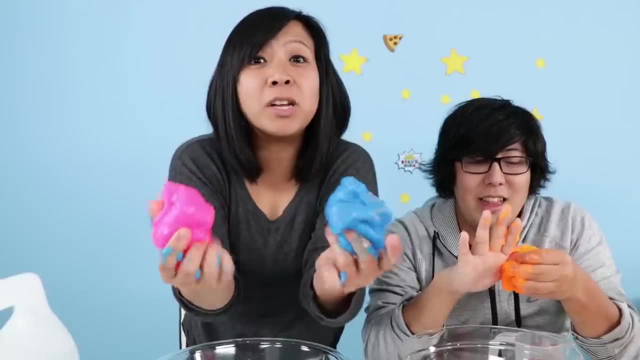 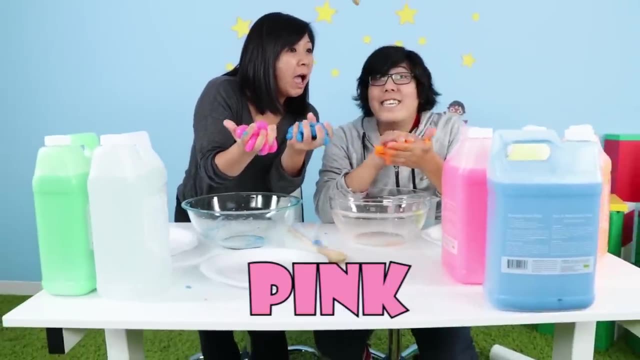 Shawn's orange. Are you gonna smash it together? We'll later. We're gonna smash them all later. okay, So we need one more color. What color are you gonna pick? Ooh, I'll pick pink, Pink, Yeah. 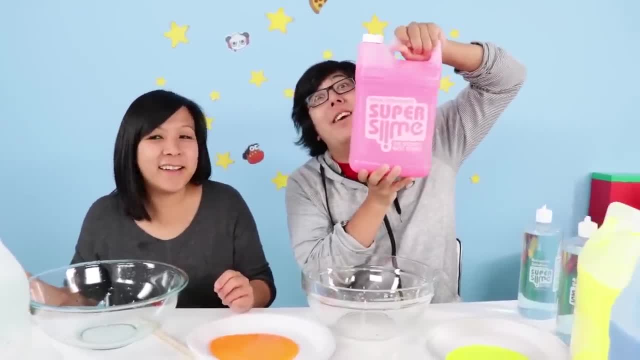 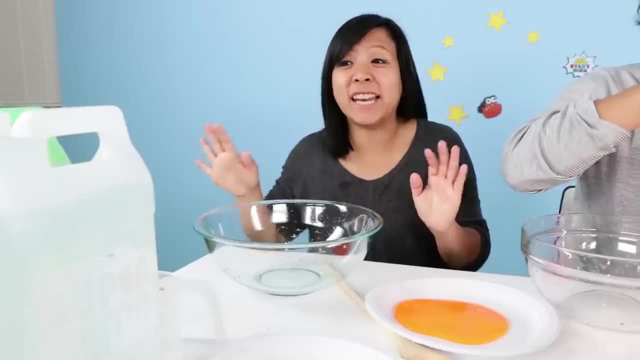 Alright, now it's time for the third color, Which is pink. for me, I'm gonna use clear, Okay. So because it's clear, we can put food coloring and make it any color. So we're gonna test it out to see what it's like. 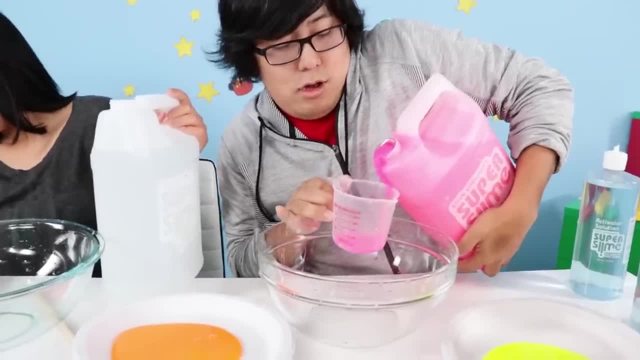 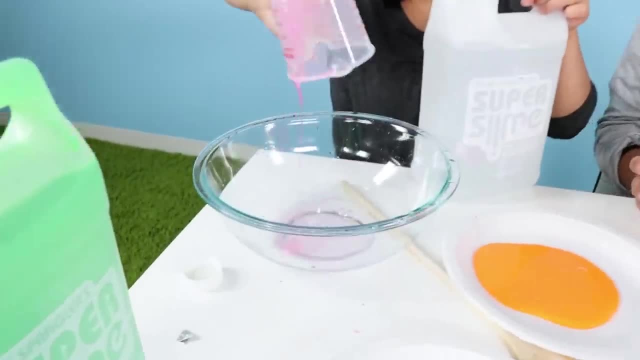 Whoa, that's not fair. Ugh, it's so heavy, Ugh Ooh, nice Ugh it's so heavy, Ugh Woo. Oh, it's not clear. It's like pink from yours. 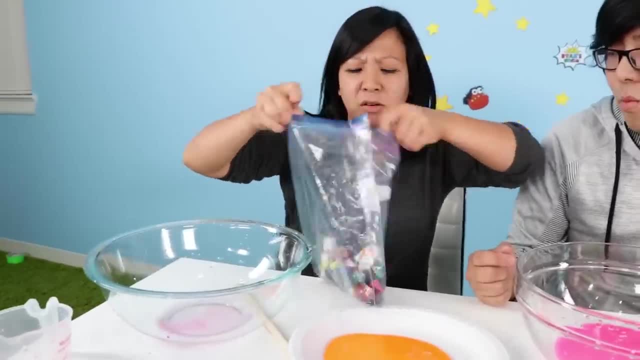 Not my fault, Ugh. Is that a batch of food coloring here? I don't know. I want to mix like two colors. Ooh. What color should I use? There's pink, There's blue, Ooh. 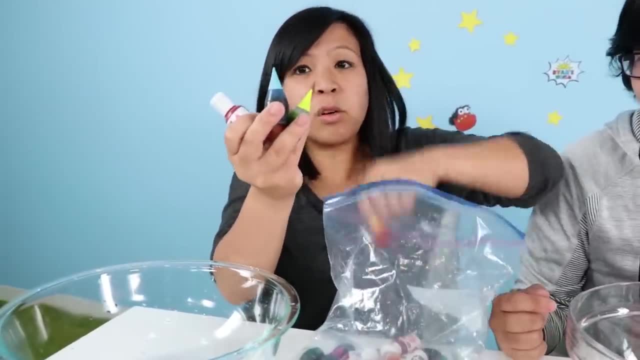 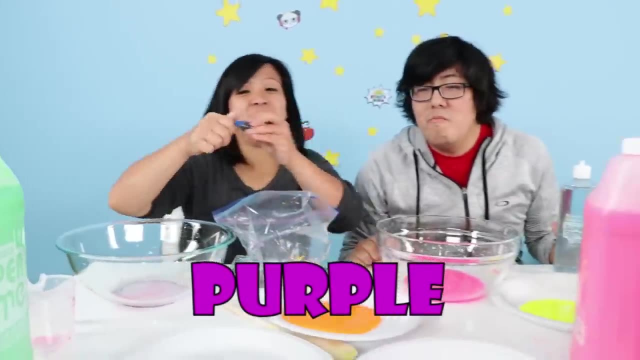 There's yellow: Ooh, What color should I choose? There's orange: Ooh, I'm gonna use blue and red together, because blue and red makes purple. So I'm gonna have purple slime. Ooh, Meet that, Hm, Don't add too much. 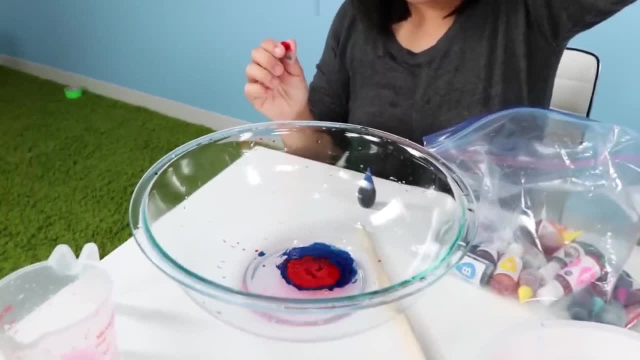 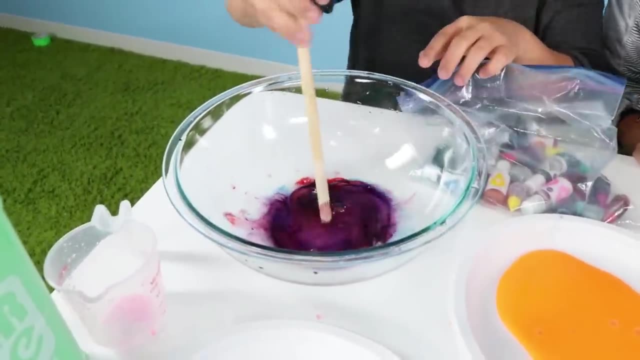 Two, Two, Okay. Speed drops, Yeah, It needs to be perfect. Boop, Okay. Ah, I think you put too much. Did I put too much? Maybe We'll see. Oh, no, It's too dark. No, I think it's coming. 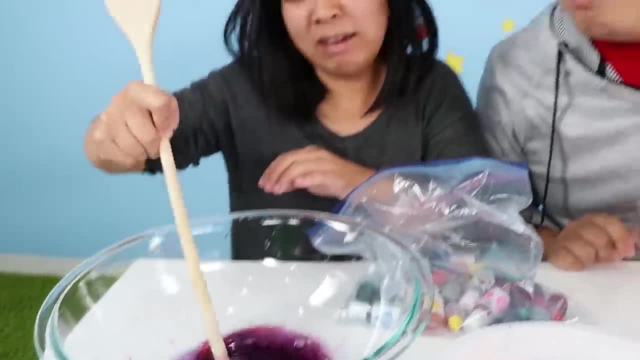 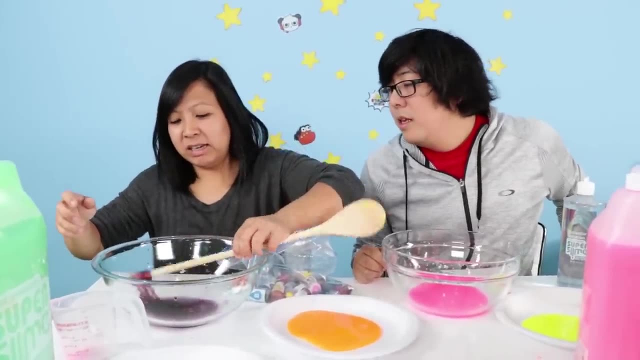 purple. I can see purple. It's too dark. Yeah, yeah, You put too much. Ah Activator- Whoa, It is purple. Yeah It is. It doesn't look. It's like slush, Whoa. 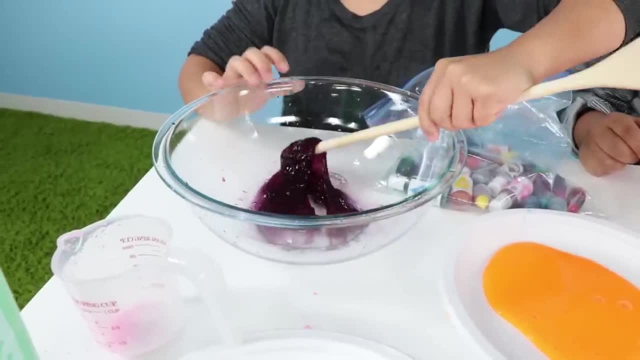 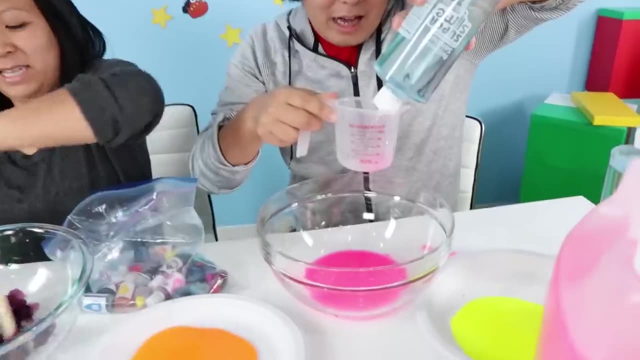 It's like slushy And it's clear color. Look at this, Whoa, I actually like it. Good job, Are you sure? Yeah, You're not just saying this Activator time? Mix it with a hand. 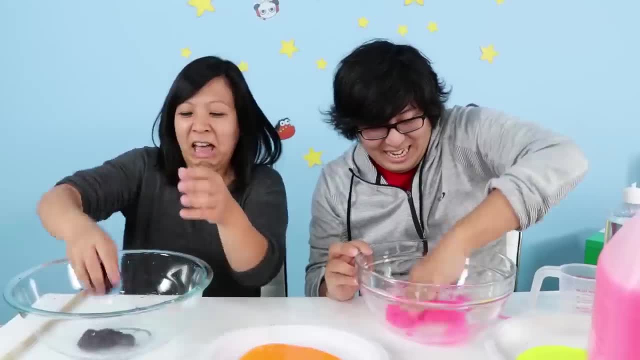 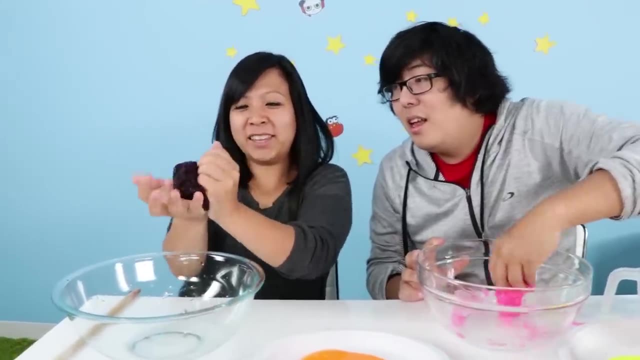 As usual, Ah, Ah, Sorry, Sorry, Sorry, Sorry, Messy. This is my purple so far. What do you guys think? I think it's a little bit too dark. It doesn't have the neon color as the others. 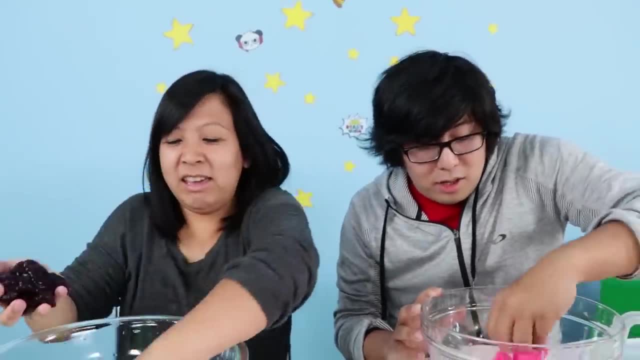 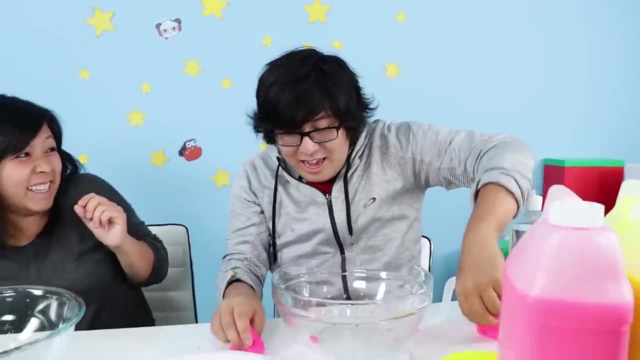 Right, Yeah, But you're gonna mix it with other colors, That's okay. Yeah, Look at that, A pink color Coming out, nice, Ah, Hey, It's okay, You're just jealous because mine came out so nice. 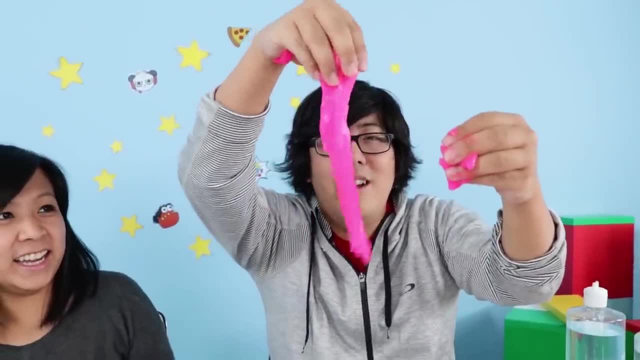 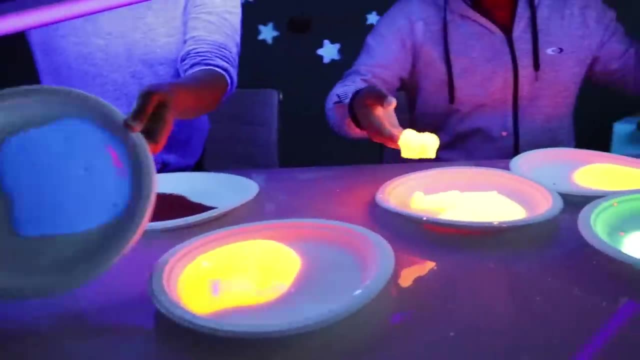 Yeah, It looks really nice. I can stretch the bubble bed too. now, Guys, look at our glowing. Look at this. Whoa, That's pretty cool. Look at mine- Whoa. Look at that. Yeah, The color glows. 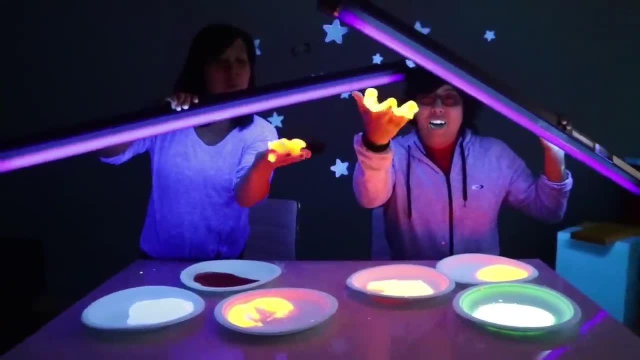 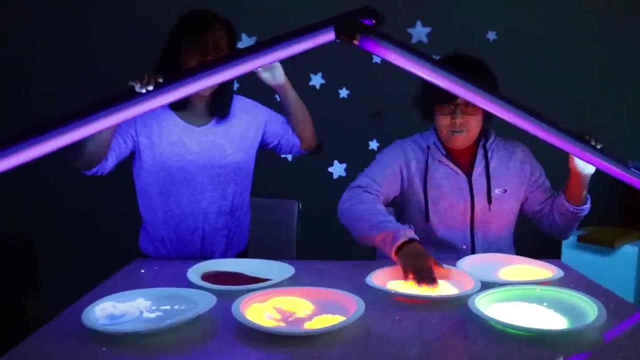 That's so cool. It looks like lava. It's hot, hot, hot, hot, hot. I like the green one. It looks like a nuclear. Yeah, Let's turn our back on the lights. Here's for the fun part. 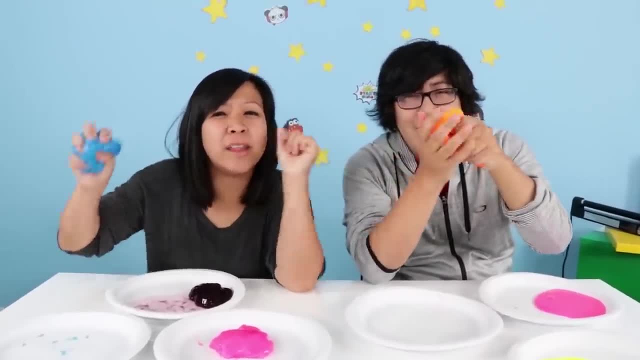 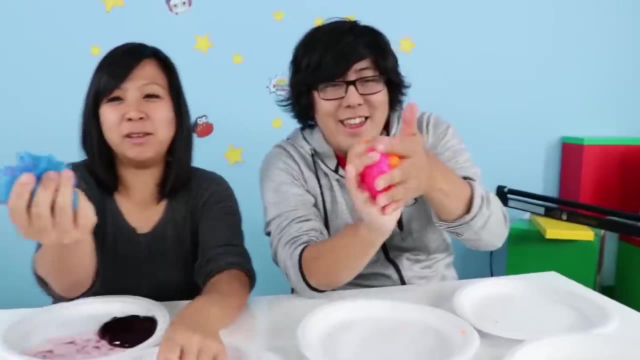 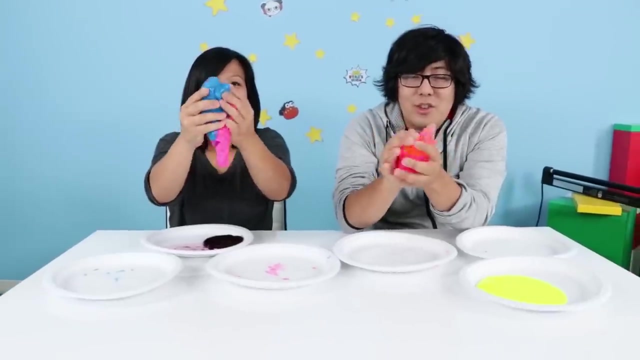 We're gonna smash our slime together and you guys let us know who create the better looking slime. okay, Mine's gonna be the one. Pink and orange. Boom, I'm gonna use pink and blue. It's fun squishing it. Yeah, What do you guys think so far? 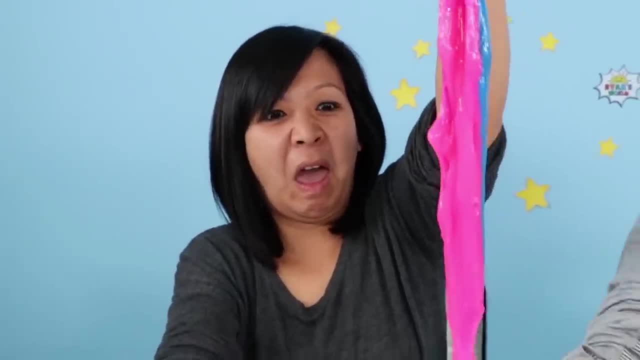 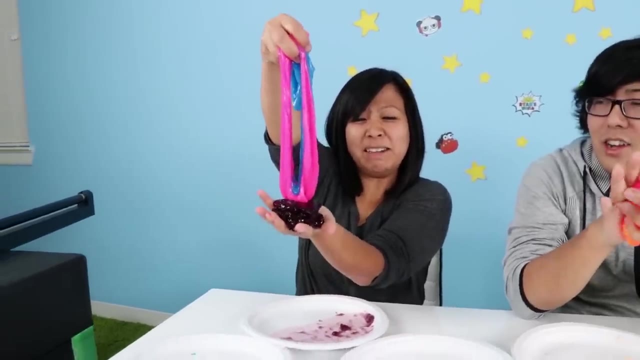 It looks like a snot, It's dripping. Hold it. Hold it. Now for the third color I'm gonna put in my purple. I don't want to. The purple doesn't look good with it. It's not gonna look good. 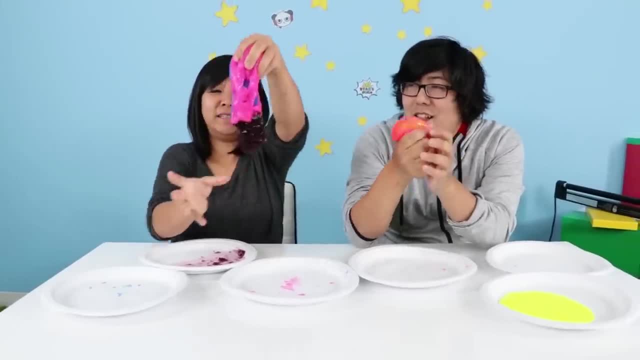 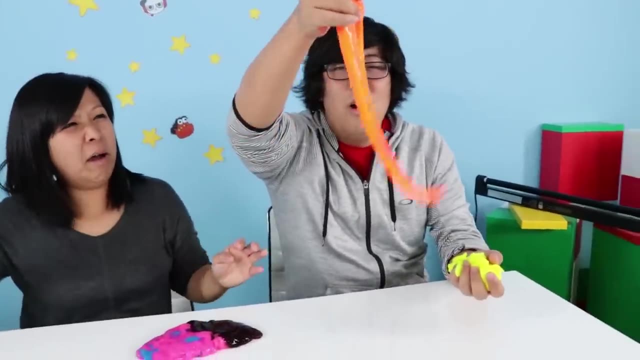 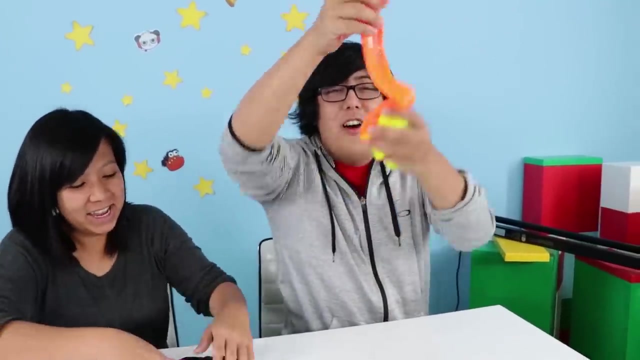 Yeah, Yeah, Yeah. What do you guys think? Am I winning? Sorry, Am I dripping, Still dripping? Oh, Be careful when you're swinging it, Don't punch it. Don't punch it, It's not for punching. 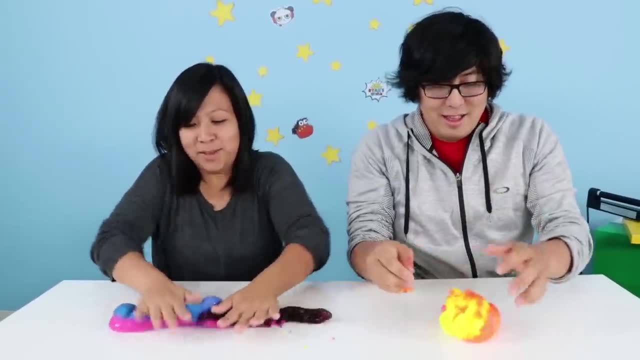 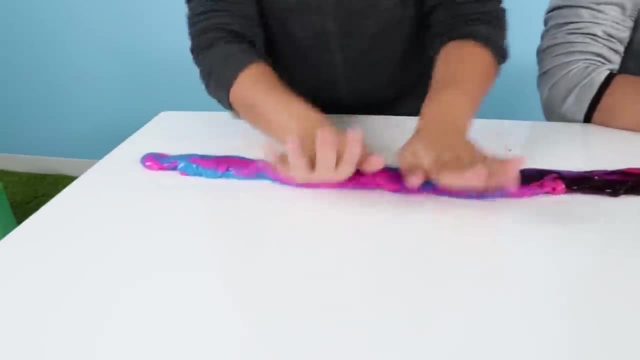 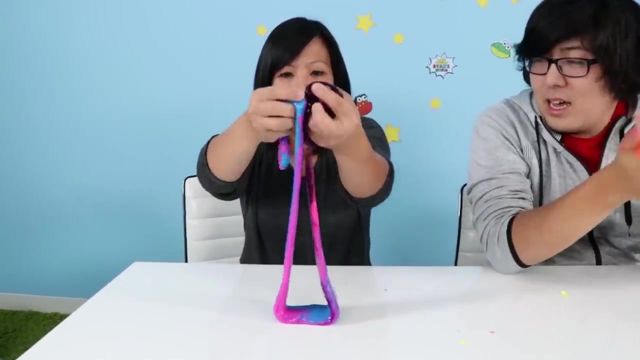 I'm mixing it with yellow. You can roll that on the table. It's bouncing. Look at this. My slime is super long. Look at this. What do you guys think about my super long slime? It looks like a galaxy space car. 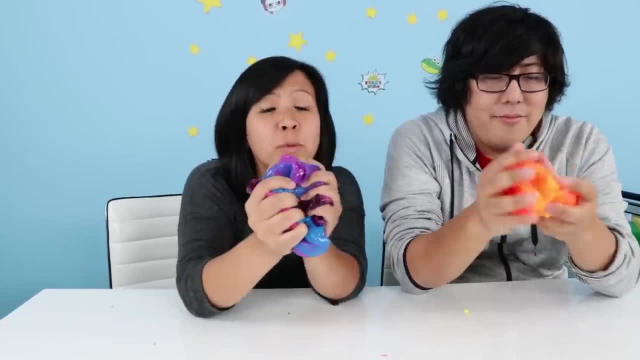 It does, doesn't it? It looks like I'm in space. It looks kinda cool. You know what's so cool about these? If you let it sit overnight, it's gonna create a really cool looking art piece. Oh really. 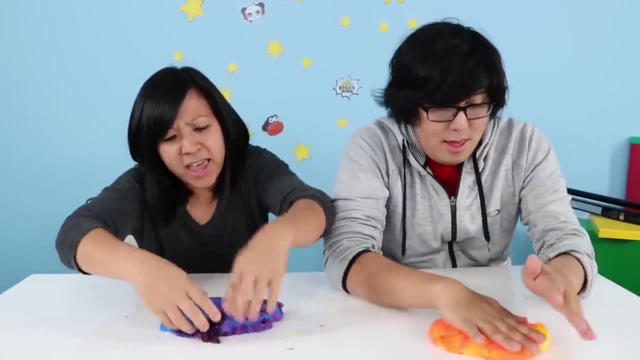 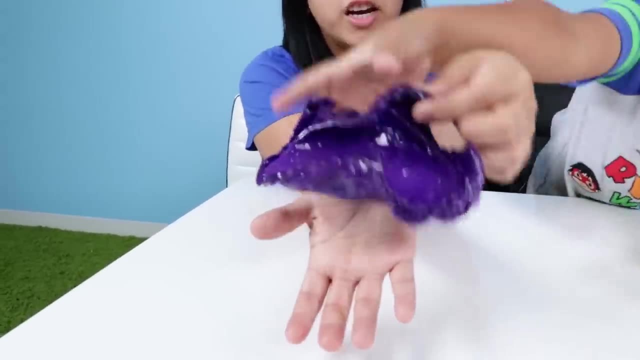 Can I make a shape? Yeah, so we're gonna make a cool shape right now and then come back tomorrow. okay, So we let our slime dry for a couple days and this is what it looks like. Some cool slime art here, I don't know. 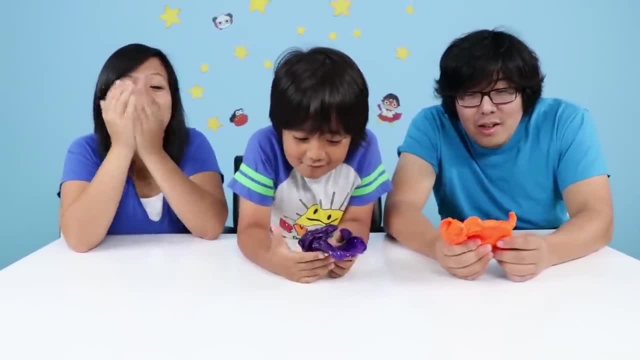 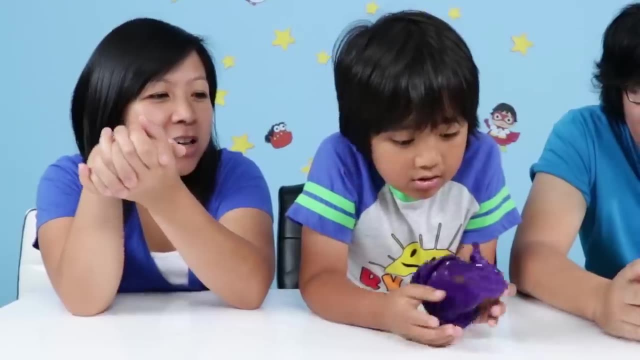 about cool. You don't know about cool. You don't think this is cool. You guys made like pretty much nothing. We worked so hard on this. Yeah, all our colors just kind of smashed together, So we actually had three colors. 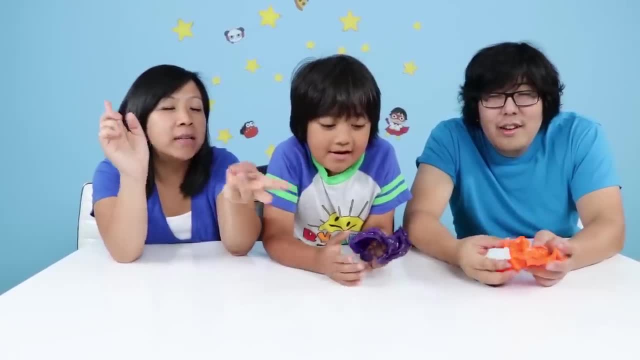 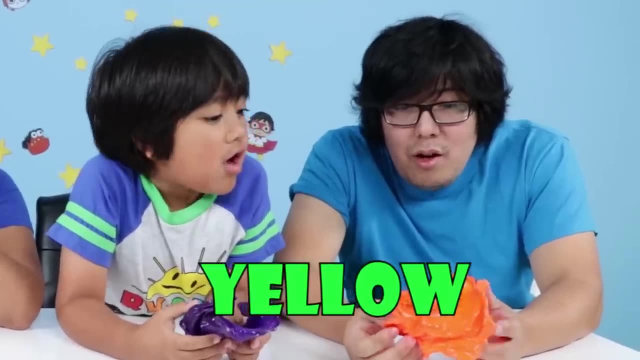 Ryan, I actually used pink, purple and blue. Oh, and the strongest color was purple. Yeah, And Daddy actually used three different colors too. I know Mine was yellow, orange and pink. Oh, that means the orange. 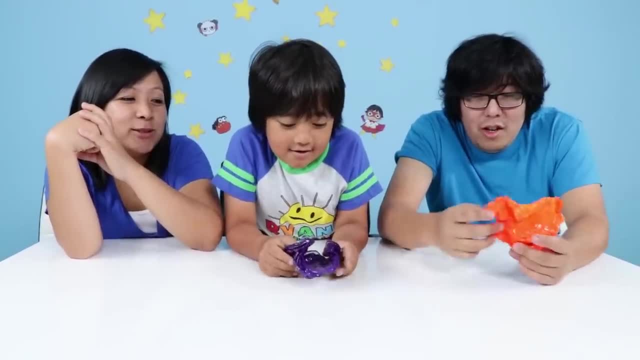 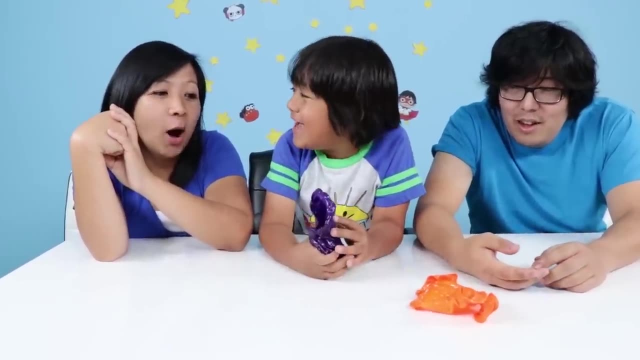 was the strongest one. No, Everything just became orange. Okay, so who won? I know it's just so hard to choose. I'm gonna judge this one First. let's see who's more breakable. Oh no, don't break this. No, don't break. 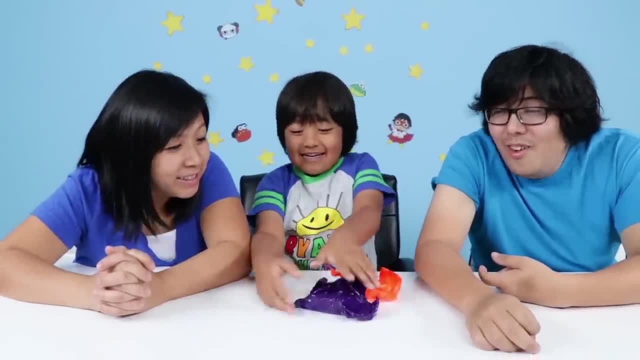 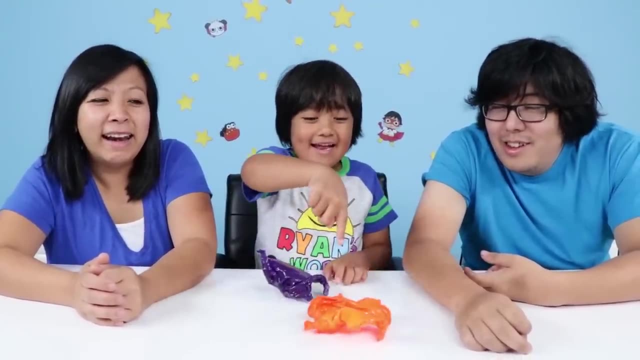 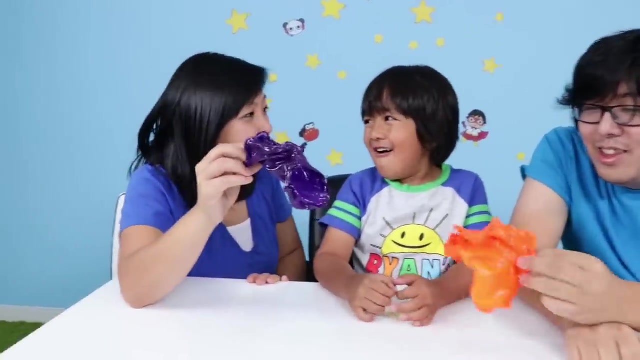 this slime? no, This is our piece. Ah Ah, Three, two, one Daddy. No, Daddy won, Thank you. What's wrong with mine? Mine looks cool. Yeah, what was the winning point of this one? 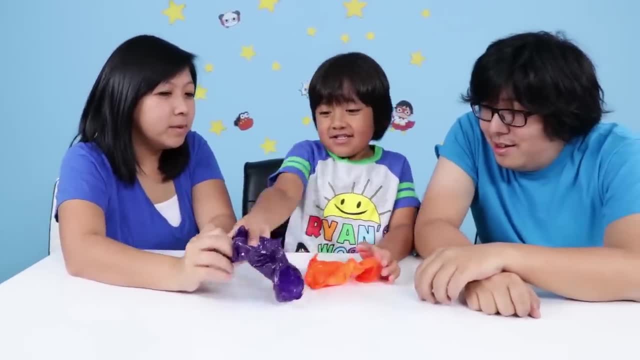 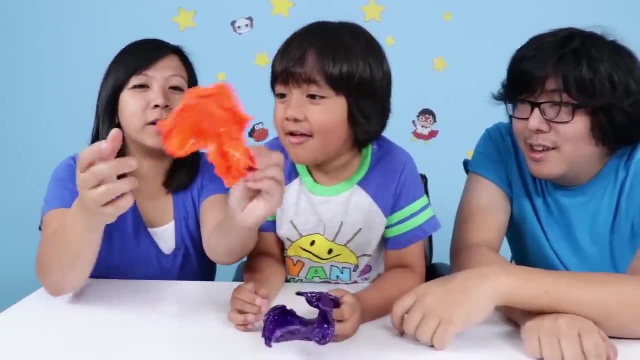 Yeah, why did Daddy beat mine? Because I can barely see anything. The way the shape is. You like Daddy's shape one better? It looks kind of like a fidget spinner. Oh yeah, Haha, That's not meant to spin. 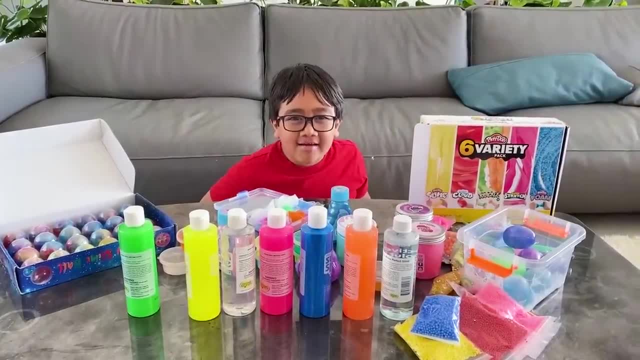 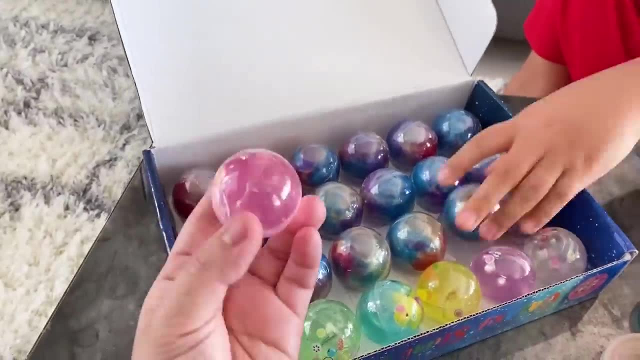 Hi guys, Today I'm doing the mixing all my slime challenge. Here's all the slime. Okay, so these are really cool. These are my favorite. These are galaxy balls And this one's clear, But look, it's like. 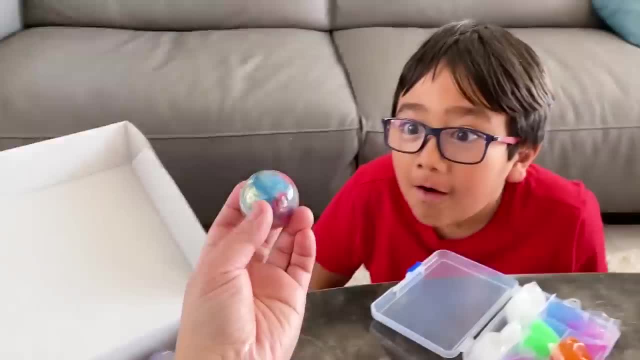 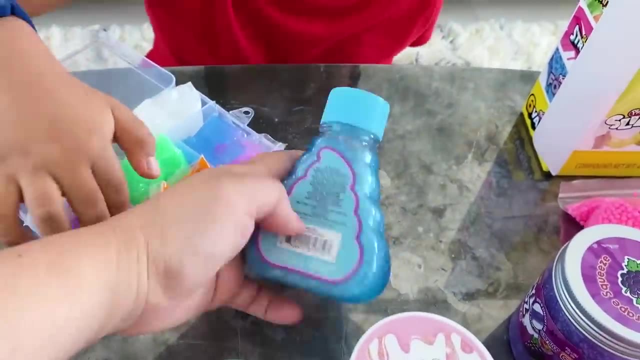 little things inside of it And these really look like galaxy. right, Yeah, These are really cool. Yeah, so these are just straight up different color slime. Oh, and these are really cool slime. They're supposed to be a mermaid slime, See. 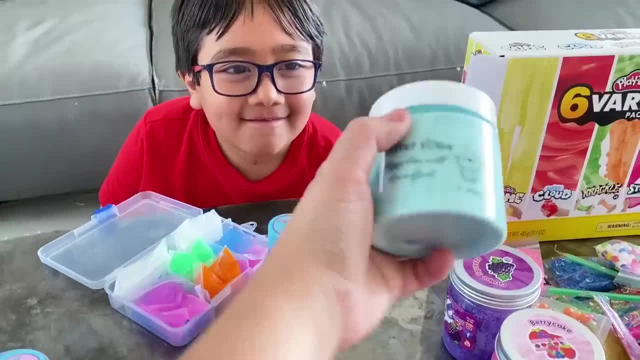 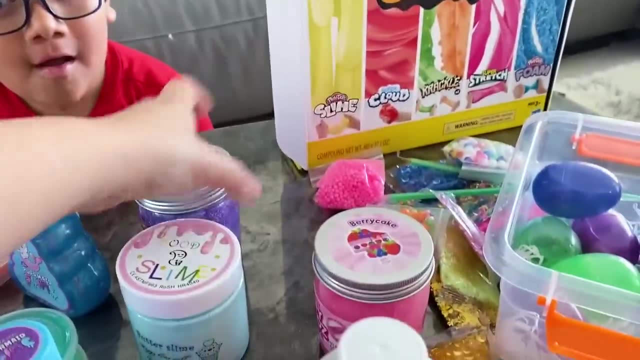 Yeah, and then we have some other ones that smells. So these are really cool. They're supposed to smell like butter, This one's supposed to smell like grape Mmm, And then my favorite berry, And we have some fun little foam. 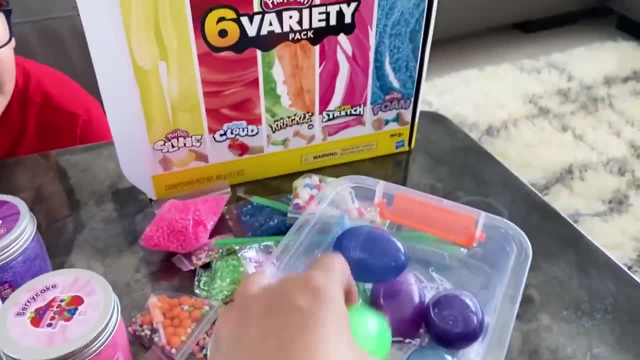 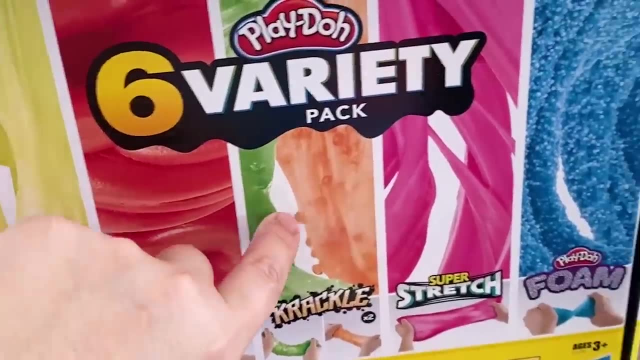 things we can add to the slime. Some egg slime is really cool, And did you know that Play-Doh also made slime here? Fluffy slime, some clouds, some slime with things inside, some foam slime and then just some other regular slime. 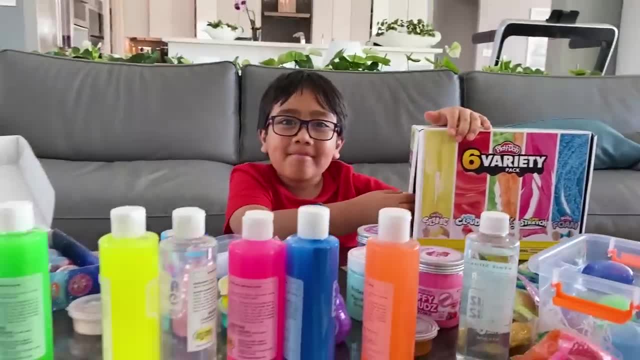 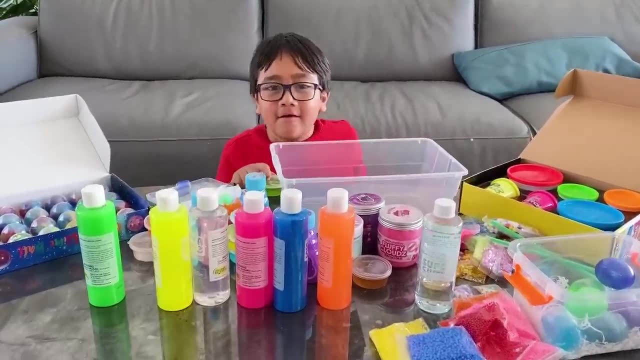 here, So hopefully it's gonna be really cool looking when we mix it together. What do you think? I think it's gonna look pretty cool. Okay, Ryan, what slime do you want to start out with? I wanna pick this one, Okay. 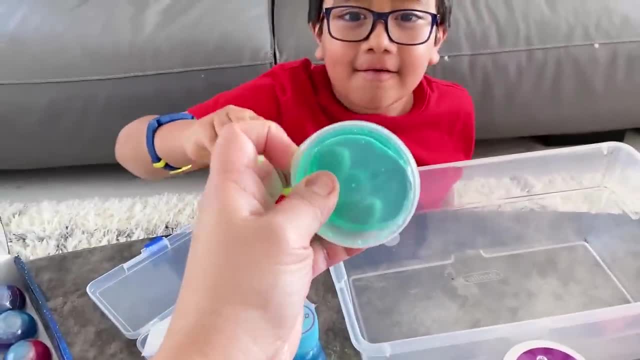 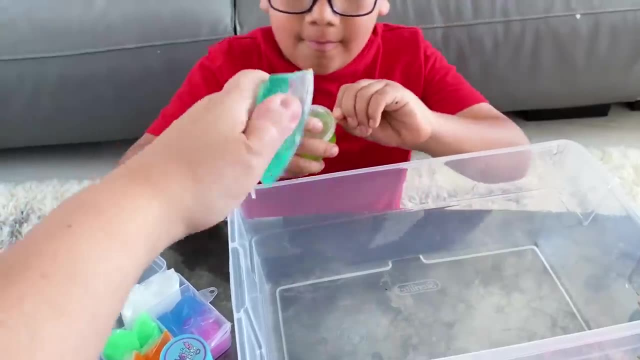 Alright, so that is green there. I want to help you open. I got some really cool blue ones. Ooh, looks good, Yeah, So we're gonna put it in. Alright, Come on. Come on, slime, Slimy, slimy, slime. 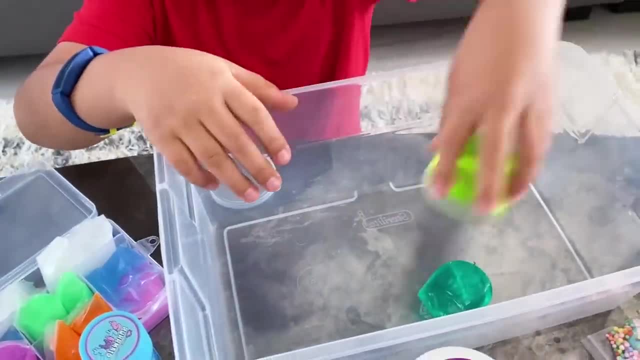 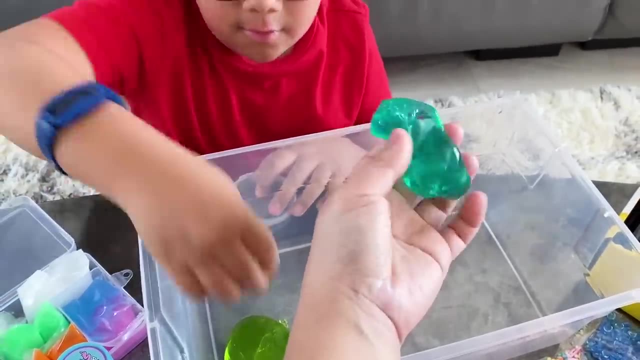 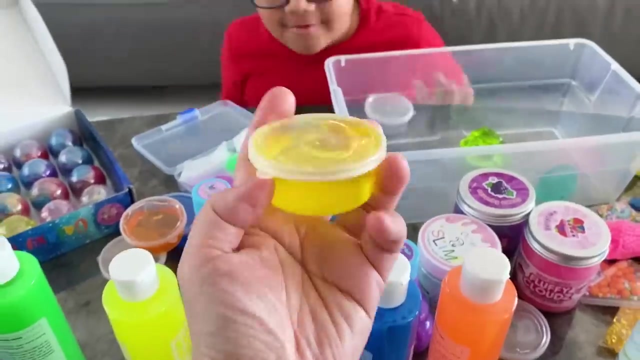 There you go, Just drop it in there. Slimy, slimy, slime, Slimy, slime. Whoa, it stays in the shape of the container. Yeah, But these are really cool. Okay, so here's a yellow color. Um, I'm gonna. 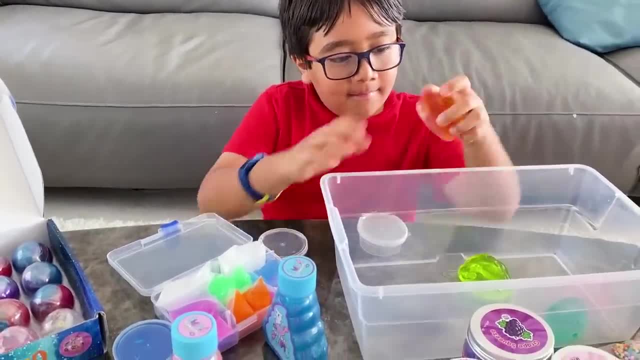 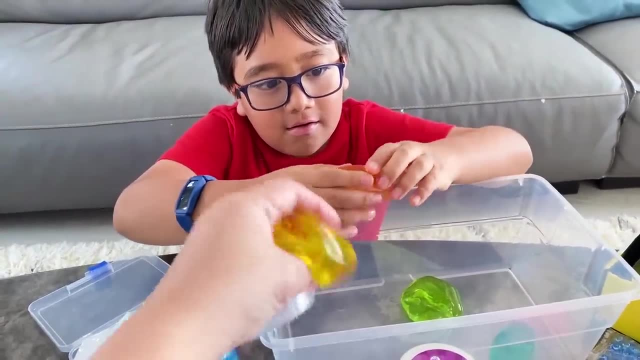 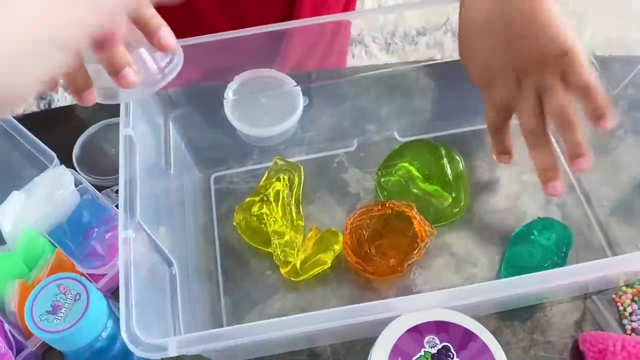 add this one, Orange, okay. Okay, here comes yellow. Ooh, they feel kind of cold, don't they? Yeah, They're pretty cold. Stick to the container. There we go. Ooh, so far mixing slime looks good, Epic slime. 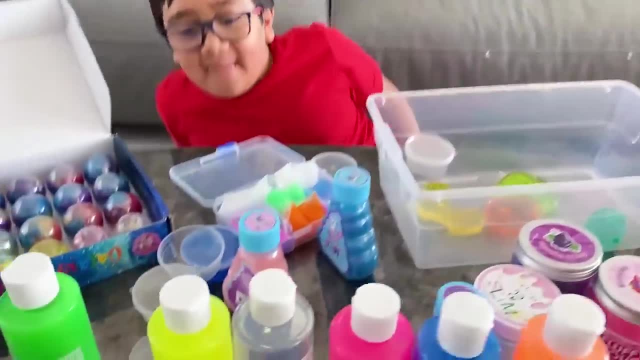 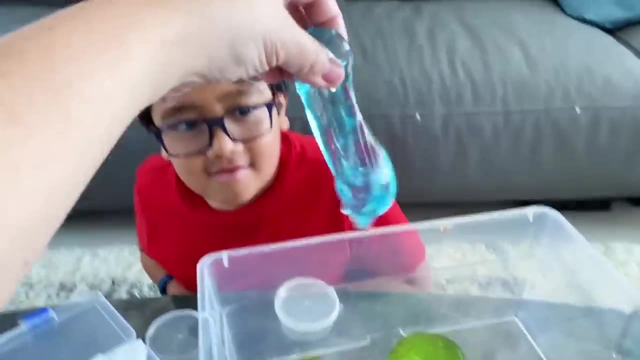 Okay, I have another blue one here. Okay, I think there's another dark blue right there. Our slime is probably gonna be blue. Come on, It looks like a snot, doesn't it? Uh yeah, I don't even know. 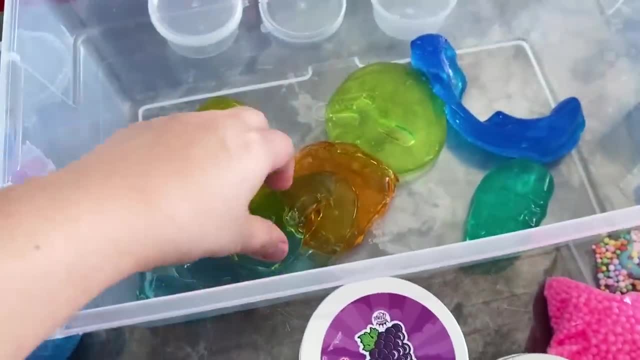 Boingy, boingy, boingy, boingy, boingy, boingy. Oh no, those two mixed together already. Give me this one. Ooh, I can't wait for you to smell it. 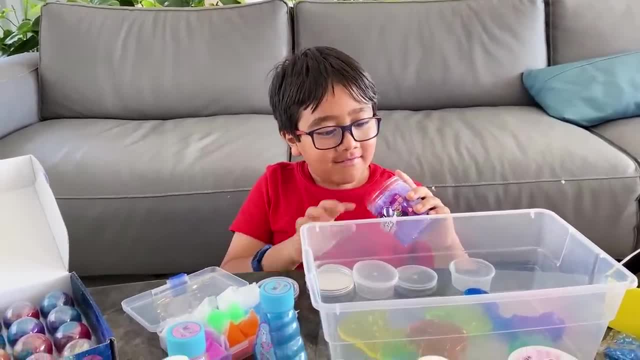 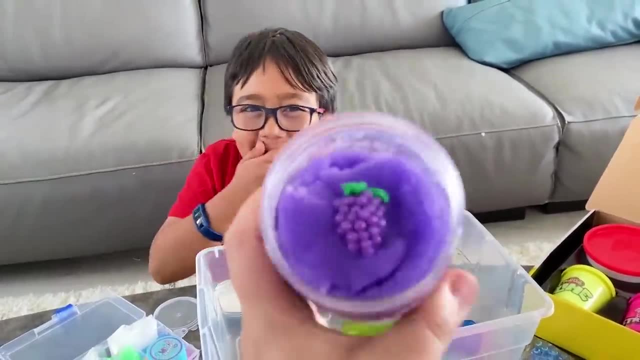 Smells pretty good. What does it smell like? Like grape, Grape. Yeah, There's like a picture of a grape here, just in case you didn't know. Smell it. Okay, guys, smell it. Ooh, But it feels different, right? Wait, is it like? 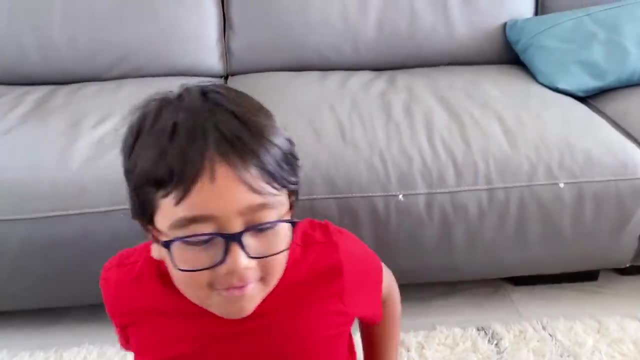 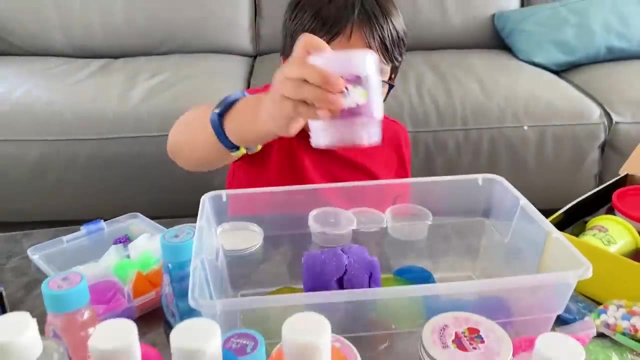 actually grapes? No, it just smells like grapes. Oh, okay, I think you're gonna have to use your hands. Oh, no, never mind. Whoa, look at this slime. These are so different. Yeah, Look at that. 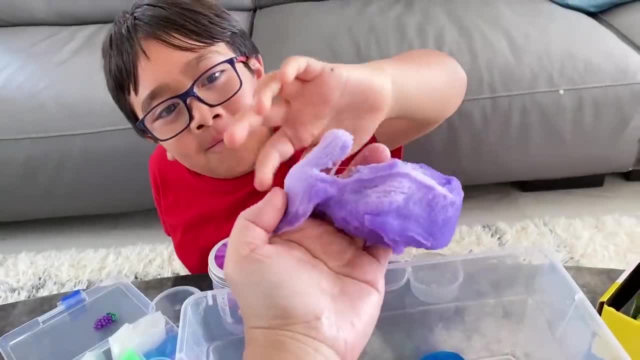 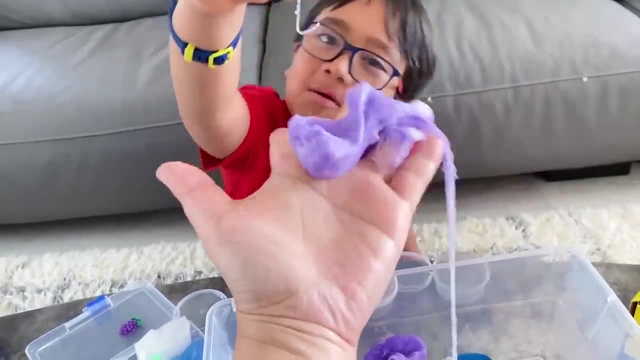 Whoa, Whoa, Whoa. what is that? Is that foam? Yeah, it feels like marshmallow, kind of. This is not regular slime. Uh-uh, Whoa. these are really cool. Do they use it for marshmallow or foam? Yeah. 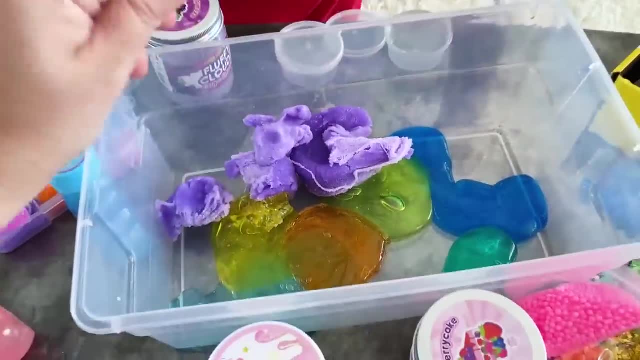 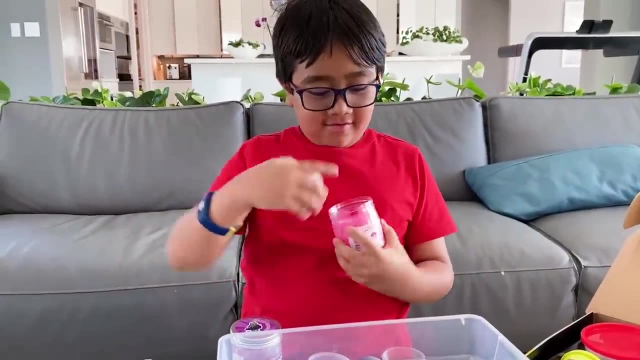 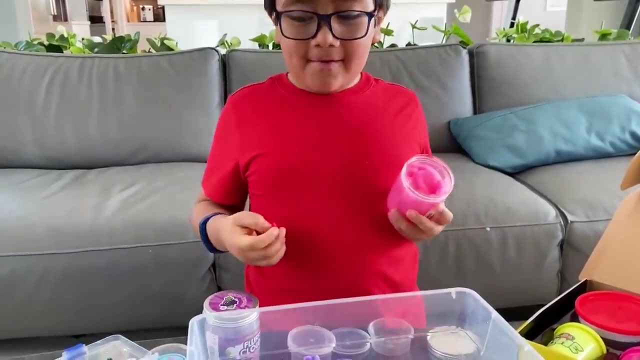 It's a different texture for sure, So that's really cool. Okay, what's next? This one? Ooh, it's supposed to be fluffy like a cloud. Mmm, Does it smell like grapes or strawberry or Strawberry? 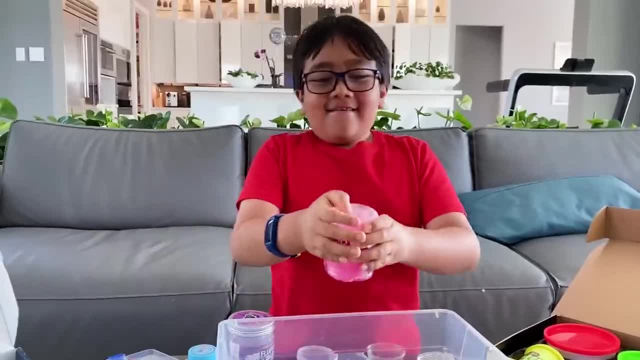 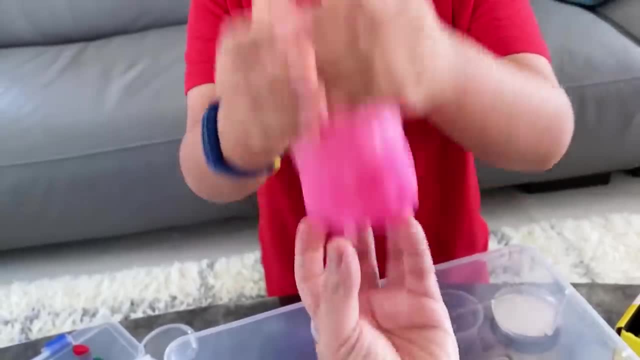 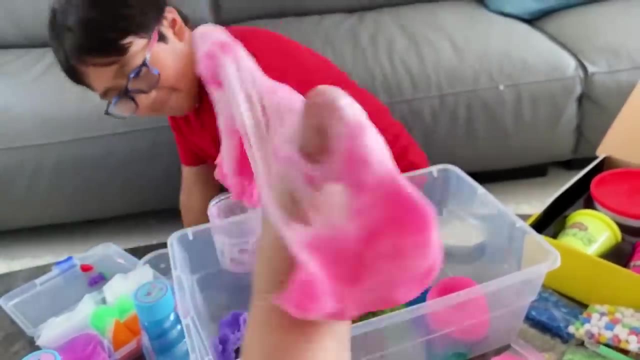 Strawberry Ryan, There we go, Just use your finger. Ah, there we go. Okay, go ahead, Pull slowly, Slowly and steady. Oh no, we broke it. Whoa, You guys like this? Whoa Feels like, looks like a. 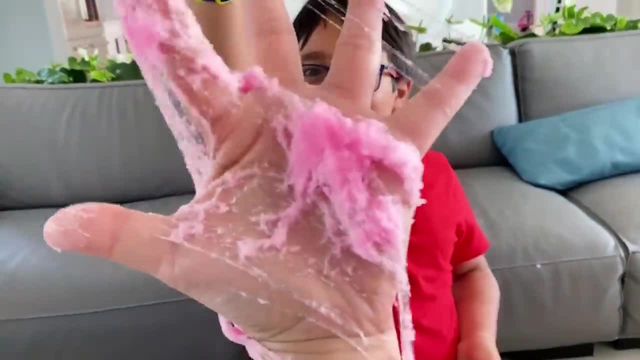 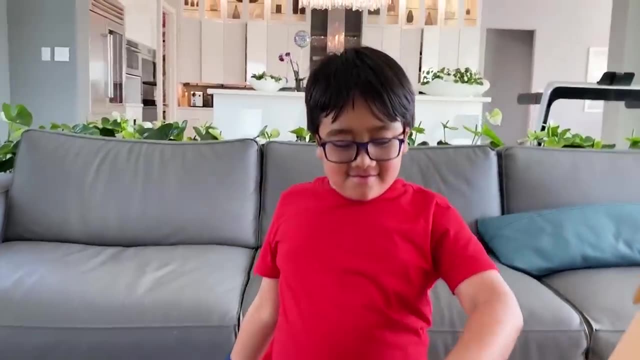 cotton web Like a spider cotton web. Ah, Okay, so far It's not edible, right? Oh, no right, Never, never eat slime, That's right. It may look good Or smell good And smell good. 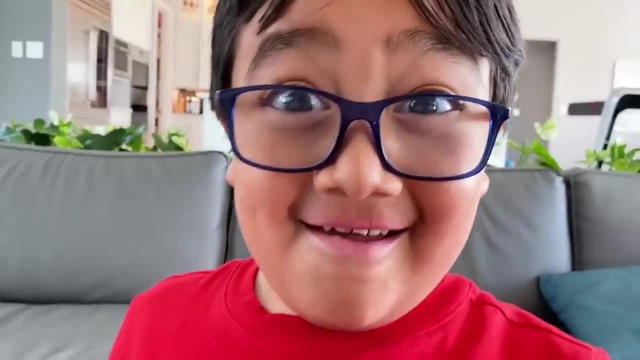 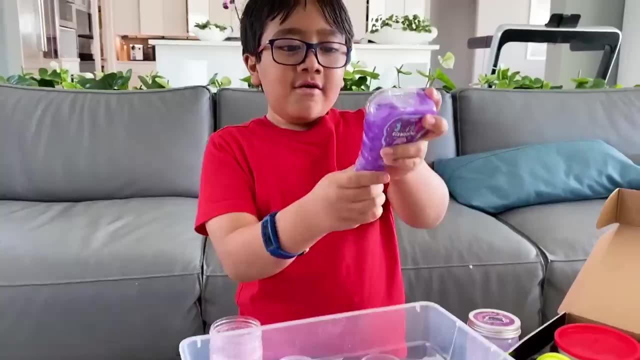 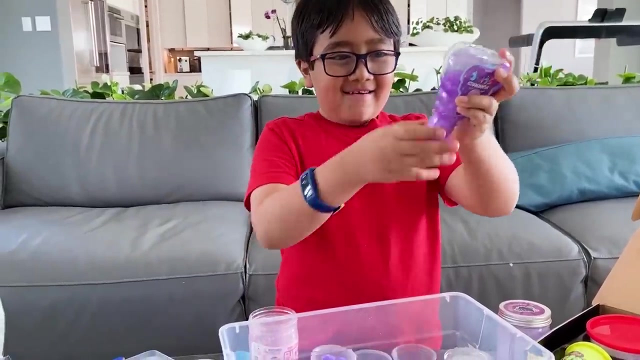 And you might think it tastes good. but do not eat slime. Let's mix this. Ooh, It might be purple or blue, So it's easy. Whoa, This kind of looks like a, like a snot, like a from your nose. 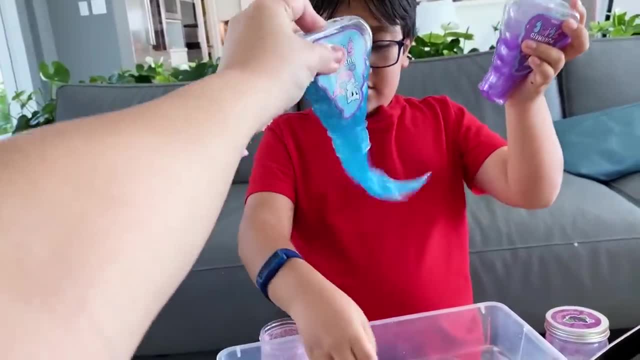 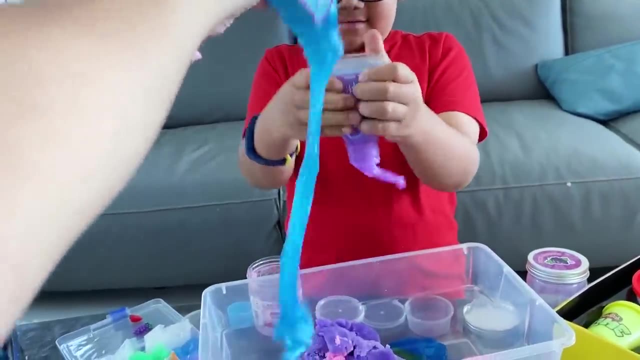 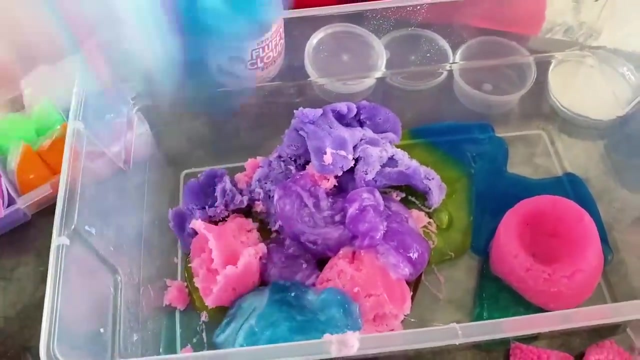 Ah, There we go. Look, Come on. Come on. Okay, so far, What do you guys think of our slime? I'm not sure if it looks good or not, But this is having a hard time. There we go. 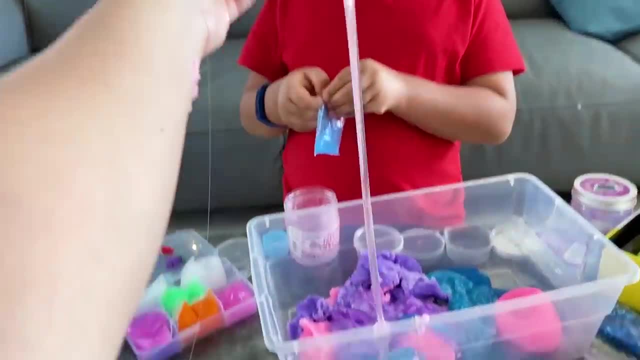 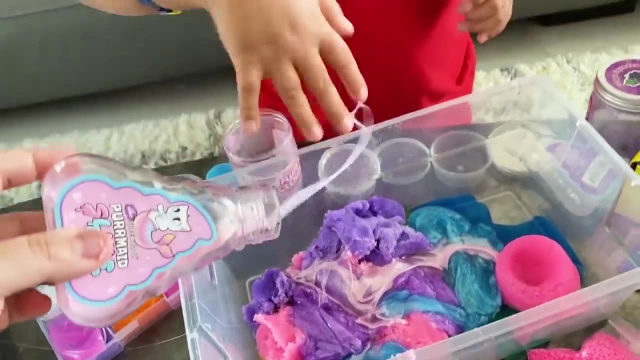 Whoa. So I'm gonna do the pink one which is coming out really fast. Oh, This is. What type of slime is it? I don't know. Oh, it's this one. Yeah, the same type. It's not slime. Oh, This slime is. 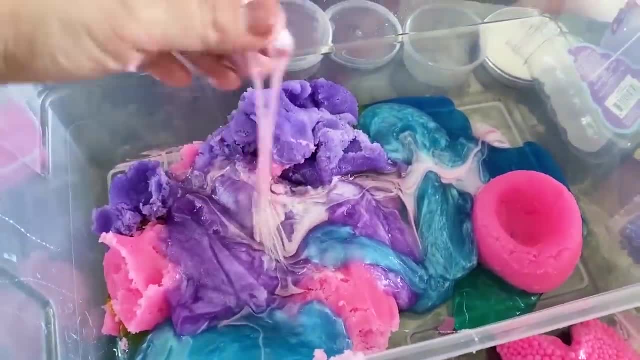 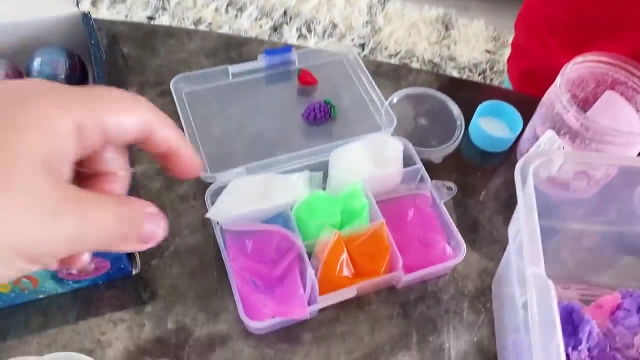 very sticky, But it's kind of like our slime. Well, that slime was sticky, huh Ooh. look at this, I'm gonna put this in. Okay, so This is like goo Goo, Yeah, Alright. so Ryan found a whole bunch of other slime. 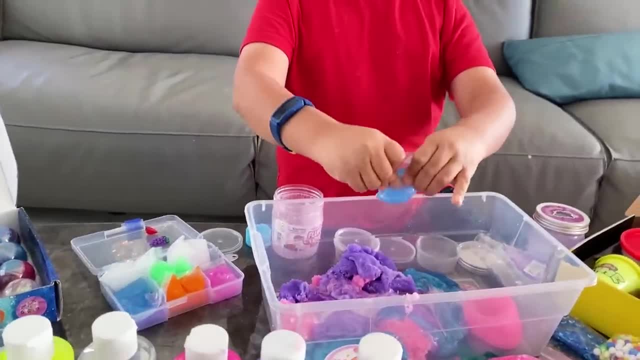 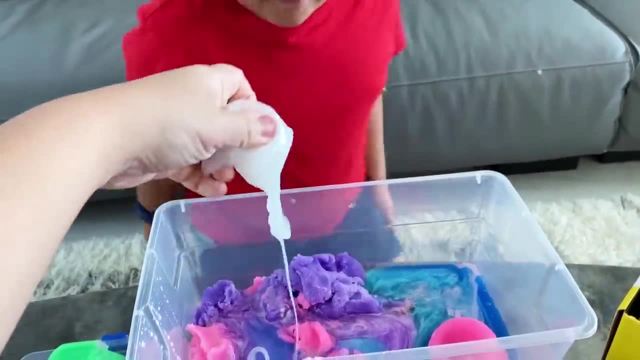 back here. We're gonna put these in. Might take a while. Uh-huh, There we go, Boom, Boom. Okay, so now I'm doing the white one. Oh no, I didn't cut very well, But it's coming down here. 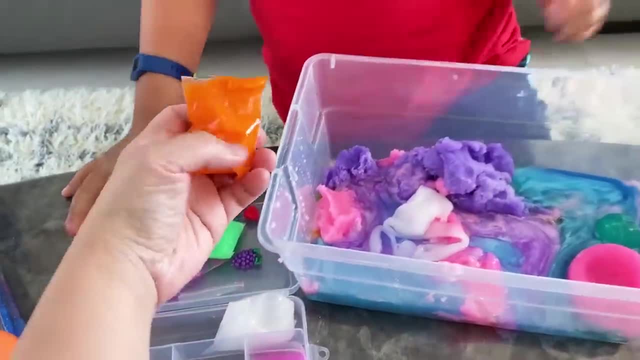 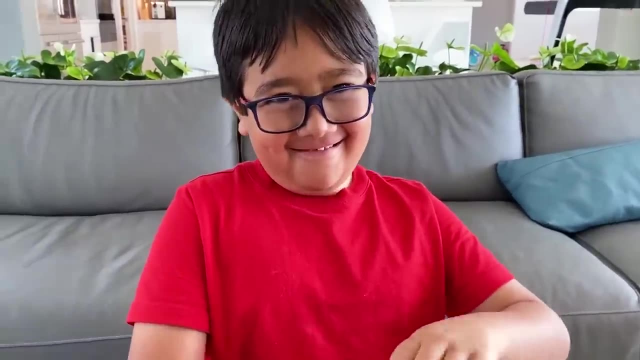 Okay, white. Okay, we have some more here. I'm gonna do orange. Okay, I'm gonna do this other one. So far it doesn't look so bad. Good Ryan, Yeah, it doesn't look that bad. Okay, here is a. 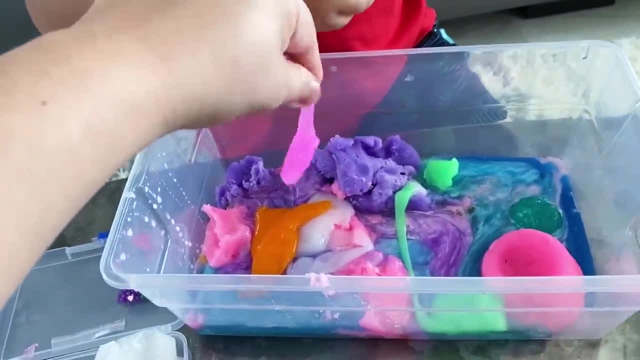 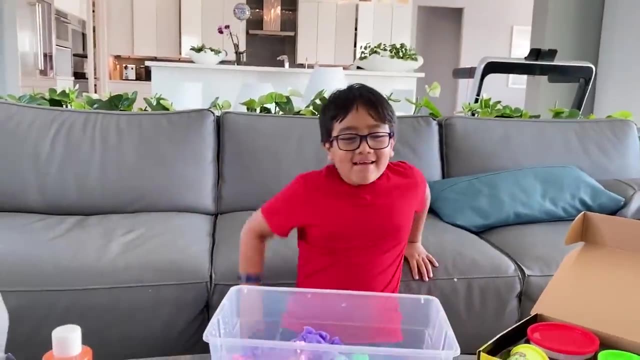 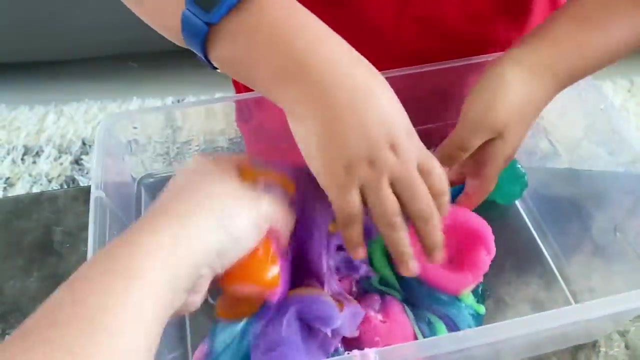 pink one. Come on, There we go. Okay, Maybe after this you want to mix, Oh yeah, Okay, Alright, Ryan, Here's the moment of truth: Mixing time. Alright, Okay, Mix with hand. Sure, Why not? 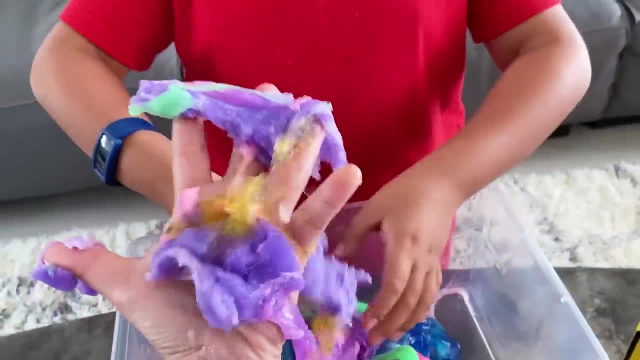 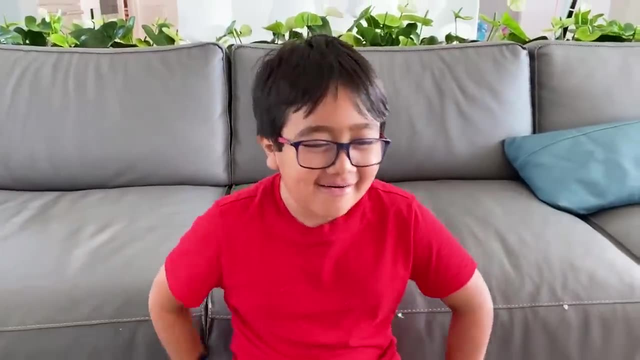 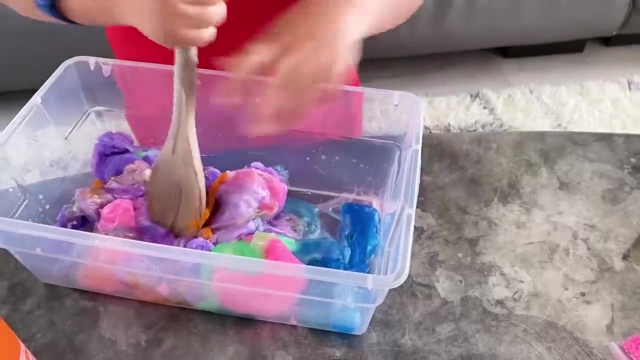 Here we go, Mixing, mixing. Oh, It kind of feels weird. It feels weird. Yeah, I'm doubting about mixing with hand. What about this? Yeah, There you go, Mix it up. No more mixing with hand. 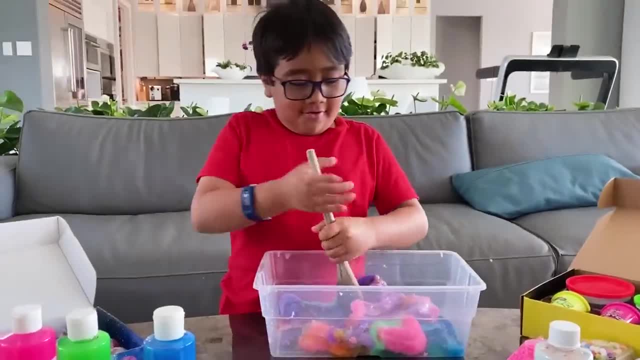 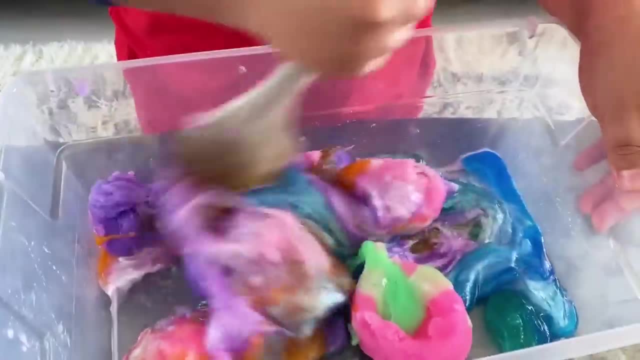 Whoa, There you go. You feel like a mad scientist. This is hard to mix, Yeah, I know. That's why I think hand is better. Oh, oh, oh, oh Oh. What do you guys think so far Is this: 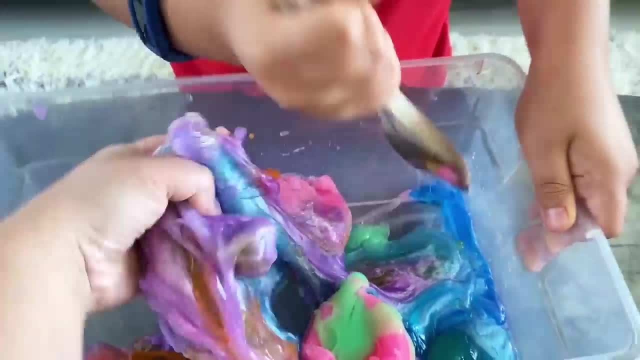 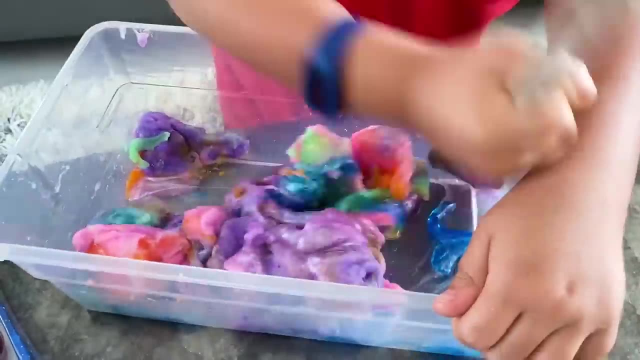 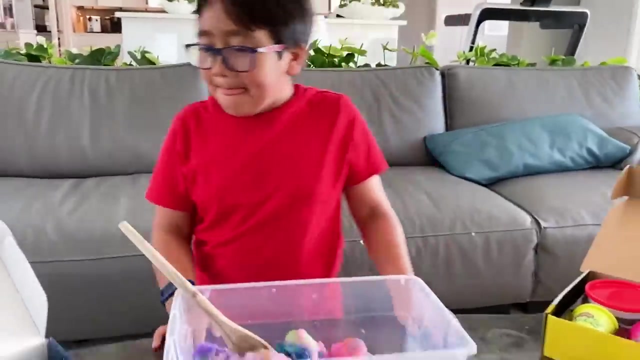 something that you guys would want to play with. It looks like purple. Yeah, It kind of still looks cool to me Like a galaxy color. Yeah, Whoa, Whoa, You done. Yeah, Okay, What slime you want to add next? 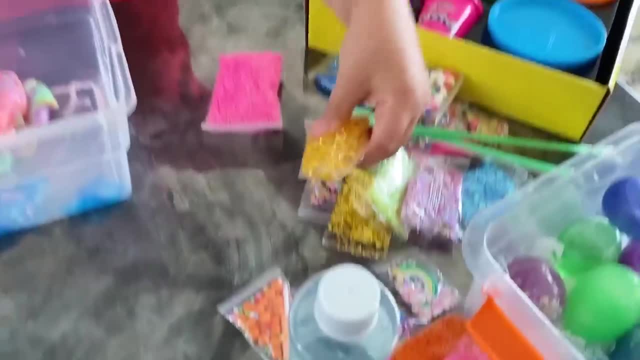 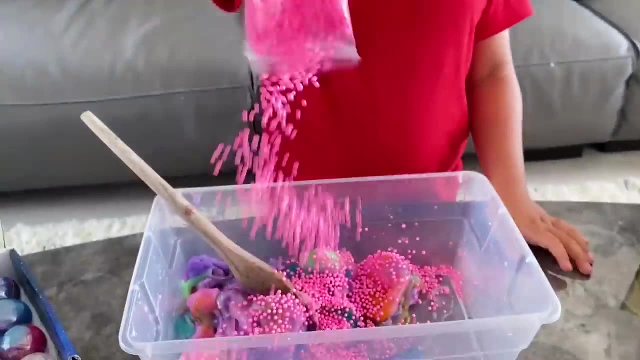 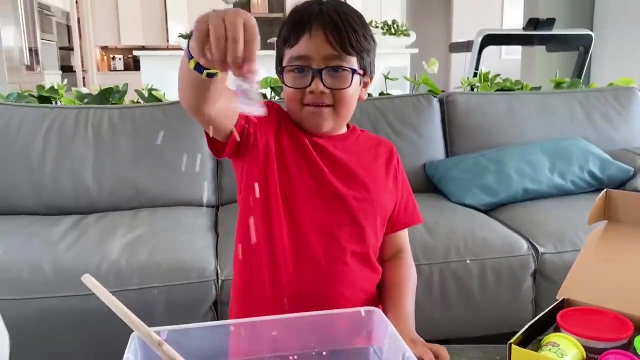 I want to add some of these actually, Oh really, Yeah, These little fun ones, Okay, So go ahead. Whoa, So these are fun. Makes a little crackling. Yeah, Wee More, A little giant. 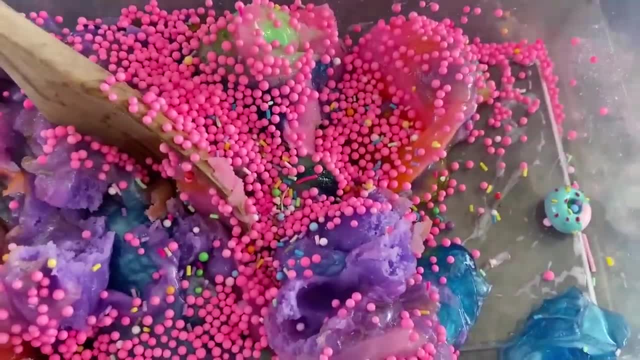 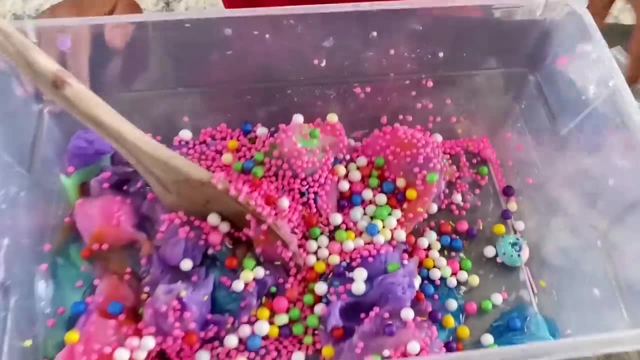 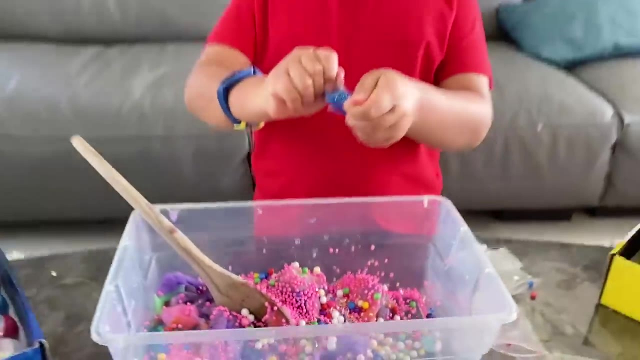 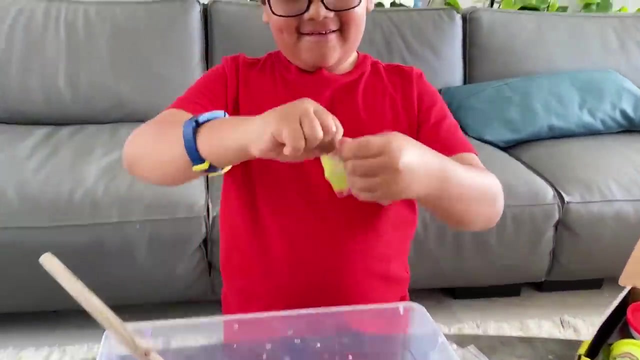 Yeah, Donuts. Oh, those are super giant size. It's raining. foam balls, Oh rainbow. Oh, Little beads. Okay, More beads. Ryan, you keep going crazy with so much beads. Beads are good. Look at those Like little. 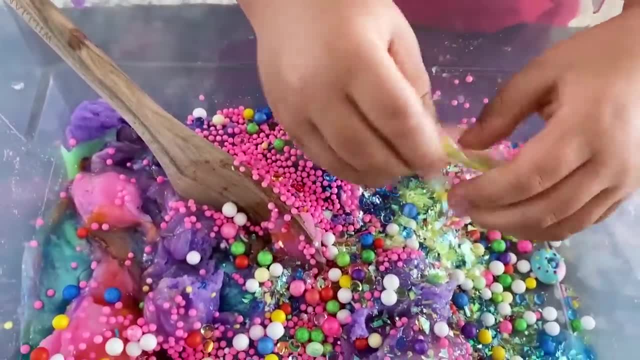 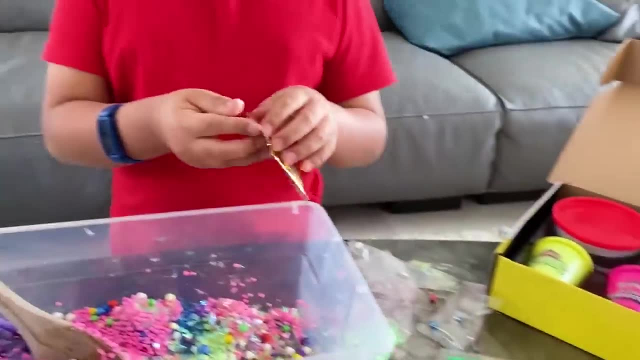 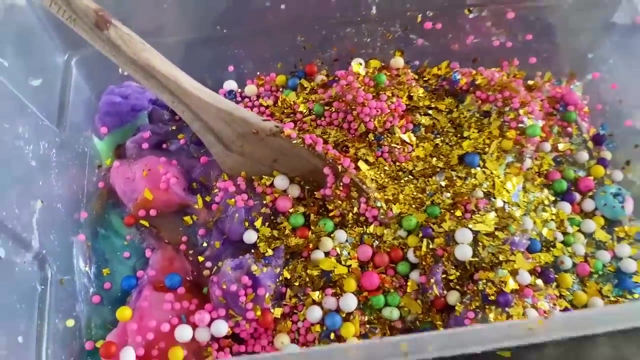 sprinkles Little ooh confetti. Yeah, there we go Confetti. Okay, Anything else Go go, go, Go party, Go party. Whoa, Ryan, I think we're going to need more slime. 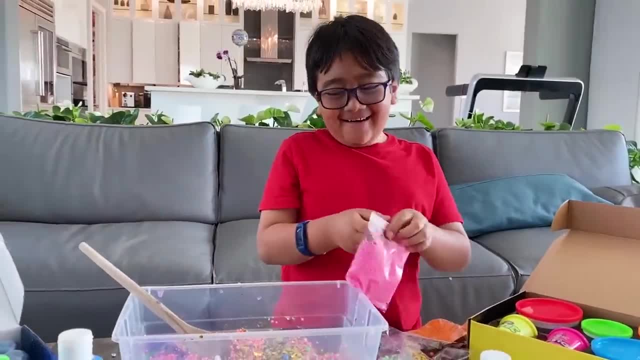 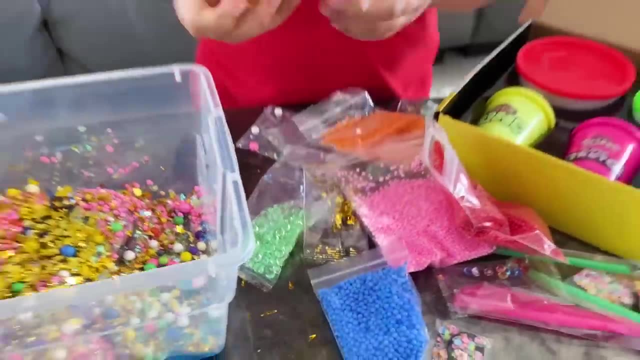 And we're going to need more of these, Do we? Yeah, I'm just going to open all of these. Oh guys, Ryan's going crazy with the foam. Is it even slime anymore? I don't know? Ooh, two at a time. 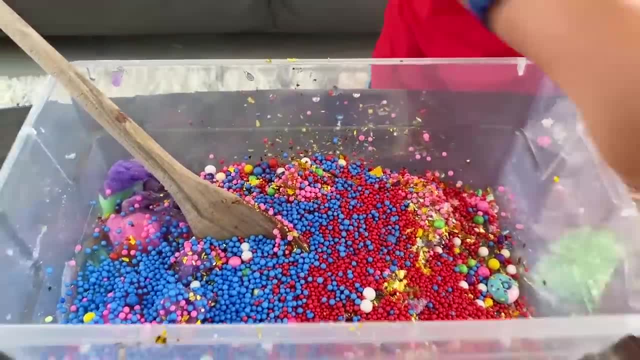 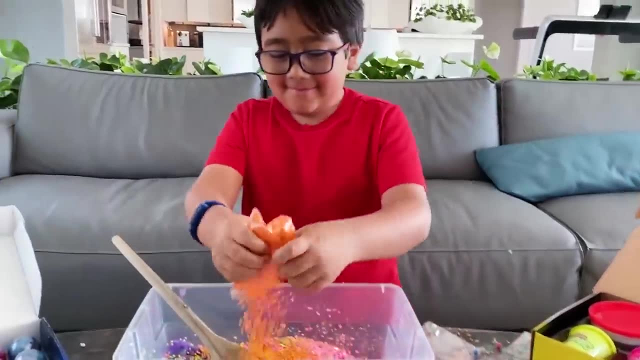 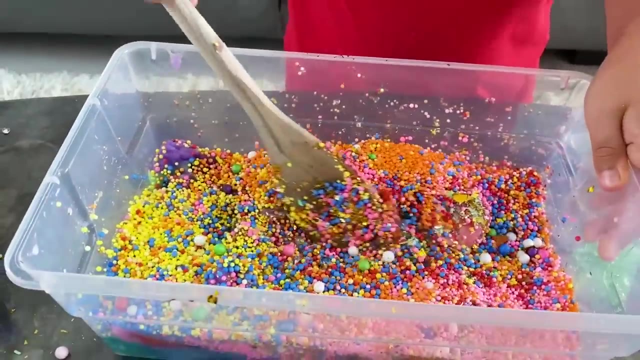 Ooh, Oh. all I see is the foam beads. I'm covering it. I can see that I'm covering all the slime. Whoa Nice, Let's mix it now. Okay, It's more like a bead party now. 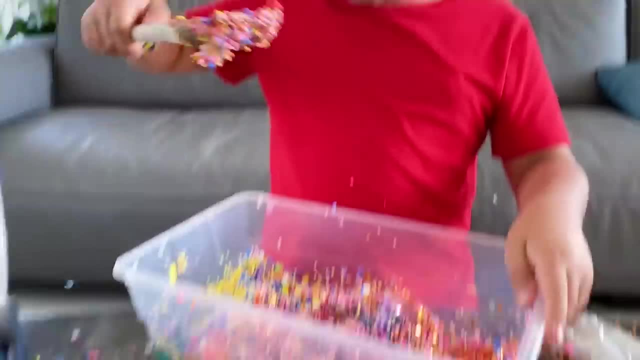 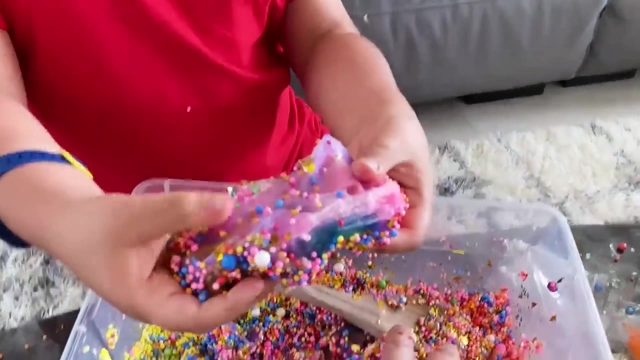 This is the slime with all the beads on it. Yeah, If I crack it open for you guys, this is what it looks like. It looks really cool. That's cool. Oh, it's the pink one and the purple one. Yeah. 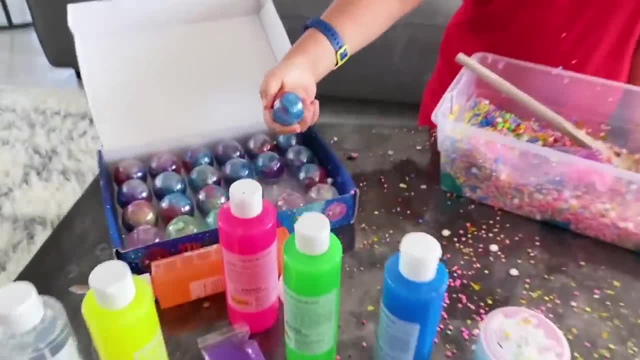 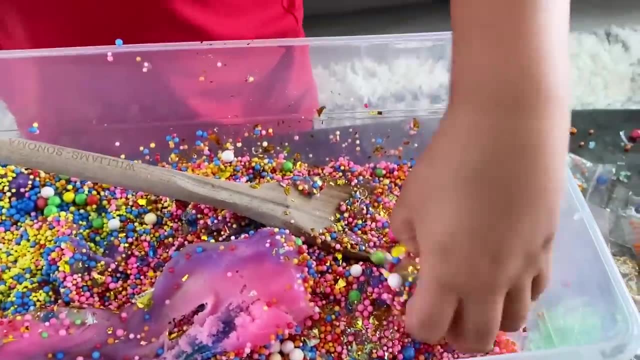 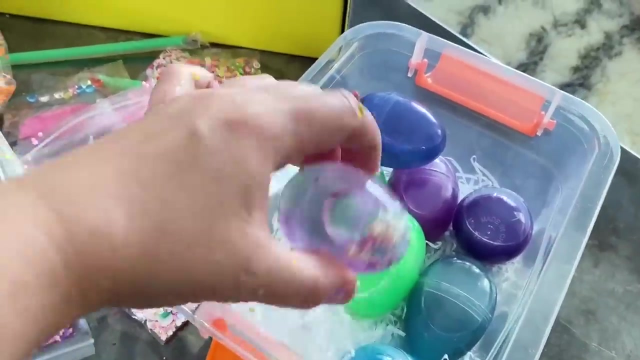 It looks super cool. I love it. Any more slime. you want to add These? Oh, these galaxy balls are really cool. Whoa, Oh, how did the ball? It already got covered, Like completely covered, Instead of Ryan dropped it. it's already covered. 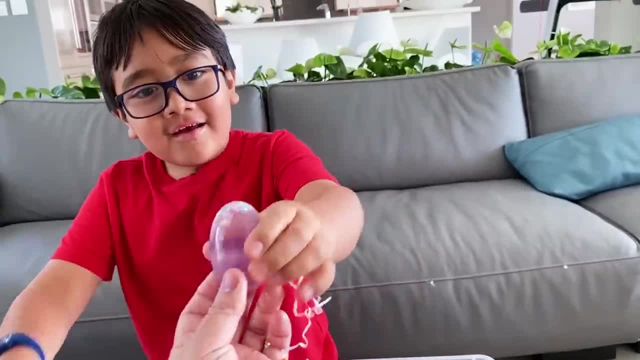 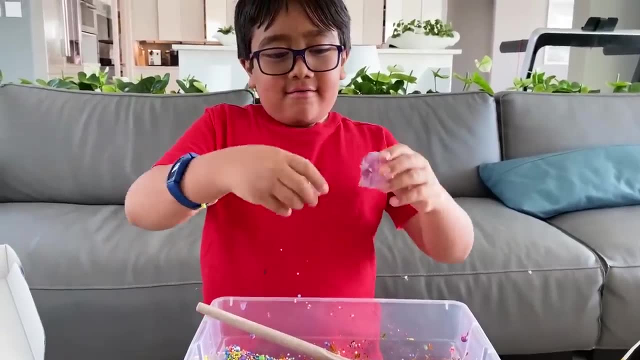 Look at this egg. You want to open this one. Look at it. That looks cool. Yeah, there's like stuff inside the eggs. Crack it. You got it, Got it. Oh oh oh. This is cool slime. 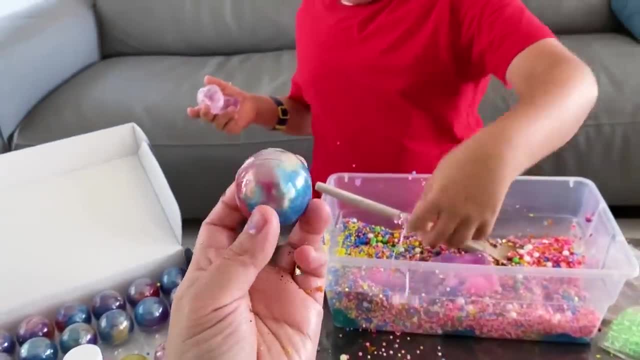 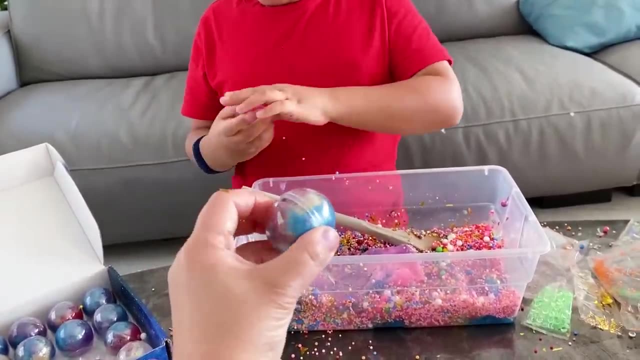 I actually want to open While you do that. I actually want to open one with more galaxy, because it looks like it stays in the shape of the ball. Yeah, Okay, let's crack it, you guys. Yeah, Okay, here we go. 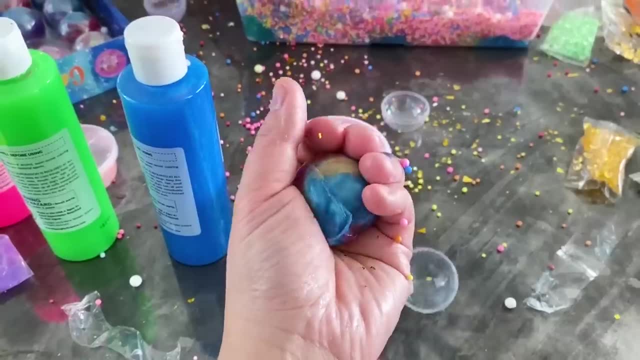 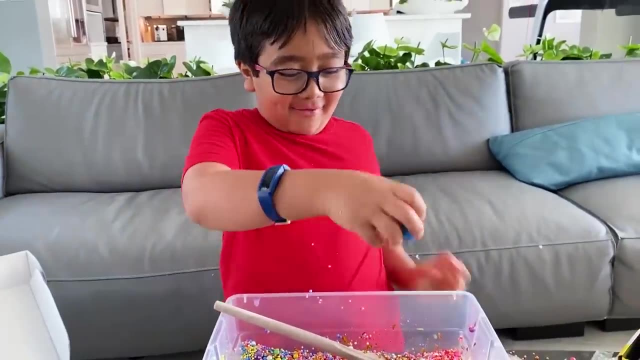 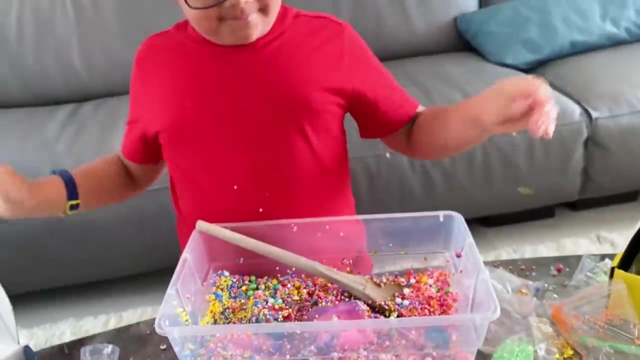 Oh Whoa, It did stay in a shape. Look, Ryan. Oh, that's cool. Yeah, Well, I'm going to drop it now. It's probably going to get covered. the instant I drop it, Probably It's already covered. 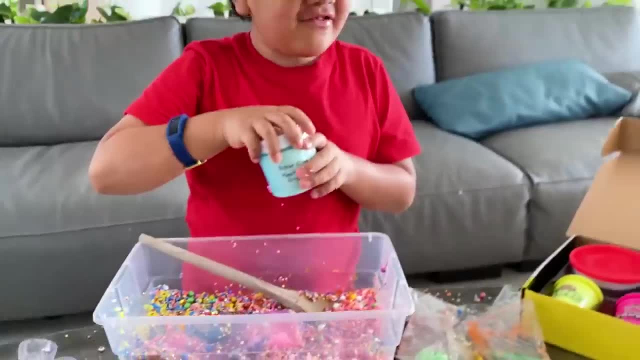 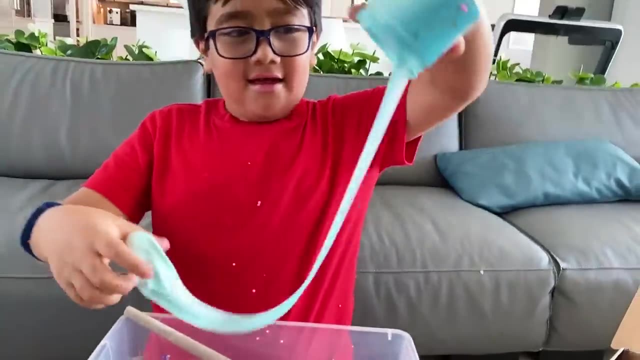 Okay, Oh, we haven't opened this one. It's supposed to be butter slime, so This is just opening everything. I know It is mixing up all my slime challenge. Oh, it does look like butter, Whoa, Whoa. 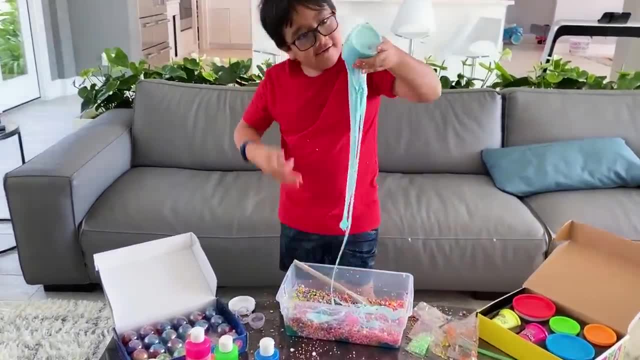 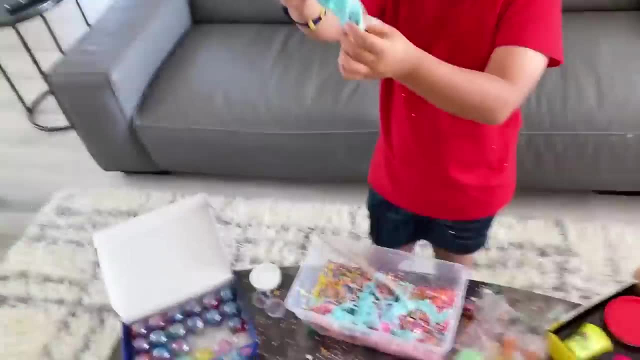 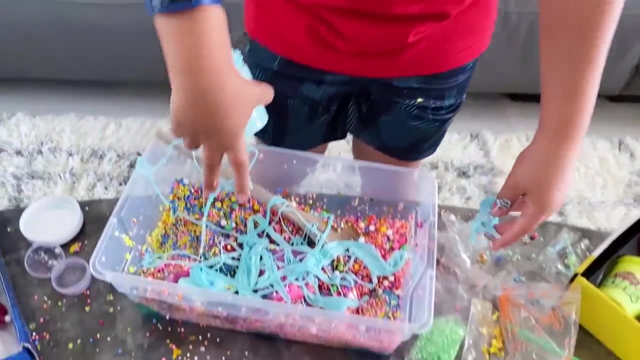 Look how long it is, guys. There you go, It's coming out, guys. Whew, You got it. There's something in here, Oh, Oh, it's like confetti. It's like a surprise confetti. Yeah, I saw another confetti thing. I think the confetti thing is in there. 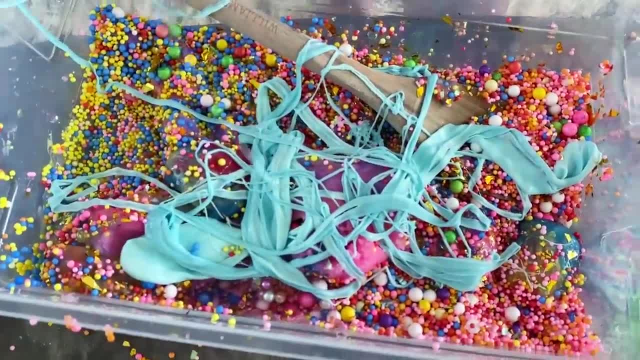 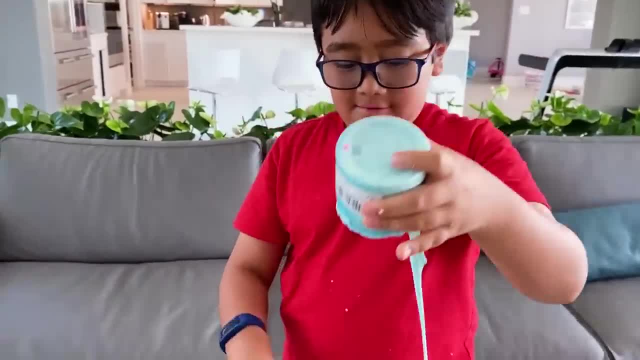 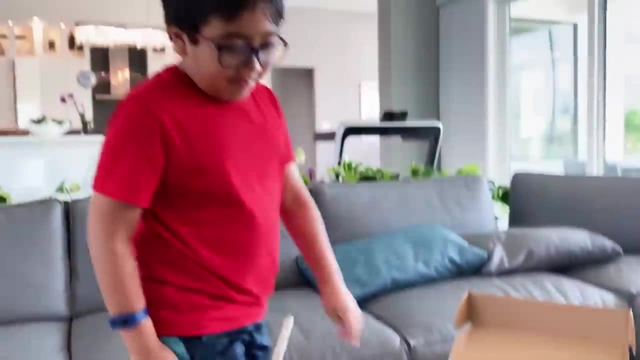 Oh, Oh, whoa, Feels like a paste. Okay, You got it. Mm-hmm, Oh, We have a few left. We can do different colors or we can try the Play-Doh slime. Let's try the Play-Doh. 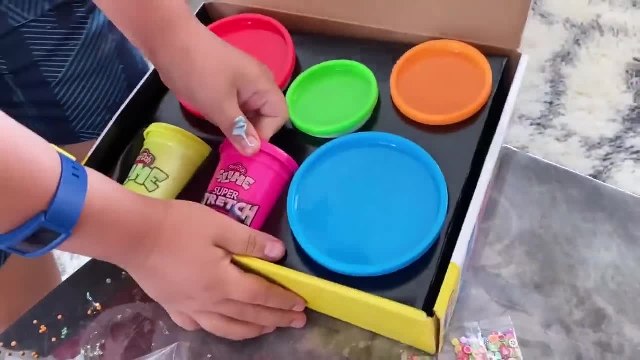 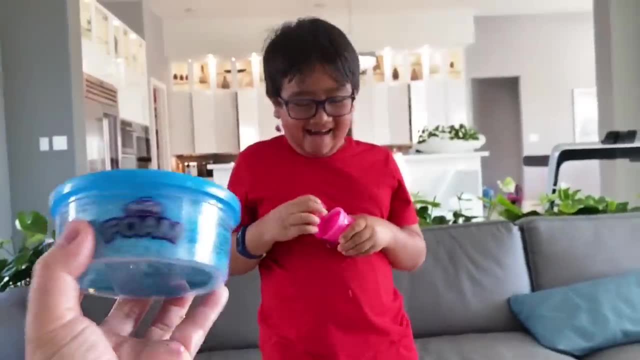 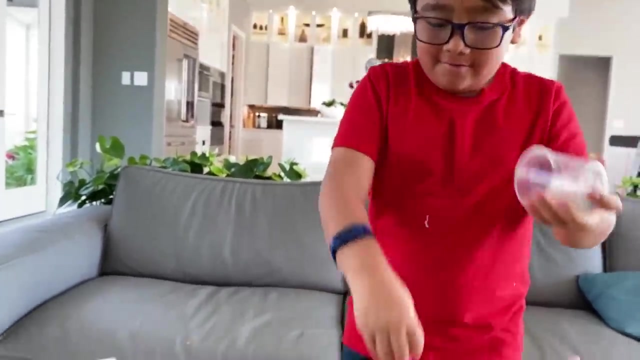 Yeah, this looks cool. I'm going to do the super stretch. Okay, Well, I'm going to do this foam one. Oh, Not like we don't have enough foam already. Yeah, Oh Yes, One of these slimes that stick together always. 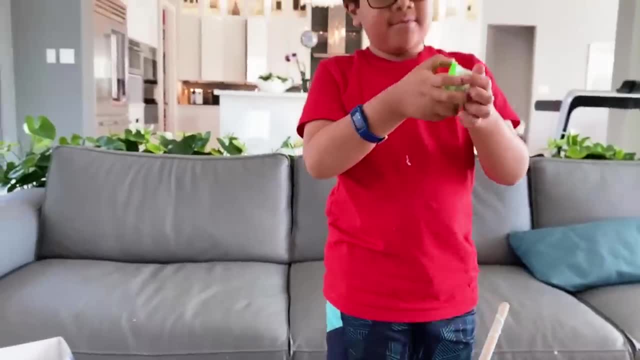 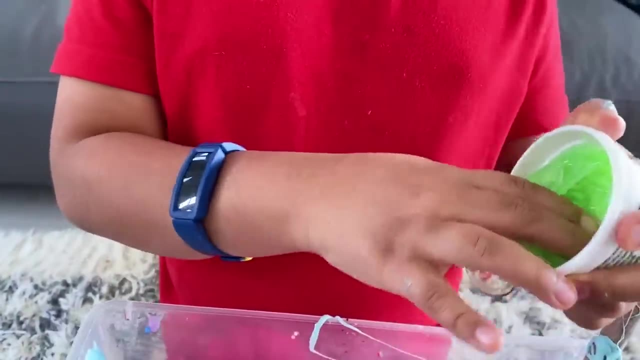 Oh, Oh, whoa. Look at the shape. Look at that. I'm doing the crackle one. Okay, Oh, I see why it's called crackle. It has stuff inside. Yeah, Does it make crackling noise? 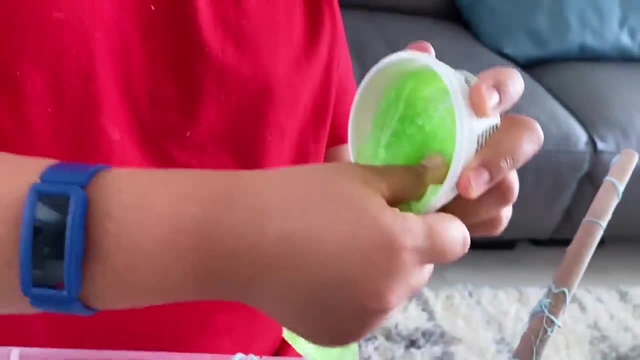 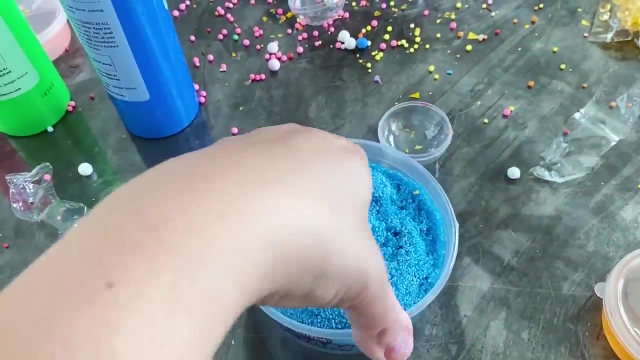 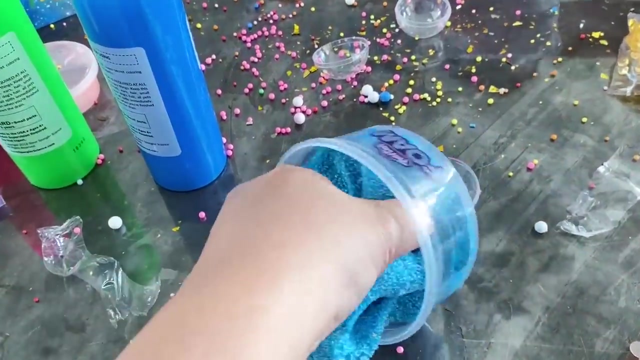 Oh yeah, It kind of does. Can you guys hear it? Yeah Whoa, Super foamy. This is definitely foam. Oh Right, It's so cool, Super Play-Doh foam. I think I need your help. 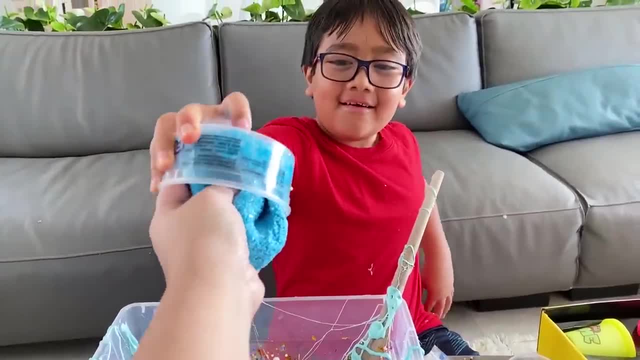 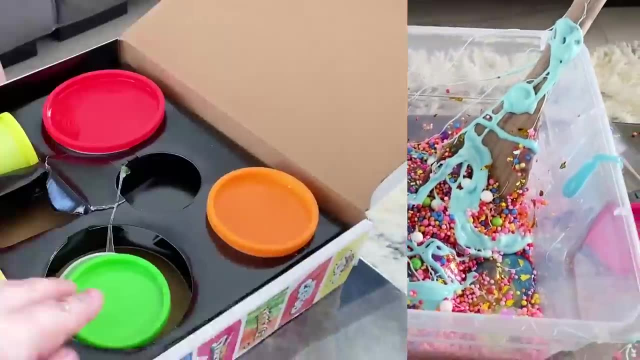 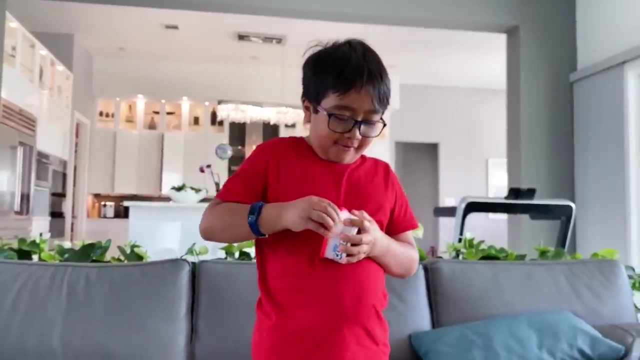 okay, Here you go, Hold the container Ready. Okay, There we go. Superman, Okay, Into our slime container, I'll do the giant one. Oh, cloud, Super cloud. So it's supposed to be really soft like a cloud. 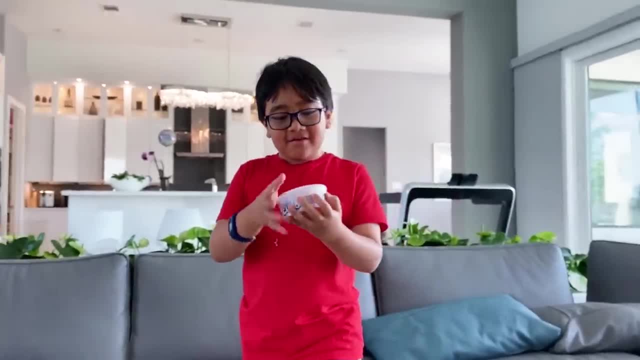 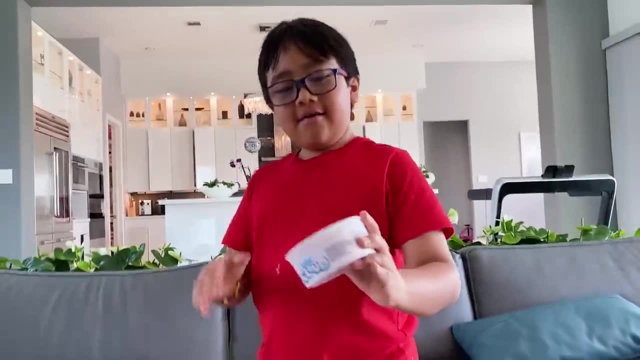 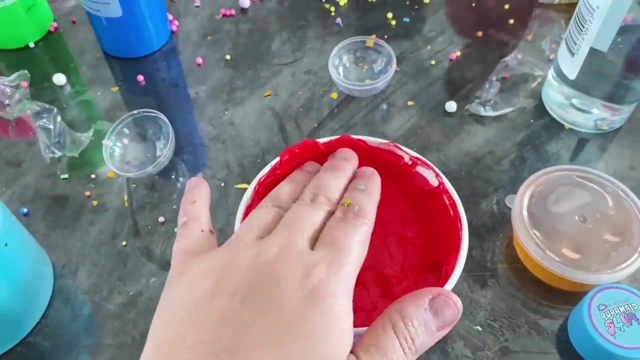 Does it feel soft? It feels kind of soft, Actually. It kind of looks like pink. Oh, it does Look Interesting. Oh, I'm afraid to touch it. It kind of sticks on you. It sticks on you, It does look like paint. 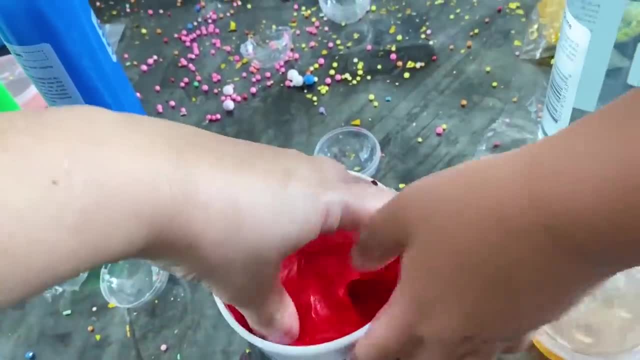 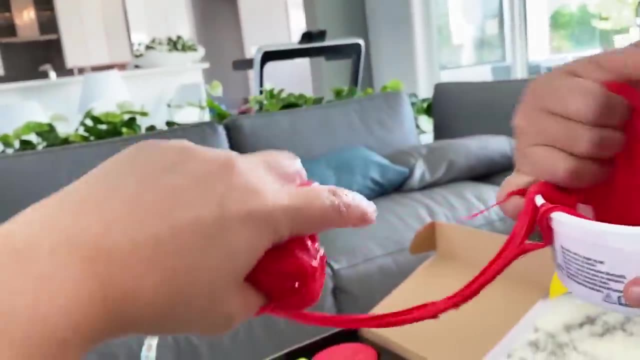 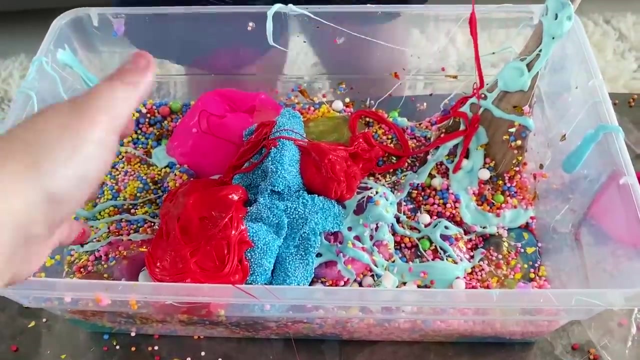 Oh, wow, Okay, I might not be able to get the whole thing out, but Ryan's going to help me, Okay, Whoa, Super super longy, There we go, Whoa. So this is our blob so far. 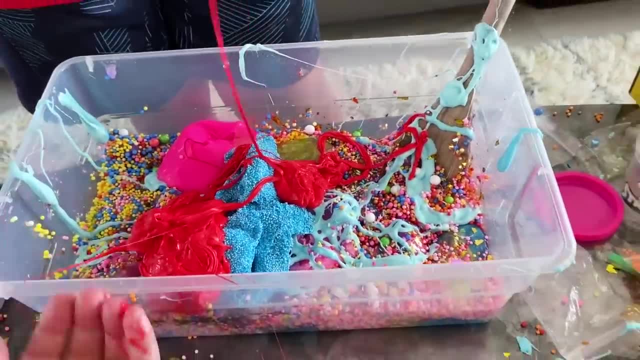 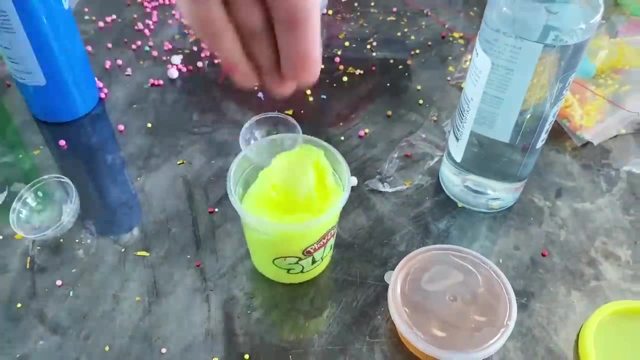 It really, really doesn't look good anymore. This is like a giant mess guys. So I got the yellow out. I'm not sure what this is supposed to be, but it looks like a little sound. Well, I feel that. 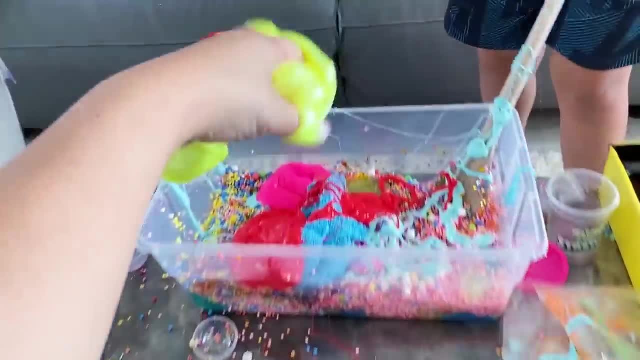 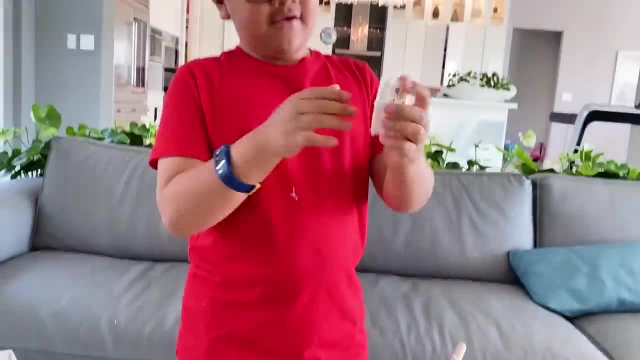 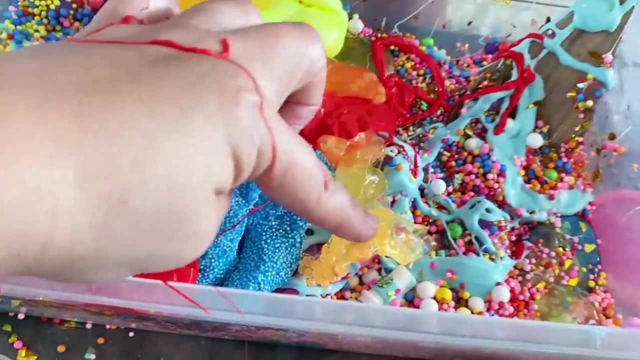 Oh, it's like that. one huh, Yeah, Okay, Into our slime container. Oh yeah, You guys hear the sound. I can hear the sound whenever you're touching it. Yeah, Okay. So there's the crackle one. 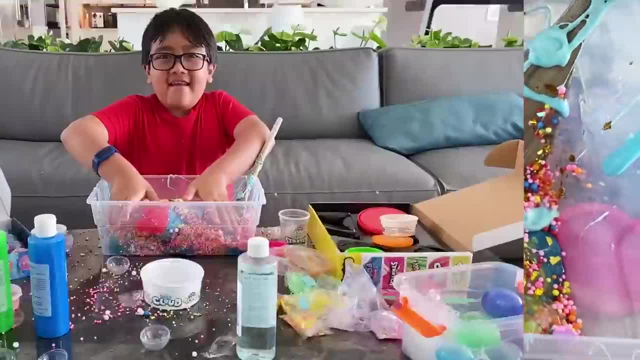 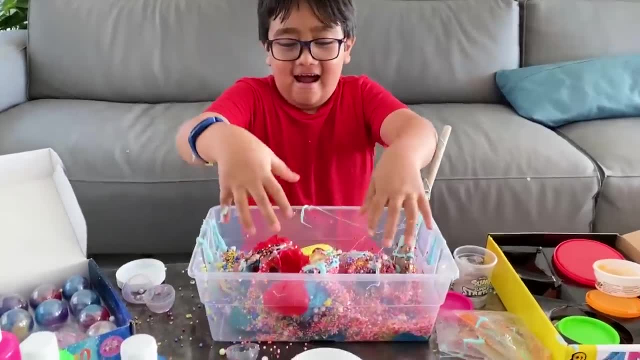 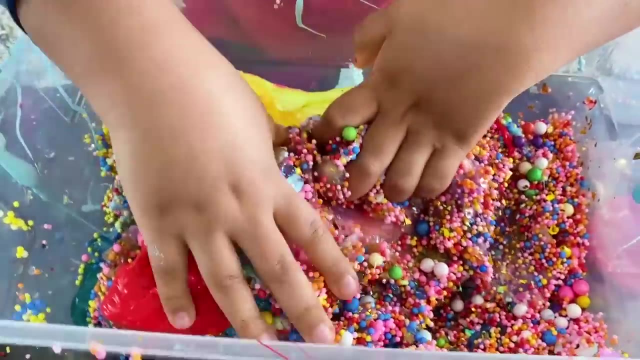 You can see the little beads inside. That looks really cool. Now mixing time. Whoa, Whoa. Can you even mix it? I don't really know. Okay, I don't think we need this anymore. We're taking this out. 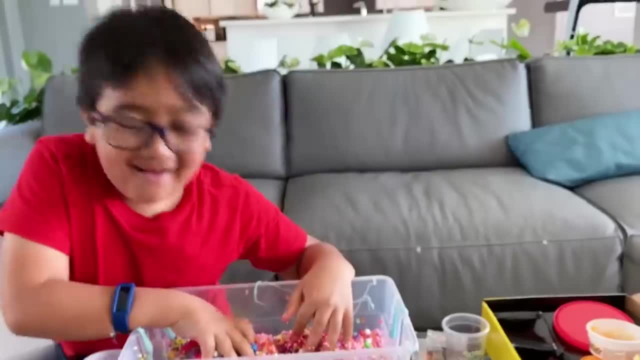 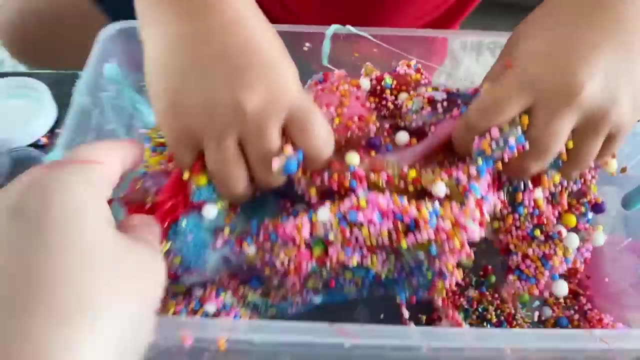 Ryan's trying to mix our slime. What do you guys think? Somebody went a little overboard with beads- Oh that one. So what do you guys think? This is our final result. We have more slime, but I think we have plenty. 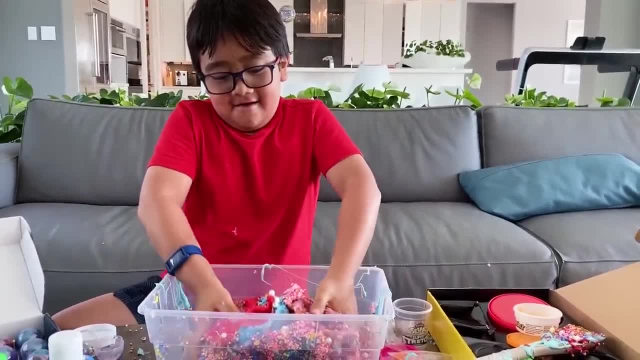 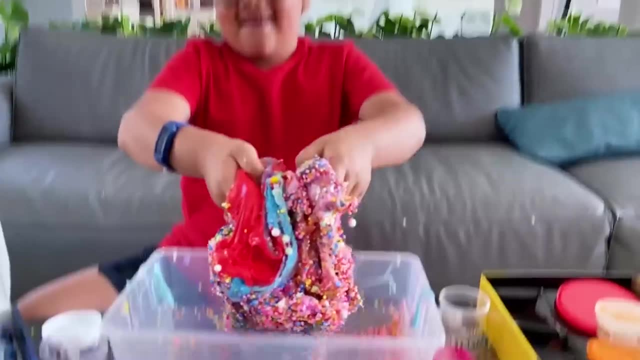 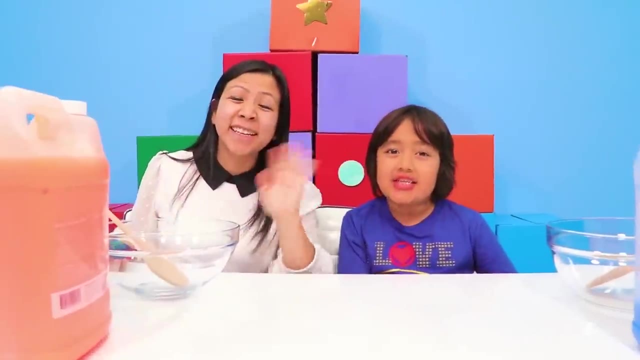 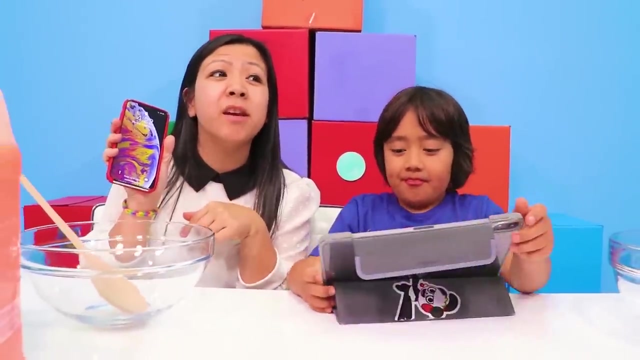 Wow, That was massive Layers and layers and layers of slime. I'm gonna karate, chop it. Okay, Hi guys, Today we're playing Siri Pick My Slime Challenge, That's right. So Siri's gonna pick our ingredients here. 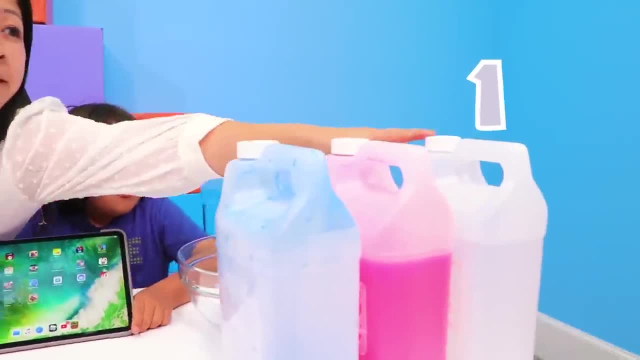 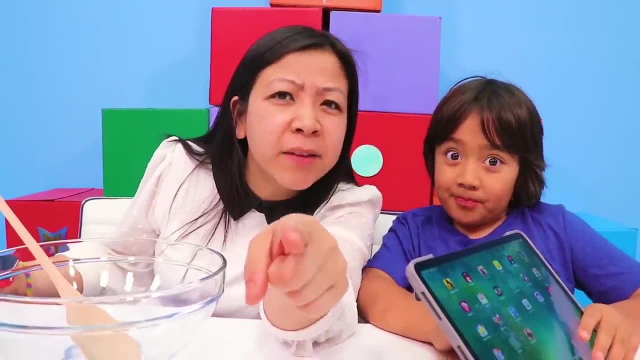 First. we're gonna start with the slime color. So we have one, two, three, four, five and six And at the end you guys decide if Siri did a good job at picking our slime. Okay, I will let Ryan go first. 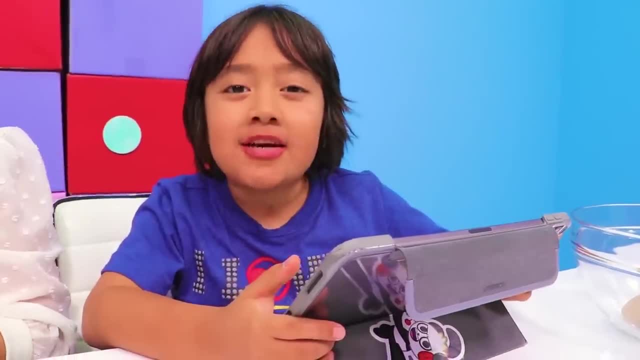 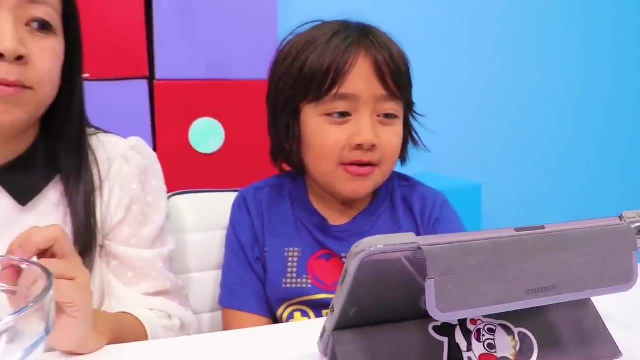 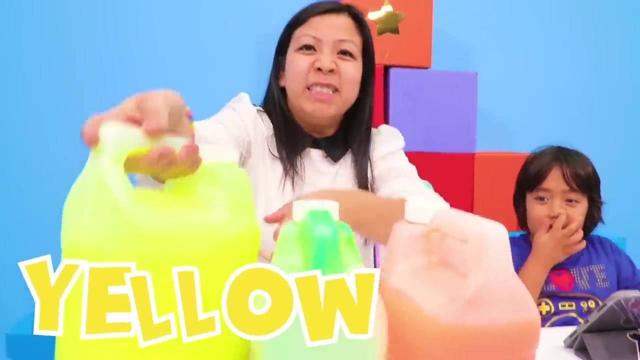 Nobody wants to get a one, I'm gonna ask Siri to pick my slime color. Siri pick a random number One. through six, It's six, Okay. So Siri picks number six, which is Yellow. Yellow- Ryan gets. 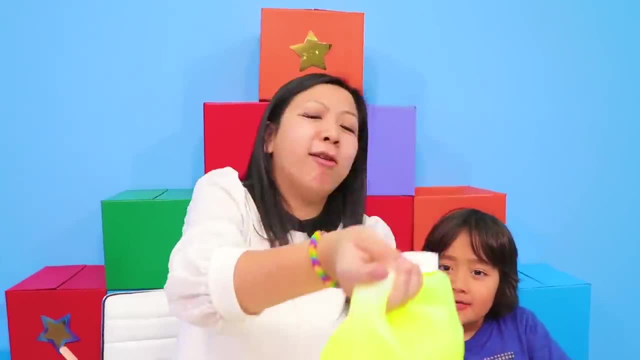 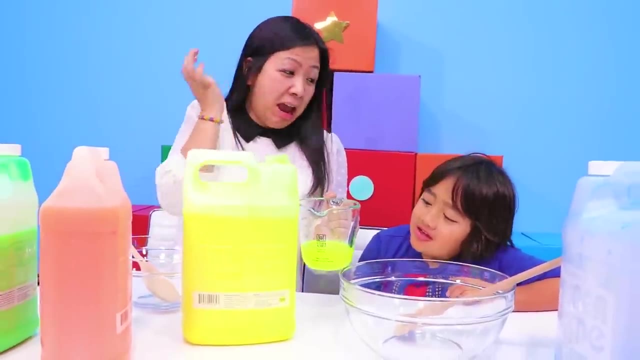 yellow slime. I was hoping for four. Ryan wanted orange. Sorry, Ryan, It looks like a. It splashed on my face. It looks like a yellow highlighter color, doesn't it? Yeah, Ryan, you can put it in. 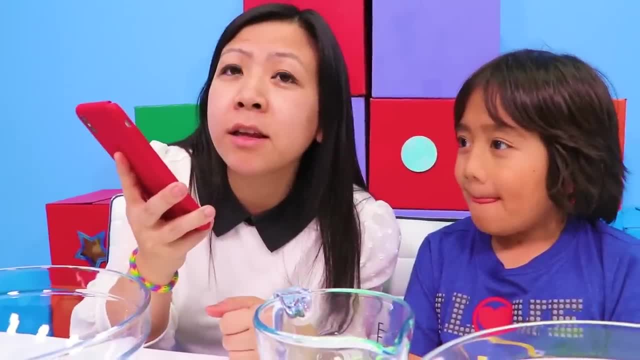 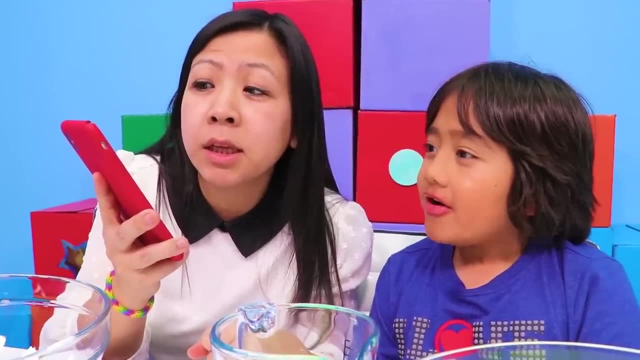 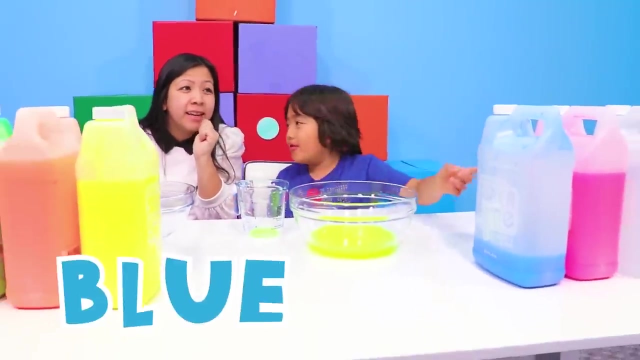 It is my turn. Hey, Siri, Pick a random number from one to six. A random number between one and six is three, Three. Which color is that, Ryan, do I get? You get blue, Blue slime. So far, Siri, you're doing a good job. 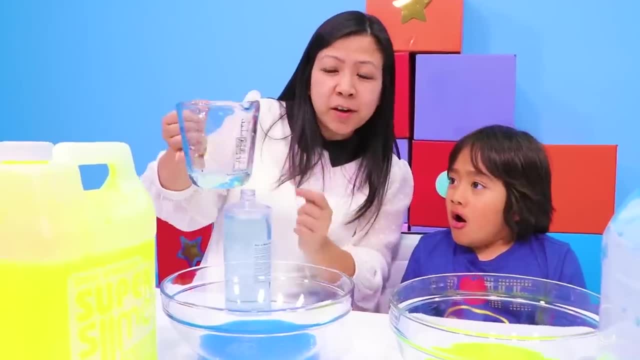 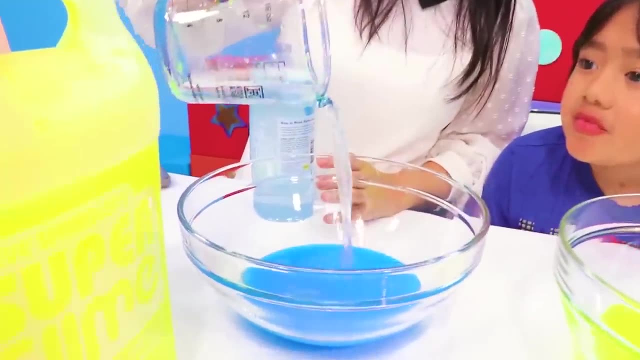 I like this color, Thank you. In order to make the slime, we need the activator, So I'm gonna put it in for Ryan. Activator for Mommy. Now it's officially slime, Let's agitate, Agitate, Agitate. 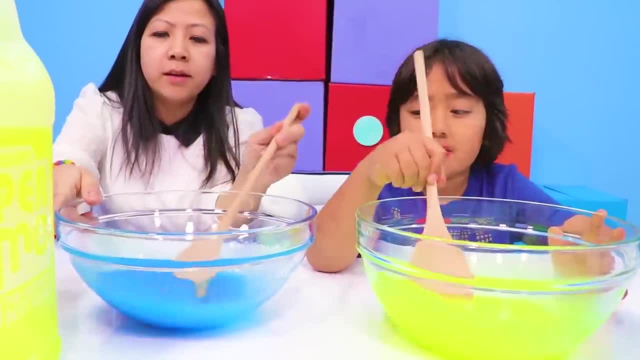 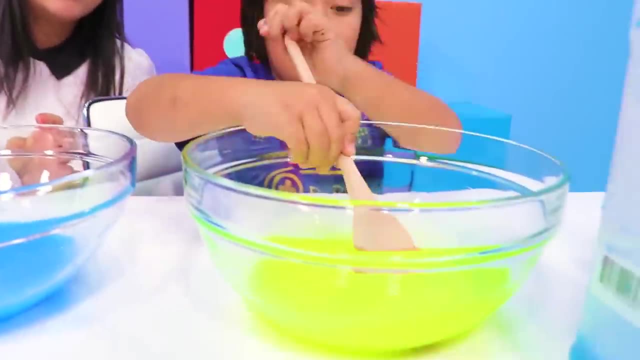 Oh, look, It's already slime for Mommy. Yeah, It's kind of already slime for me, but Look at this, Mine's just a little too liquid. Whoa, Mine's already slime. Look, Yeah, If you twist it around. 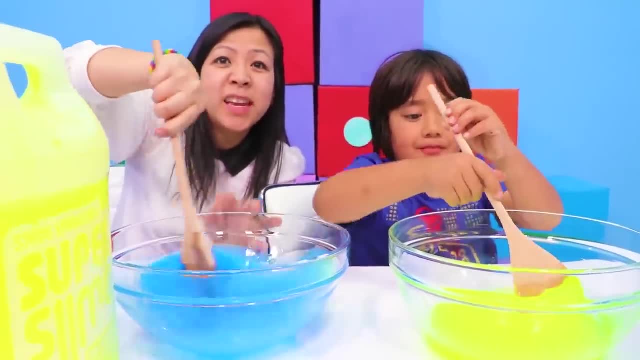 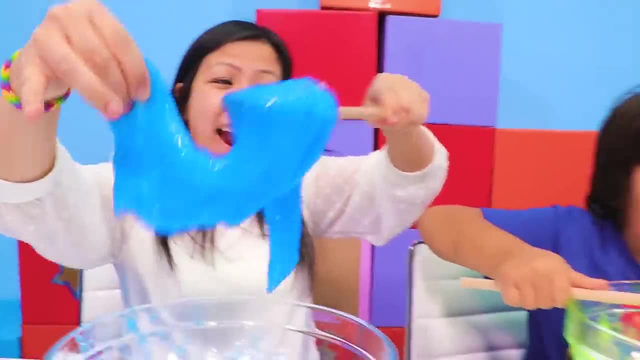 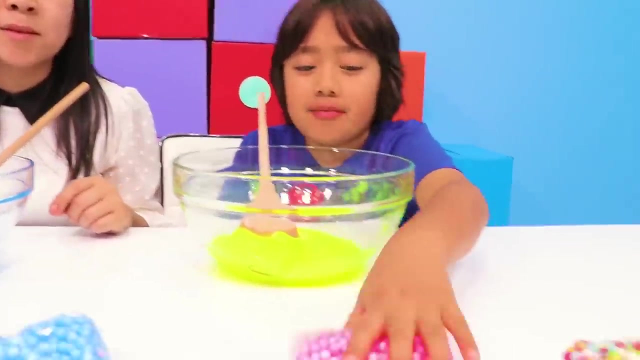 Twist it around. Okay, We're gonna just swirl for the next minute. Here's our slime. I think mine's pretty good. Look at this. Whoa. What about yours, Ryan? I like it. Next, we're gonna add stuff in our slime. 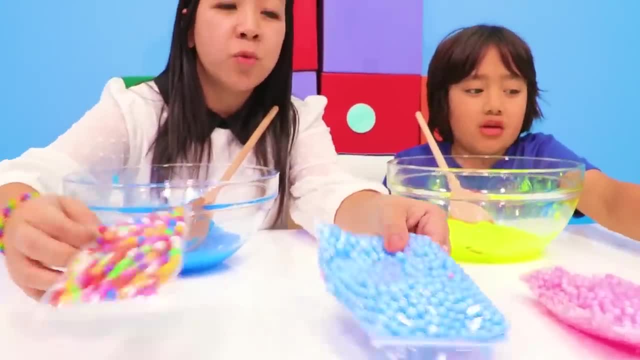 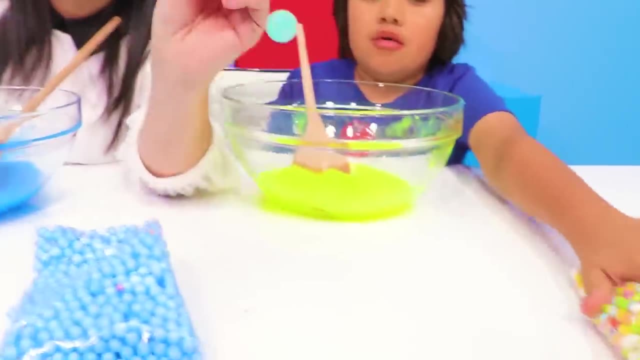 Giant foam balls. Ooh, So which color do you want Siri to pick, Ryan? So I wanted to pick this one. Okay, Well, I want Siri to pick pink. Let's ask Siri. Siri pick a random number. 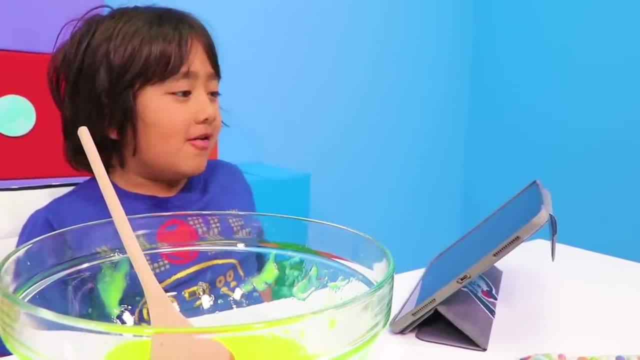 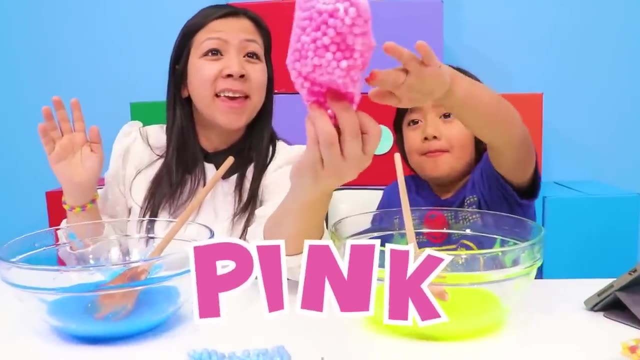 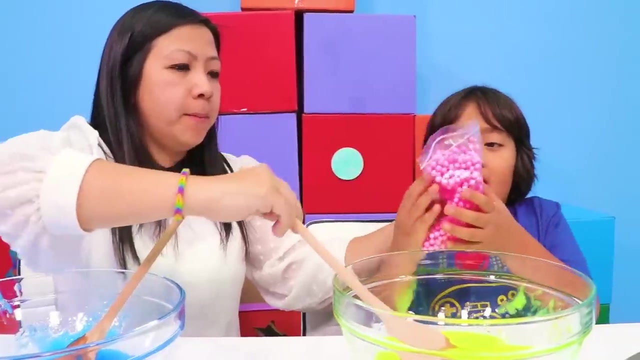 one through four, It's two. Oh, Which one is two? I got the one you wanted. Yeah, So Ryan got pink. There you go. Is that what you want? Yeah, Now I have to get really lucky with Siri if I want. 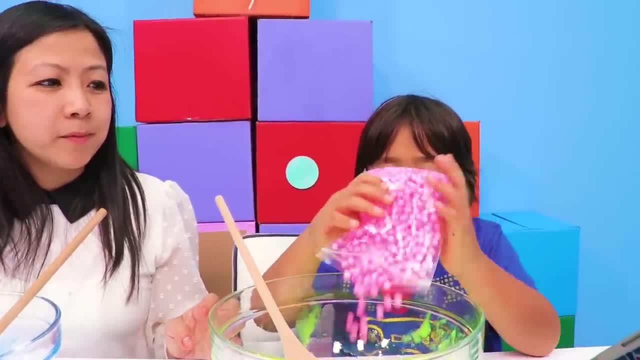 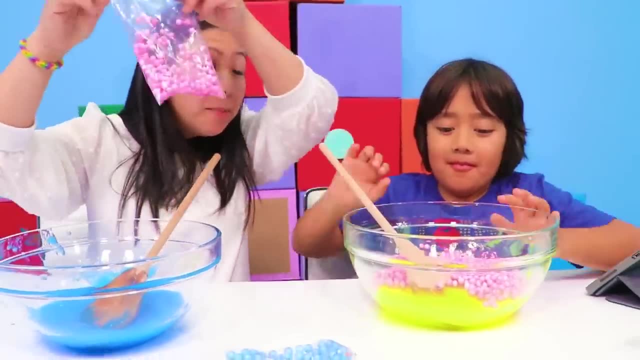 to get a good color. That's true, Alright, Whoa, I put too much Ryan, that's a lot of pink foam beads Look. So while Ryan's mixing, I'm gonna ask Siri for my color. Hey, Siri. 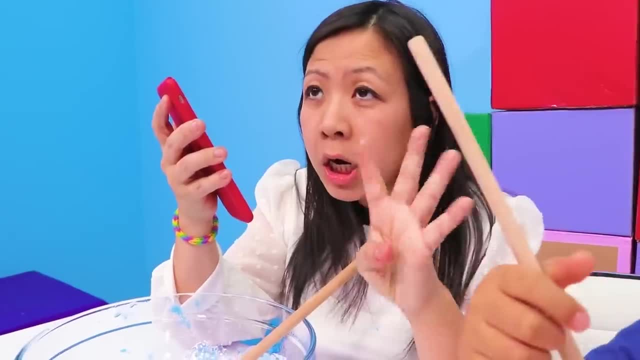 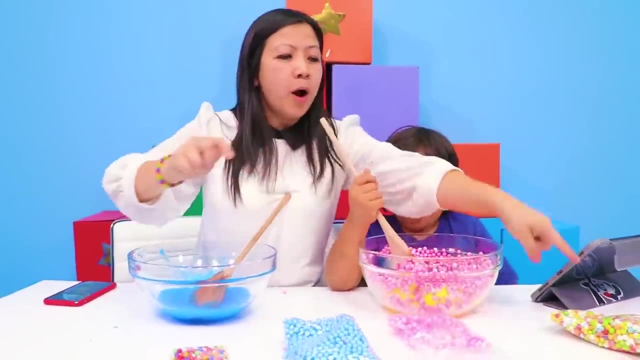 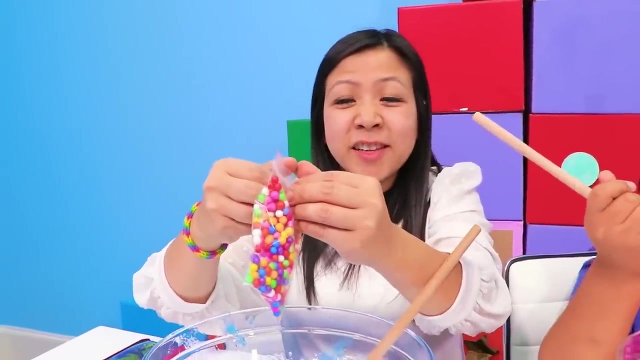 Pick a random number from one through four. A random number between one and four is four, Four. Okay, So one, two, three, four. I got the colorful one. Mine's looking good, Siri, Thank you. Here comes the foam. 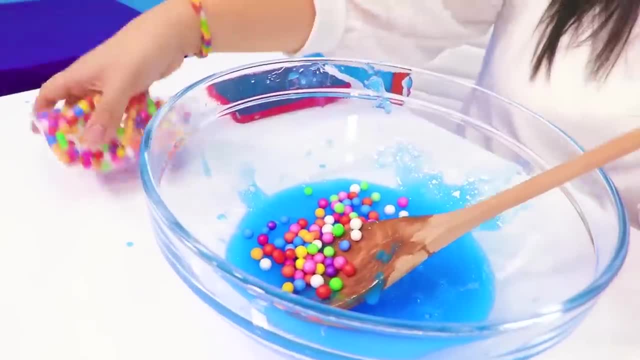 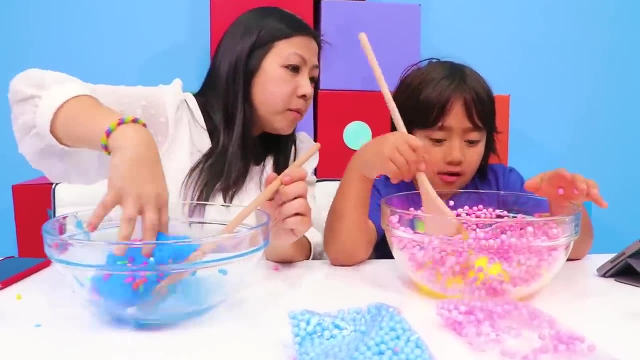 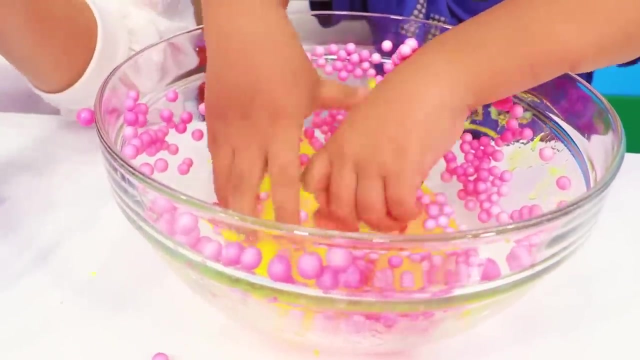 Whee, Not too much. There we go, Mixing it up, Mixing it up. Okay, So how's Ryan looking? Oh, foamy, Foamy. Which one do you like better so far? Mine or Mommy's? 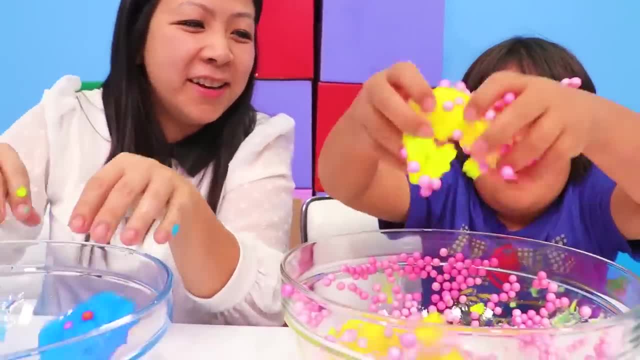 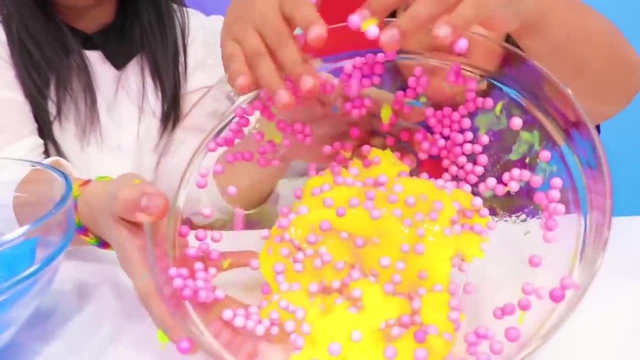 Mine. right, Ryan. Ryan has too much pink foam. I don't like mine. He doesn't like his Look at this. You guys like this? Now we have other things to put into our slime. We have this one. 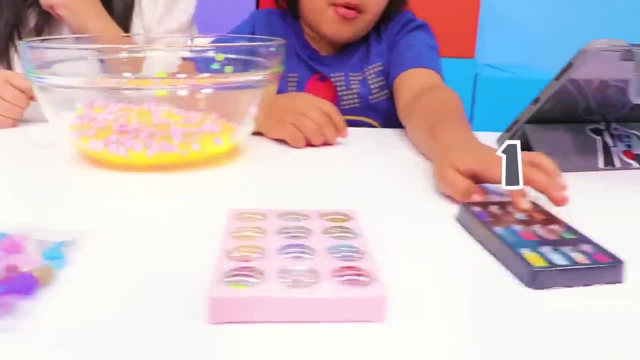 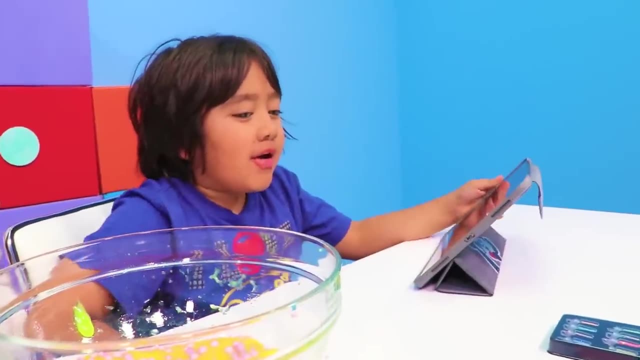 this one and this one. So this is number one, This is number two, This is number three. Ryan's gonna go first. Let's see what Siri picks. Siri pick a random number One through three. The answer is two. 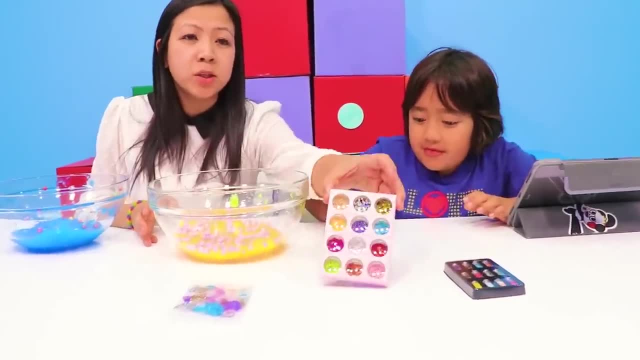 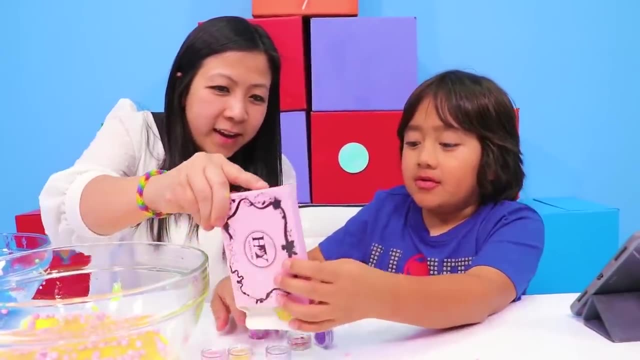 Ooh, that's a good choice. So Ryan has a whole bunch of glitter here, So that's really cool Here. I guess you can add any of this you like. I'll add this one. Okay, I pick purple. 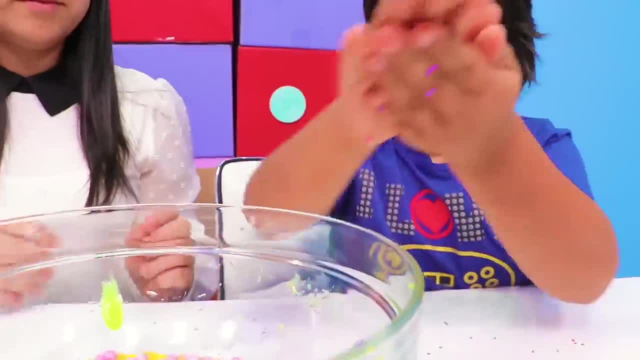 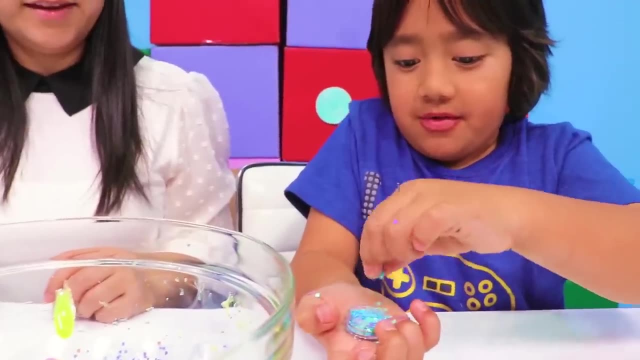 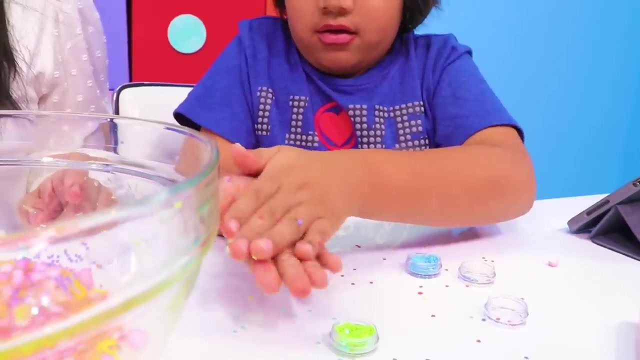 green, blue and a seashell Sprinkle. That's cute. I like the pink color, Purple, I like that, So I'm gonna get some of it. I'm gonna get some of this. Okay, Save some for me. 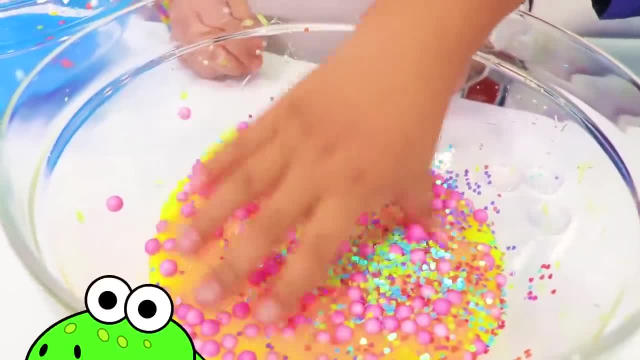 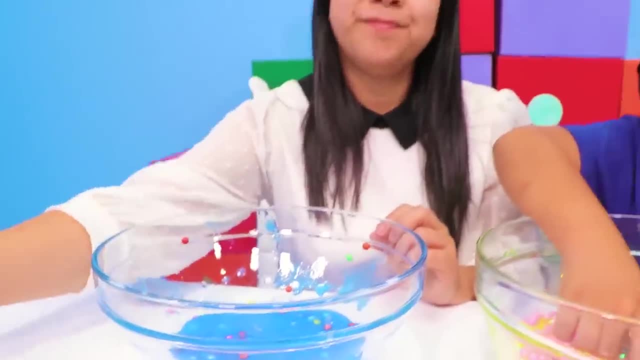 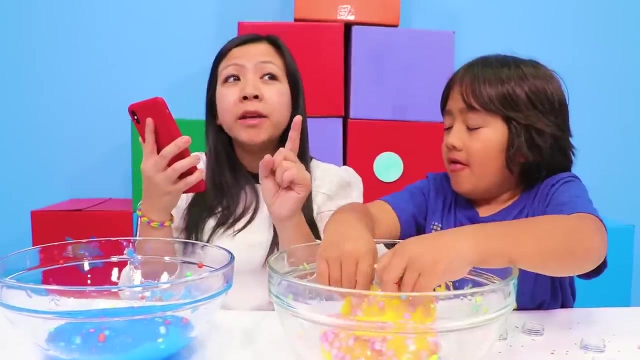 Oh wow. So there's Ryan's slime so far Looking good. It is my turn. Ryan looks pretty good so far, but I think I can beat him. So Siri time. Hey, Siri, Pick a random number from one to. 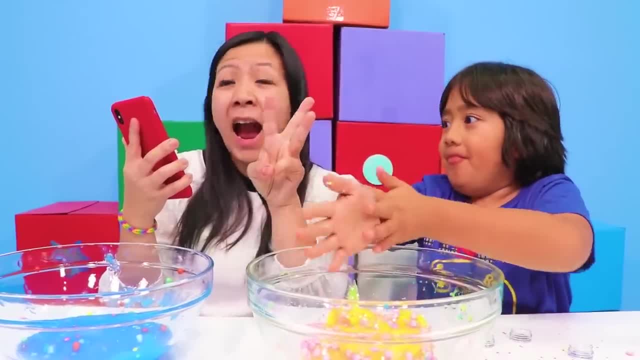 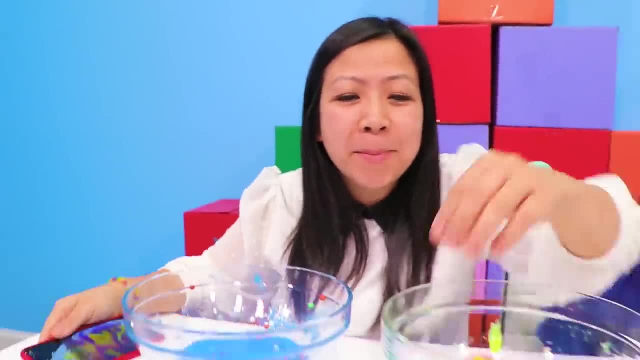 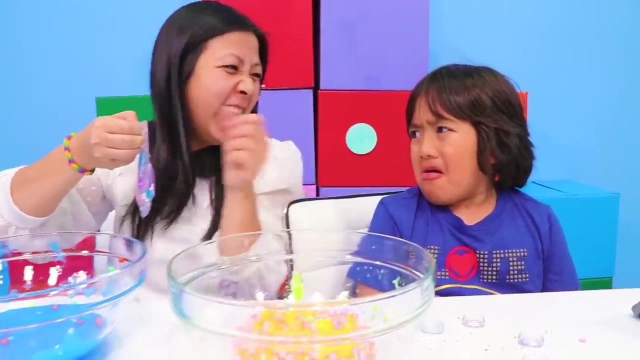 three. A random number between one and three is three. I got three. Look Three. Okay, So you know what that means. Mermaid tails for me, So excited. No, I don't think you'll win with that. Look at this. 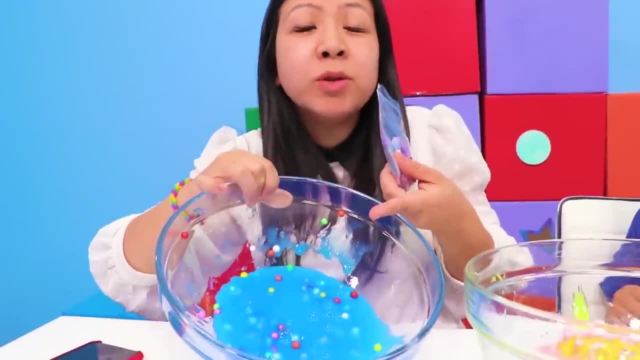 Oh wait, Look. No, It's perfect, because my slime is blue, so it looks like they're in the ocean. So that's why there's mermaids, Duh Mermaids. Look at this, It's gonna look kinda weird. 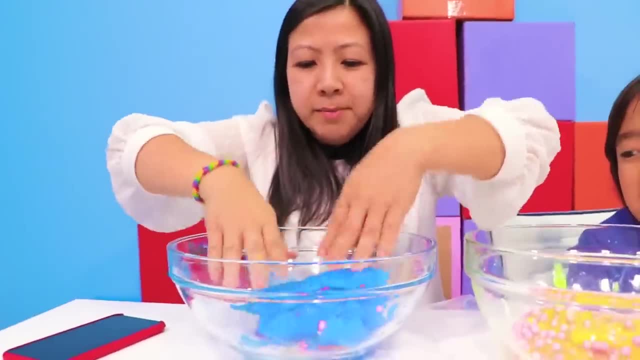 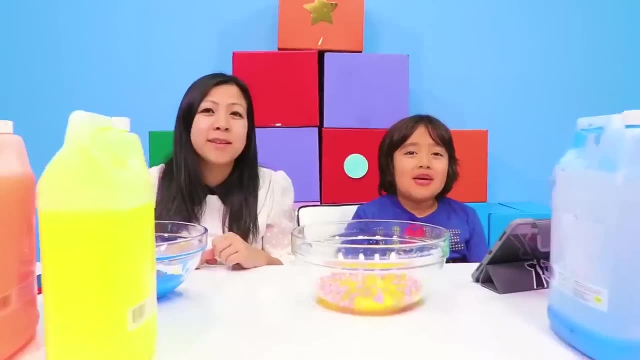 There you go. Alright, I'm gonna mix it up. Mermaids in my ocean slime- How can you mix it up? It's literally plastic. There you go, Bam, To make it fun, Siri's gonna do a second slime color for us, So it's gonna make mine look. 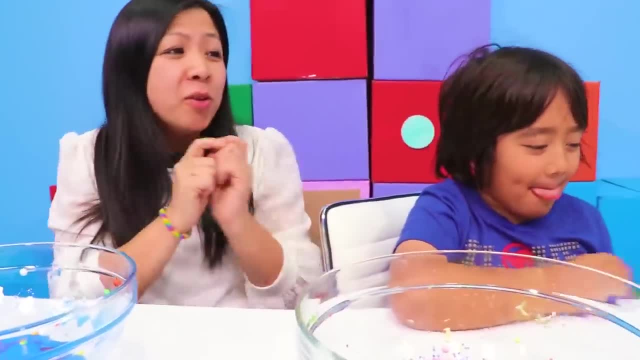 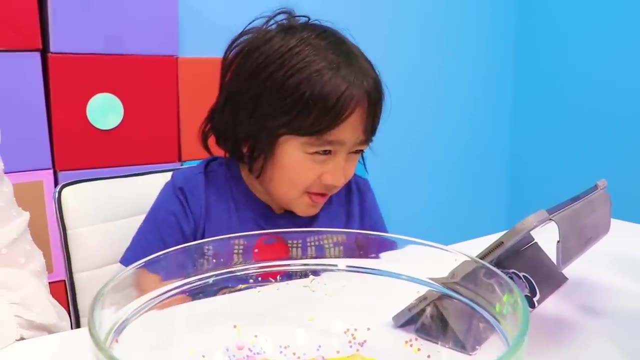 better and Mommy's look worse. We'll see about that. Okay, Ryan, You go first. Hey, Siri Pick a random number One through six. It's five, Whoa. So Siri picked five for Ryan. Let's see. 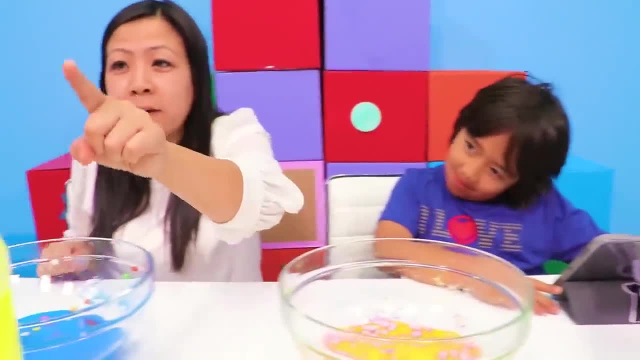 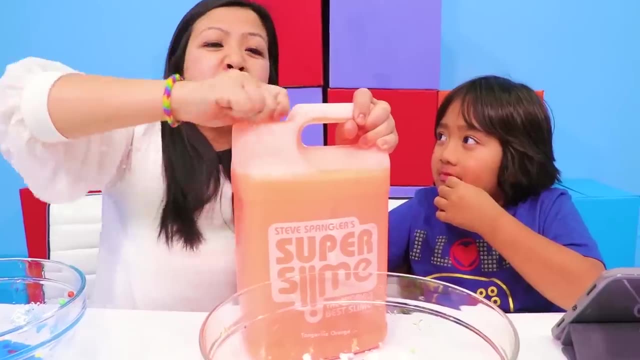 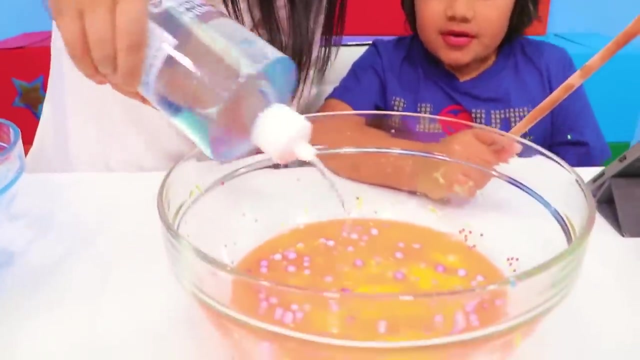 One, two, three, four, five. Ryan, you got orange for your slime. Yay, Tell me when to stop Stop. Give Ryan some activator solution There. it is Alright Time to agitate, Alright, Okay. 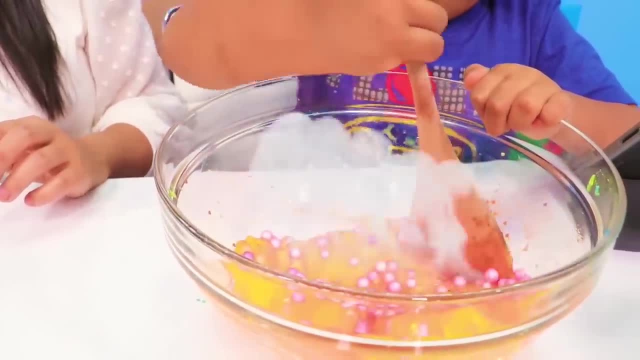 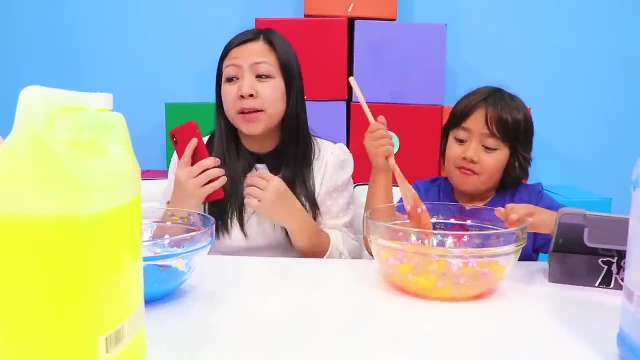 Whoa, It looks like a. It looks like you're cooking something While Ryan is mixing his two colors. I'm gonna ask Siri to pick my color too. I hope Siri picks green. So Siri, pick number six, please. 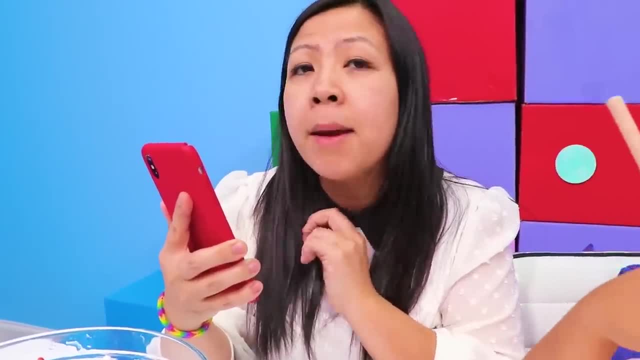 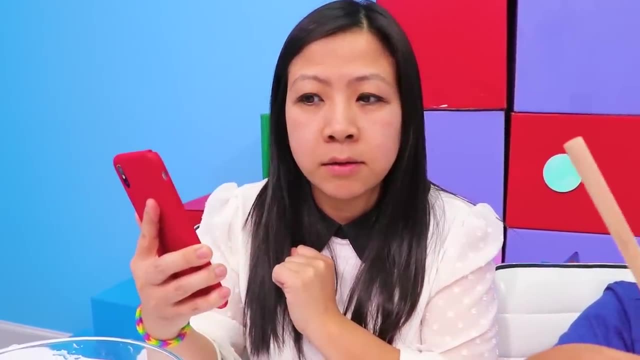 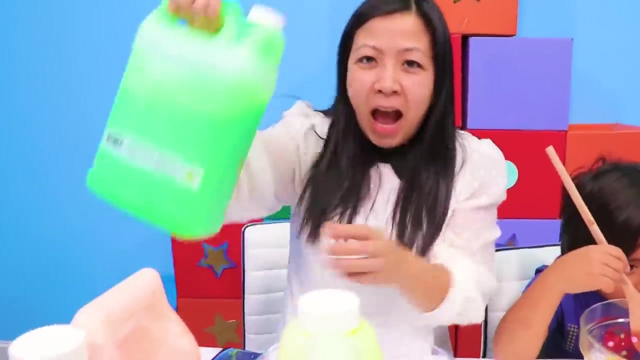 Hey, Siri, Pick a random number from one to six, A random number between one and six, six. So Siri says six, Yay, I got six. Whoa Yay Green slime, Whoa My orange kind of makes like an outline, Oh I. 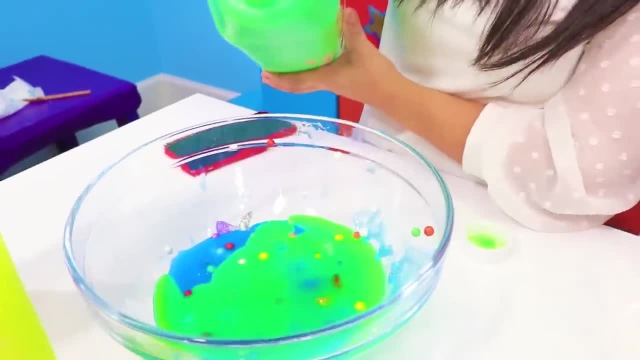 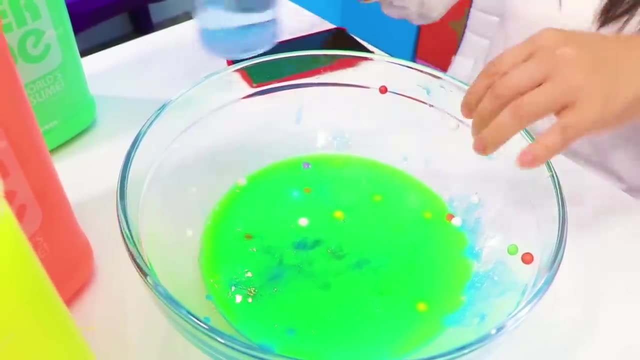 like yours, Ryan. Yours looks good. Whoa, Look at this. Whoa Activator into Ryan's. I'm putting activators into mine. Whoa. What do you guys think so far of these two colors? Is it pretty? Did Siri do a good job of picking? 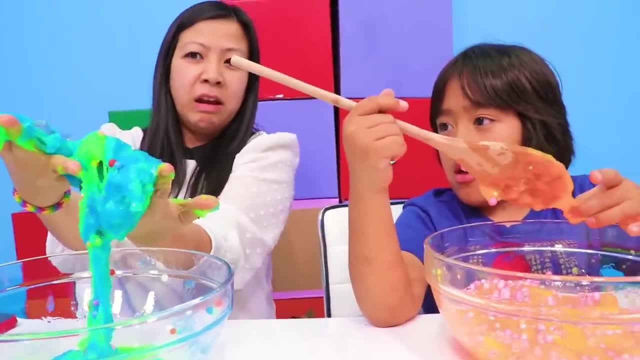 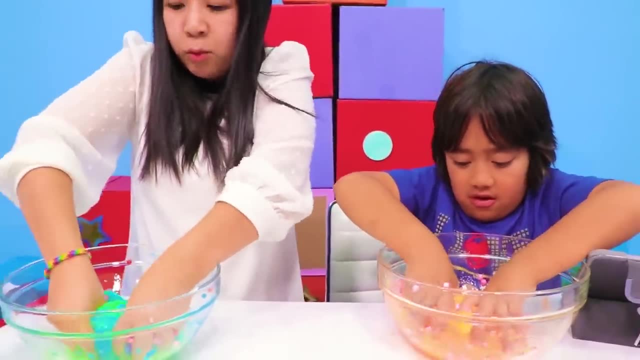 my colors. What do you think, Ryan? Is this a winning color? Oh, There's a hair in my slime. We're both using our hands. Let us know which slime is better. Here's mine so far, Here and here is. 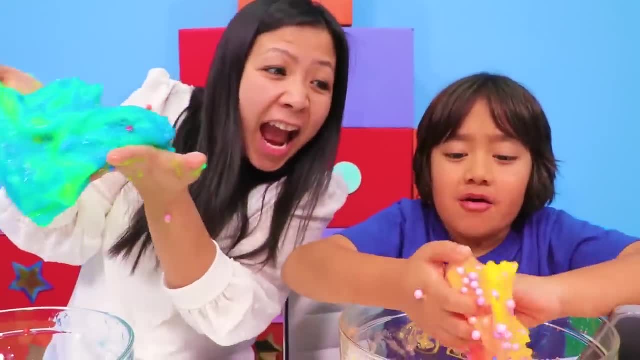 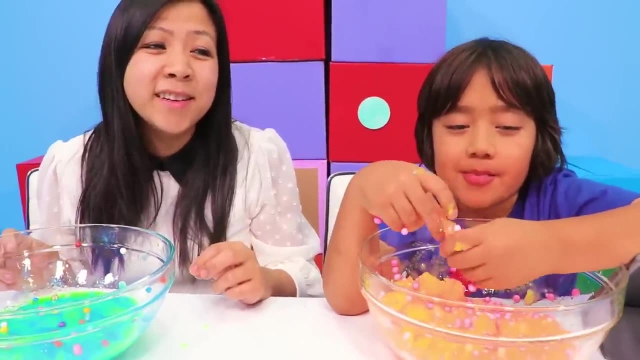 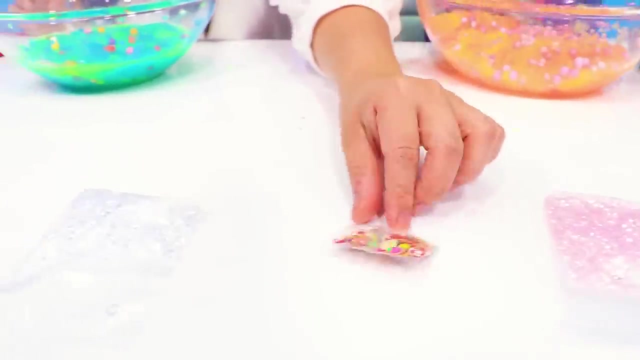 mine so far. Who's better guys? Mine's yellow with an orange outline, Ooh Whoa. And here's some more toppings for Siri to pick: Blue beads, some really cool unicorns. some pink beads, some cute little watermelon fruit. 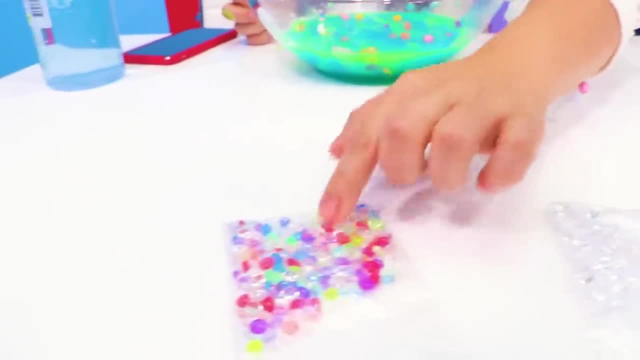 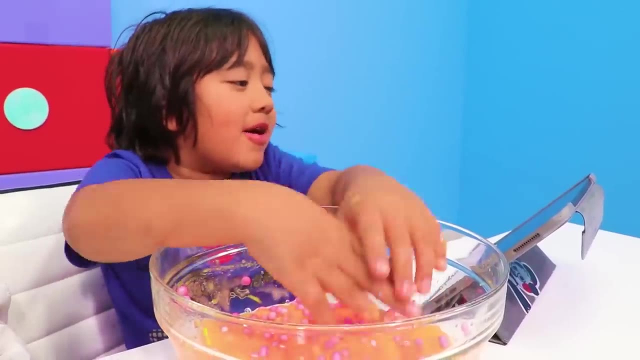 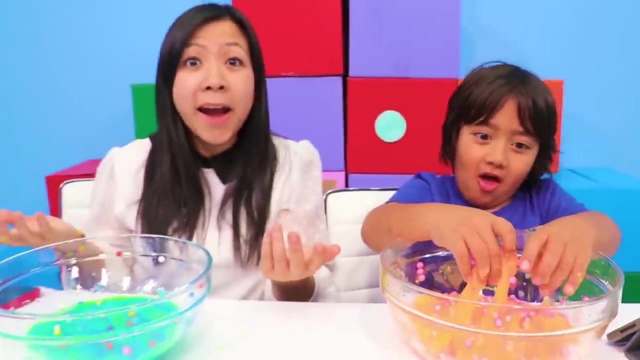 things: some clear beads and some rainbow beads. Pick this one, Siri. Yeah, I want six or one. Okay, All right, Ryan's first, Siri. pick a random number One through six. The answer is one One. 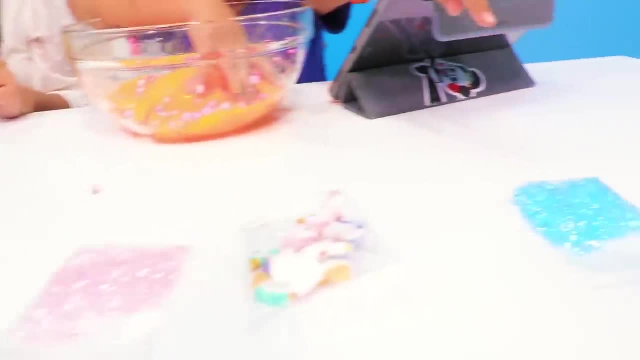 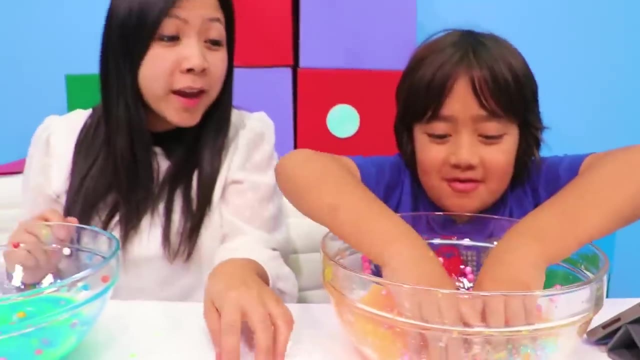 So what did you get, Ryan? I got the blue one. Nice, I'm gonna use all of it. Whoa, The whole thing. Yeah, sure, So not too. I don't know if it's even enough, anyways, Yeah. 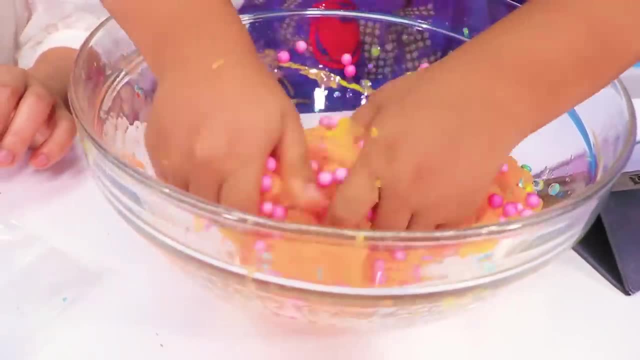 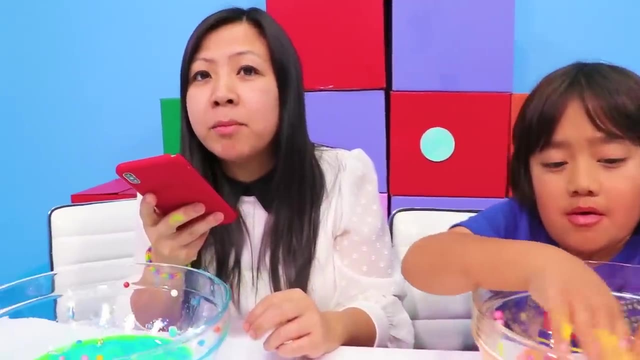 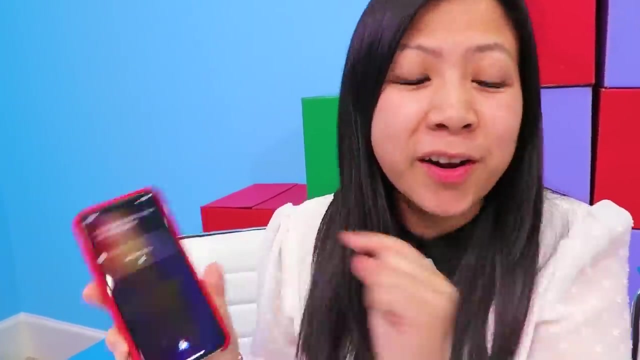 Yours just looks orange. now, While Ryan's mixing, let's pick mine. Hey, Siri, Pick a random number from one through six. A random number between one and six is four, Four, Okay, So Ryan was one. He used it all. 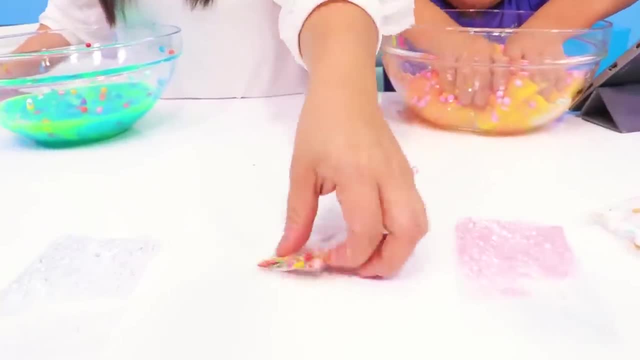 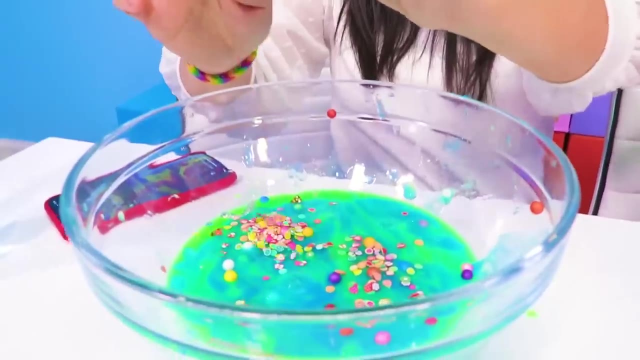 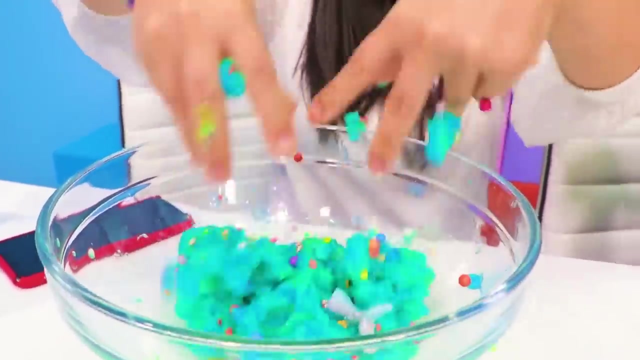 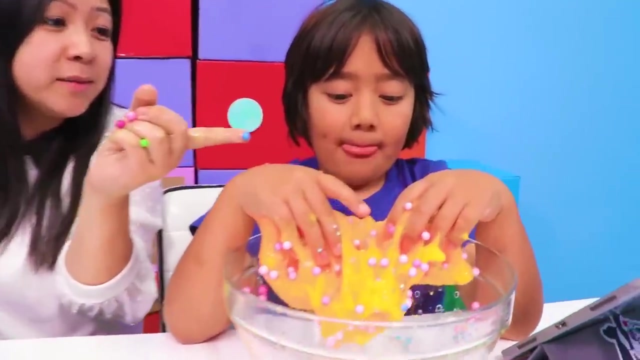 Two, three and four. Oh, What are these? Okay, Dumping the whole thing in Mix time, So crunchy. Okay, guys, I think we are done. Tell us which Siri did a better job: Ryan's Siri or?